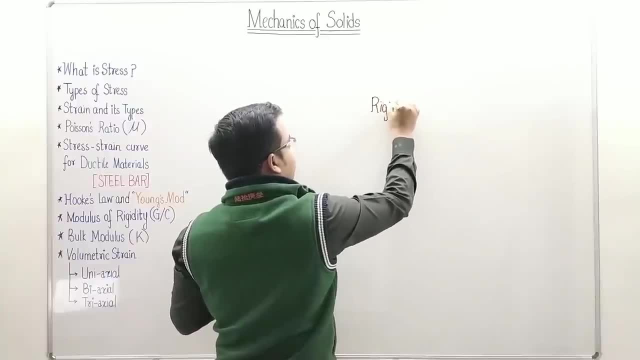 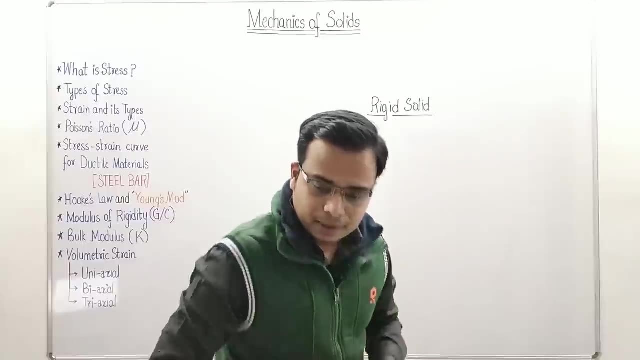 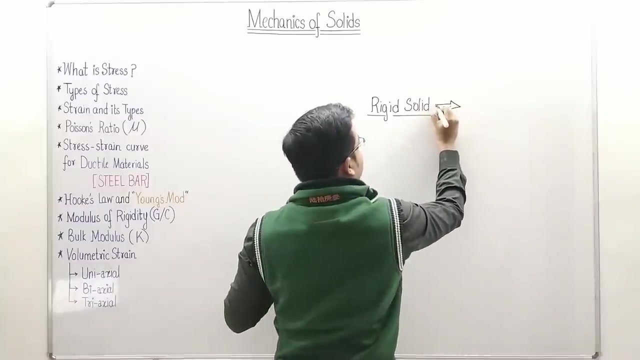 described as a rigid, solid, Rigid, solid. Okay Now guys, I'm pretty much sure that in your first year of engineering you must have gone through engineering mechanics, And in engineering mechanics- let me just write this: engineering mechanics, or applied mechanics. 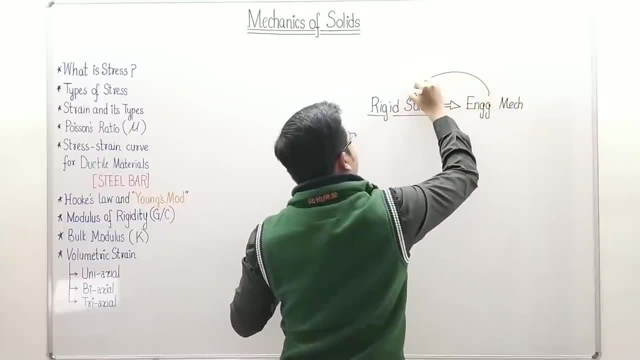 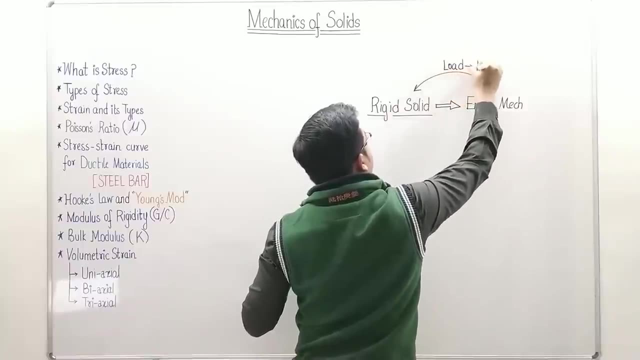 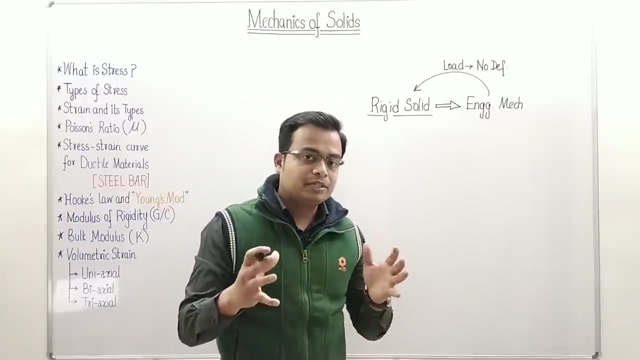 Okay, Here we studied about rigid solids. That means whenever we applied the load, whenever we applied the load, there were absolutely no deformation. Okay, So if on applying a load there is absolutely no deformation, then that particular case falls in the category of rigid. 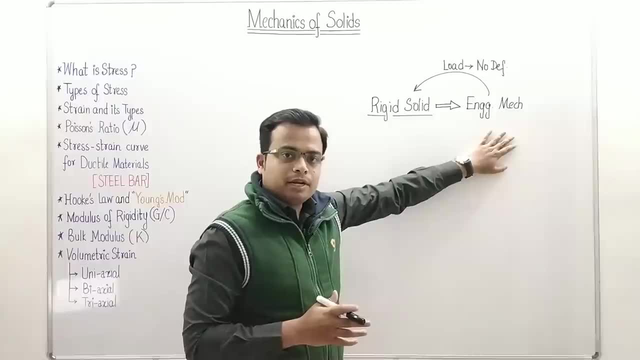 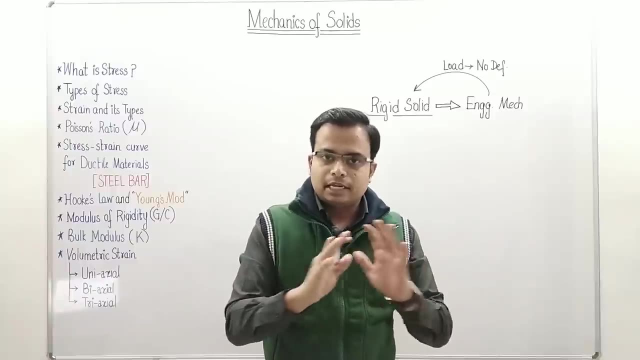 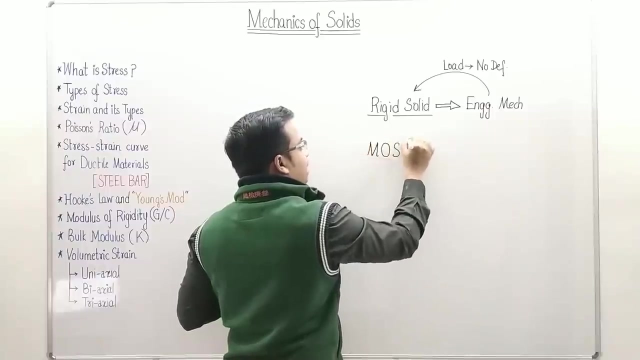 solid or engineering mechanics. Right, So in engineering mechanics, basically, whenever you applied a load, whenever you applied a force, no change in shape and size of the object takes place, That's for sure. But as far as mechanics of solids is concerned- I'm writing this in short- Or mechanics of materials M-O-M, Or 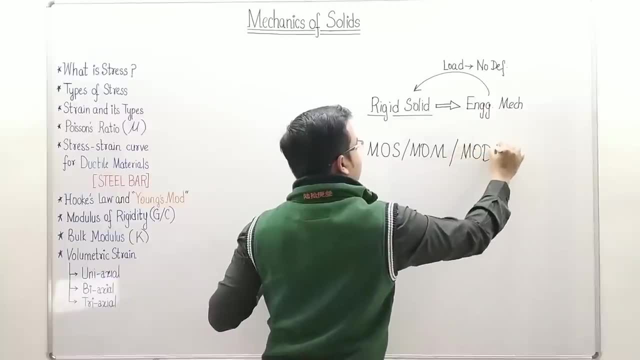 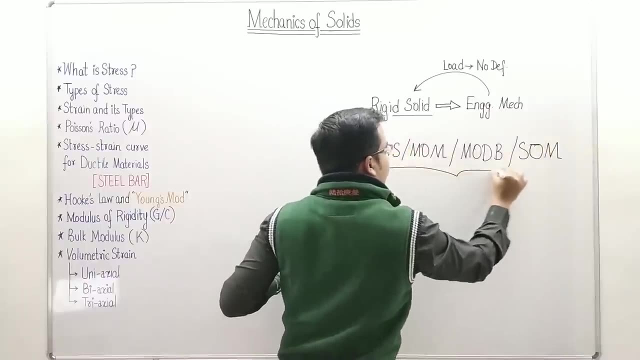 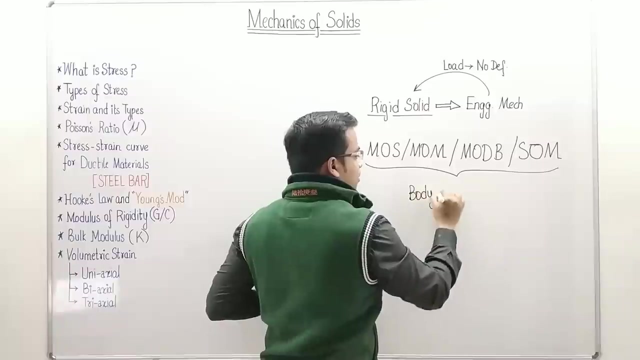 mechanics of deformable bodies is concerned, Or strength of materials- SOM- Some people call it SOM In all of these cases. well, they pretty much mean the same thing Here: the body is deformable. That is the main element which differentiates this engineering mechanics from. 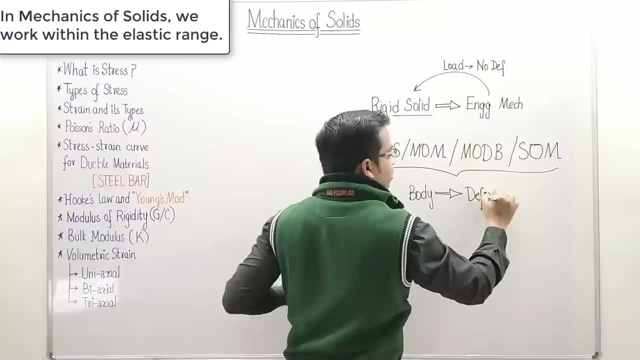 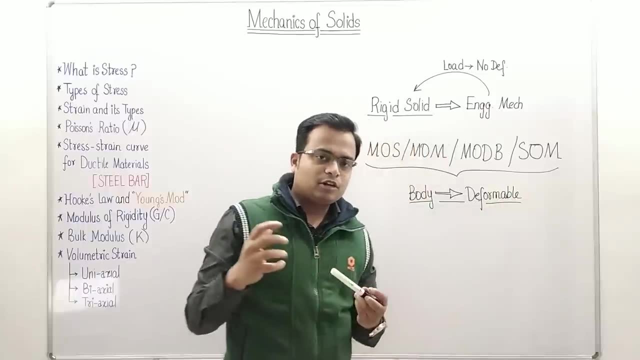 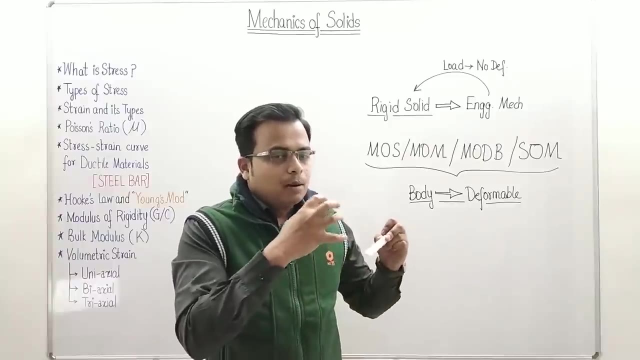 mechanics of solids. Here, the body that we are going to take into consideration is a deformable body And, as an engineer- whether you're a civil engineer or a mechanical engineer- it becomes extremely essential to know, on applying a particular amount of load or magnitude of load. 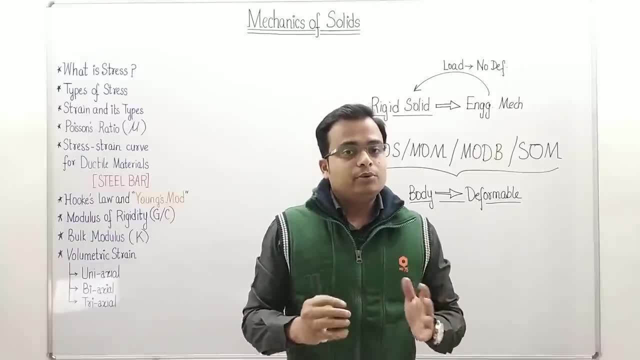 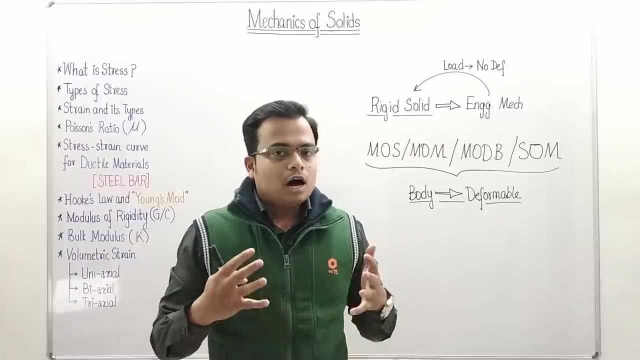 you should know how much deformation is going to happen. So in engineering mechanics, you should be able to know how much deformation is going to take place. Okay, Or in a very general sense, you should be able to realize, you should be able to work out how much load. 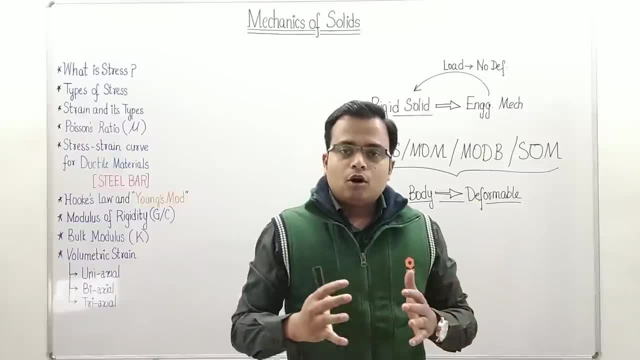 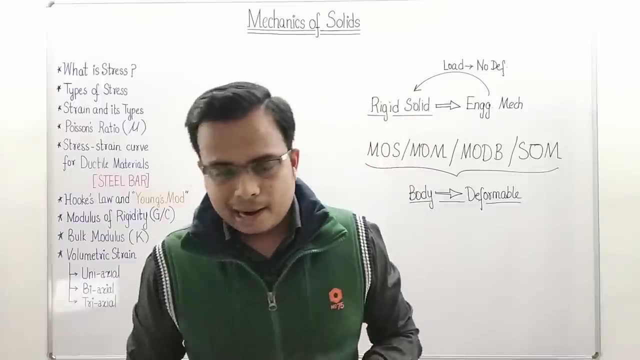 does, does a particular machine element or a structural member is able to withstand? All these things are extremely important. Now let's take this session forward, And the first thing that I'm going to talk about is the different kinds of loads, which are. 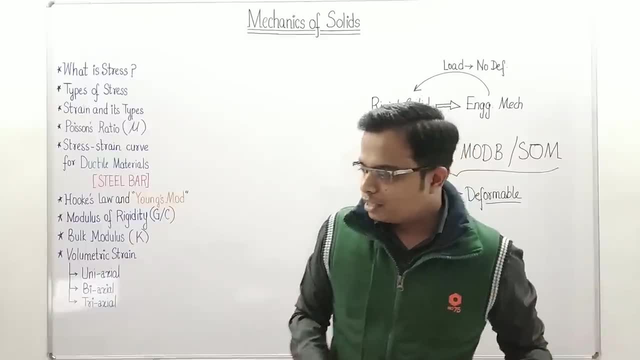 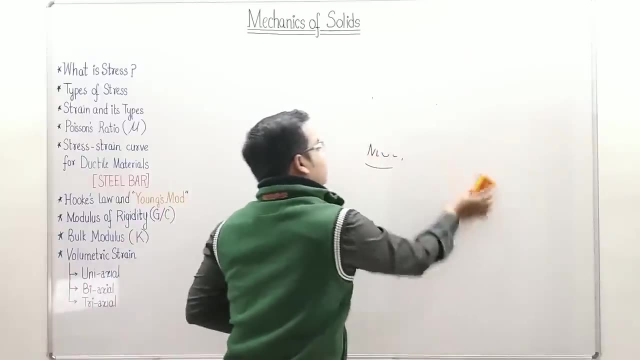 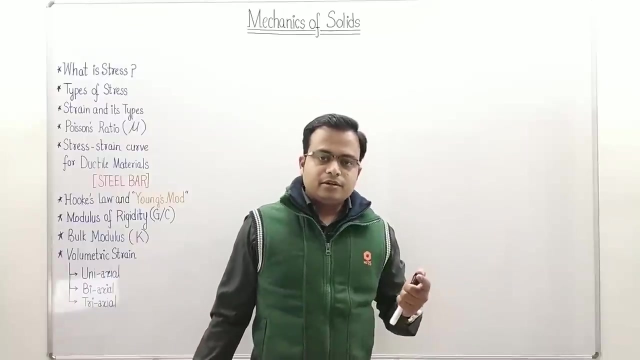 applied on the rigid bodies, or even deformable bodies, for that matter. So let's take this session forward, and here we go Now. some of you guys may be wondering as to why we are learning this course Now. as an engineer, you will come across designing, and whenever you want to design. 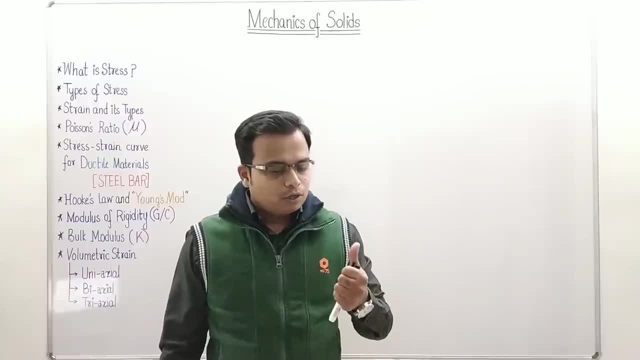 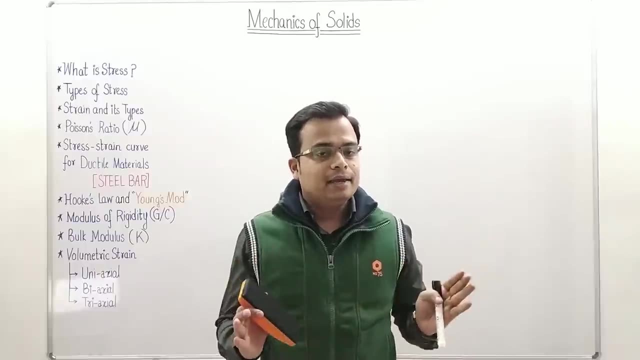 something, be it a machine part or even a structural member, you've got to make sure that your design- number one- is safe. second, it is durable. that means the active life period is quite high. and thirdly, it has got to be economical. so you have to check all of these points and only then. 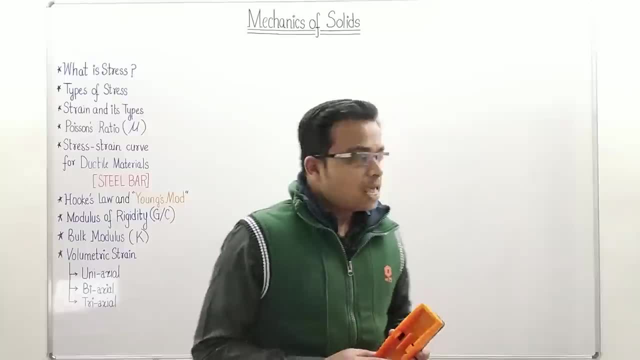 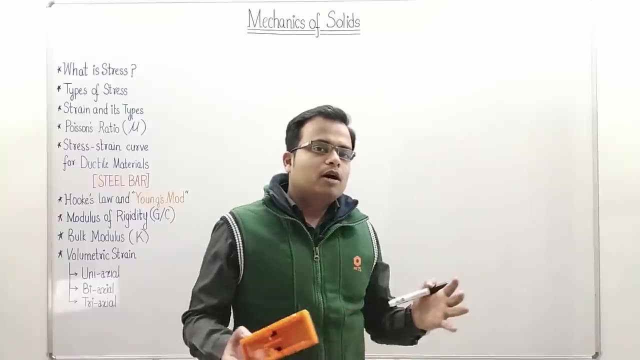 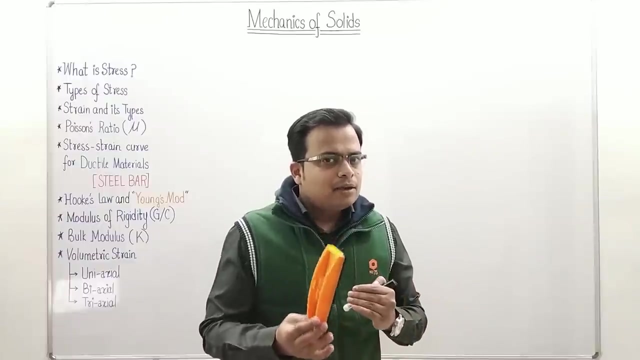 your design should be sanctioned. So that's the entire idea behind learning this course. Now, here we'll try to apply loads on different solids, different objects, and we'll try to work out how much deformation takes place- okay, both along the direction of load and also perpendicular to the 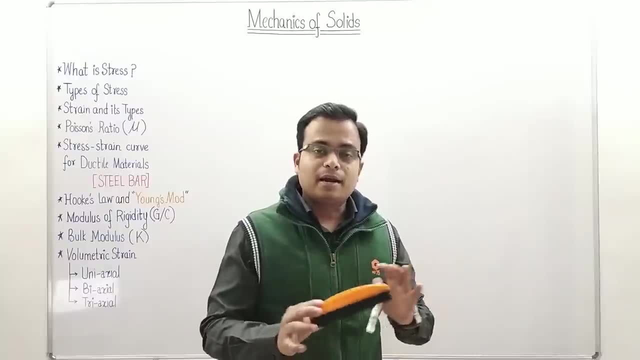 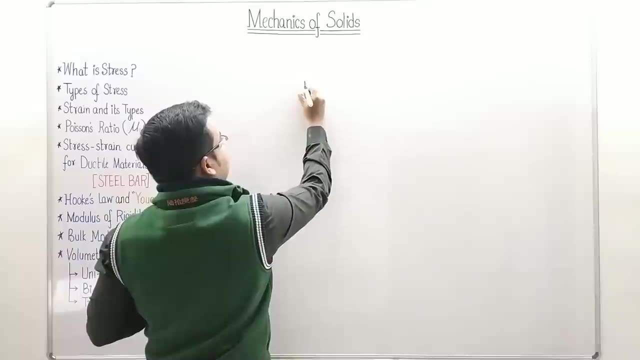 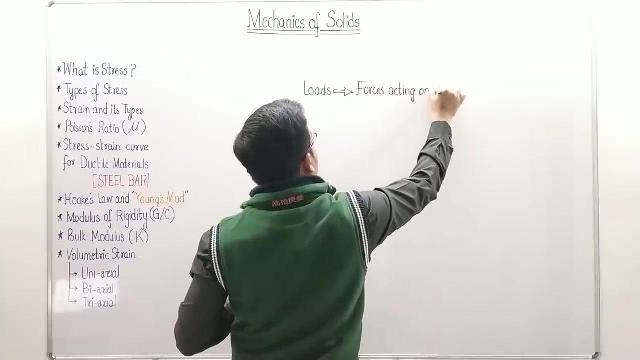 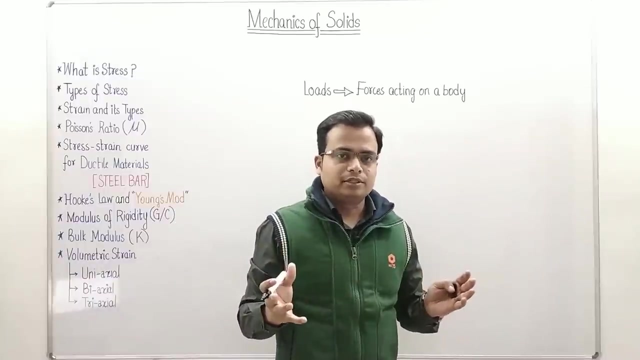 direction of load. you'll eventually realize how all of these things pan out. Okay, the first thing is loads. What are loads? Loads are nothing but the forces acting on a body. okay, so whenever a force acts on a body that is regarded as a load in the environment of mechanics of solids, you can see and specifically we'll be. 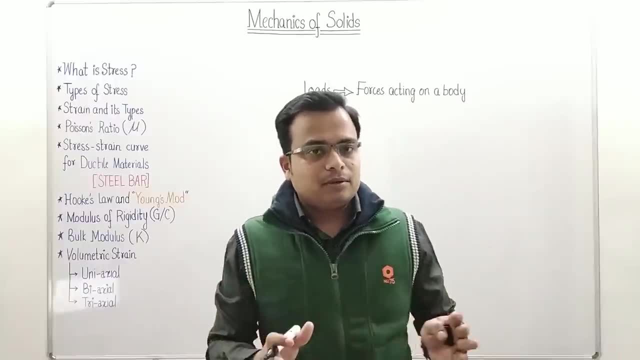 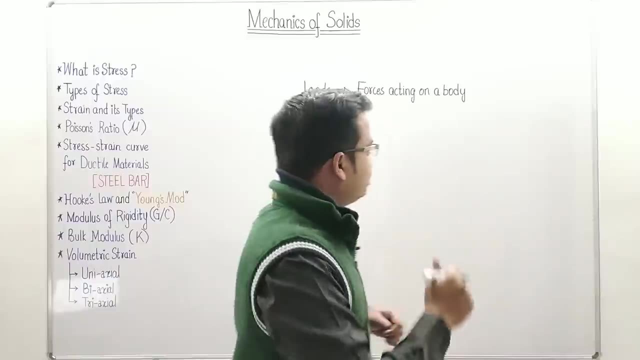 dealing with loads, although they mean the same thing, but in the environment of mechanics, of solids we will be dealing. we'll be calling all the forces loads In the form of loads, so what exactly they are and what are the different types of loads. let's say: 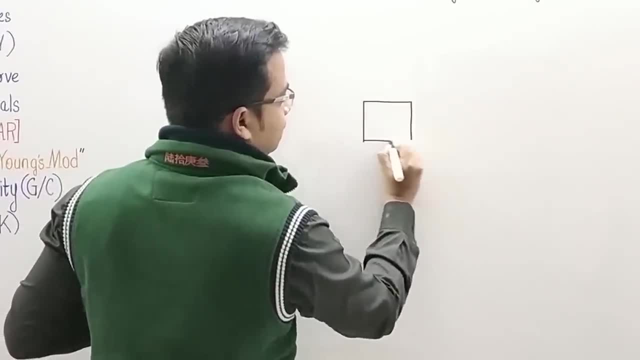 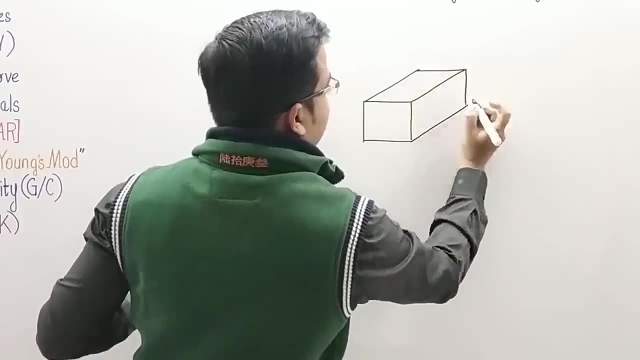 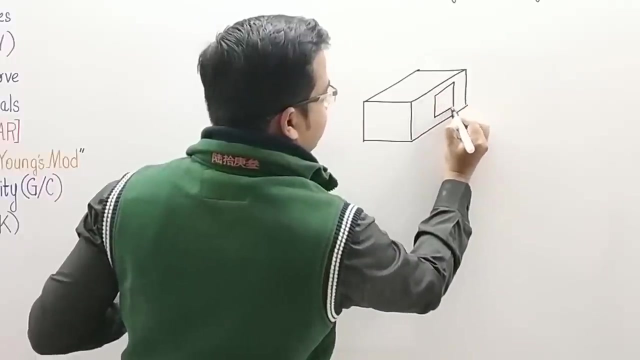 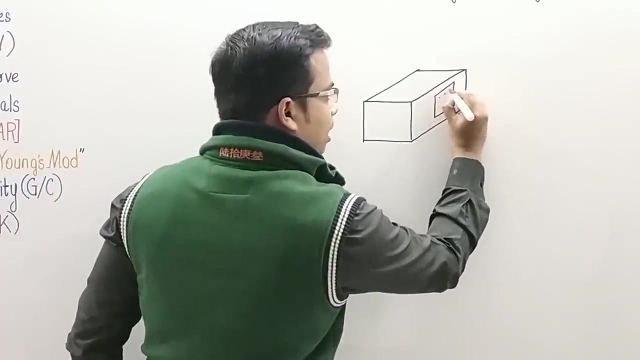 we've got a cube over here, not a cube, but a cuboid. let's say yeah, and what I'll try to do is just take into consideration this much amount of area. so what's happening in this area? let me just use a different color. what's really happening is: there are different points, okay, and 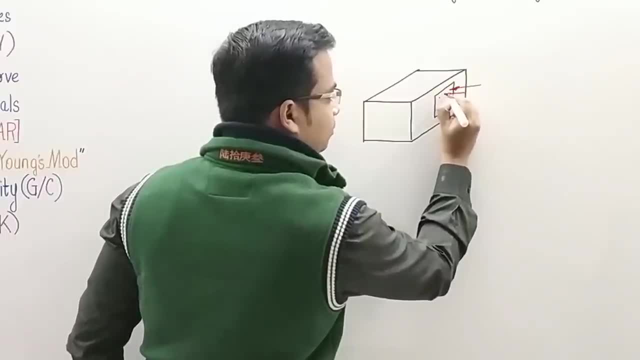 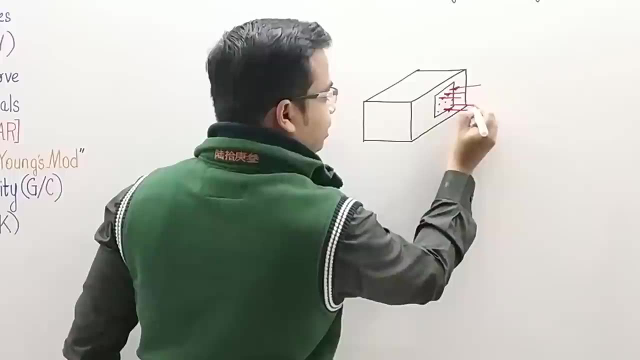 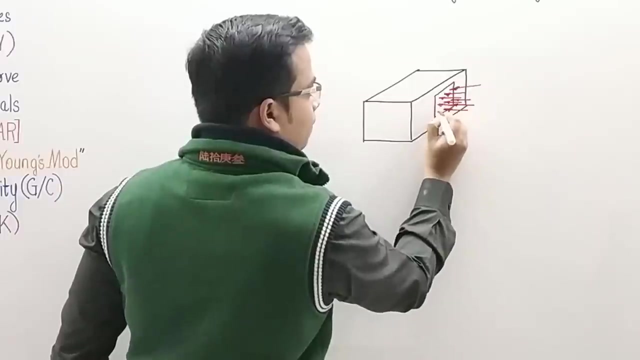 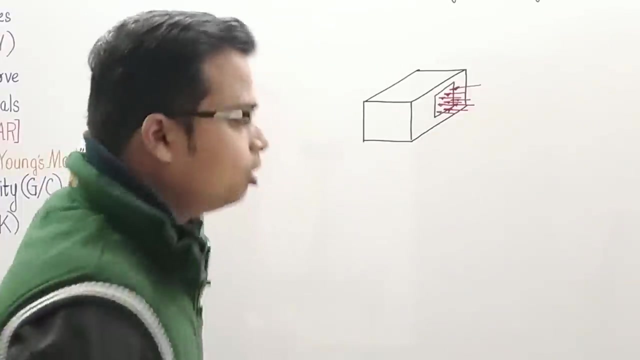 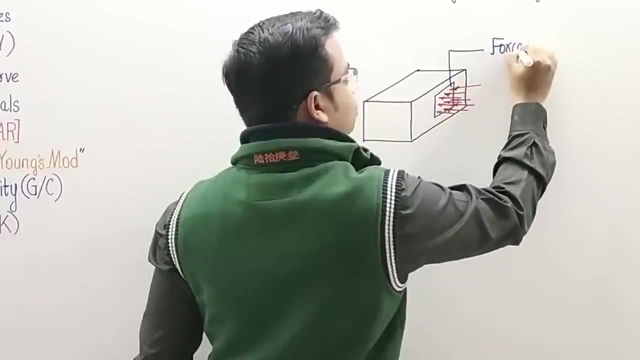 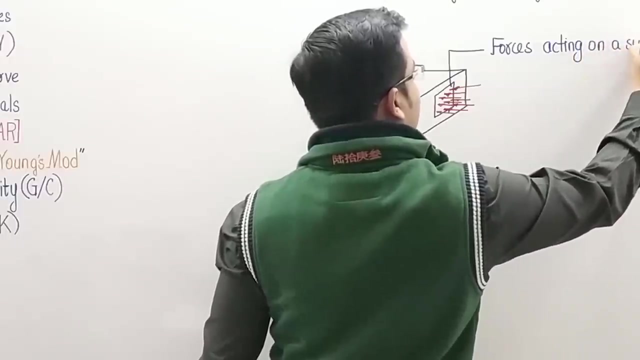 all those points. there are forces acting here, also here, here, here, here, here, everywhere forces are acting right. so all these forces actually are acting on a particular area, so all these forces are acting on a particular area, Force is acting on an area or acting on a surface, and hence all these collectively can be represented. 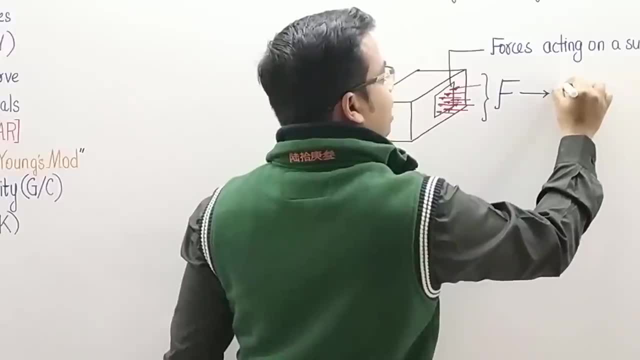 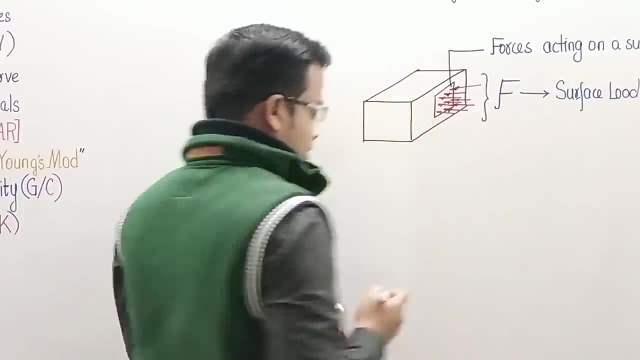 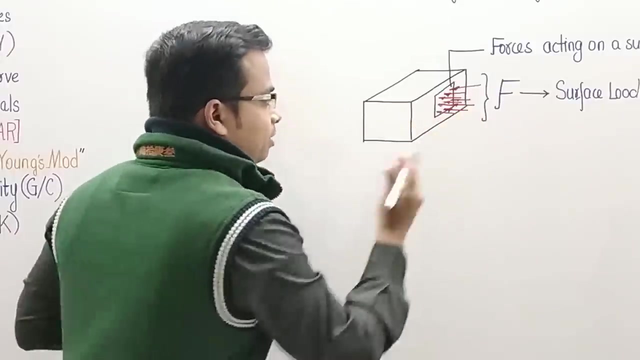 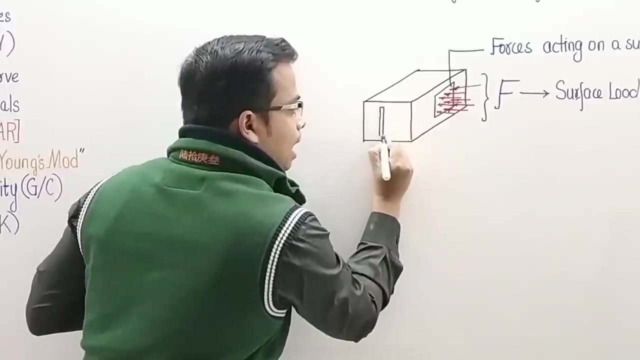 by one larger force, which is basically referred to as a surface load, right, so that's surface load point. okay, and that's the area. Now, if the area becomes narrower, then the case would be something like this: okay, and here, if the force acts, what happens? let me just show you. it would be something. 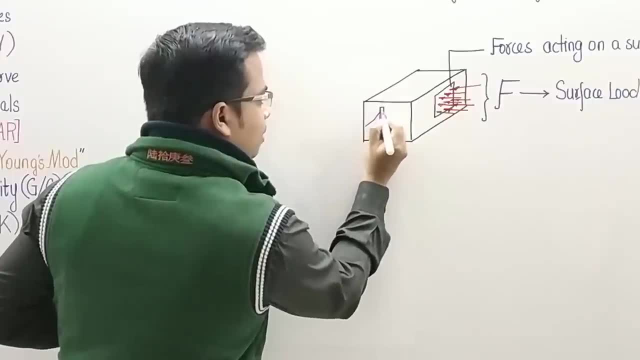 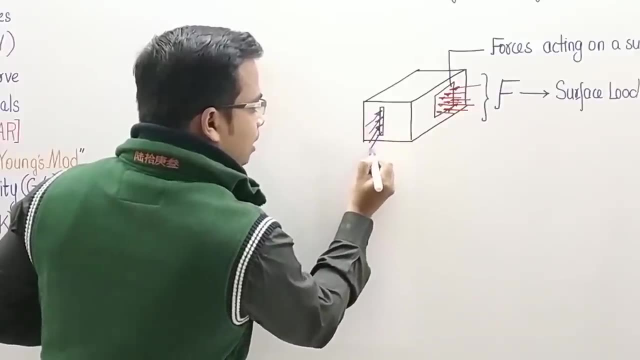 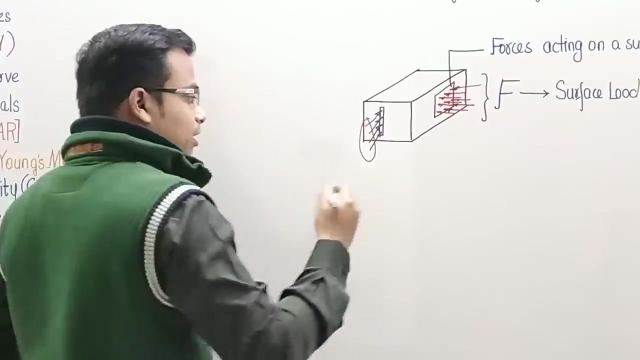 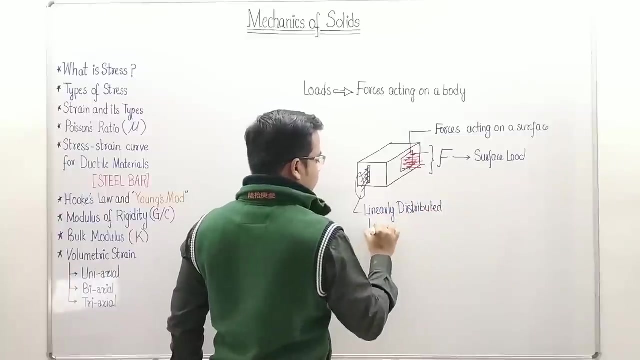 like this- let me have different points over here- like this: all the forces are acting here also and here. so this arrangement of force, this collection of force or this bunch of force, is what is referred to as a linearly distributed load. now, guys, just think about this. what happens? 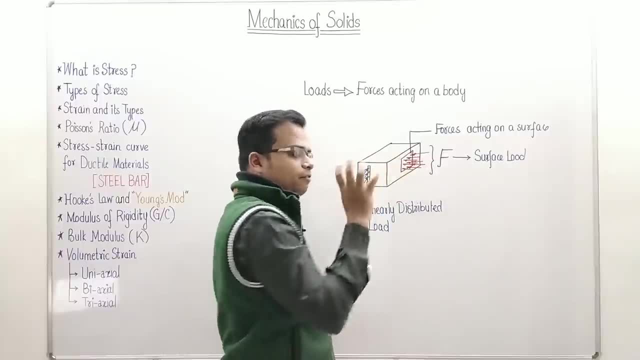 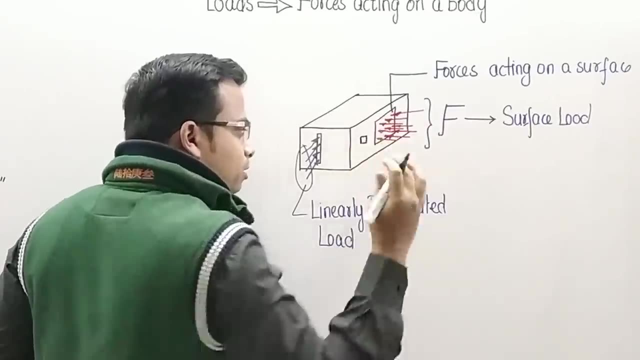 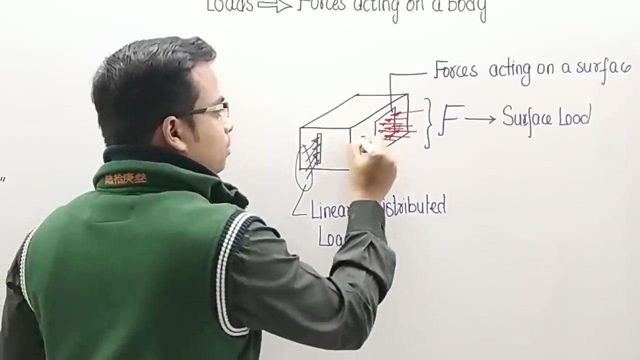 if this surface becomes very small? this is surface a. if it becomes very small, what will happen? so, when this becomes very small, let's say this: much smaller. okay, just zoom into this. it becomes this, much so on. In that case, only one force will concentrate like this. Only one force will. 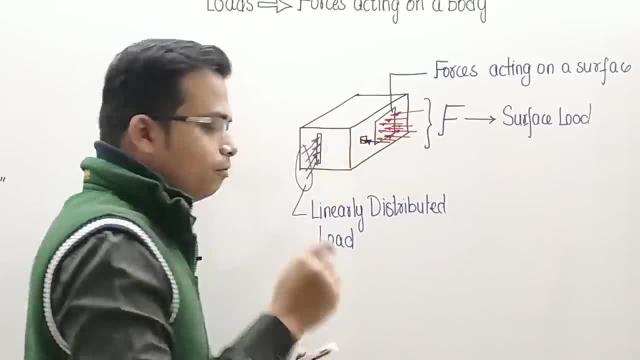 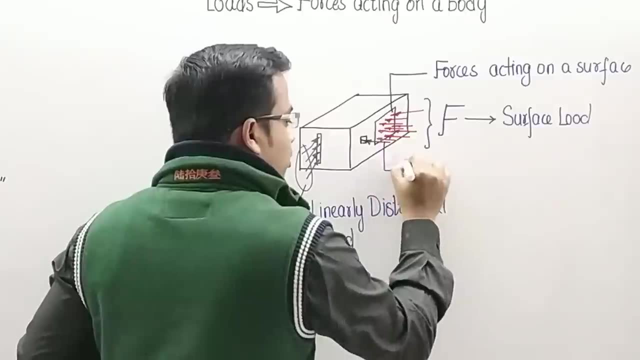 be concentrating like this, And hence, when there is only one force and when the area is very, very small, it absolutely becomes a point. In that case, that sort of a load is what is referred to as a point load, And it can also be referred to as a concentrated load, since it is concentrated. 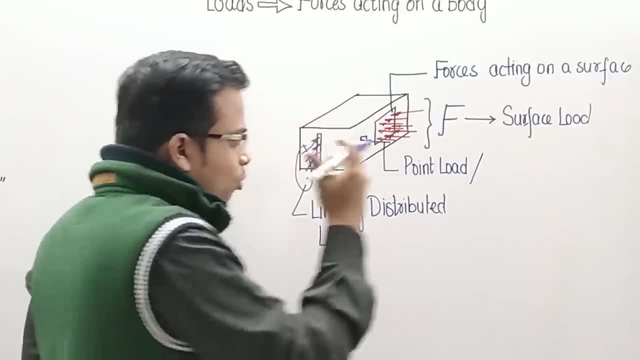 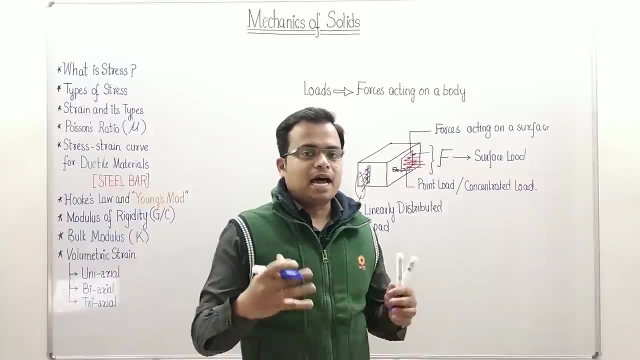 on a particular area, very small area, okay, or a very small point, Okay. now there is something which we refer to as axial load, Okay, and there is something which is also known as an eccentric load, So let us just go through them, Okay, but before that, 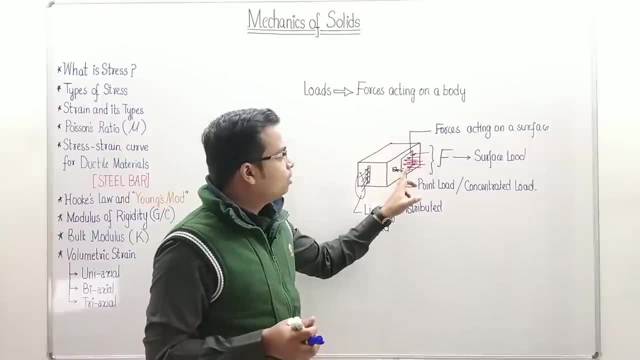 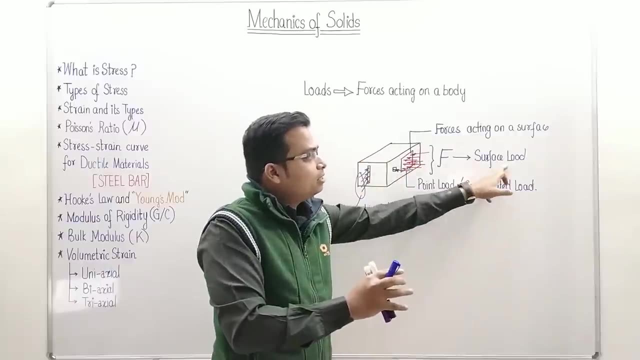 let me just revise this, recapitulate everything. So load: if there are a bunch of forces acting on a particular surface- okay, bunch of loads acting on a particular surface- then that would be regarded as a surface load. And if you've got a bunch of forces along a very narrow area, 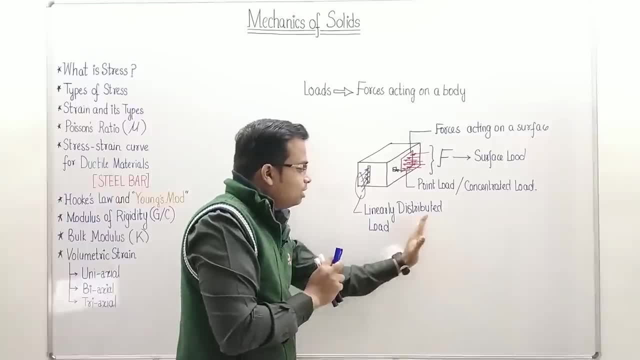 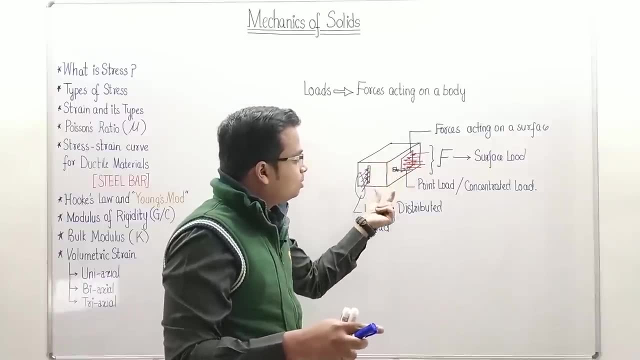 almost linear, then they are going to be considered as a surface load, And if you've got a bunch of forces, then they are referred to as linearly distributed load, And this is something which you will see in case of beams right, And then if the area becomes very small, then obviously 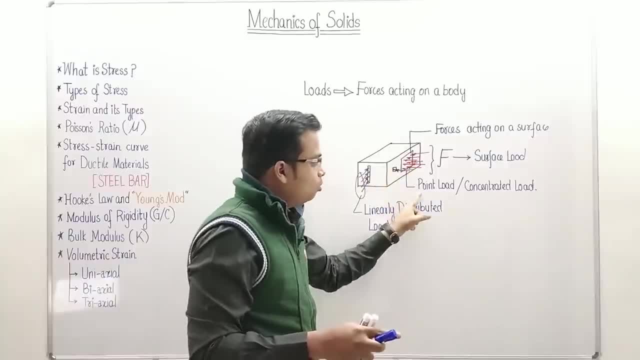 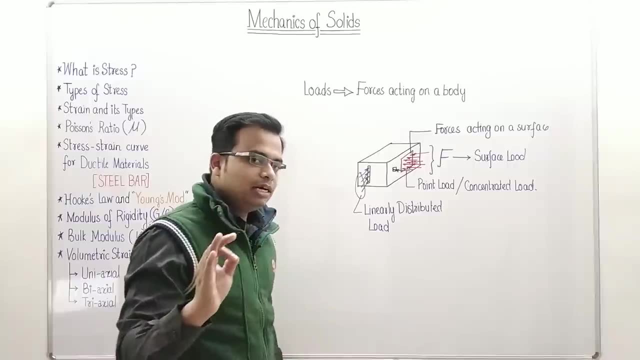 obviously the load is going to be single, or a point load, or a concentrated load. all of them mean the same thing. Okay, so that was all about the different kinds of loads. Now let me just go ahead and tell you what exactly is the meaning of an axial load. 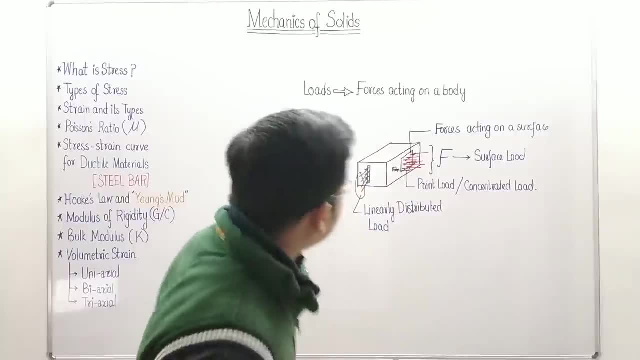 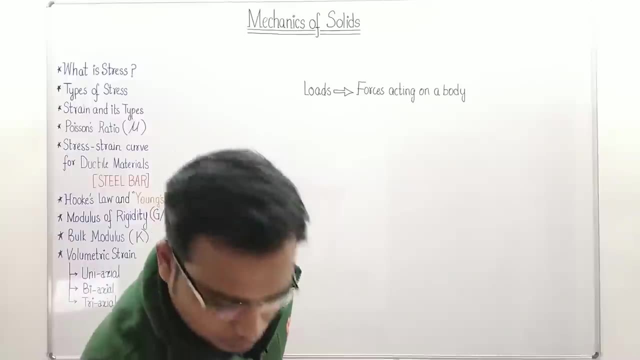 And how is it different from an eccentric load For that? well, I need to wrap this. Here we go Now. what I'll try to do is: let me have a vertical member now, And it's something like this: let me just draw this: 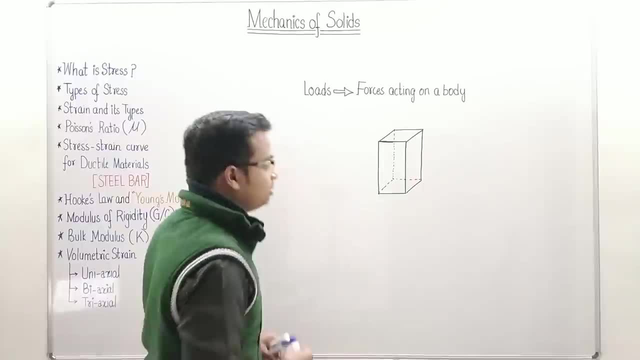 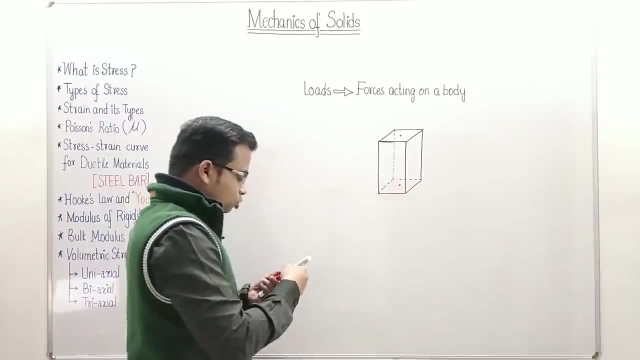 So, guys, the case is like this. let me just show you if I can just have the center point of this square above. let's say, we have the center point like this And we have a center here also, And if I can just join these two centers with the help of a line. 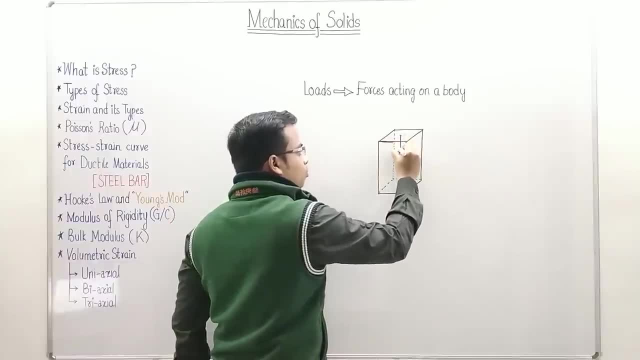 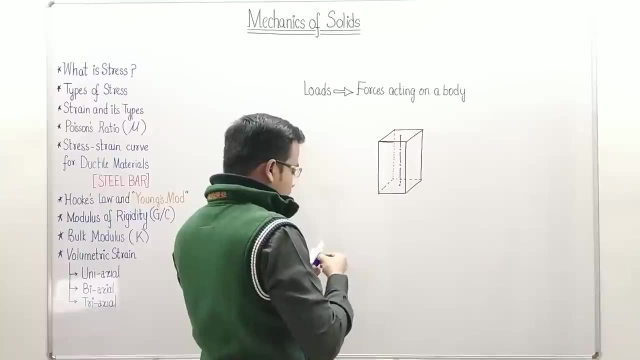 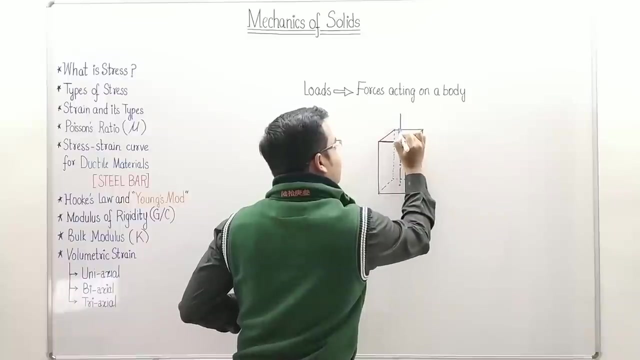 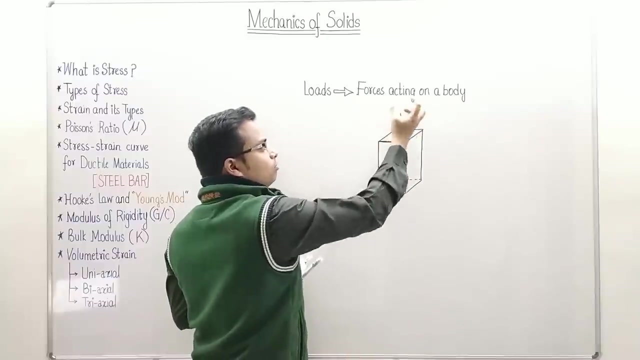 purple color. this would be qualifying as the axis. Okay, Right, That's the axis. So if a load is acting along the axis like this, like this, then this load is. the nature of the load is such that it is going to pass through. 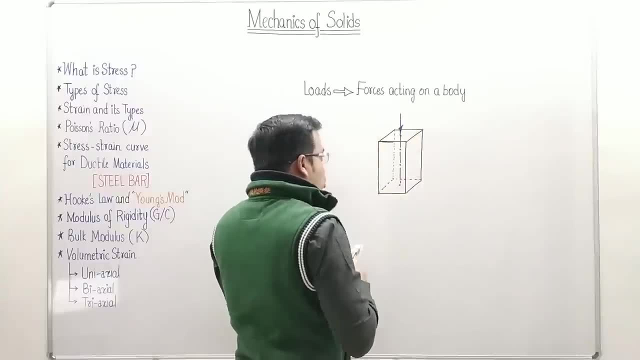 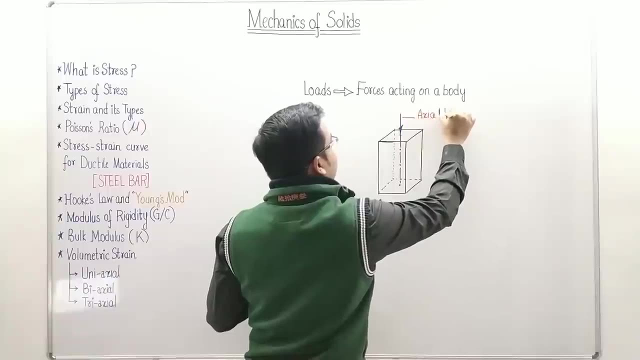 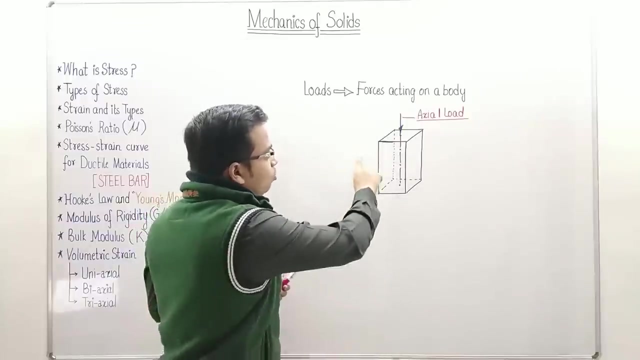 the entire axis, isn't it? Such a load is what Is referred to as an axial load. Now you guys might be wondering what exactly is an eccentric load? So let me just show you if the load is not axial, if it is at a certain distance away. 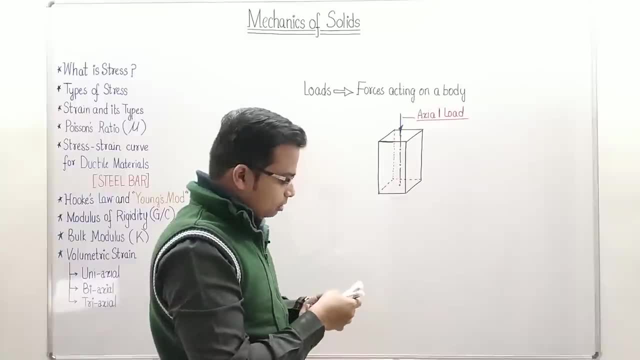 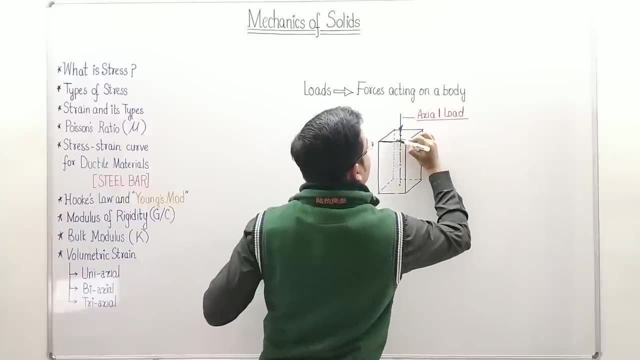 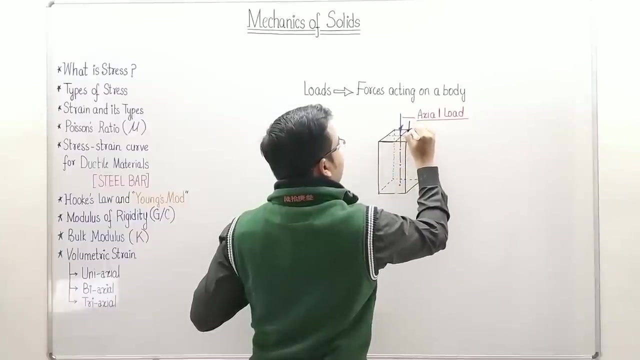 from the centroid, then it is an eccentric load. It's something like this. Just zoom into it And let me just show you. if the load is not here, Instead the load is okay, something like this, Somewhere here, Right, Then this load is what is referred to as an eccentric load. 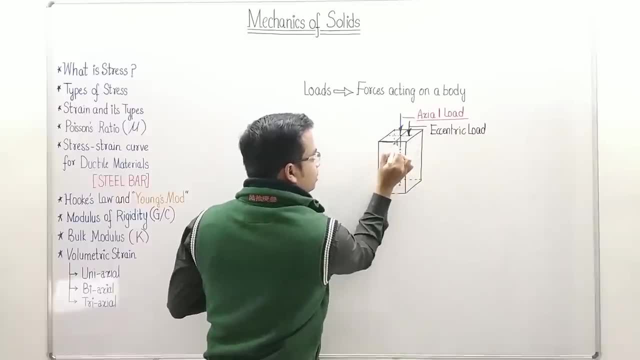 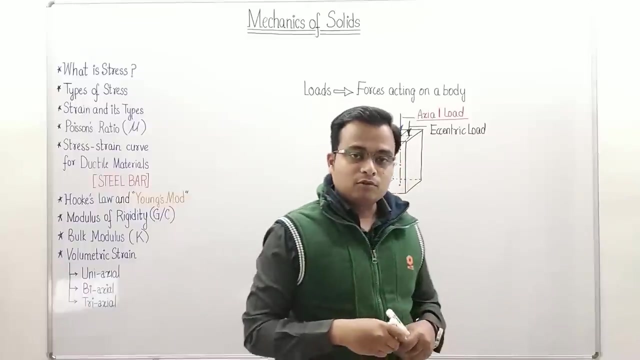 And how much is centric will. that can be worked out if we just try to extend this. Yeah, This distance over here is the eccentricity, okay, and this has to be measured always from the center. So these were all the types of loads. Now we have seen surface load. you have seen linearly distributed load. 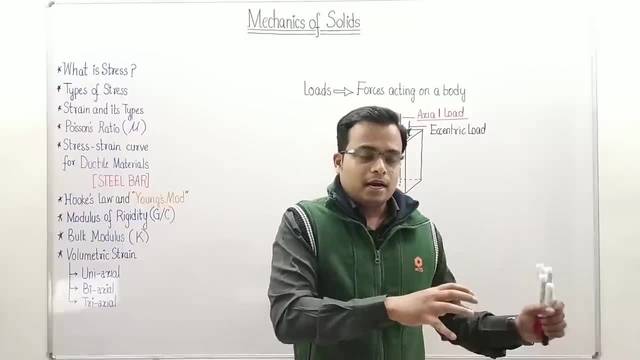 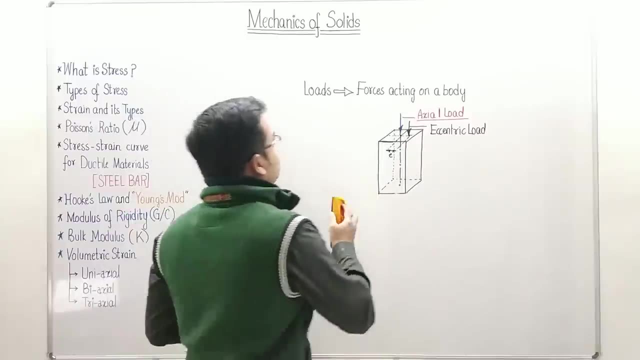 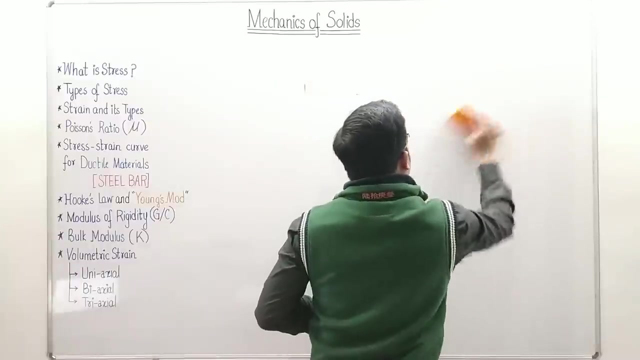 and you have seen point load, concentrated load. you've seen axial load, and how is it different from an eccentric load? So these were basically the classification of loads which you will be encountering in mechanical solids. Okay, one more thing, that is, in case of beams, you'll realize. 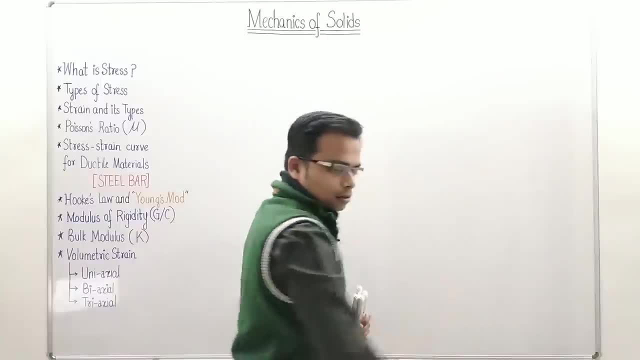 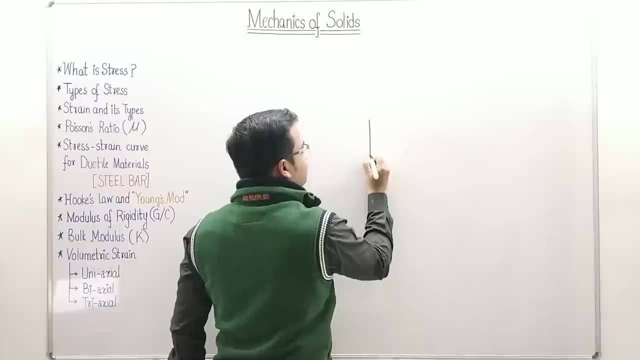 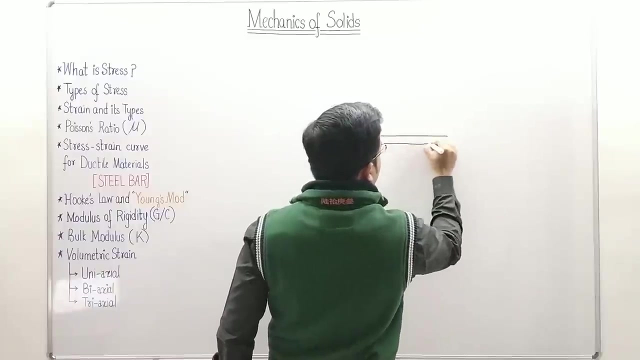 this, you'll see linearly or uniformly distributed loads. let's say you've got a fixed support and there is a beam over here- Okay, like this, And let's just assume that this beam has. when you look at it from over here, from the right hand side, it looks like this: 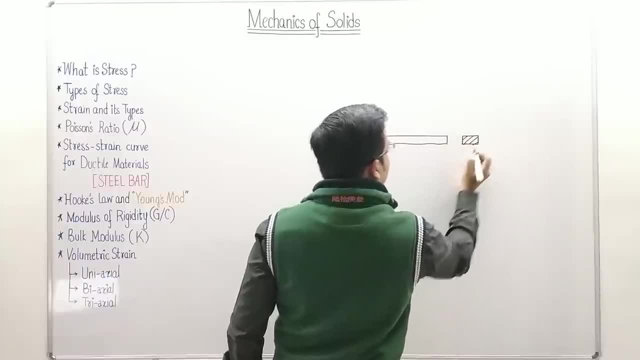 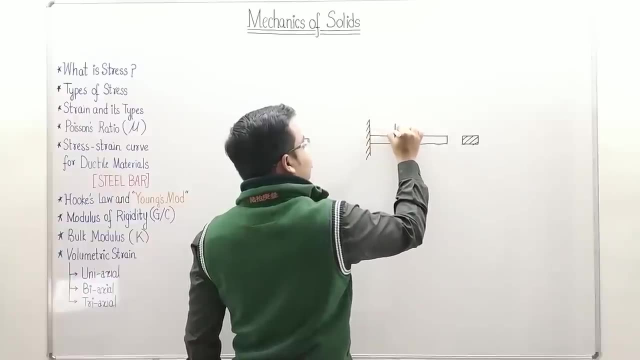 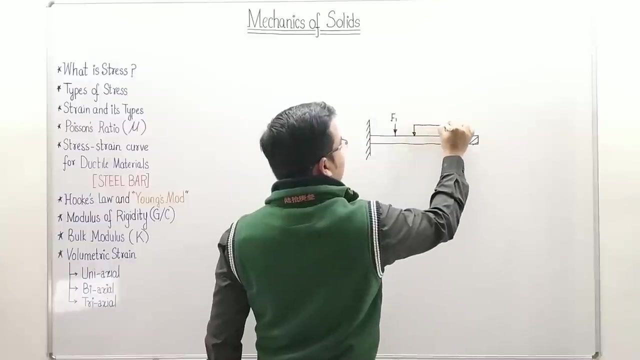 the cross section is this sort: Okay, Now, this is just a load at a point, let's say F1.. And then there will be in some of the books you'll find diagrams like this. This basically is a cantilever beam, by the way, Okay, something like: 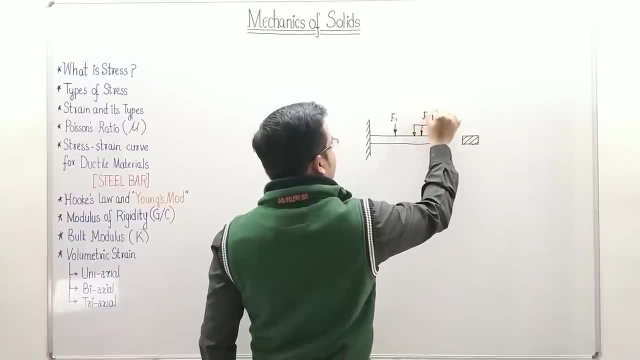 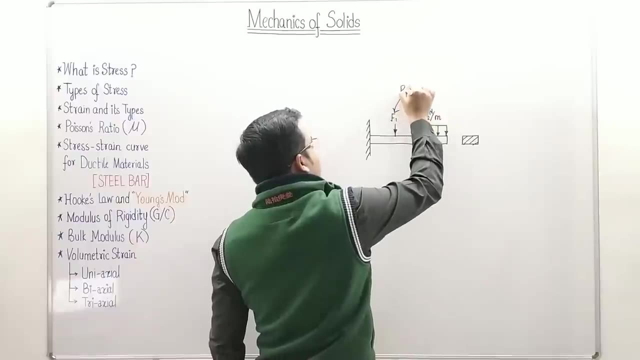 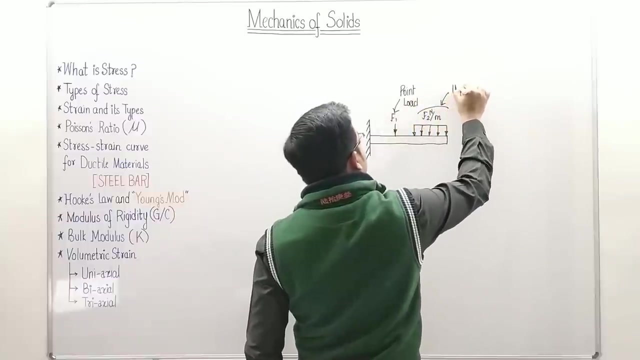 this. diagrams like this, And over here you'll be written: F2 per meter, newtons or kilonewtons, whatever it may be. This, basically, is a point load, And over here this is what is referred to as a uniformly distributed load. 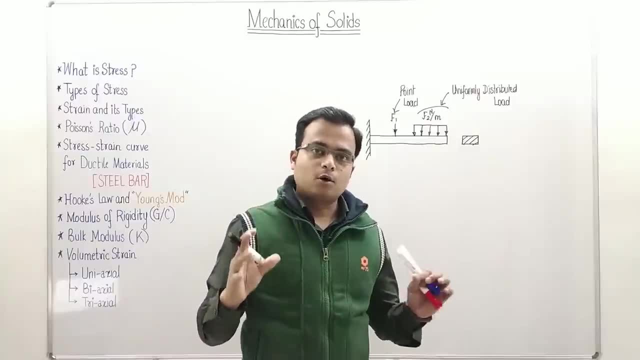 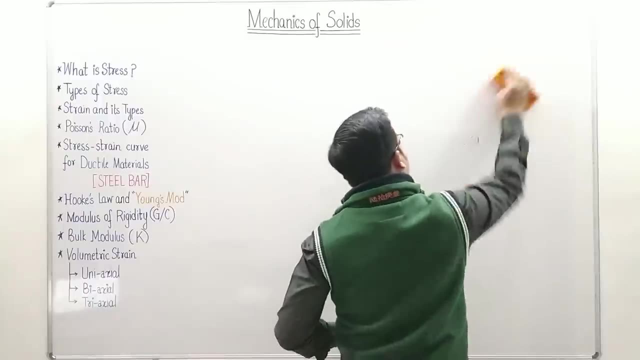 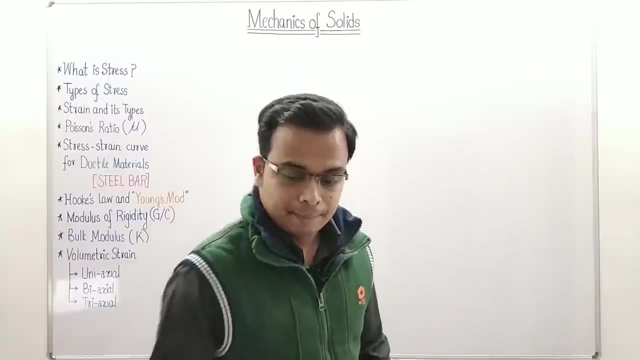 Okay, now let's take the session forward. And now let's talk about the real, that is, stress. Okay, so here we go. So, in order to understand stress again, let me give you a demonstration, And this is going to be very, very, very helpful. 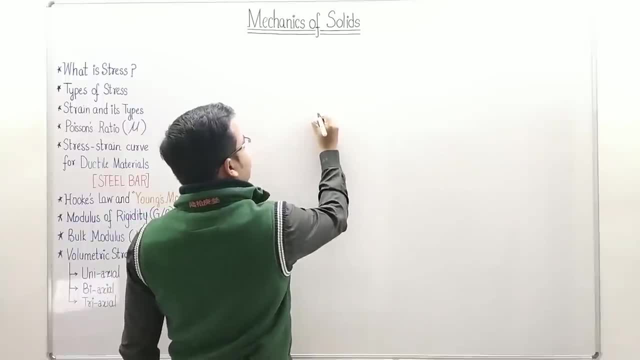 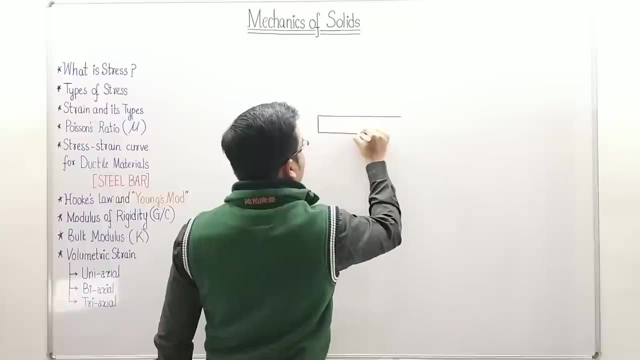 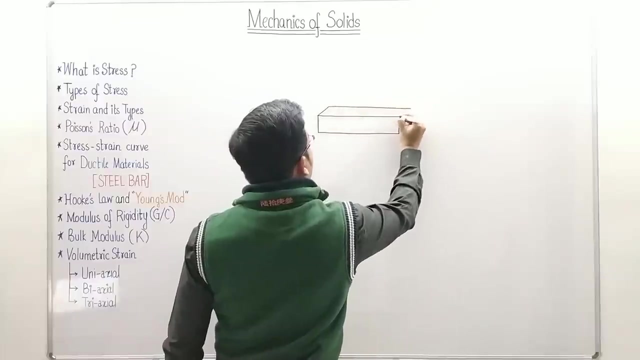 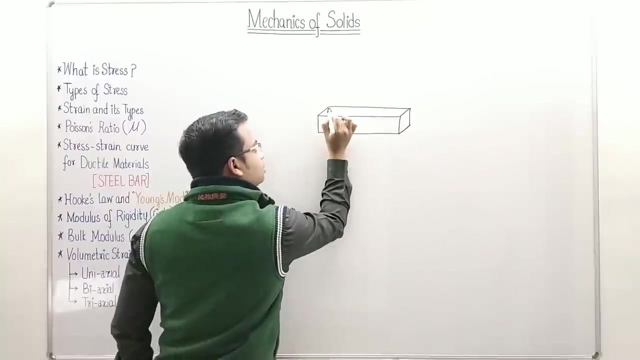 Okay, so let's begin Right. Let's say this: over here is a rectangular bar. Let me just do all of this in 3D. Yeah, Now, what what's really happening is. you can just have the cross section here, also at the back. Let me just extend this. 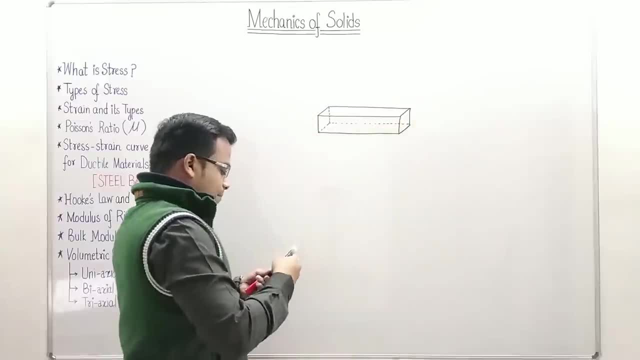 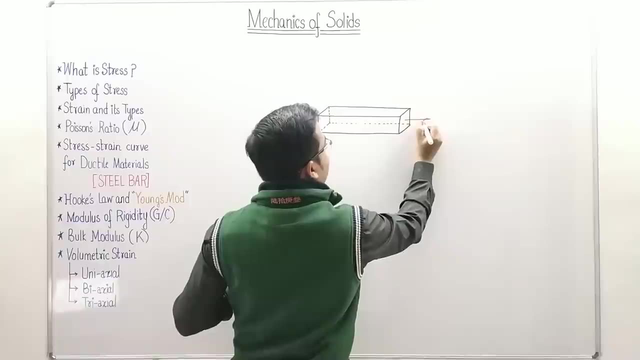 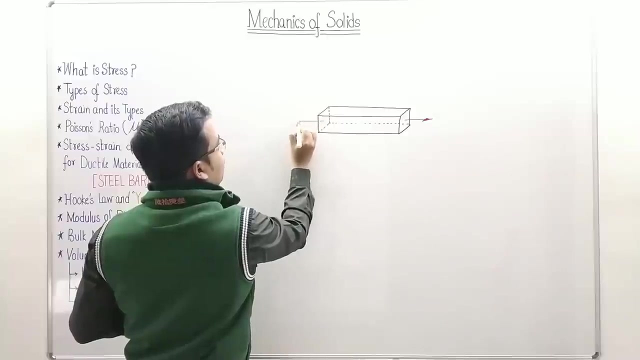 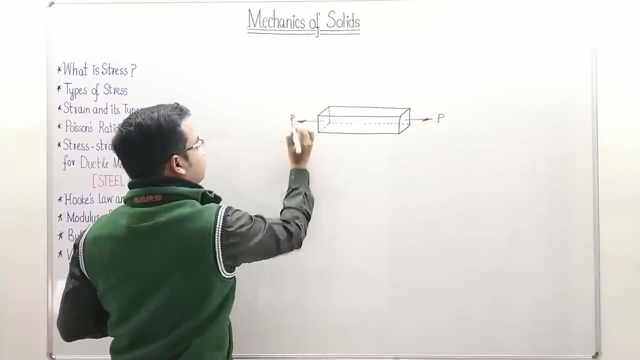 Until we reach here. So what is happening inside, rather outside, there is an external loading, Yeah, So this, this, this entire block is being pulled, Okay, let's say by a force P, in from both directions, obviously. So what we'll try to do is we'll try to focus on a particular cross section. let's say: 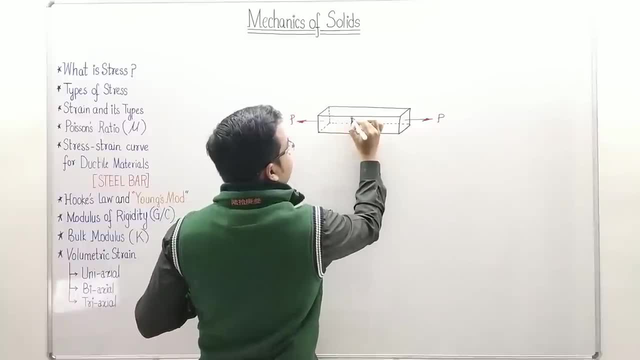 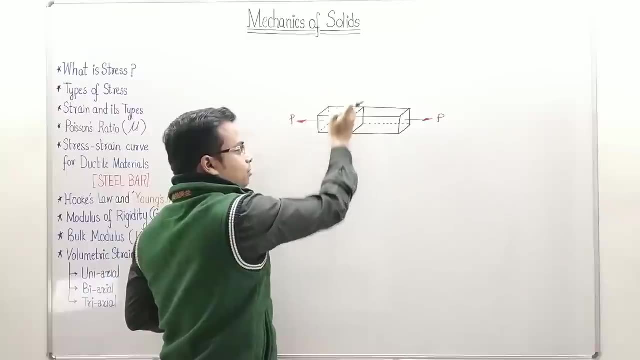 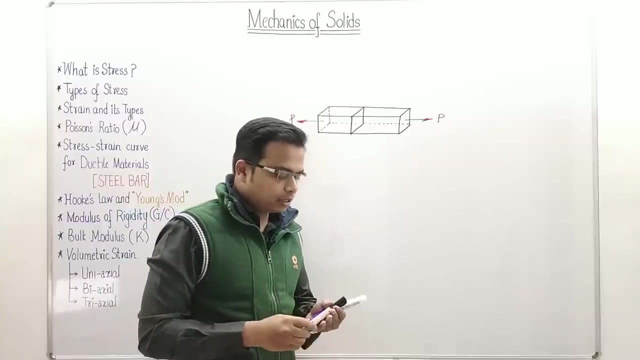 We are going to focus on this cross section. So what if I just cut this with respect to somewhere along this line? if I try to cut this object, what will happen? How will the internal fibers react to this? Let us just take this case. 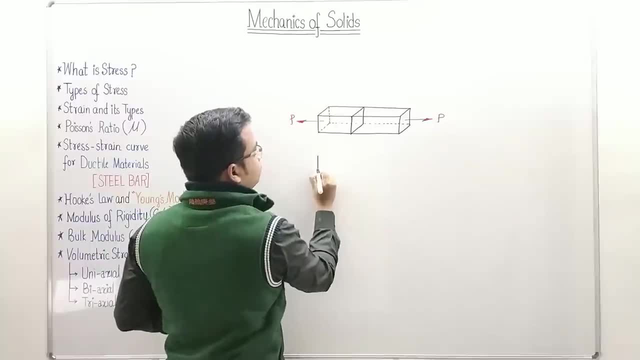 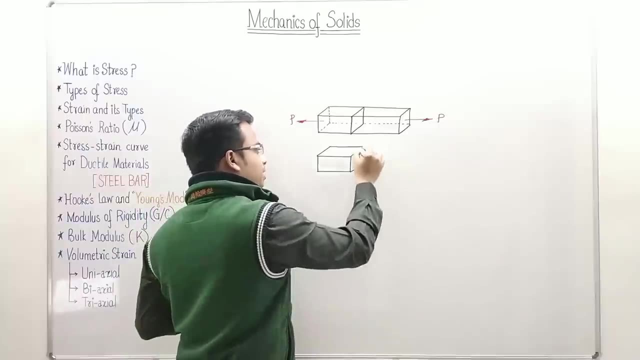 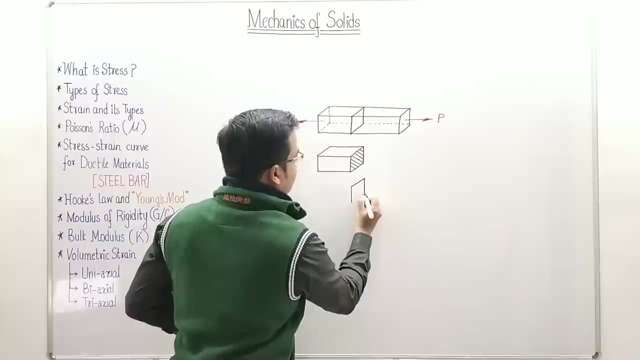 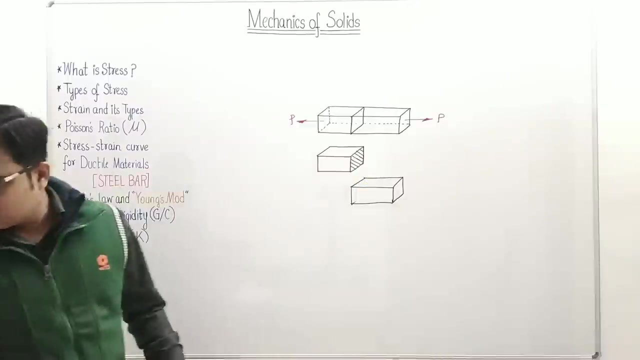 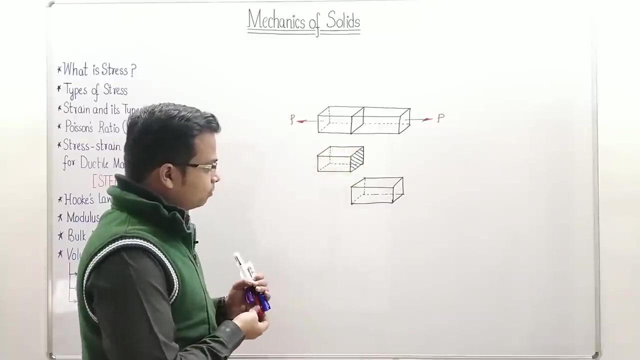 Okay, let me just draw this much portion right Now. guys, if you just watch this carefully, this is the area under investigation. guys, please take a careful look at this. So a force In the left hand side direction is being applied over here, isn't it? 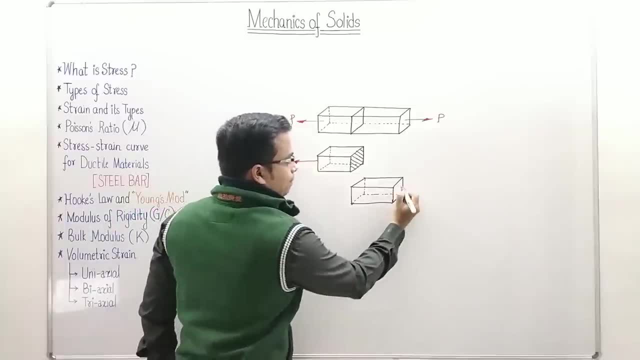 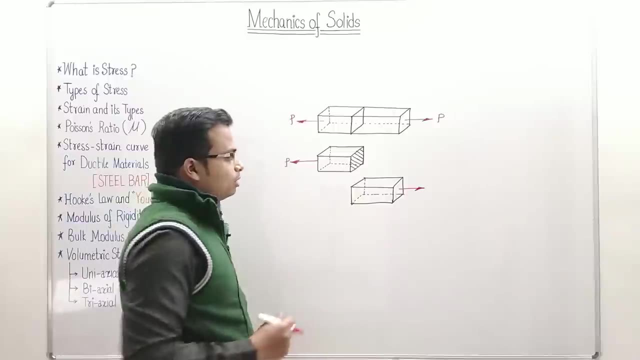 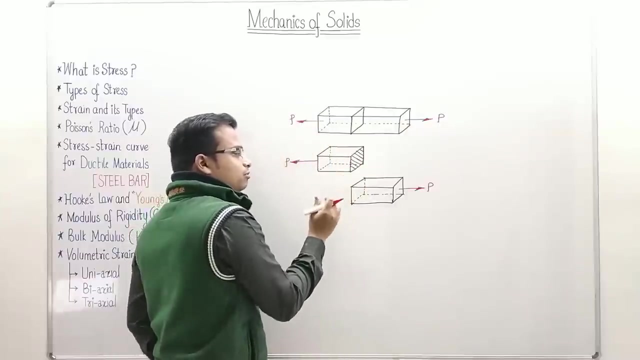 That the name of that force is P, or load is P, and over here also. So you can basically say that it has been pulled with a load P from both the directions. What will happen? What will happen here? So here the fibers will be such they will try to regain its original shape and size. 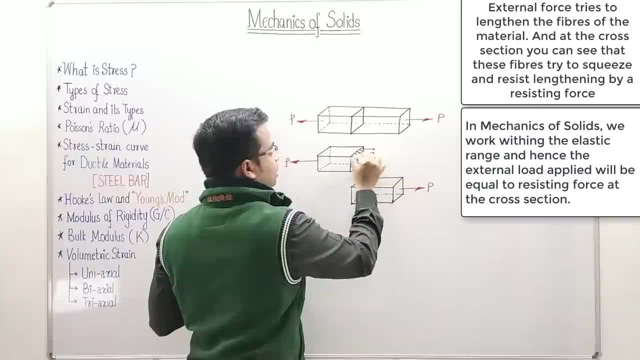 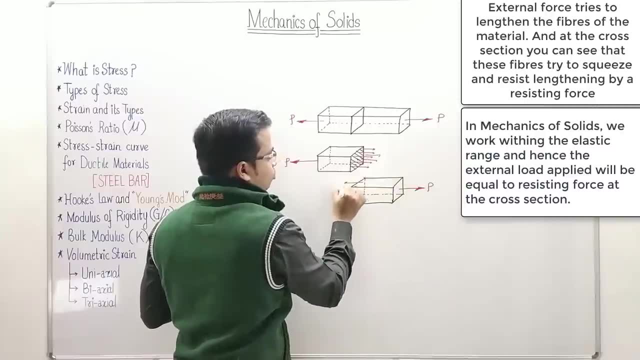 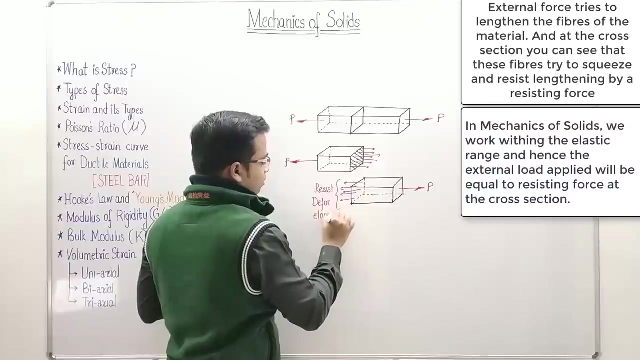 And in that process, each and everywhere along this area, forces will generate. Okay, here also, at each and every point, forces will generate. Now, the nature of these forces will be such: they will resist. they will resist what? deformation? or you can also say, they will resist elongation, isn't it? 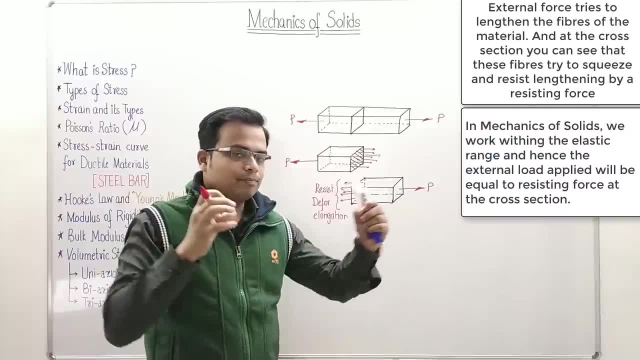 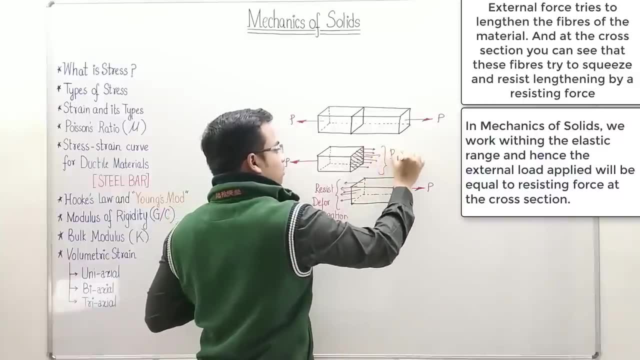 Now, the nature of these two forces is such that it will always try to elongate, it will always try to extend the length of this entire object. And here also, Okay, There is going to be resistance offered. There is going to be resistance offered by the fibers over here. 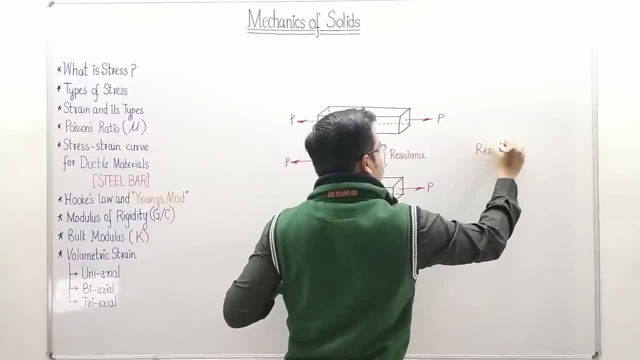 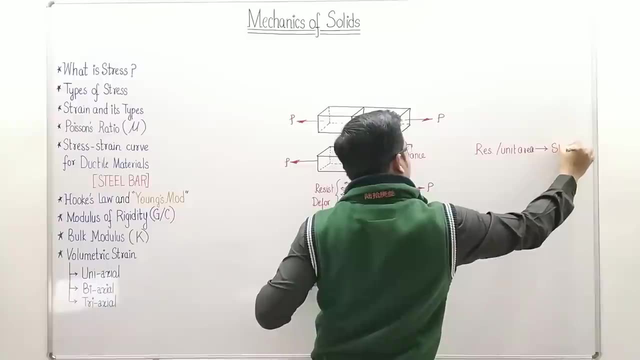 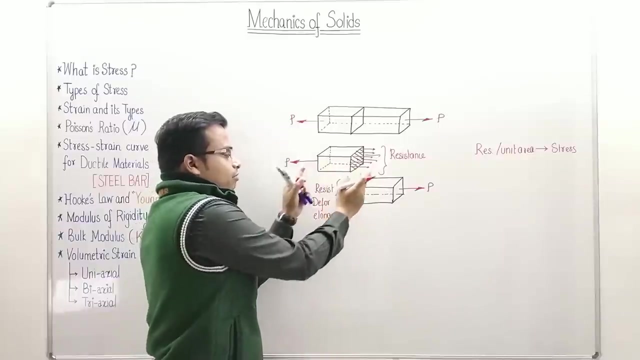 And this resistance per unit area is what is referred to as stress. Let me make it very clear What happens when you apply force and if you do a cross section, okay, somewhere here it will try to regain its original shape and size and in that process it will try to develop. 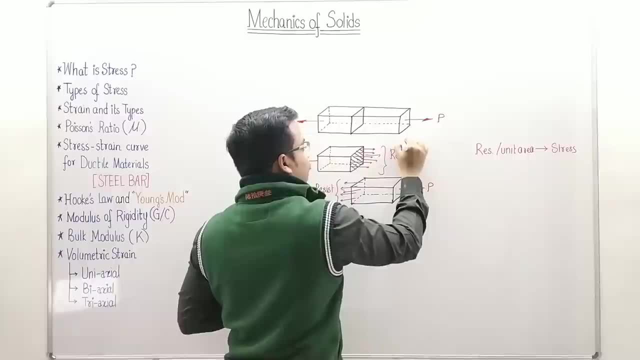 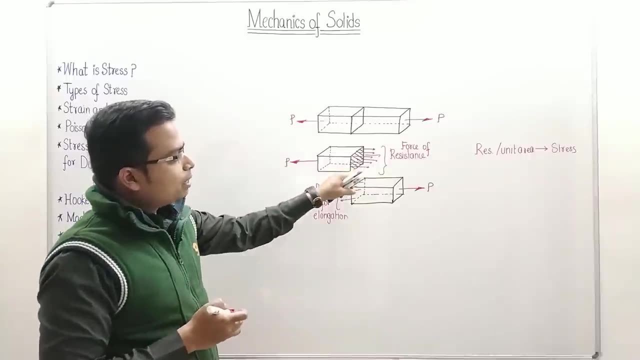 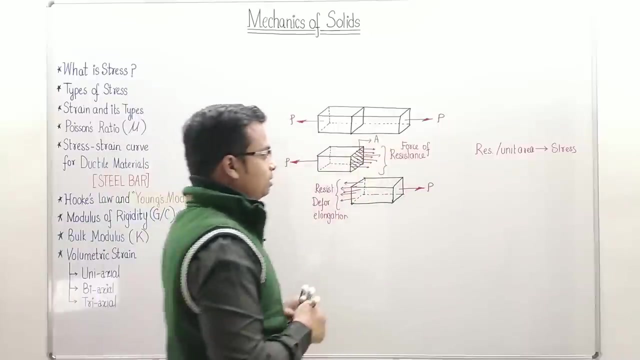 a resisting force. Okay, so this is basically the force of resistance. force of resistance. Now, this force of resistance per unit area. per unit area means this: H- this is area A is what is referred to as stress. So let me just finally write it over here. 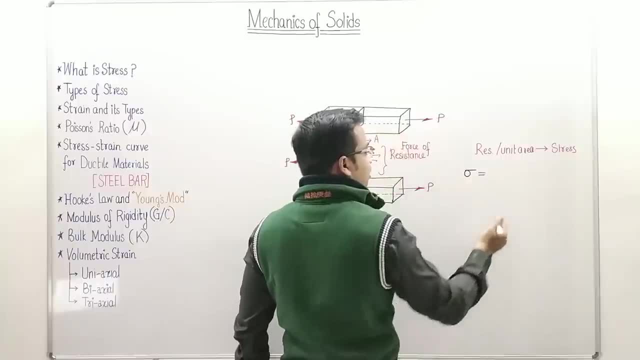 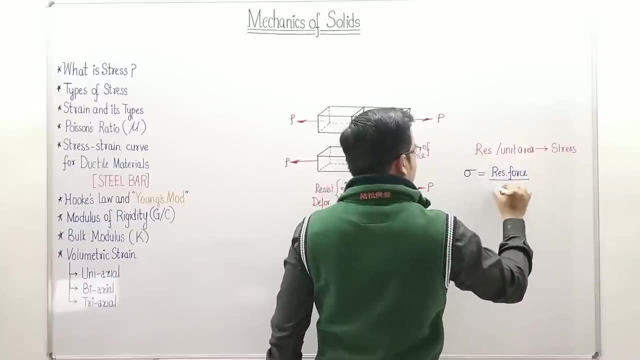 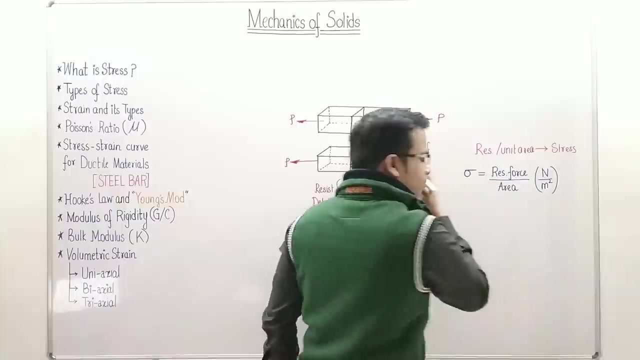 Sigma is the stress, So stress is represented by sigma and this is actually equal to the resisting force. resisting force, Okay, Divided by the area in which that force has developed, And this is computed in Newton's per meter square, or some people also work it out in: 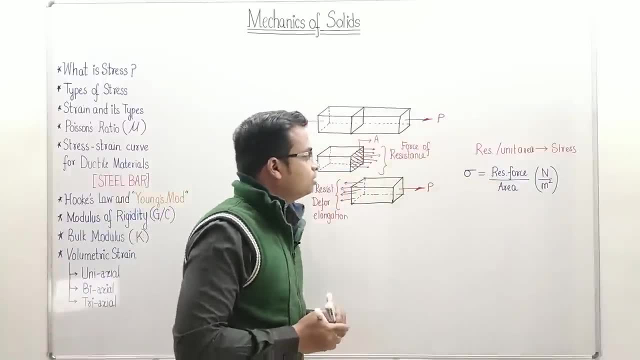 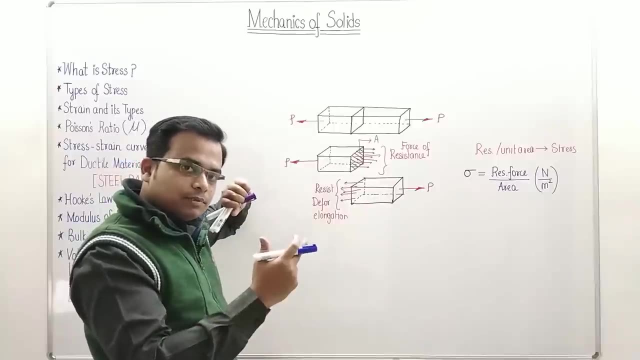 Newton per millimeter square. That completely depends on how you make an assessment of that. So this is basically the entire idea of how. as to how you can assess stress right Now, let us take this session forward and let us try to work out all the different types. 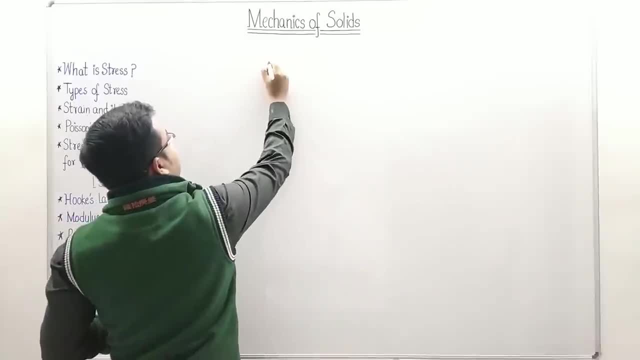 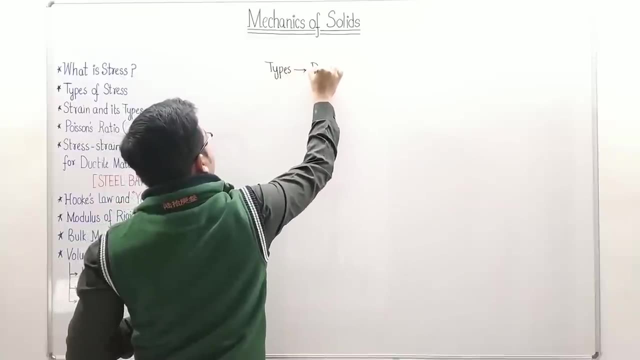 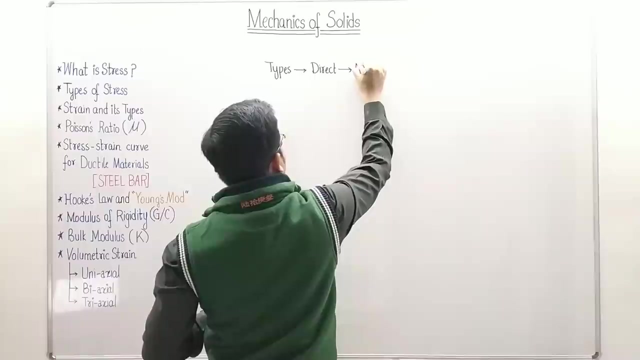 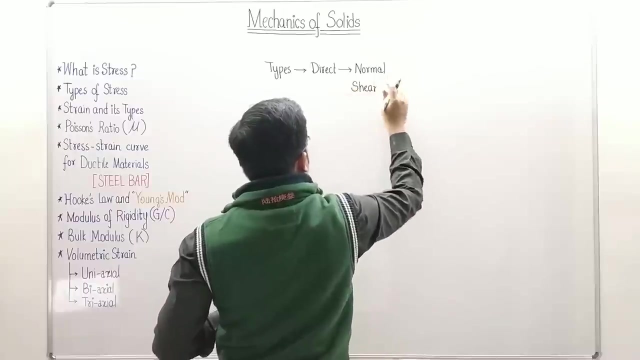 of stresses. So here we go. Okay, So basically there are three types of stress. The first type is direct, And when I say direct, it is again divided into two types. It is normal and shear, normal and shear. And when I speak about normal, it is again divided into two types. 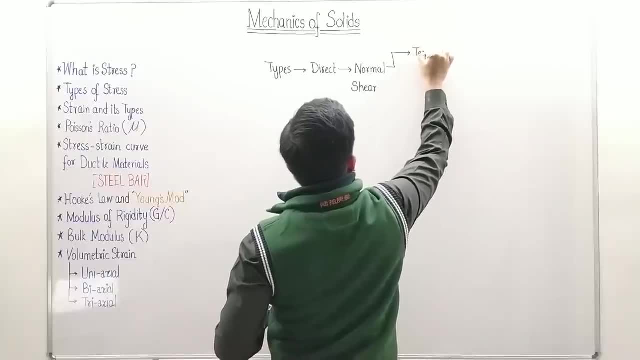 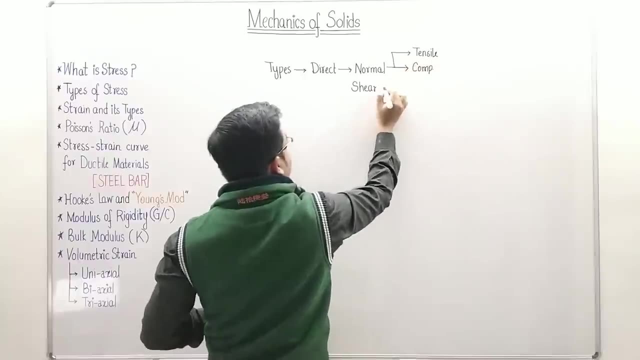 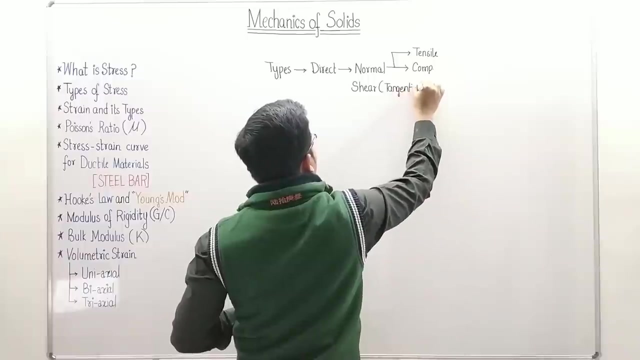 This is normal tensile. and one more particular is there. That is normal tensile. This is normal tensile. This is normal compressive. Now, this is a completely different category and this is where tangential forces come into the picture. We will talk about that eventually, do not worry. 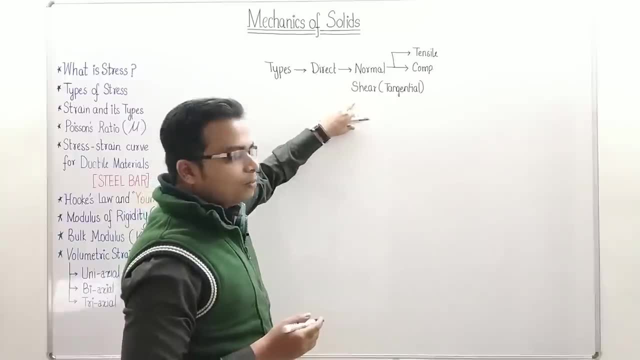 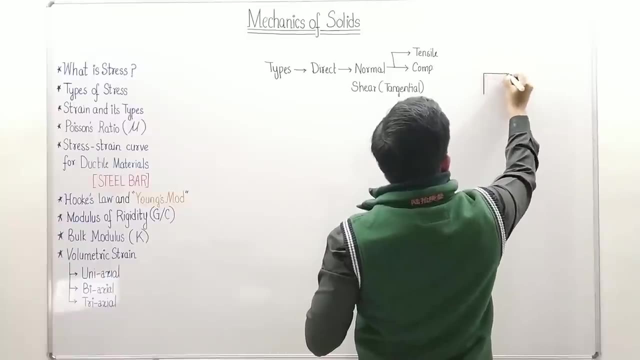 Okay, So what exactly is normal stress And how is it different from a shear stress? Let us work it out. Let me explain you with the help of a simple example. let us say we have got a block over here And let us just say that this block is kept. 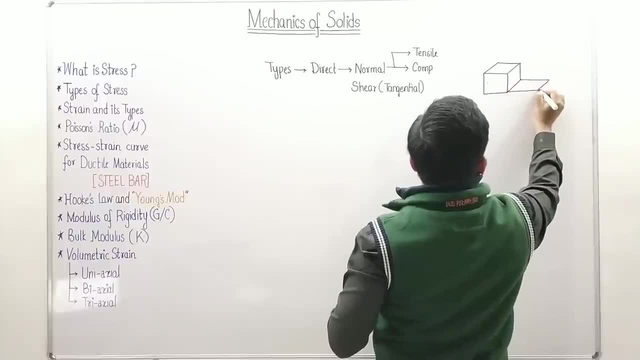 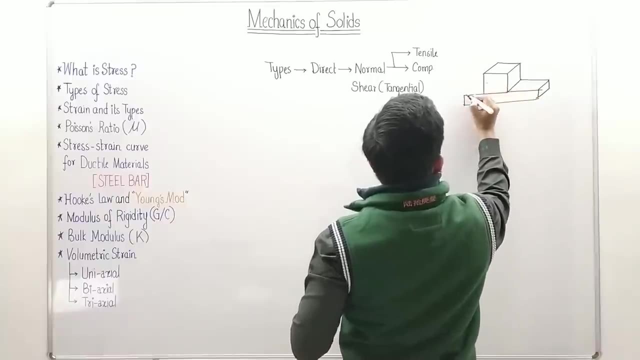 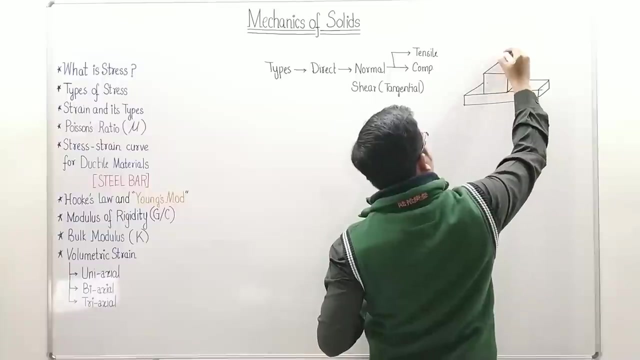 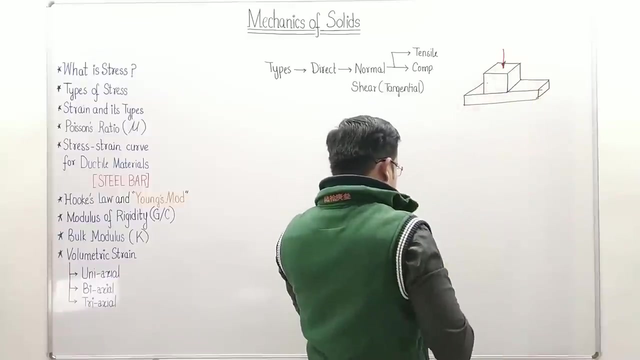 Okay, On a platform This much thick, Okay, Okay, that is good. Now what happens if you apply a force? So when you apply a force like this, right, and let us say, this force is actually perpendicular, Perpendicular. 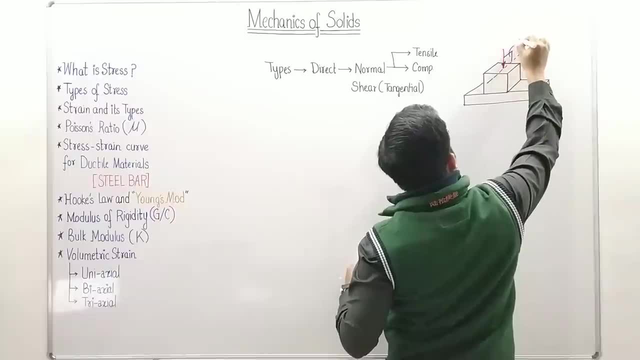 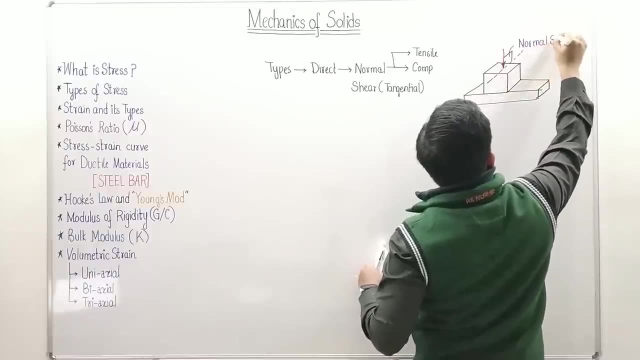 Perpendicular. Okay, So if this is perpendicular, then the kind of force that we are dealing with, or the kind of stress developed, will be a normal stress. Now, if you take a careful look at this and let us say, this dimension is represented by 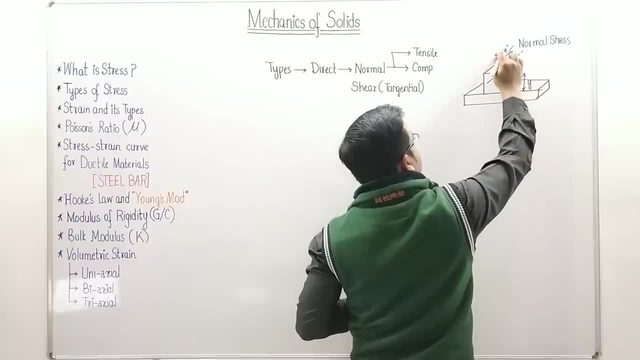 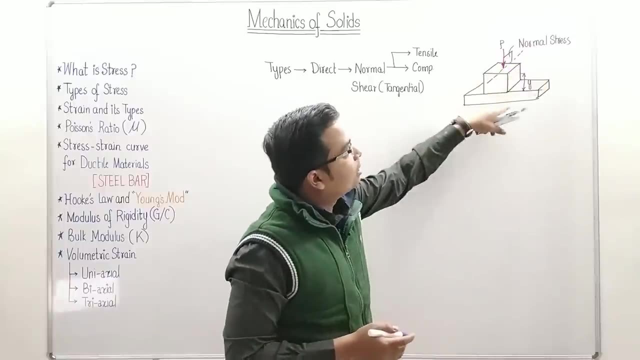 Y. The nature of this load is such. the nature of this load P is such that it will try to reduce this dimension. Okay, It will try to compress the object along the Y direction, and that is why the stress generated in this case is referred to as. 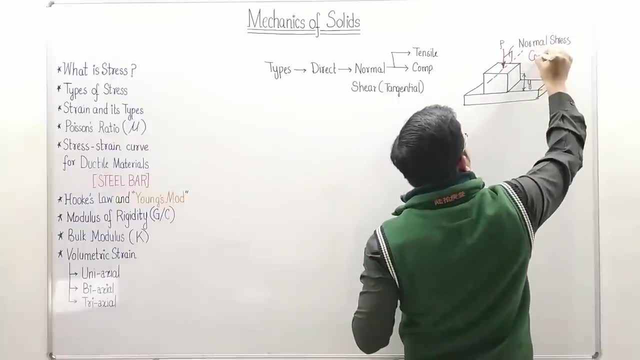 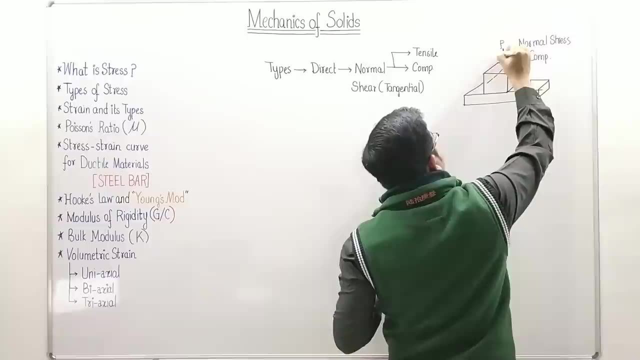 The normal compressive stress. So this is going to be normal compressive stress. And now, if I change the direction of force, if I do it like this, in that case let us say this is fixed. This is fixed to this platform. 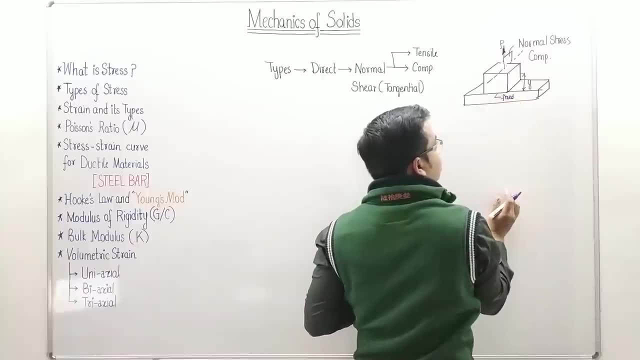 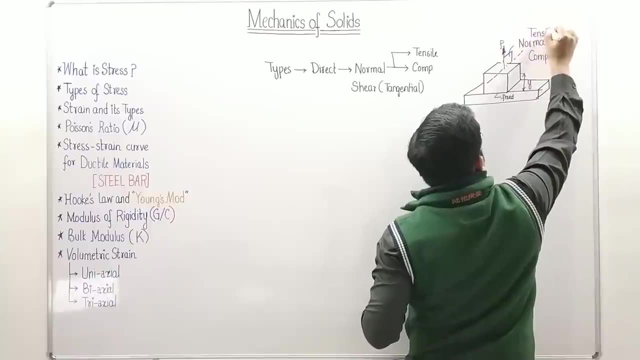 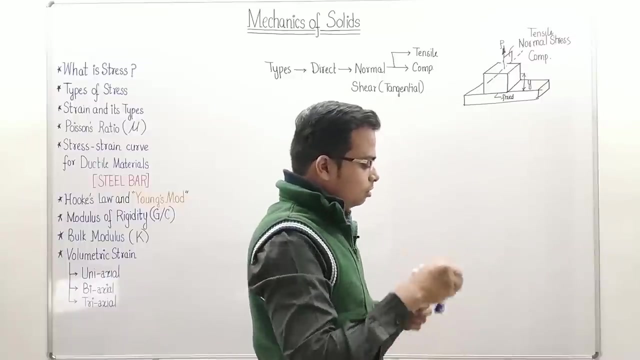 This is fixed, Otherwise it will go up. if this is fixed and if you try to pull it in the upper direction, in that case it is going to be a case of normal tensile stress or the stress developed. Okay, So if the stress developed along this cross section- let me just draw this along- any 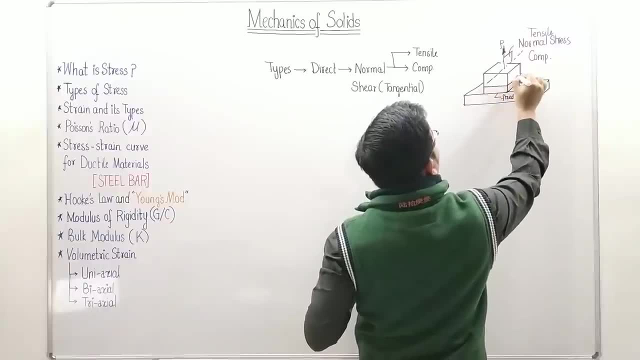 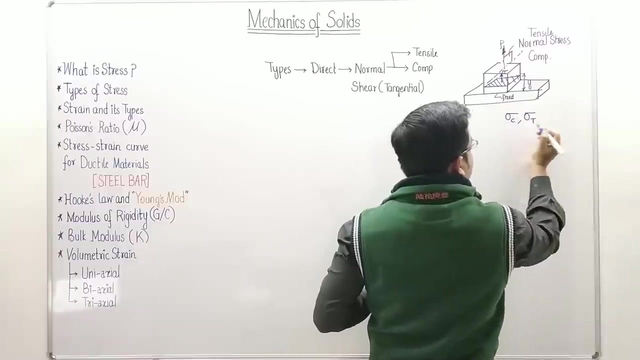 cross section, cross section. like this, stress developed along this cross section sigma will be normal. So basically, there is a normal compressive stress, there is normal tensile stress- sigma c and sigma t- and where the units are going to be same, it is stress. 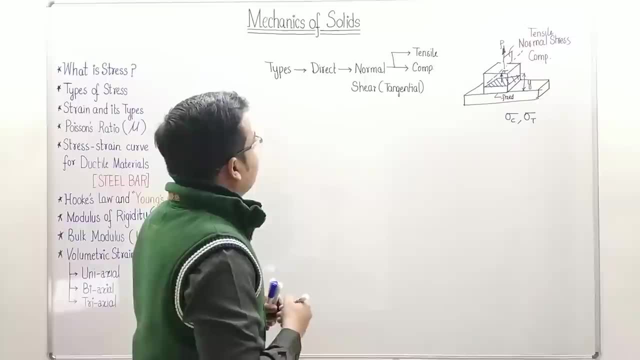 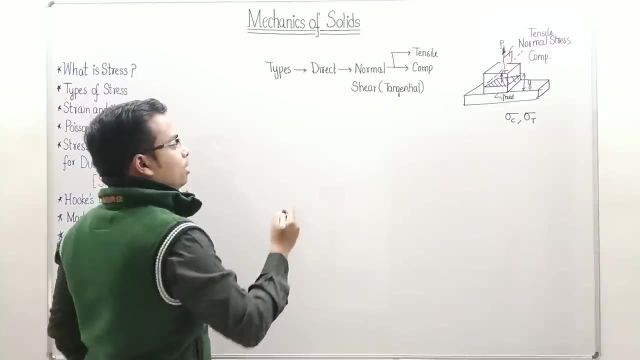 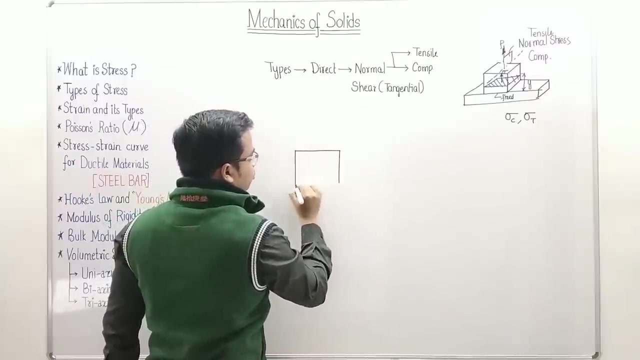 Okay, So the next thing that we are going to talk about is the shear stress. So take a look at what shear stress is Again. for that, I need to draw a diagram again, Again, let us work in 3D. As I have told you, in case of shear stresses, we have to work in tangential forces. 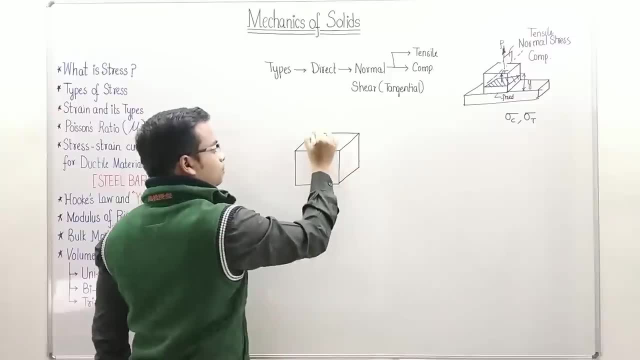 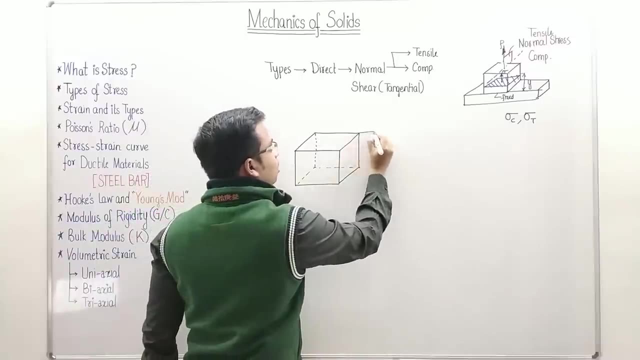 And how exactly are they different from normal forces? let us see that. So here the idea is to apply a force. Okay, So watch this case. The forces being applied are of this nature. let me just draw this, okay, like this: 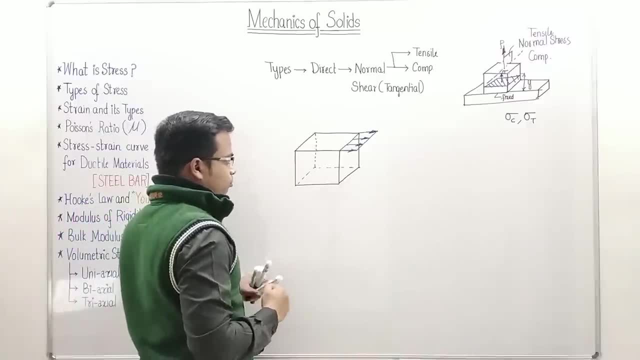 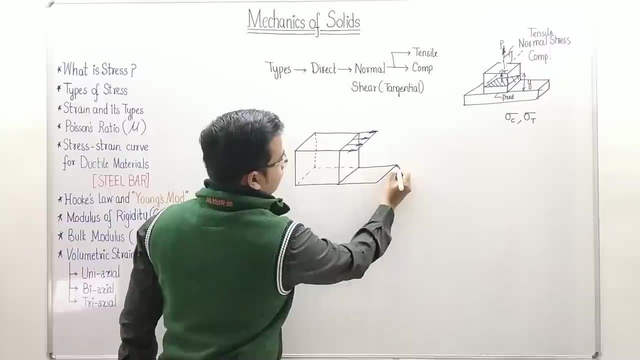 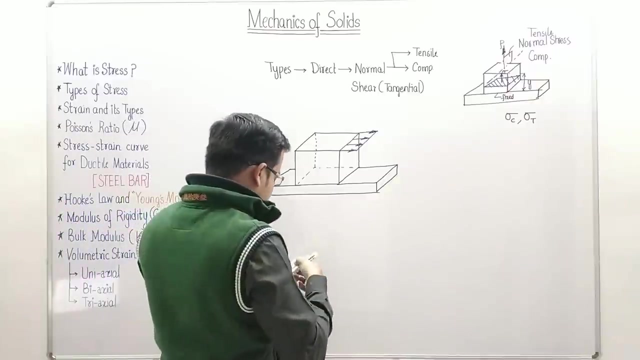 What will happen? Let us say I am fixing this portion. This portion is fixed. Let me put this into a platform above a platform. So at any cross section, At any given cross section, let us say I am talking about this cross section. 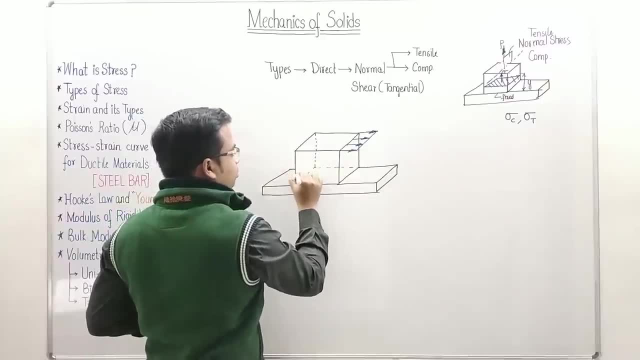 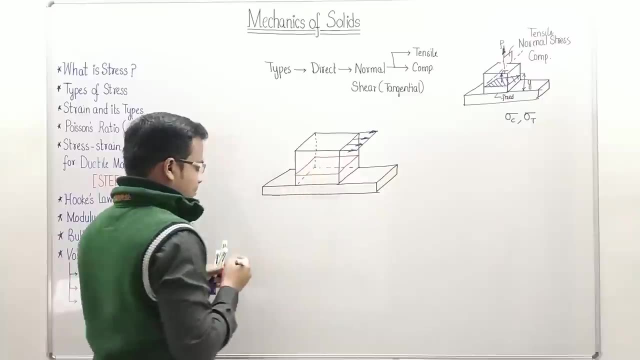 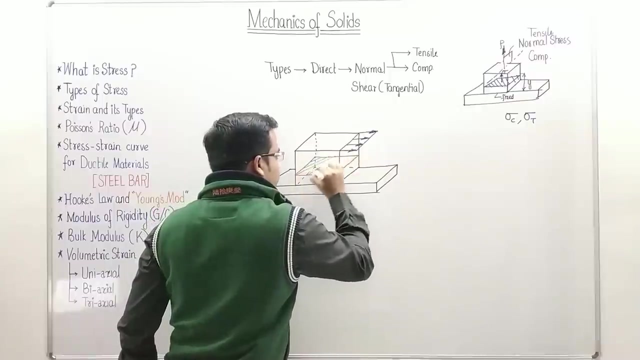 Okay, Let me cut it like this: horizontally: I am talking about this cross section. Here we go, Here. here I am talking about this cross section. What will happen? And let us take a look as to what is really happening along this cross section. 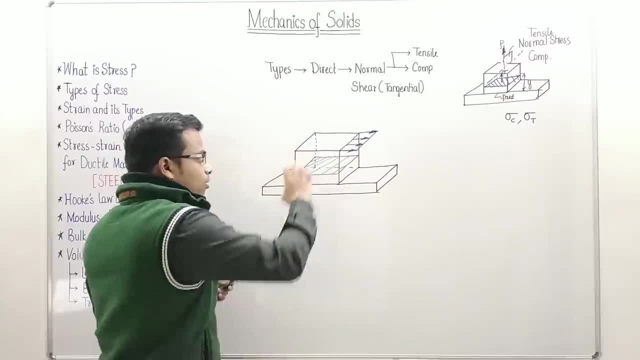 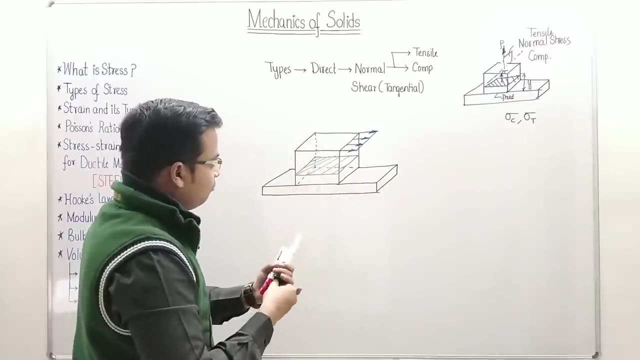 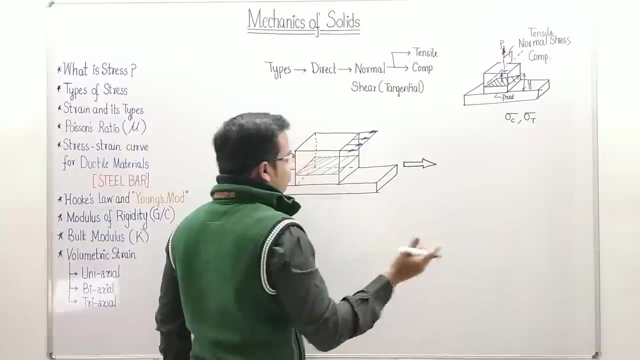 Let us take a look. So what we will do- Above portion and bottom portion- Let me just separate these two portions With respect to this cross section. So the stuff that you will get to see now is this: Sheer stress is a bit confusing, but eventually all of that will be worked out. 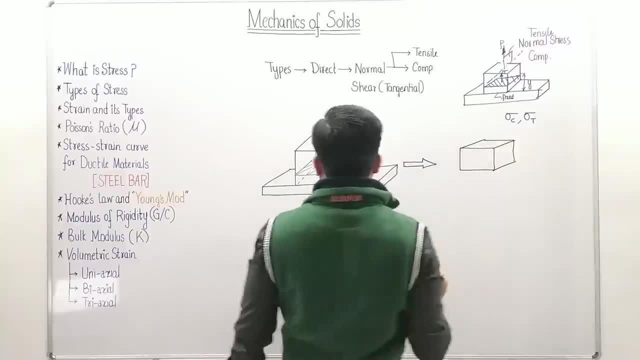 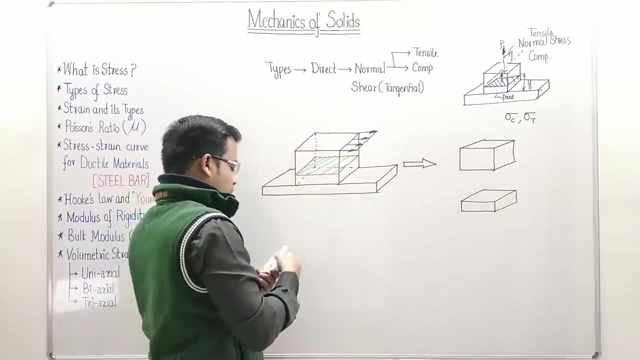 You will see that. Okay, So what is happening? What is happening If you are going to apply a force over here- And this is the tangential force by the gate, And let us call this force by V, Okay, So what is happening? 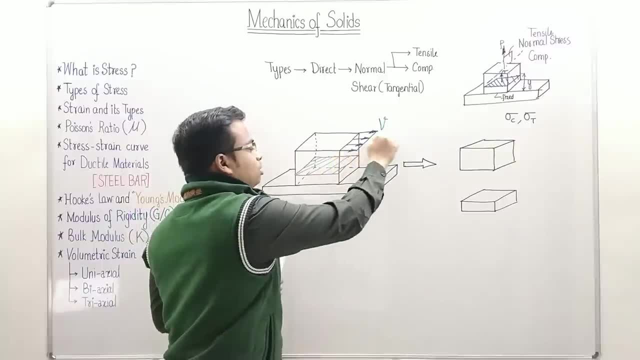 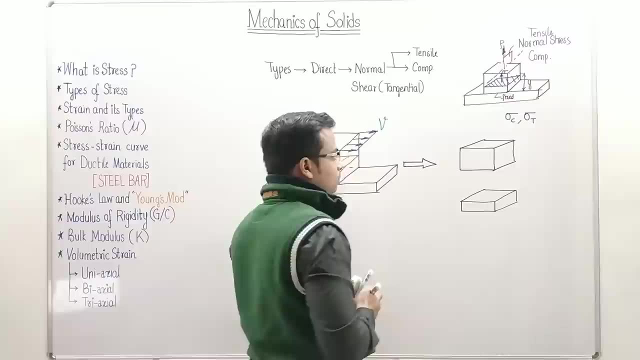 What is happening If you are going to apply a force over here? The collection of all these forces. If you sum up all these forces, You can replace all of them with a single force, And let us say that force is represented by V. Okay, 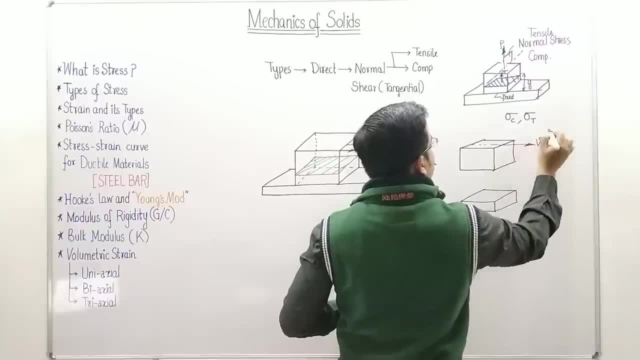 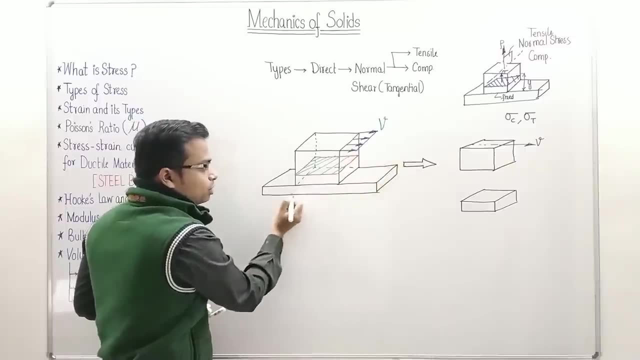 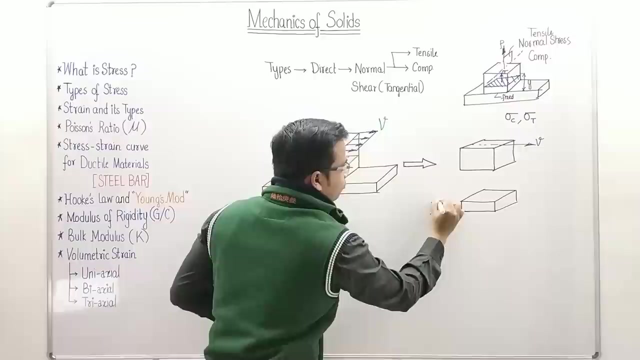 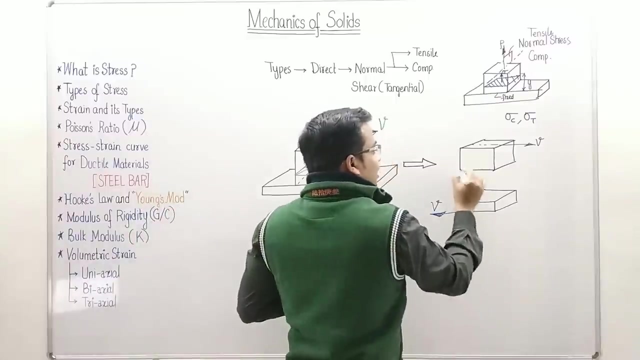 Now, if there is a V force over here, then it is going to be balanced by a force from this fixed portion. So there is going to be a similar force over here also, Isn't it? That is going to be V again. Now, if you watch carefully, this block will remain in equilibrium. 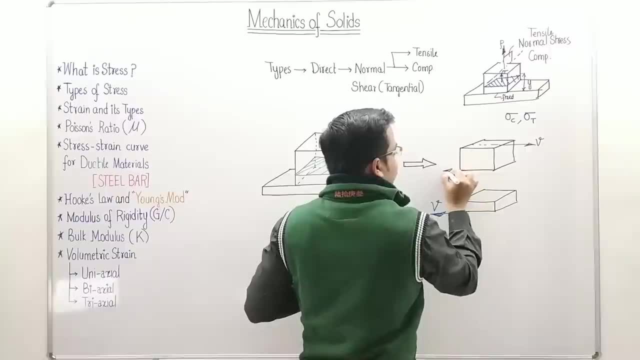 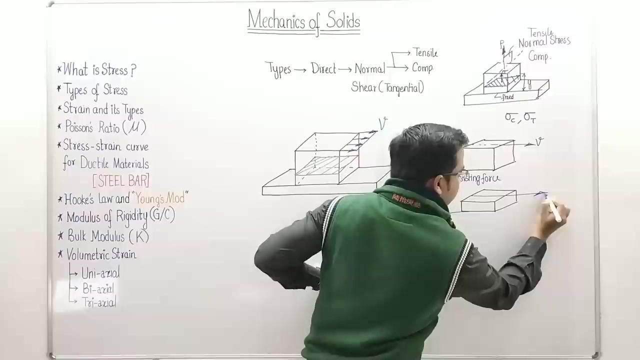 Now, the resisting force will develop something of this sort. This is the resisting force, Resisting force. And here, if it is, if this is the tangential force, then the resisting force will be developing like this: Again, this is the resisting force. 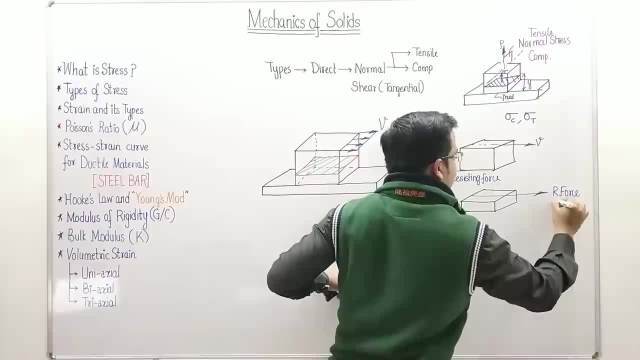 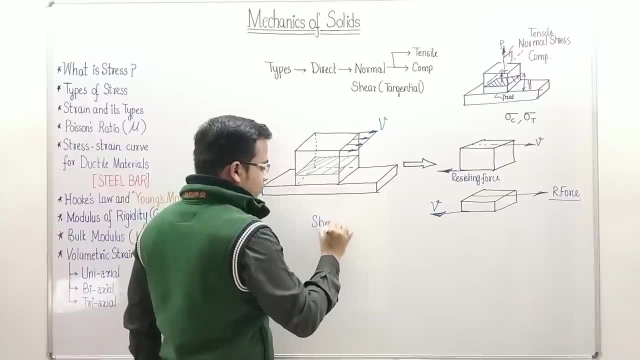 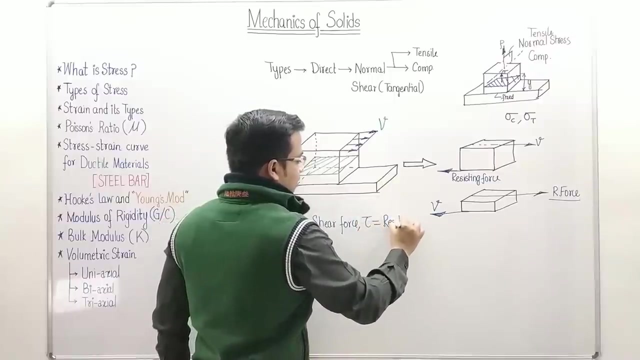 Let me just write it as Rf: Resisting force. Okay, Now, as far as the definition of shear force is concerned, it is represented first of all by tau. Right Shear force is actually represented by tau and it is equal to the resisting tangential. 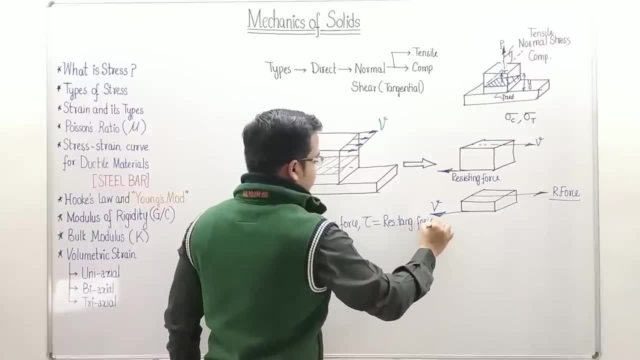 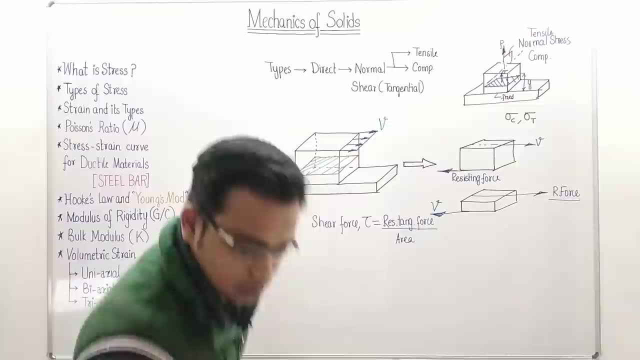 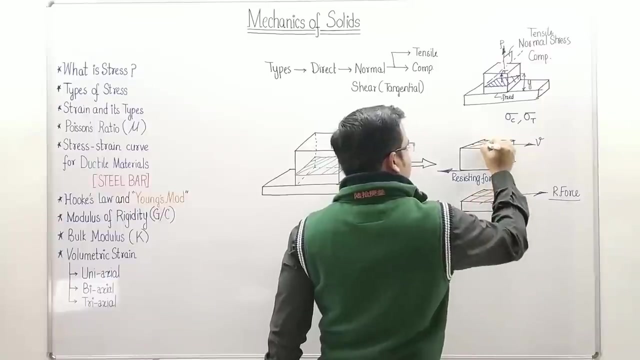 force. I am not writing it entirely Per unit area, And what is the area that I am talking about? The area that I am talking about is this: Kya, This is the area. Okay, This is the area that I am talking about. 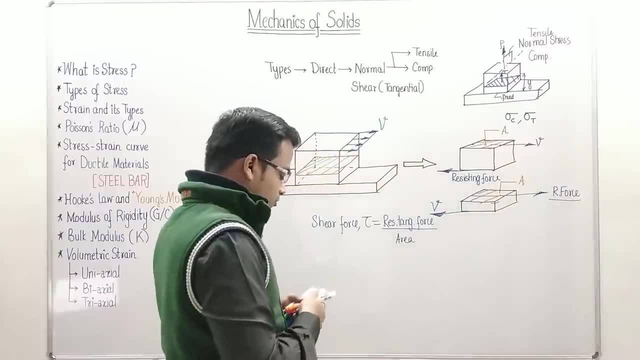 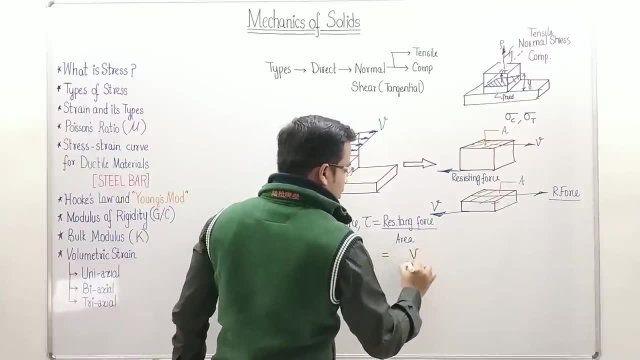 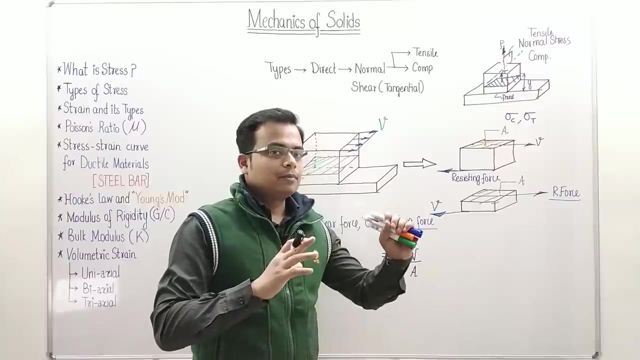 A, A. So the resisting tangential force with respect to area will give you the magnitude of shear force. So that is going to be equal to V upon A. Now always remember, guys, in mechanics of solids we have to go until the elastic limit. 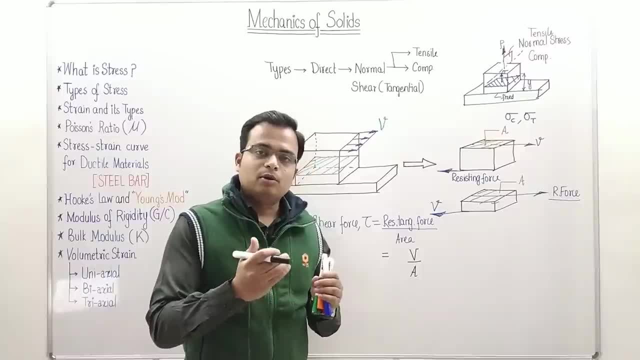 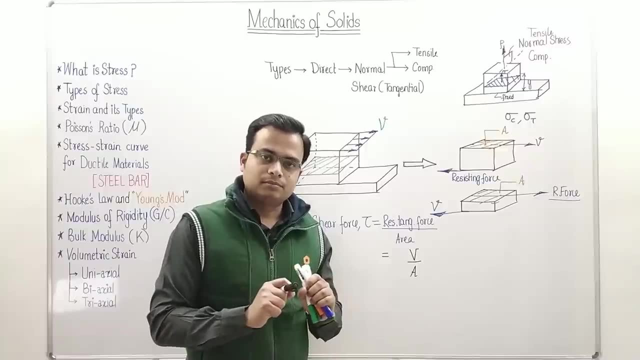 is reached, Or the force that we are going to apply should be below the elastic limit. Okay, That means, after removing the force, the material should be able to regain its original shape and size. And also there are some more assumptions that the material has to be homogenous. 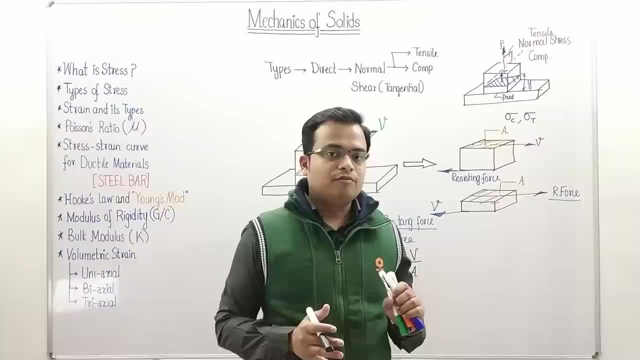 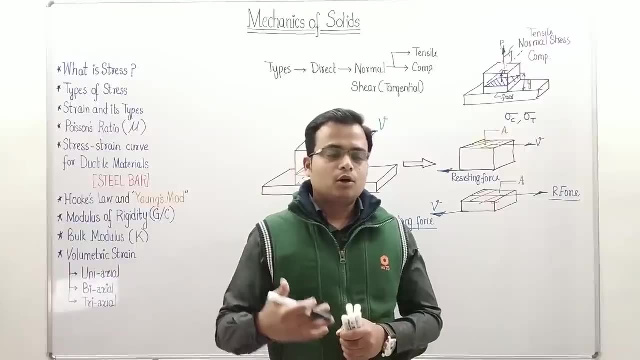 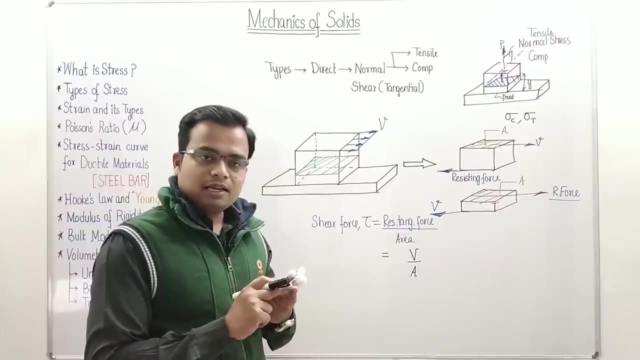 It has to be isotropic. These are the conditions which we will be considering always in, in fact in every chapter, be it bending torsion column, anywhere. So the material has always got to be homogenous. By homogenous, I mean to say that the physical and mechanical properties will remain constant. 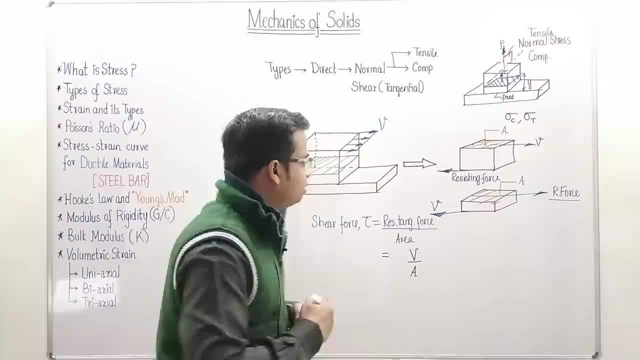 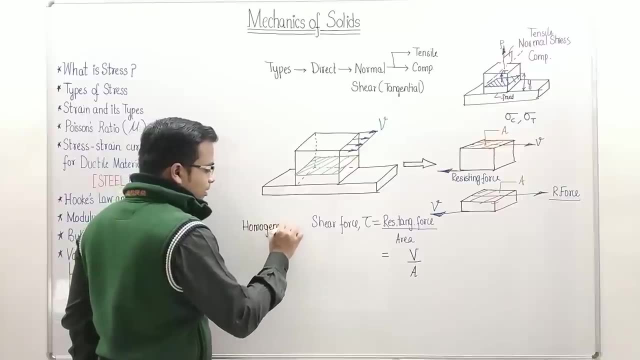 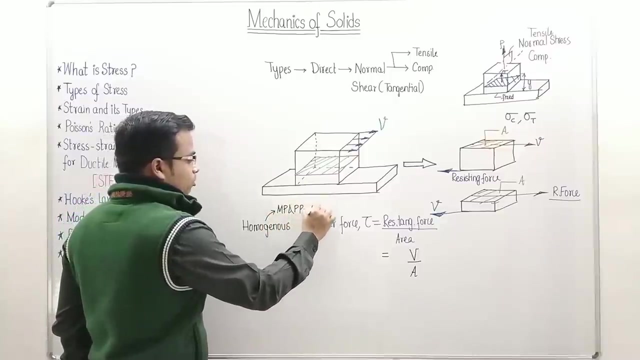 throughout the entire volume. Okay, If we just write this, materials are going to remain homogenous. That means the material properties, mechanical properties, and mechanical properties and physical properties remain constant throughout. Secondly, isotropic: That means there are certain mechanical properties which actually are different in different 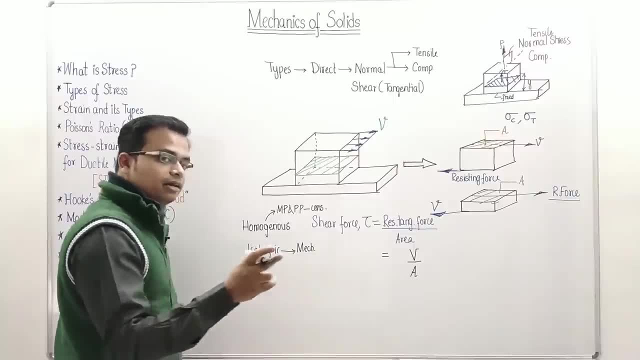 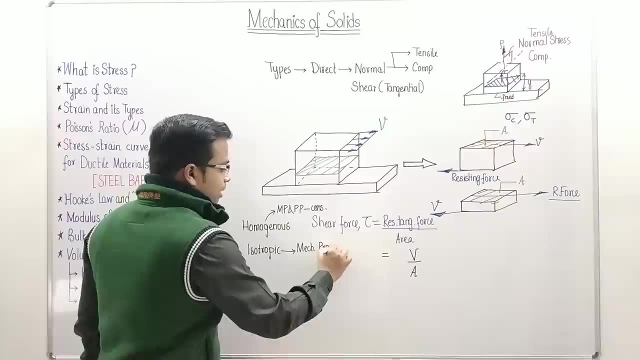 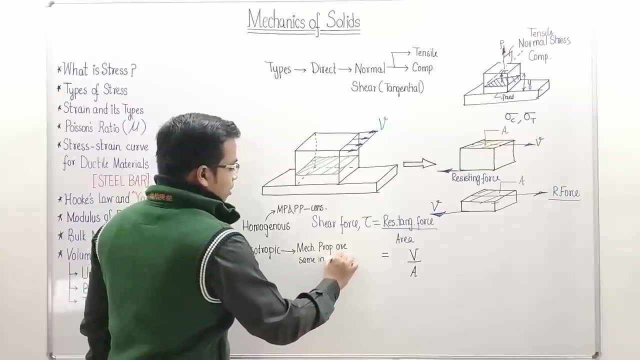 directions. That means x, y and z direction. it is an isotropic, But we are going to assume that the material properties or the mechanical properties are same in all the directions are same in x, y and z directions. So I think you should note this down. 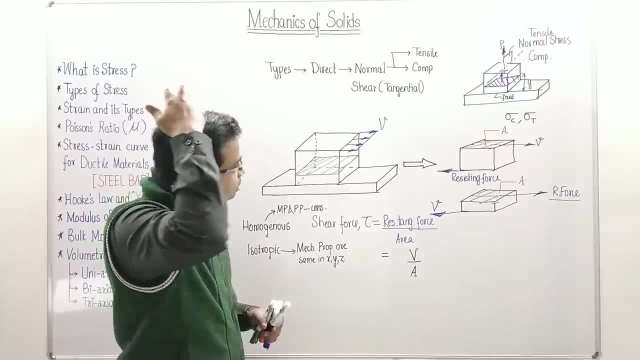 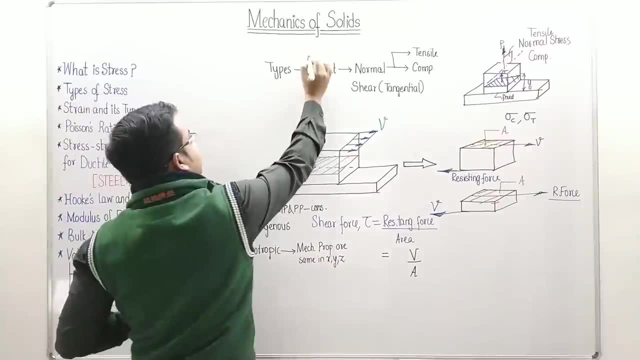 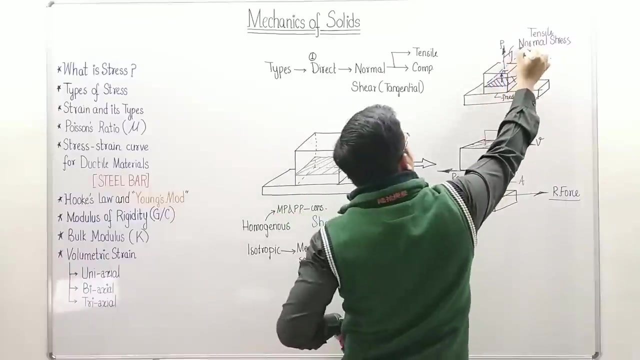 This is going to be very important. Okay, So this was the entire stuff regarding what is known as a shear force. So the first type is, or the first category was, direct stress. Again, we saw normal shear. So if the force applied- load is acting at an angle of 90 degrees, it is normal stress. 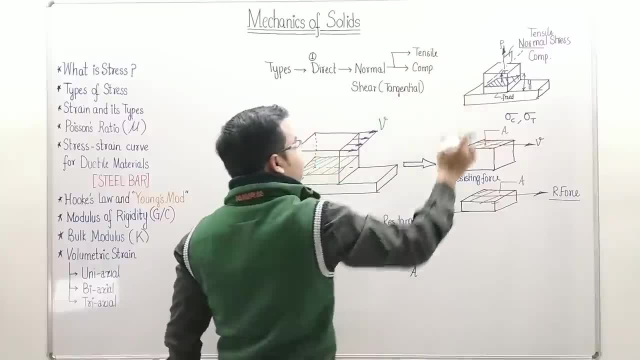 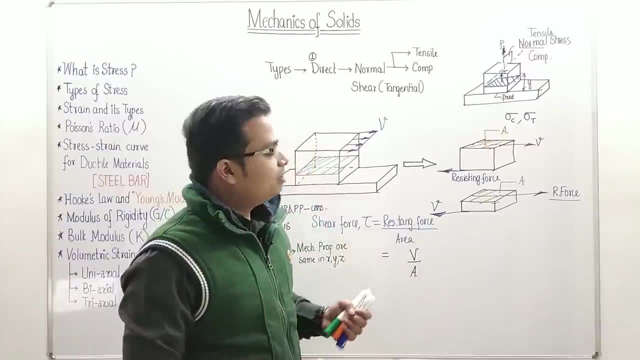 Okay, And it could be of two nature: tensile and compressive. If it is trying to extend the length of the bar, then it is a tensile, normal stress, And if it is trying to reduce the length of a bar, then it is normal, compressive stress. 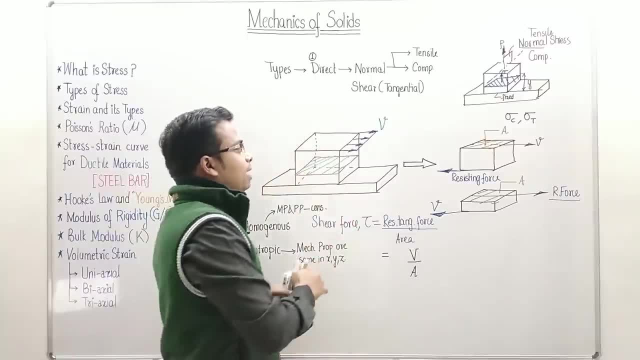 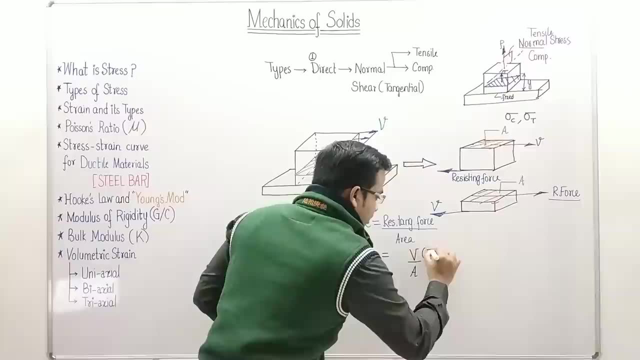 And then we saw shear stress, And shear stress: the force applied is tangential in nature, And you saw the entire analysis Here: the tangential force. Let me just write this: The tangential force, or the force acting through the area, has to be taken into consideration. 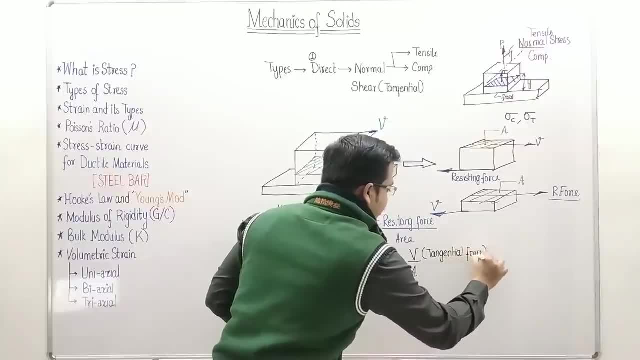 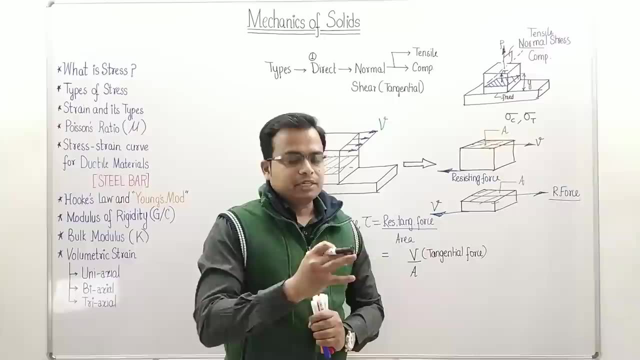 and not the normal force. So to differentiate these two stresses: normal stress and shear stress. In normal stress the normal load is taken into account. You just need to work out whether the normal load is compressive in nature or tensile in. 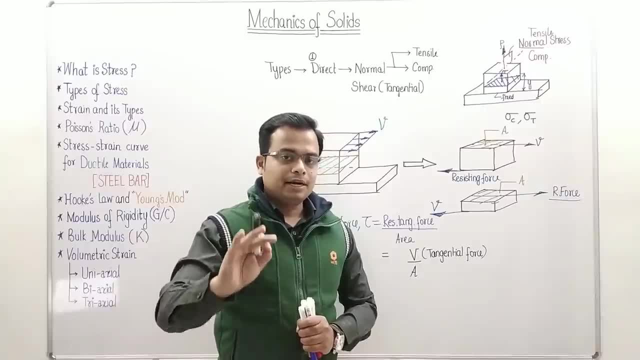 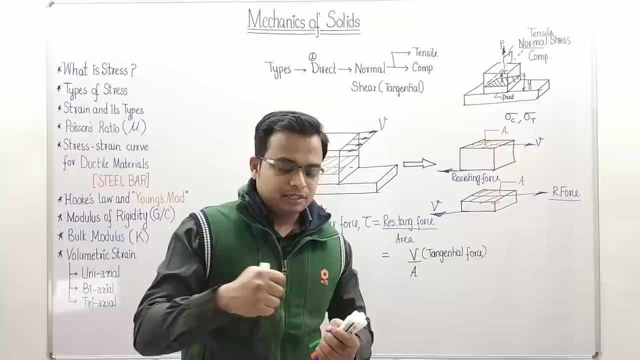 nature. If it is compressive in nature, the stress induced will be of the shear force. The shear force induced will be of the compressive nature or the compressive stress. If the load applied is tensile in nature, that means it is trying to extend the length. 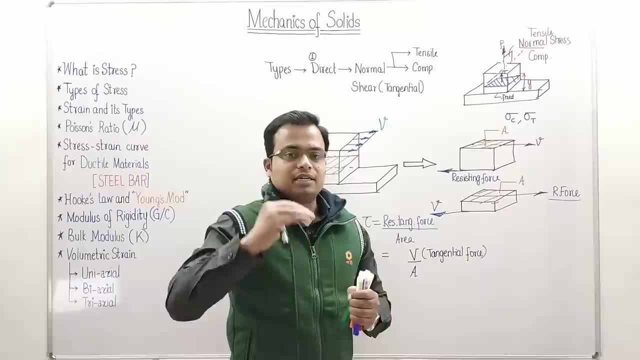 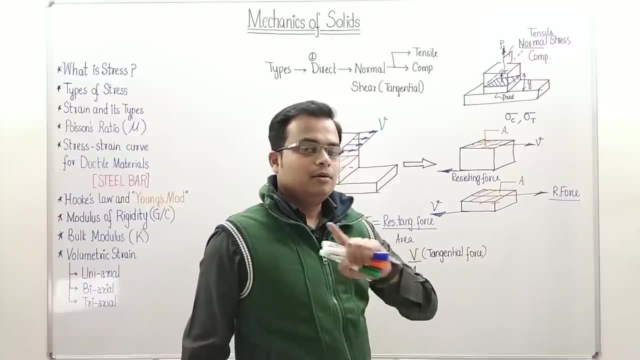 of the bar, then the stress developed will be normal tensile stress. And if the applied load is tangential to the surface, then in that case the stress developed will be shear stress or a tangential stress. you can say: So that was all about direct stress. 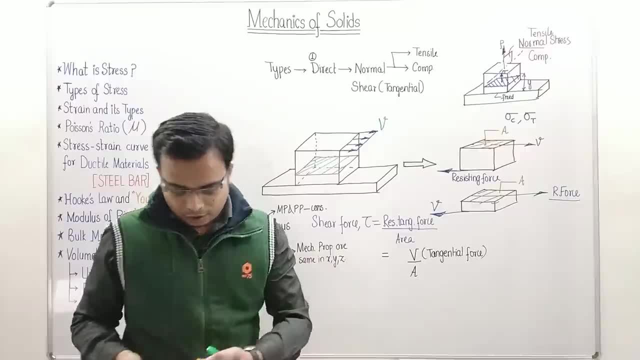 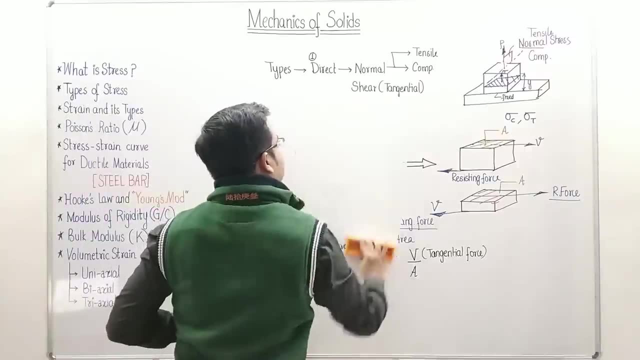 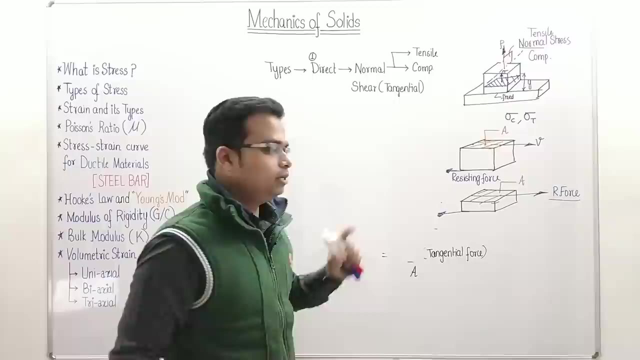 Now let us take a look at indirect stress. Here we go. Okay, So, guys, it would be better if you can just keep on pausing the video in between and noting down all of these stuff, because this is going to really help you. 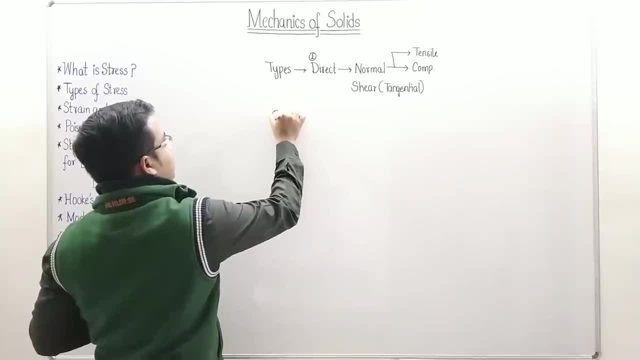 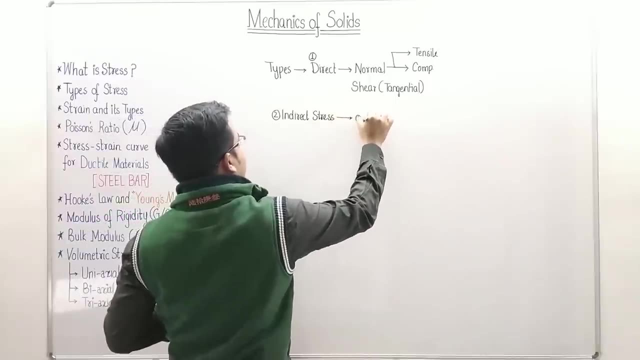 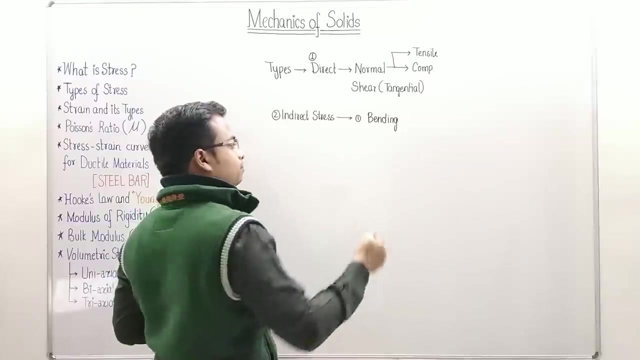 Okay, the second kind of stress that I'll talk about is the indirect stress. Now again, indirect stress are of two types. Number one is bending And number two distortion. That means whenever a beam bends, there is going to be a bending stress. 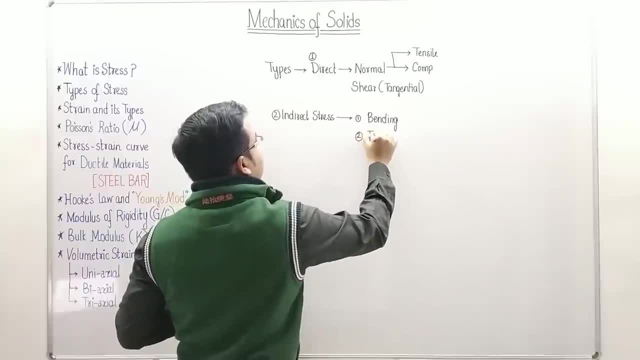 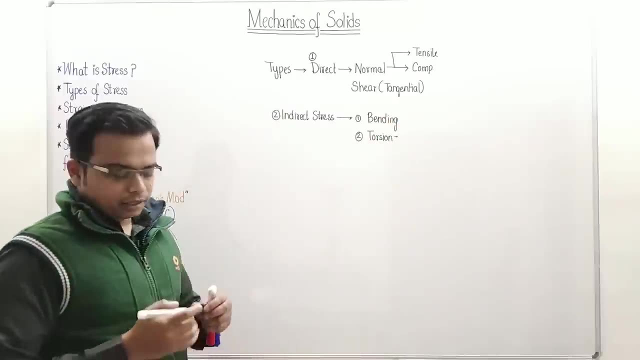 And whenever a beam twists, there is going to be a torsional stress And basically shear stresses are generated, Torsional, let me just write torsional First of all. let me just show you, rather give you a demonstration as to what is bending. 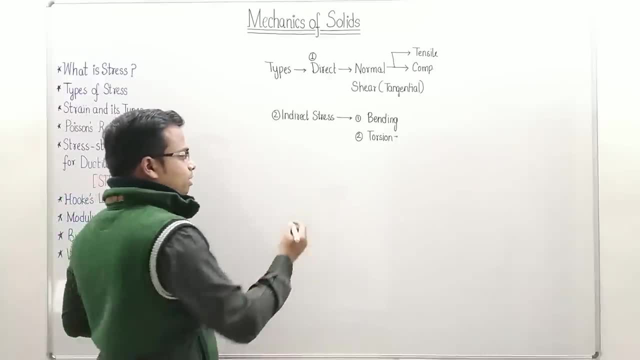 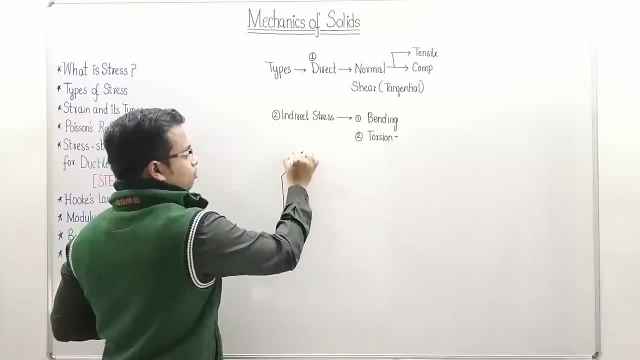 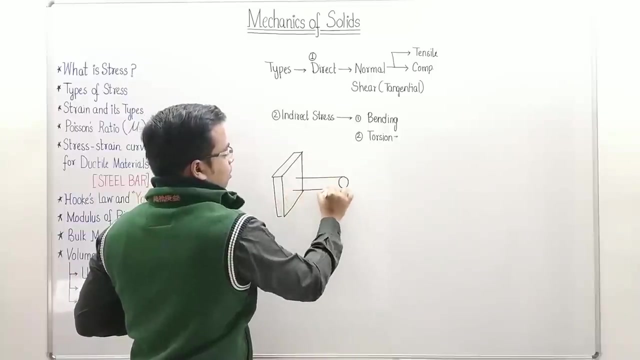 and how is it different from torsional? So just take a look at this. Let's say, this is some portion of the wall, Okay, And here we have a beam, sort of in the circular form, Okay, And what happens if I applied a load right here? 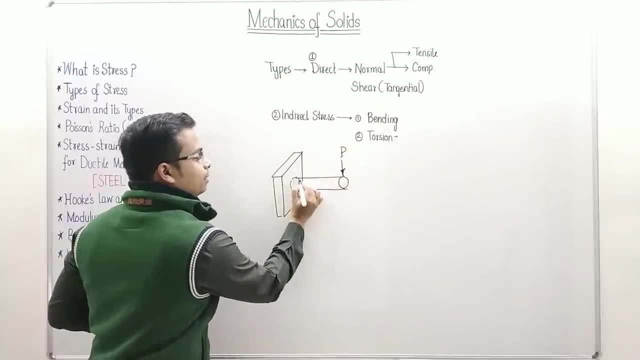 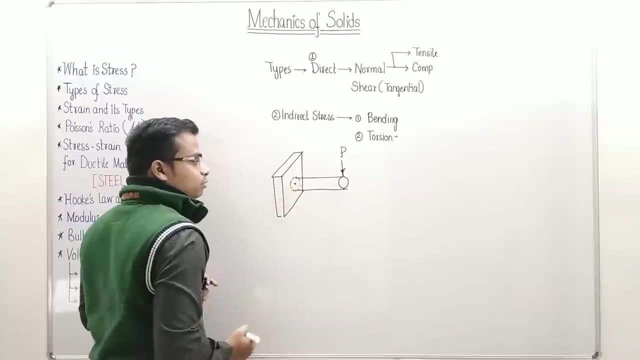 Let's say load B. There is going to be some bending moment somewhere here. There is going to be a maximum bending moment, if I can say so at this fixed point, And if I say that the length of the beam is represented by L. 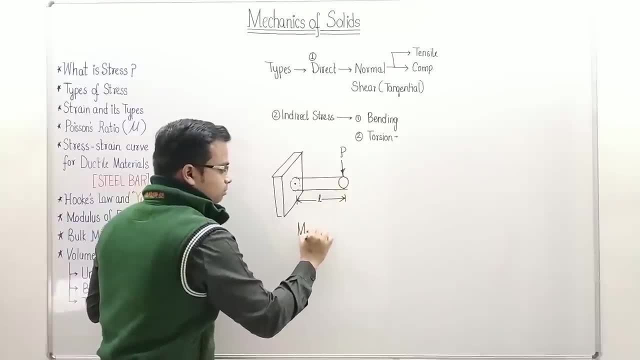 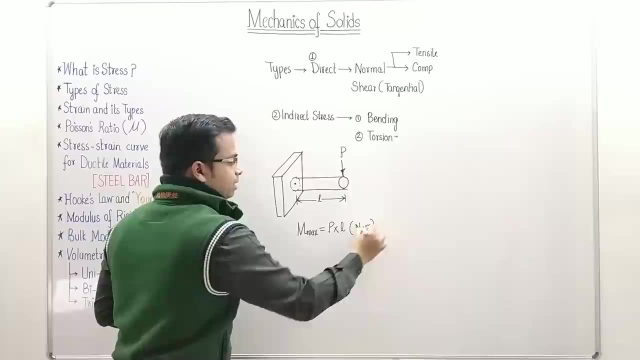 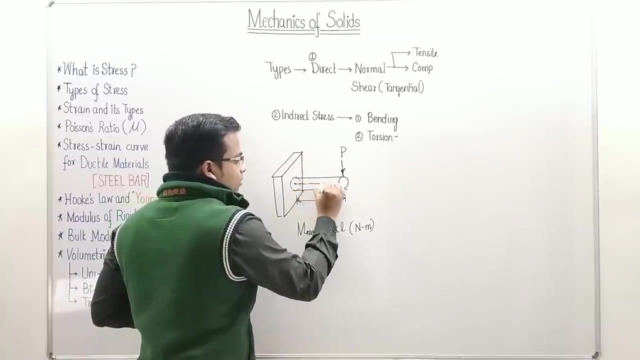 The bending moment. the maximum value of bending moment will be equal to P into L, Isn't it? And this is obviously going to work out in Newton meters, or Newton millimeters, whatever. So let's say this is the axis When this load is applied, obviously there is going to be some kind of deformation. 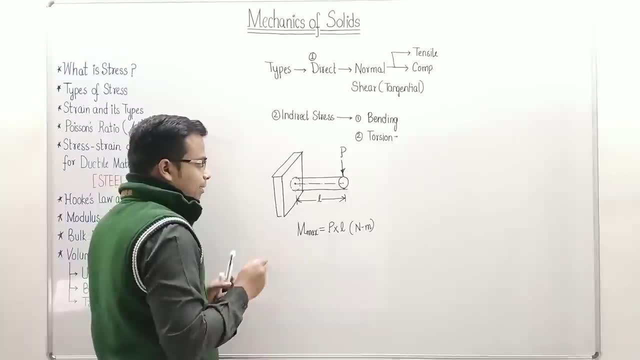 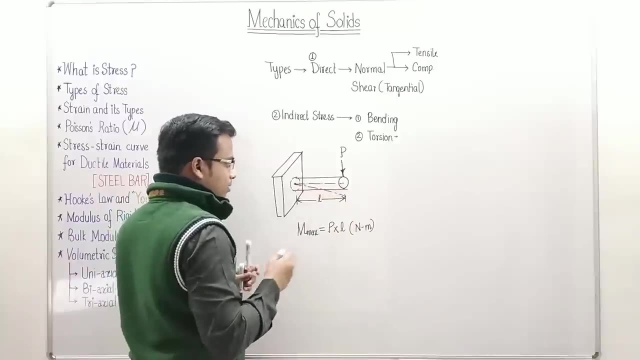 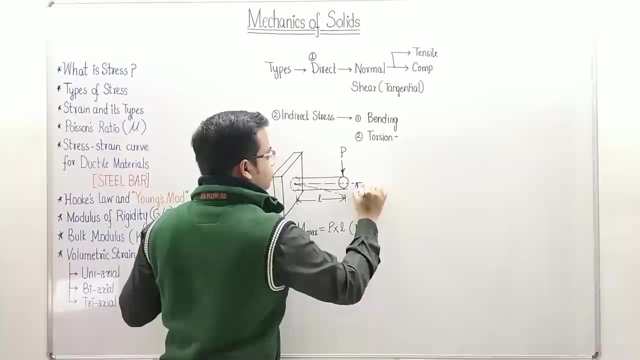 What will happen After some time, The axis will bend like this: Okay, And this over here is what is referred to as the deflection or the maximum deflection. This right here is the deflection Right. So whenever a beam bends, there is going to be a deflection at all the points across the axis. 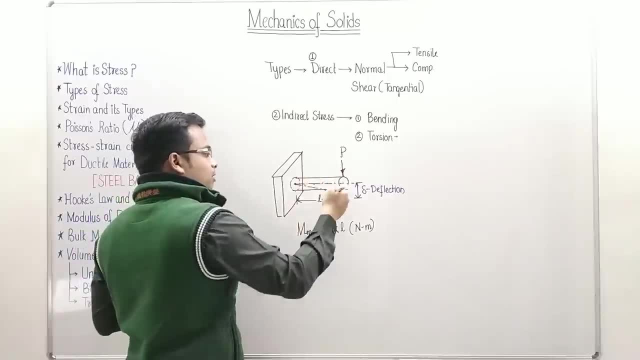 But at the free end. in case of this cantilever beam, at the free end we'll see a maximum deflection. Cantilever, Okay Beam, And this is circular cross section, by the way. Okay, So what is torsion? 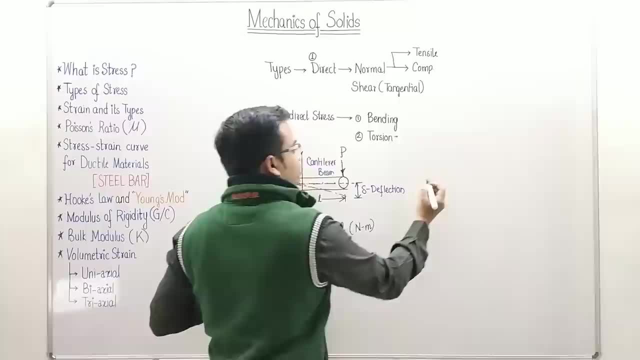 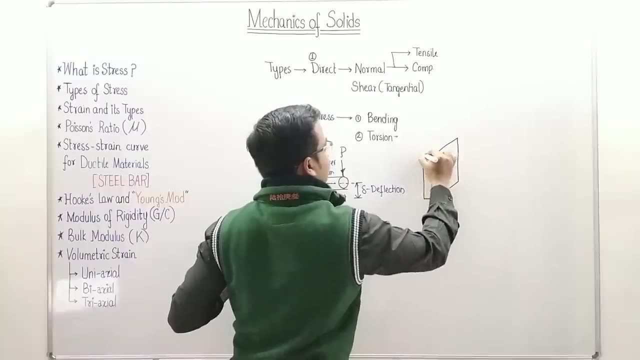 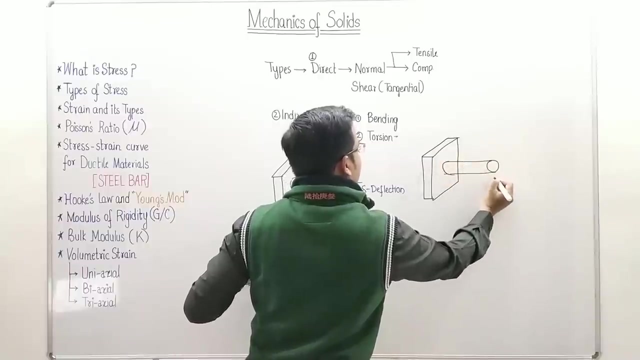 Now take a careful look at this Again. the object is going to remain same. Let me again make a wall over here like this, And let me just extend this Right. What if I? This is fixed. What if I twist it like this: 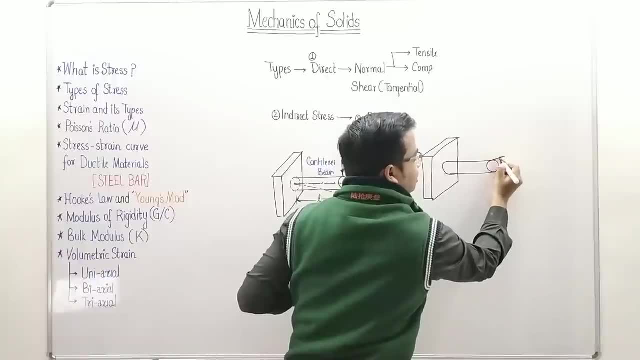 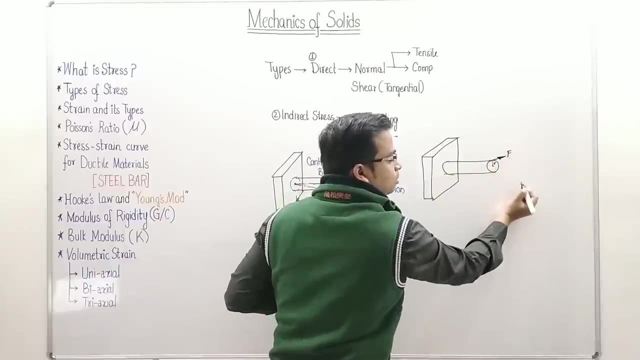 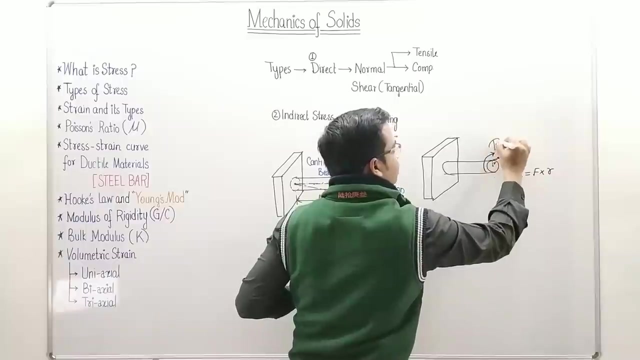 Twist it. What if I apply a force which is tangential to this circumference And if, say, this radius is r, This is force. Okay, Then some sort of torque is going to be developed, force multiplied by r. And this gives rise to twisting moment. 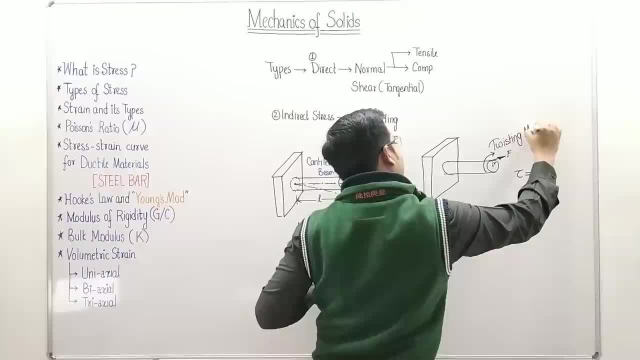 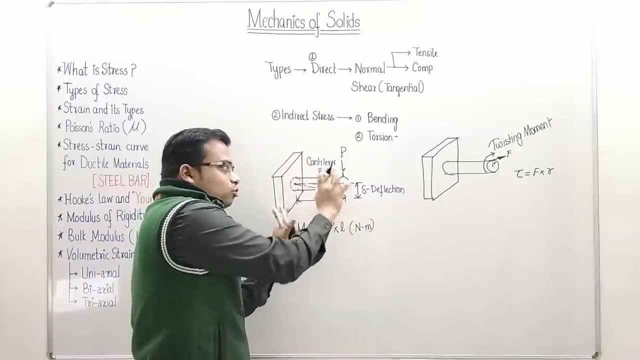 This is nothing but twisting moment. Rather, this is what is referred to as twisting moment, And here the beam is bending. So, With regards to bending, the moment produced is bending moment And at the fixed point or at the fixed end, the bending moment is going to be maximum. 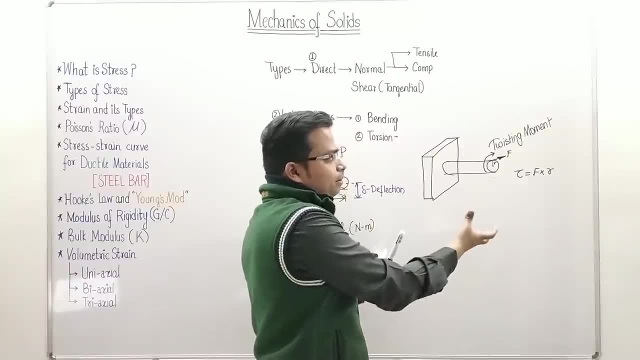 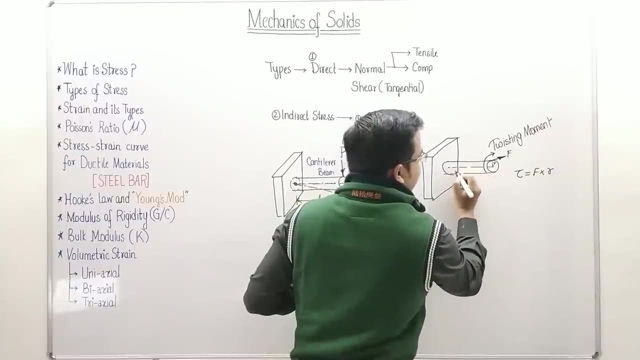 Here you can clearly see that we are not bending the beam, But what we are trying to do is we are trying to twist the beam, Okay, And in that case original axis would have been here, But now, after twisting, it will go somewhere here. 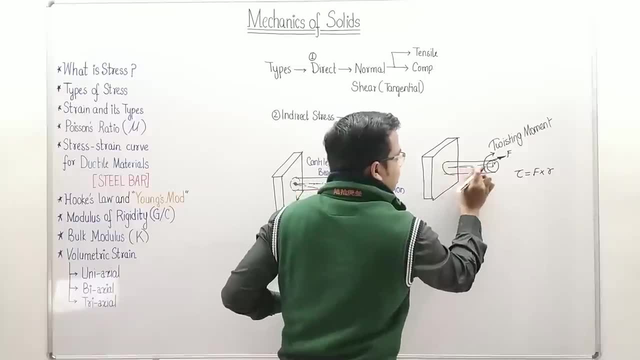 Like this: Okay, Not the axis. But if I say that Initially, Initially, Let us just try to understand this. Initially, let us say the fiber was here, But after twisting, the fiber will go here. Okay, By a certain angle. 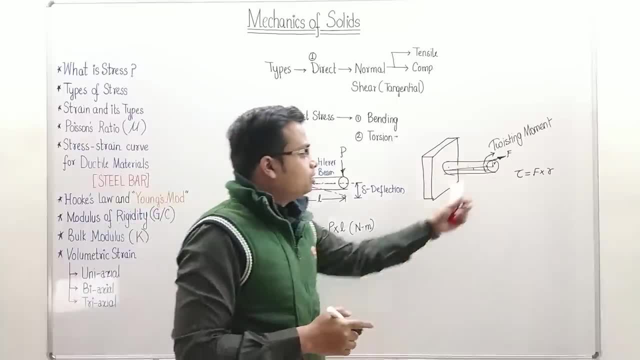 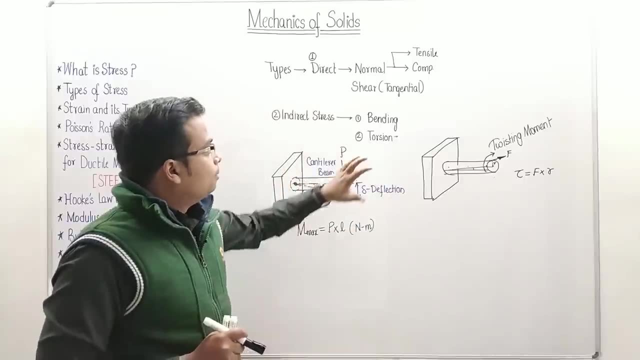 And we can actually work out how much angle that is equal to with the help of the torsion formula, And all of those things will be worked out in this particular lecture series on mechanics of solids. This was all about bending. Okay, The stress generated in case of bending. 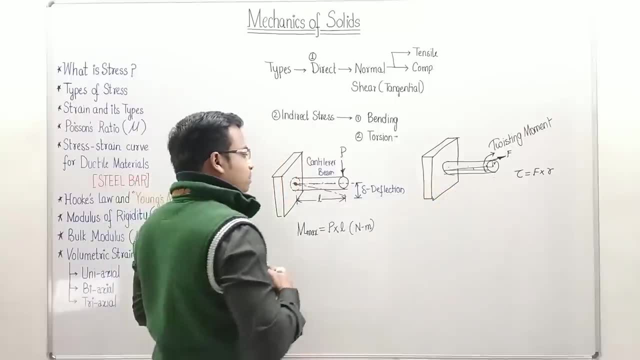 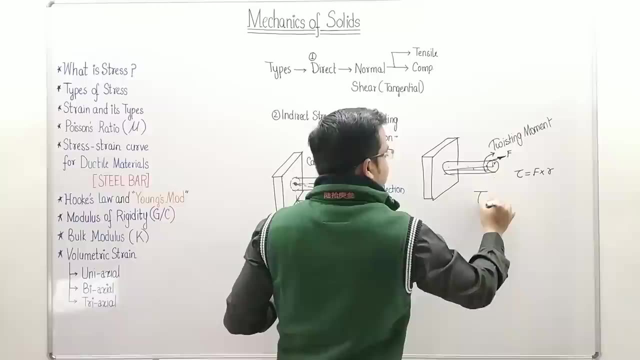 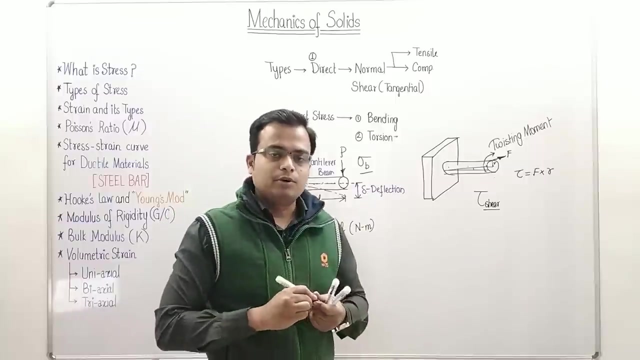 And this is twisting moment. Now the bending stress is basically represented by sigma b And the twisting moment. in case of this twisting moment, shear stresses are generated, And the formula for both of them will be dealt in the upcoming chapters. Right now, we are going to talk about simple stress and strain. 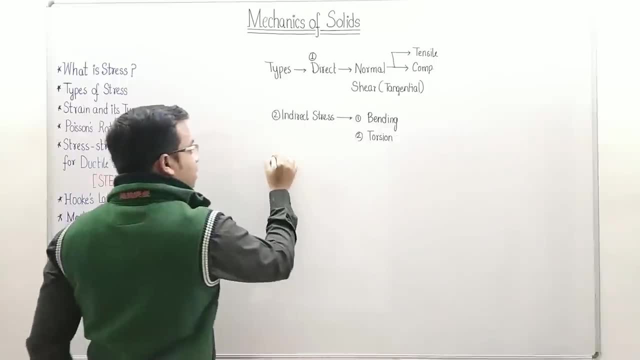 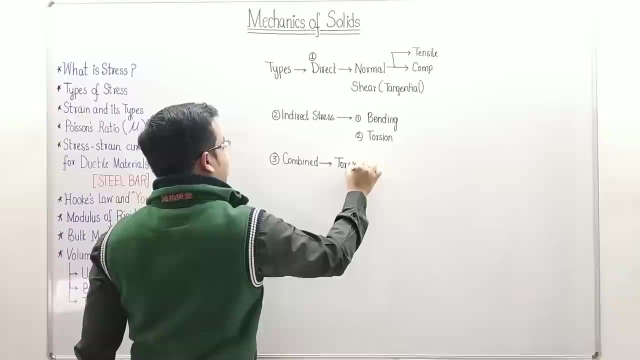 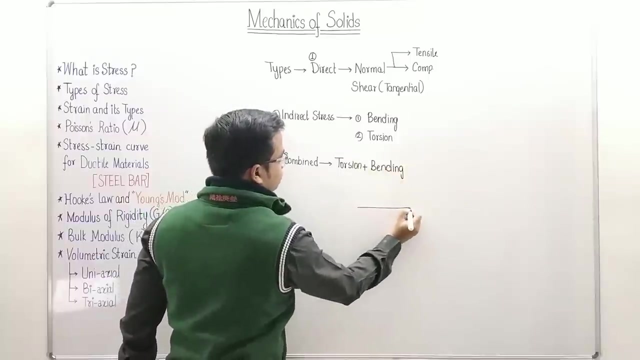 So let us continue this Now, guys. the third kind of stress that I am going to talk about is the combined one: Torsion and bending. Both of them are happening at the same time. Okay, So if you have got an object like this, just like the previous one, 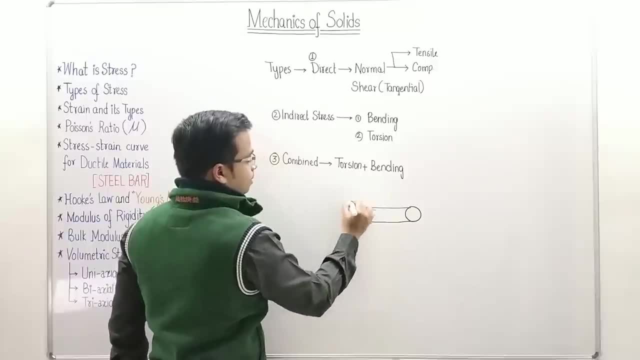 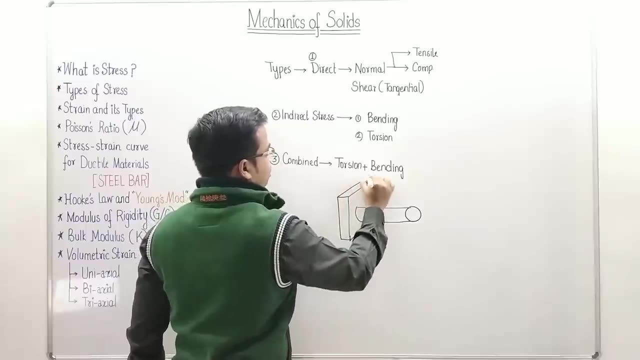 And let us just say it is fixed Right, Fixed to a wall. let us say, If there is twisting moment and if there is also a load at here, So there is going to be twisting moment over here and there is going to be bending moment. 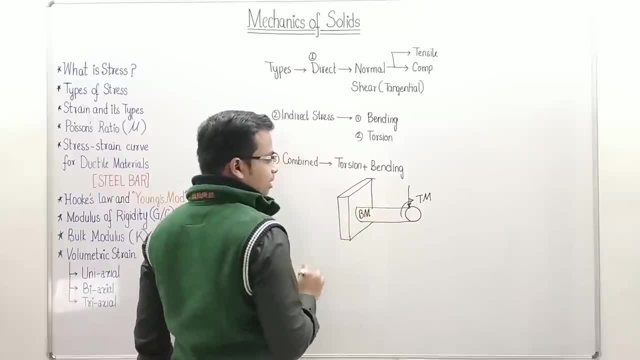 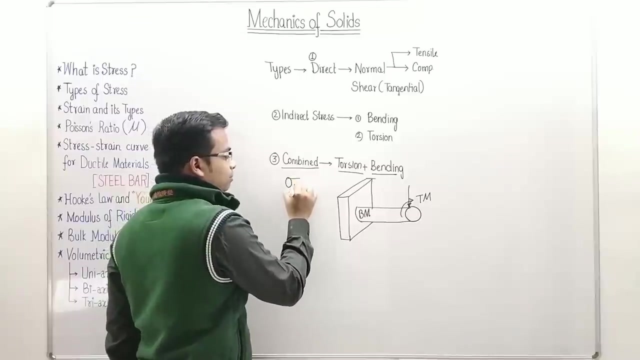 at the fixed end, Rather the maximum bending moment, If both of these things are happening at the same time. If both of these things are happening simultaneously, Then this gives rise to the concept of combined torsion and bending, Where both the effects, rather the stress, has to be calculated, considering both bending. 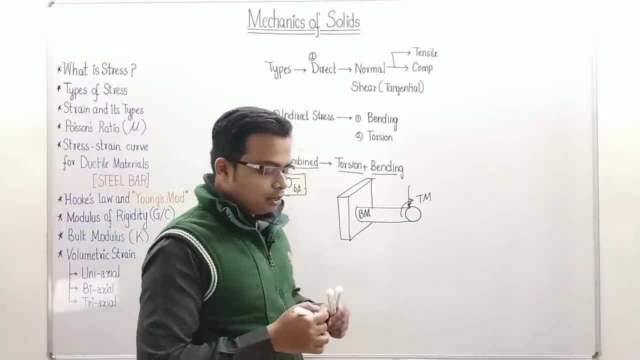 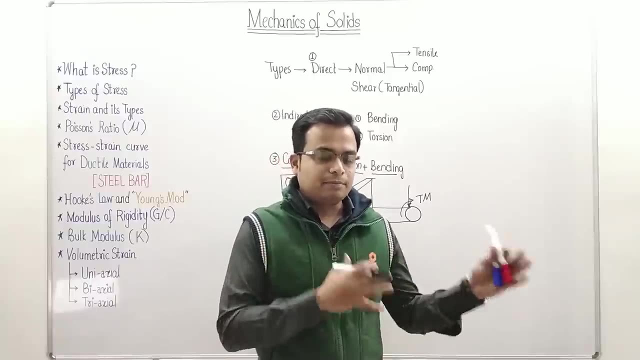 as well as torsion. So we will work out all of these things, But initially it is very important to understand the basic principles of stress. Okay, So bending of beams, it is a separate chapter. Then, with respect to torsion, there is again a separate chapter. 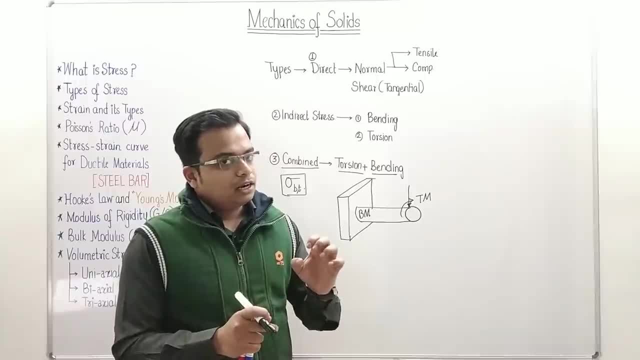 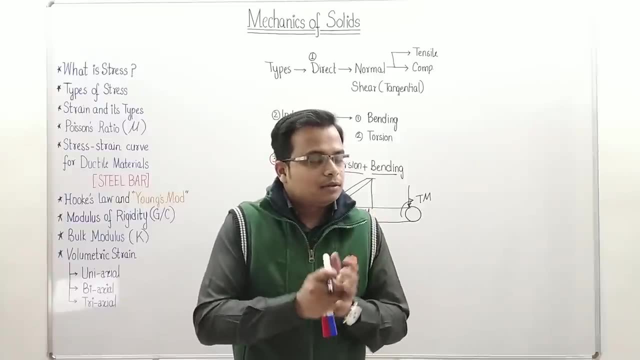 And then there is a combination in which you will see a particular machine part is subjected to both torsion and bending, And how these stresses can be calculated. in that case I will be working it out for you, But that is going to happen in a later lecture number. 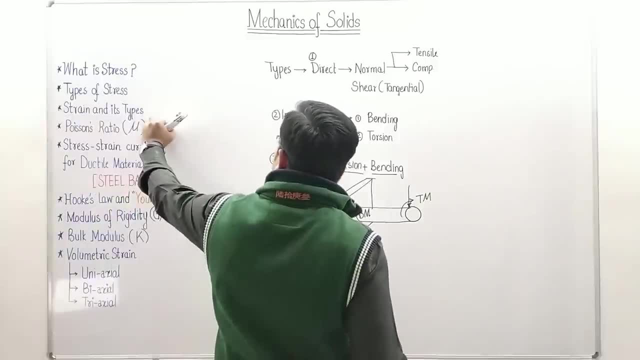 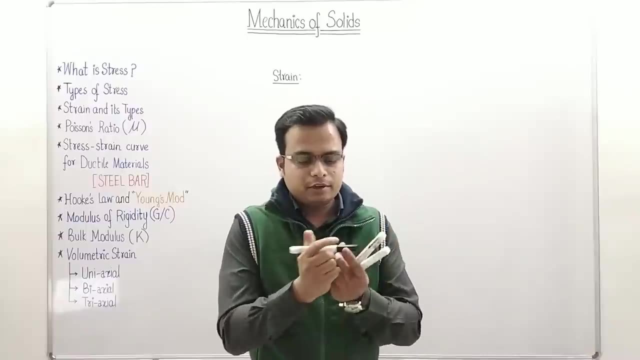 Okay Now what we are going to do. We are going to study strain and what are the different types of strain. So just think about this. If you have got a member over here, Okay, If I just consider this, If I apply load, what will happen? 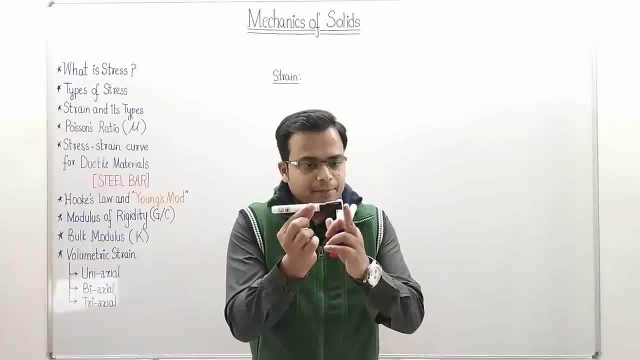 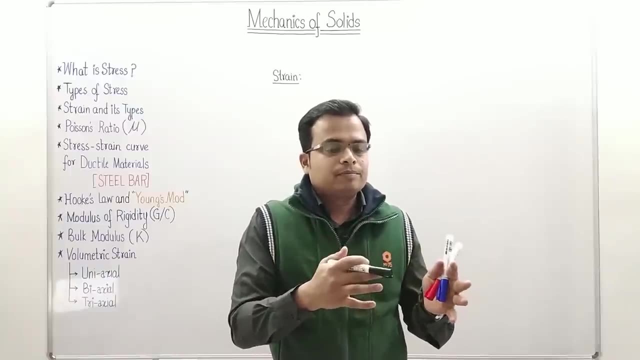 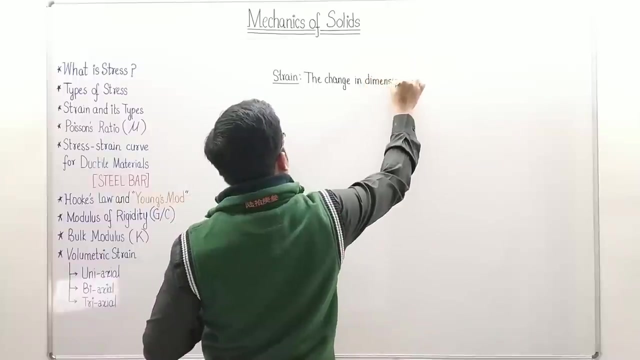 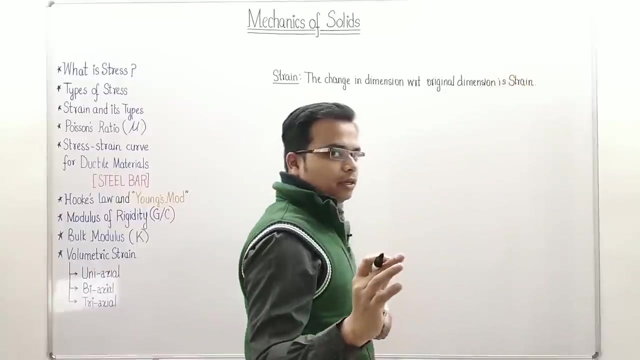 There is going to be some deformation, It might happen that the length may increase from here or from here, Right. So the change in dimension with respect to original dimension is what is referred to as strain. Let me just write this One more thing which you guys should note: that dimension, it is a ratio of dimensions. 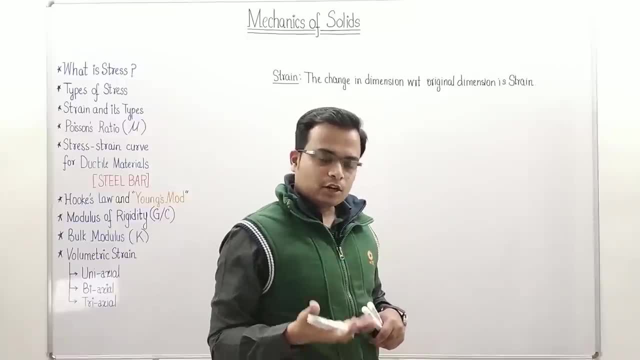 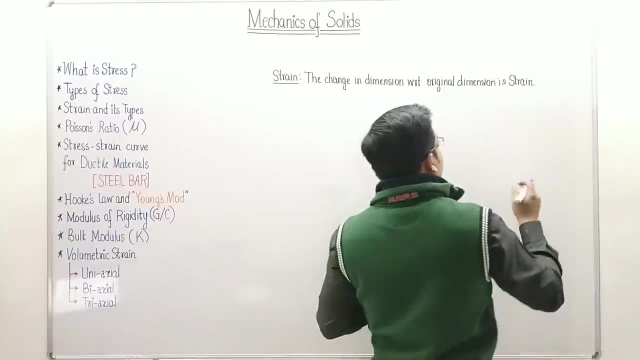 In the numerator you have change in dimension And in the denominator we have the original dimension. So dimension divided by dimension is a dimensionless quantity. you can say: Okay, Not a dimensionless, but a unitless quantity, It is unitless. 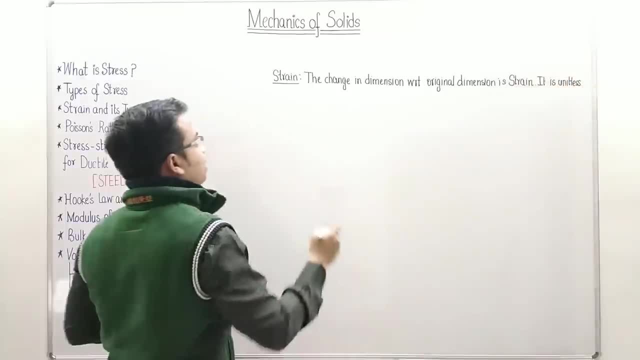 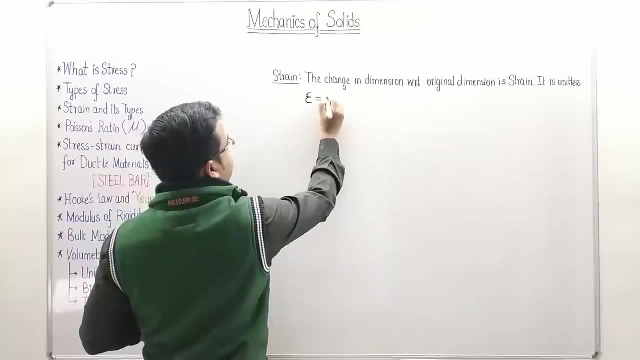 Now, if I were to formulate this mathematically, strain is basically represented by this Greek number or this Greek alphabet, Epsilon, you can say. Some people also write strain as simply E, So I am going to be following this: E, It. 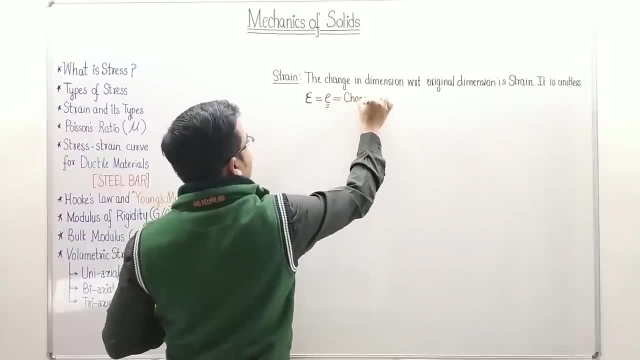 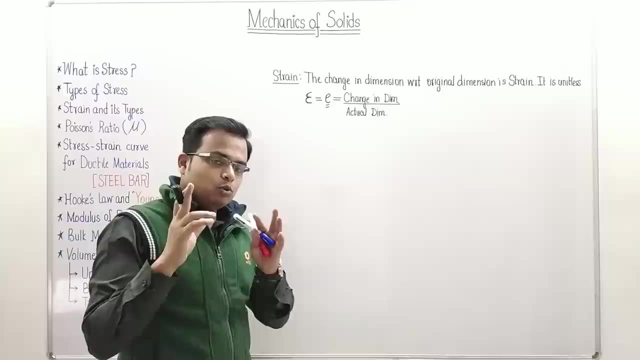 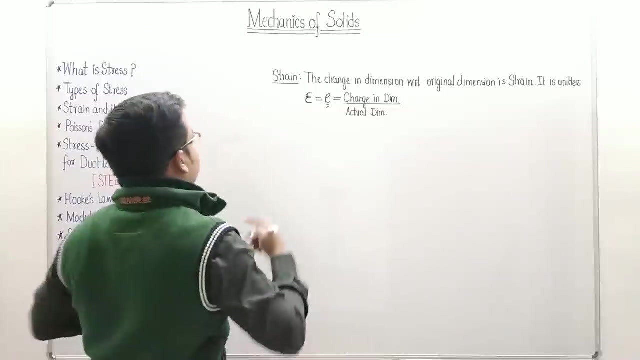 is the change in dimension with respect to original dimension. Now again, strain can be divided into two categories. One is the longitudinal strain or the linear strain, and the second type is the lateral strain. Let me just illustrate the different types of strain. Number one is the linear strain, or longitudinal strain. 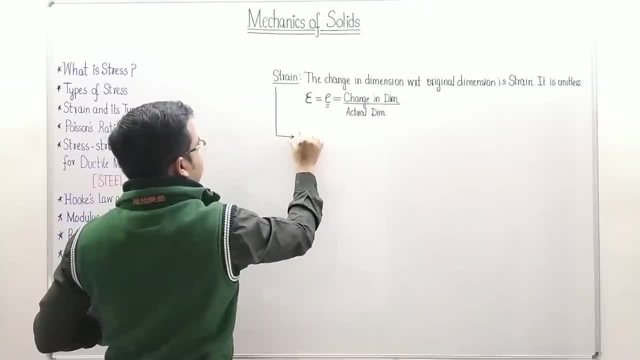 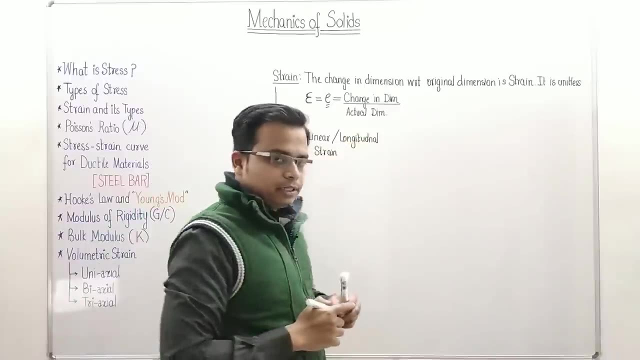 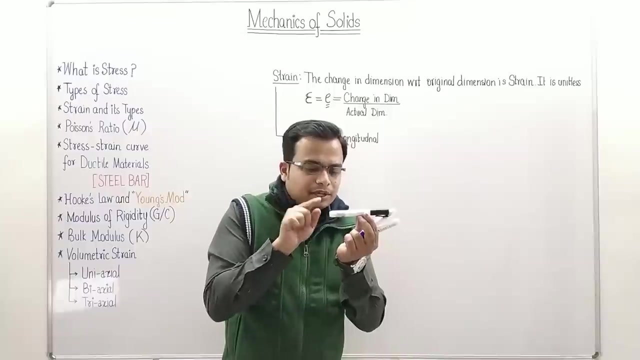 Now, guys, if you are applying load, it is similar to strain factor. Let us write this: E, This is the strain factor And this is the longitudinal strain, or the longitudinal strain. Okay, If you are applying load over here and over here, and obviously there is going to be some, 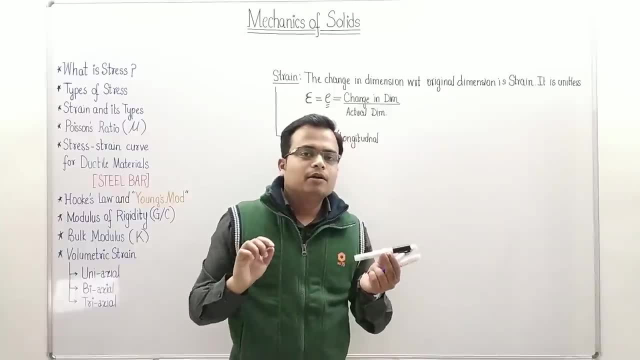 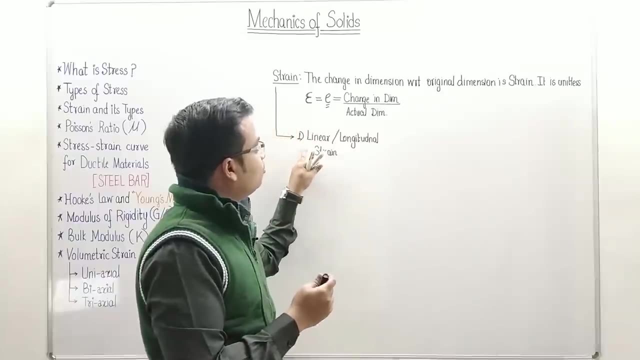 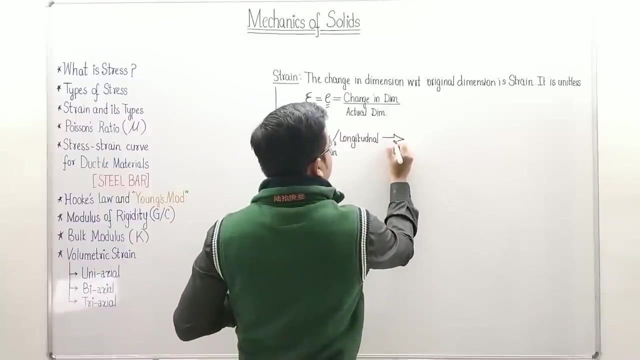 increase in length along this direction and this direction. So if there is a change in dimension along the direction of force, then that sort of a strain is what is referred to as a linear or longitudinal strain. okay, along the direction of force. So in short, I can just write it as it happens in the: along the direction of force. 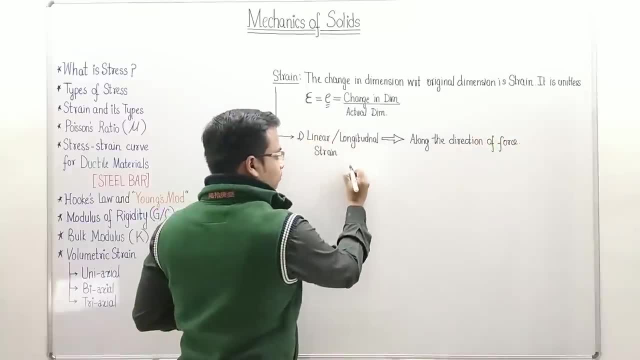 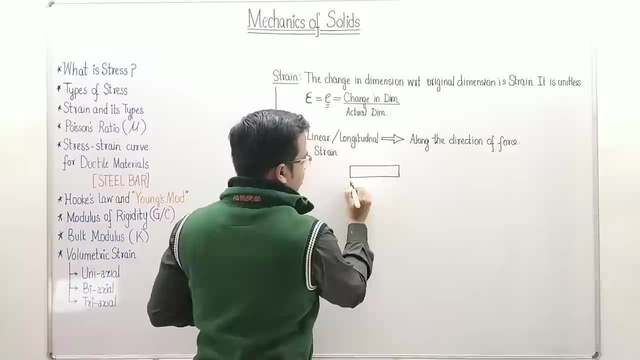 Just to give you a demonstration, let me take a very plain case. okay, Let's say that the original length is represented by n and let me just fix up this portion. Let me just fix this. What happens if you apply a load P? 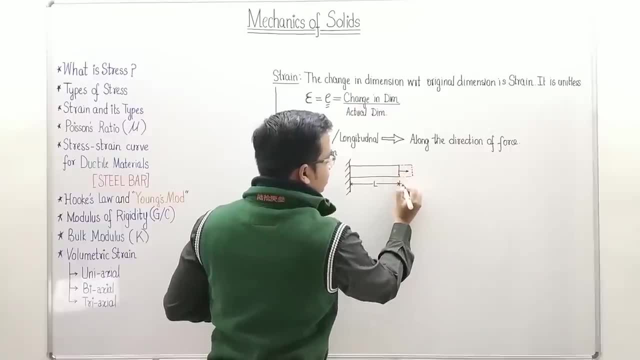 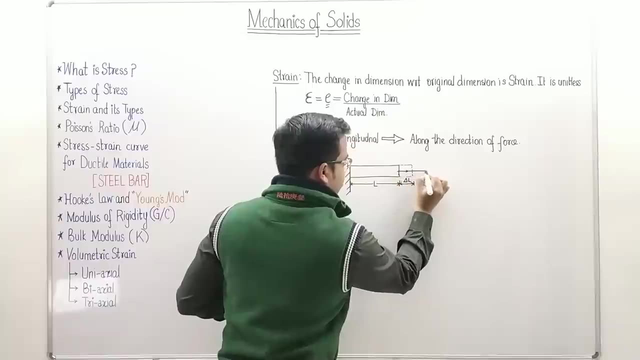 So after some time you are going to realize that the length of the bar has increased by a certain amount and this length is represented by, let's say, delta n. okay, The force applied is this much. Let's say we have applied a force P which is going to pass through the axis and axial 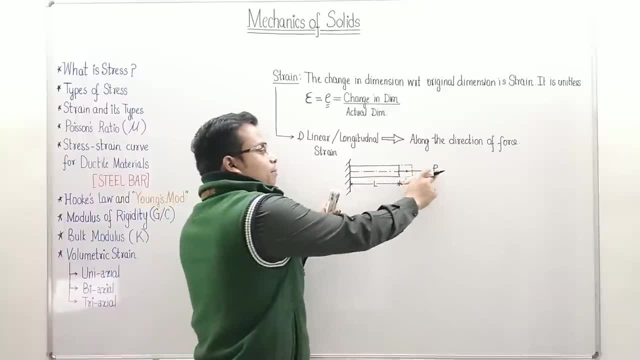 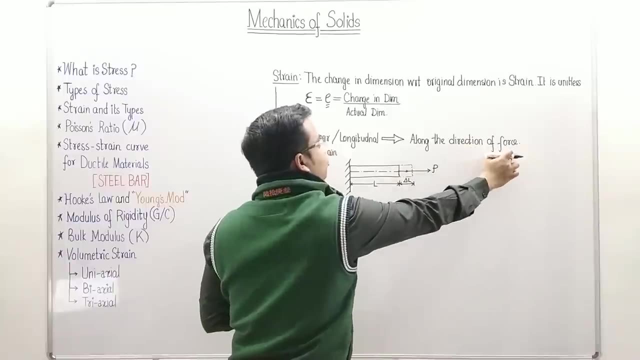 load is something that we have taken into consideration. Due to this load applied, there is an elongation in the direction of load. So if the elongation takes place in the or along the direction of force, then that sort of a strain is a longitudinal or a linear strain. 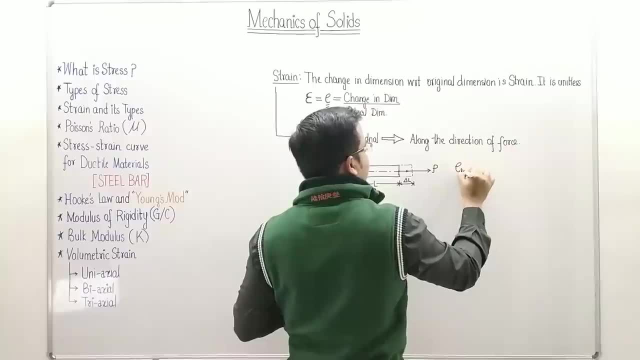 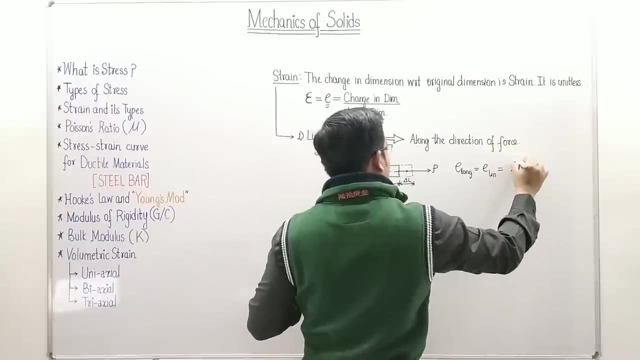 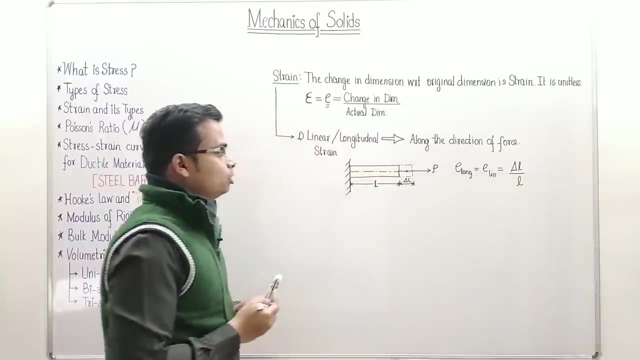 And if I were to formulate this mathematically: E-L-O-N-G or E-L-I-N, Okay, Okay. So in linear or longitudinal change in dimension, that is delta L divided by the original dimension, that is L. small l, okay, small l, fine. 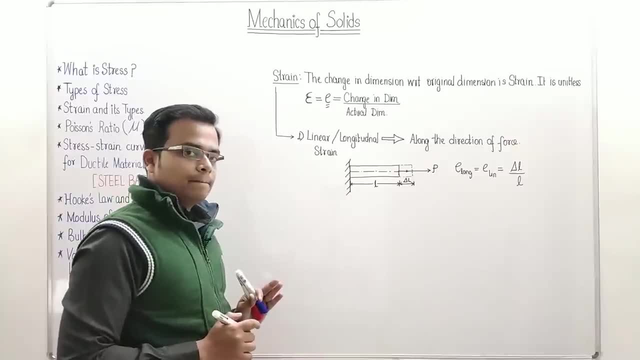 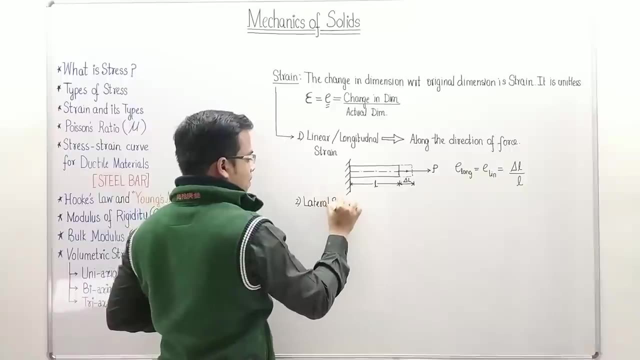 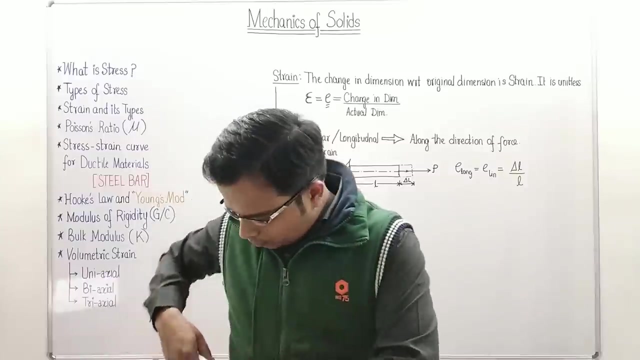 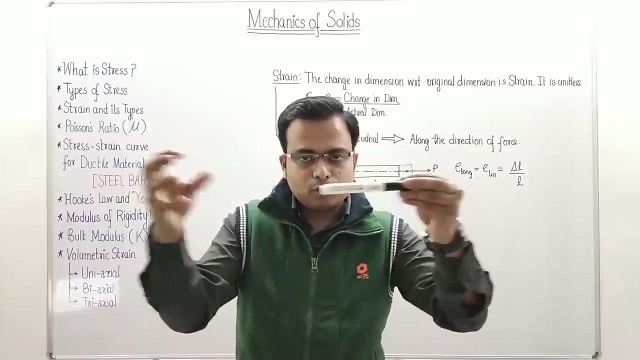 So this is how you can work out linear or longitudinal strain, And some of you guys might have worked out what exactly could be lateral strain. Okay, now, in order to understand lateral strain, just watch this. Hmm, So now apply load P P from both the direction. what will happen? 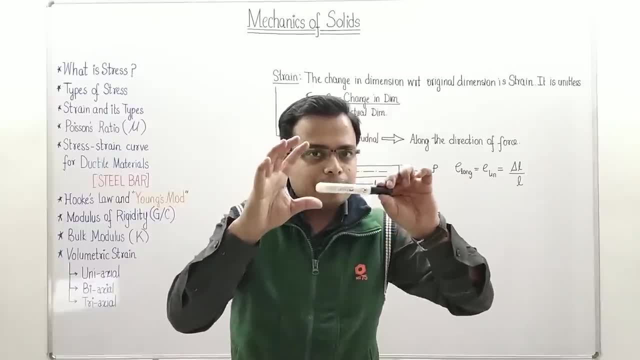 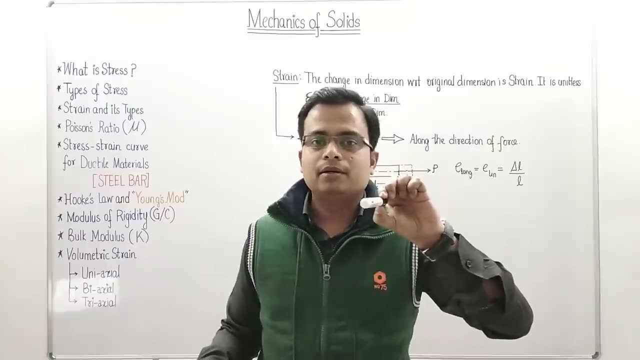 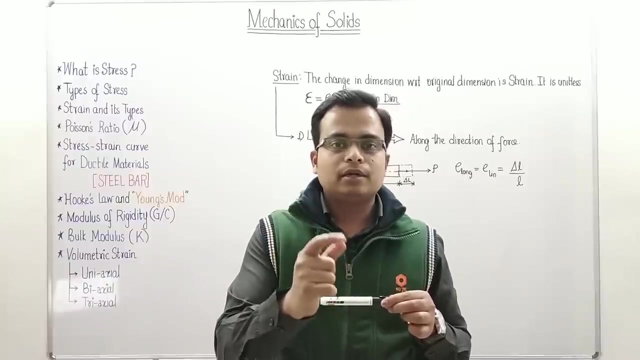 It will elongate along the direction of load, But at the same time, if you watch from here, this diameter will continuously reduce, isn't it? That is lateral strain, a strain which actually happens simultaneously. perpendicular to the direction of applied load is the lateral strain. 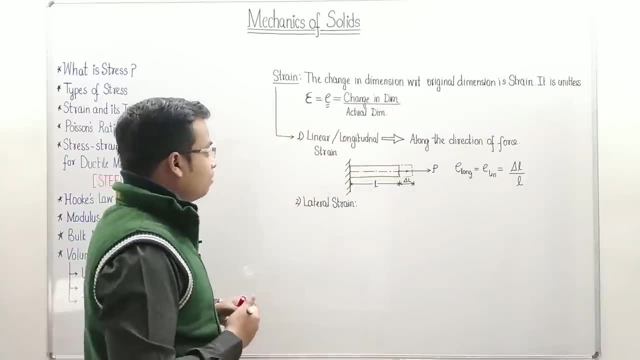 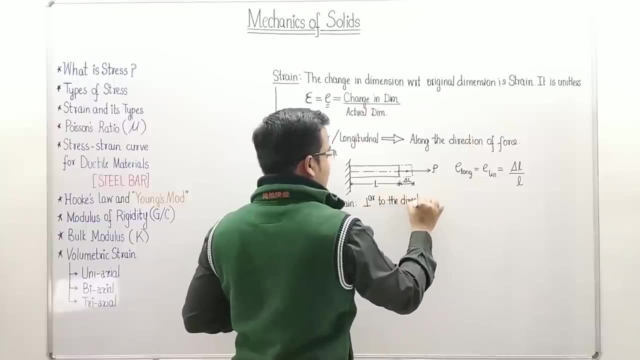 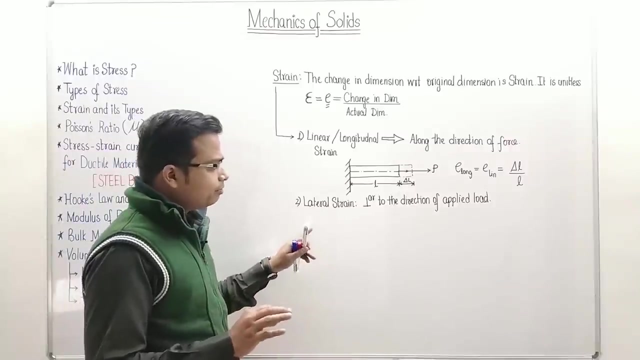 Okay, Okay. So to understand this- well, I've got to. first of all, let me just write this: This is perpendicular to the direction of applied load. Now let us try to understand this lateral strain with the help of a very simple example. 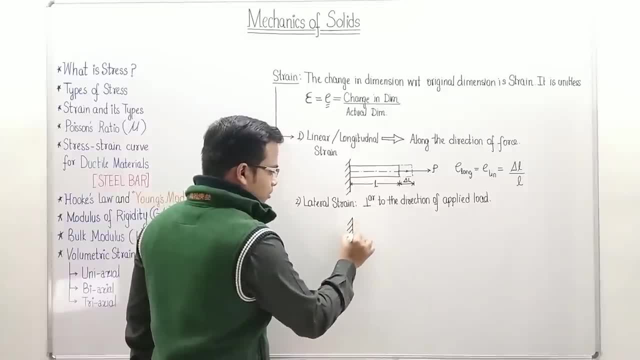 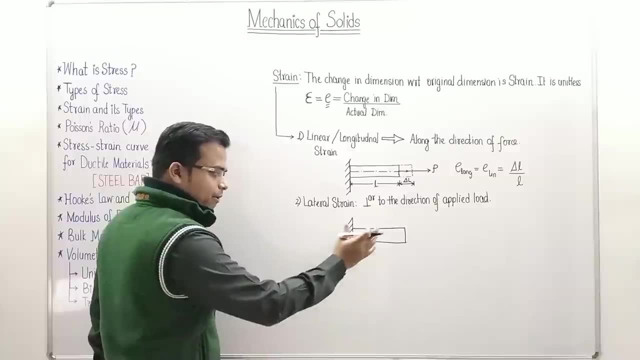 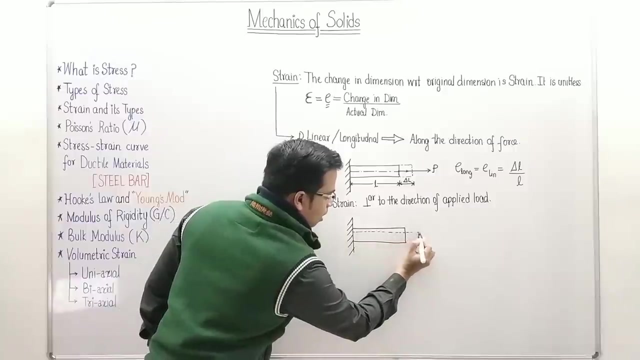 And here we go. Let me just first of all have a fixed support and we have a member like this: Okay, What we'll try to do, we'll apply a force along this direction, Right, And now what will happen is this? okay, something like this will happen. 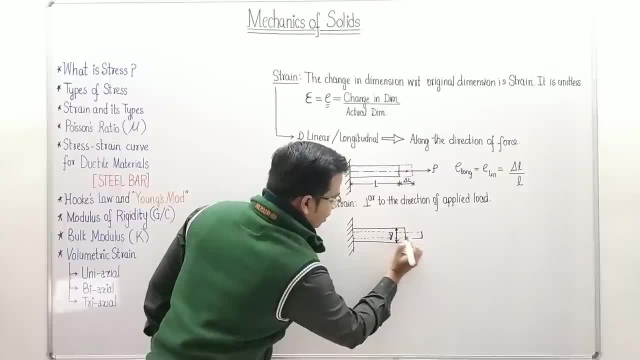 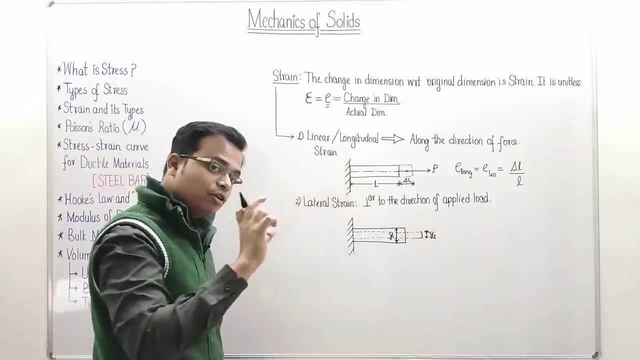 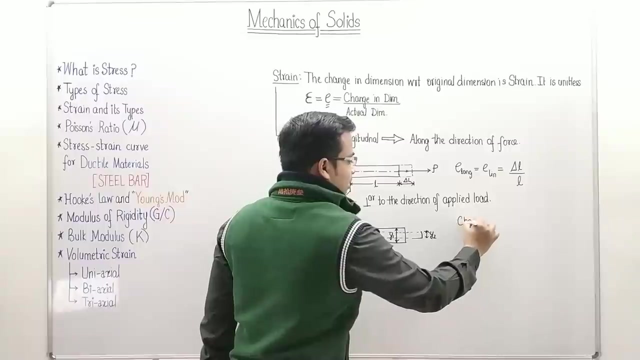 Originally this was Y. Let's say this is Y1, initially it was Y1, now it has become Y2.. So obviously some deformation has taken place. Some reduction in length has taken place. That reduction is the change in length. Okay. 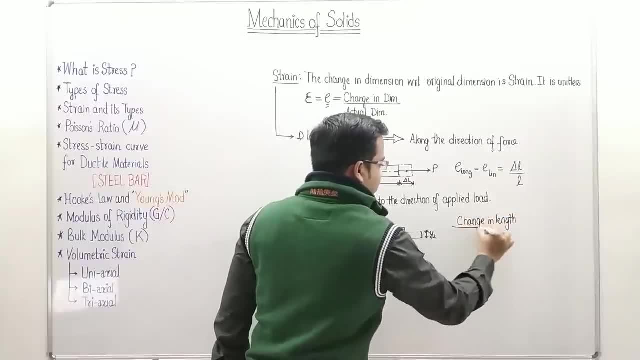 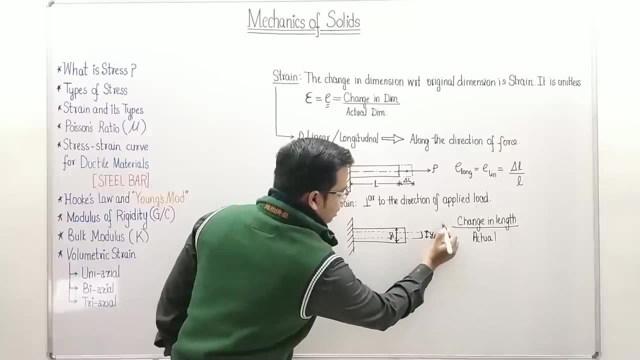 Change in length, Let me just write it over here. And that change in length with respect to the actual length is going to give you the lateral strain. Now, guys, remember we are applying force along this direction, force applying along this direction. 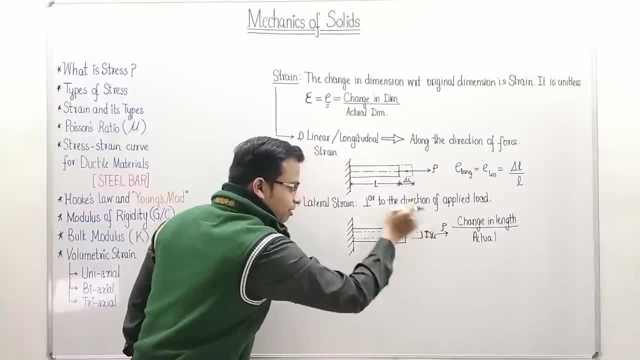 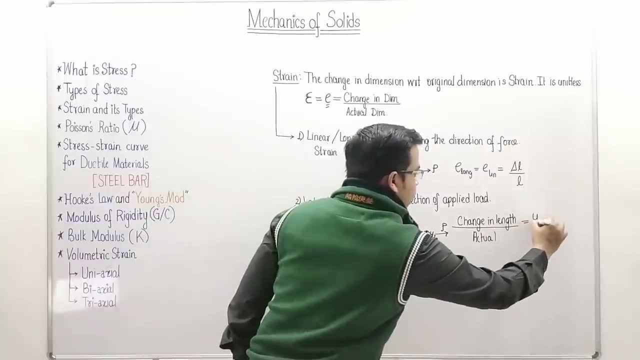 And this inner direction perpendicular to that of the applied force. if you watch carefully, this is reducing. Okay. So the change in length is how much Y1 minus Y2.. That's going to be equal to Y1 minus Y2 with respect to the original actual length that. 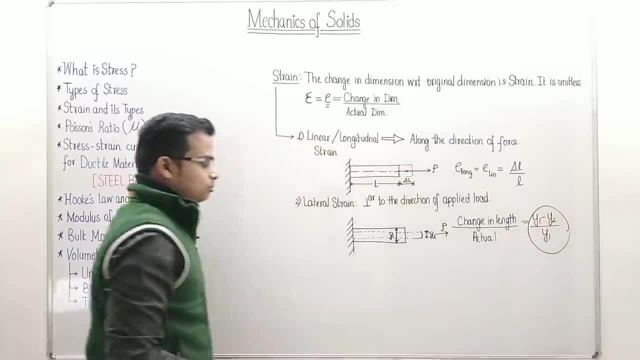 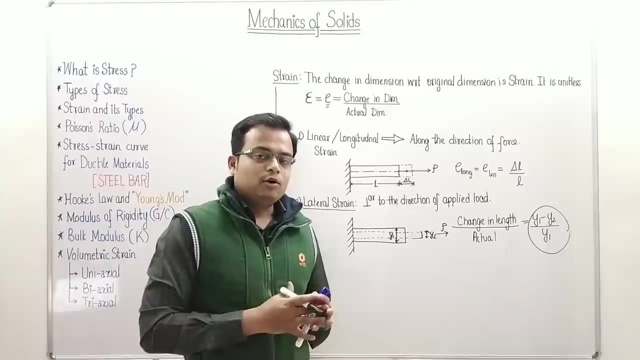 is going to be Y1.. So this ratio also Okay. This is what is referred to as the lateral strain. Always remember: if, in the direction of applied load, we are working out the change in dimension with respect to original dimension, that is what is referred to as the linear or longitudinal. 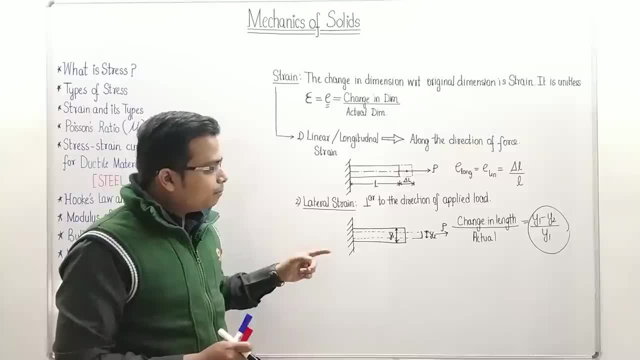 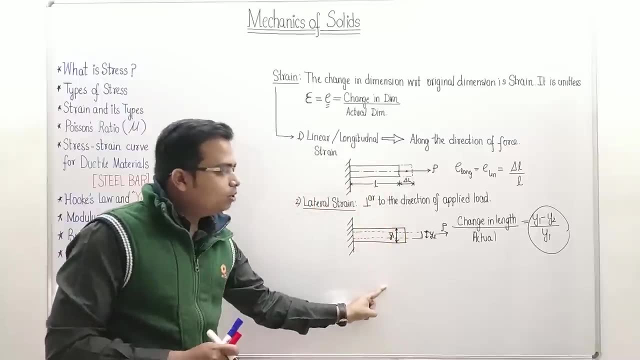 strain. Now, if you're trying to make an assessment perpendicular to the direction of the applied load somewhere here- this is the applied loads direction and this is in a direction perpendicular to that of the applied load- then in that case the change in dimension 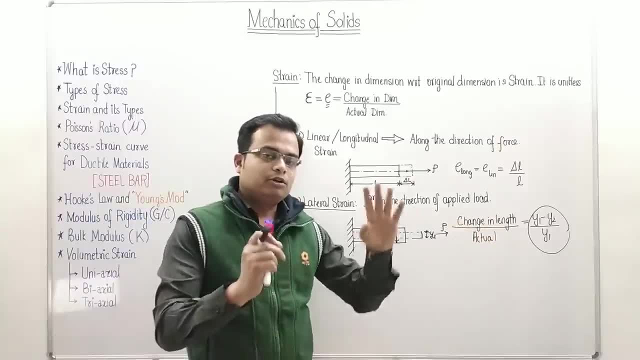 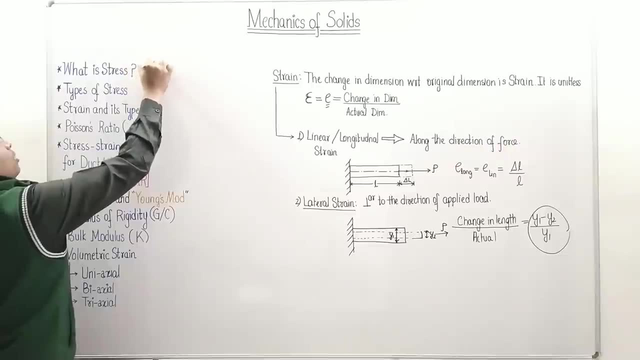 Y1 minus Y2 with respect to the applied load, Y2 with respect to the actual dimension is going to give you the lateral strain. Okay, So we've discussed a whole lot of topics, we've learned what is stress, we have seen 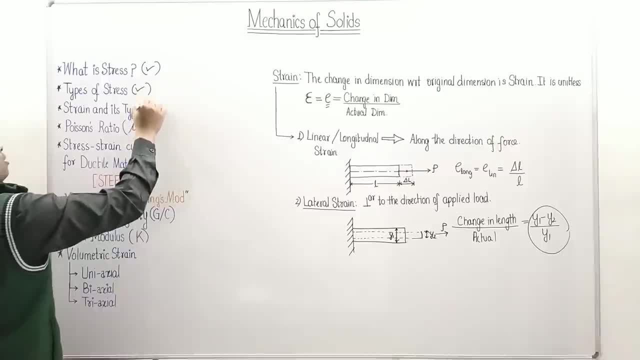 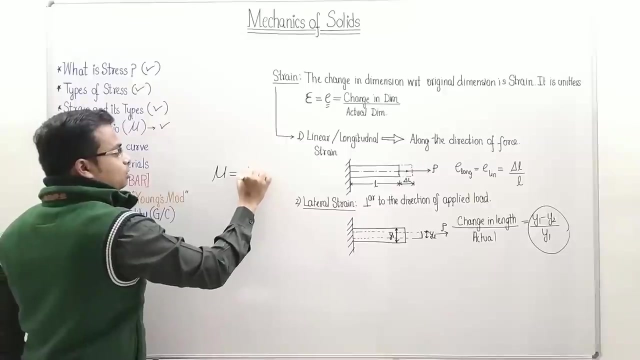 the types of stress in the form of direct, indirect and combined forms. you've seen strain and its types. Now, another term which is extremely important is the Poisson's ratio. Now, this is basically something which is represented by mu Poisson's ratio and it is actually 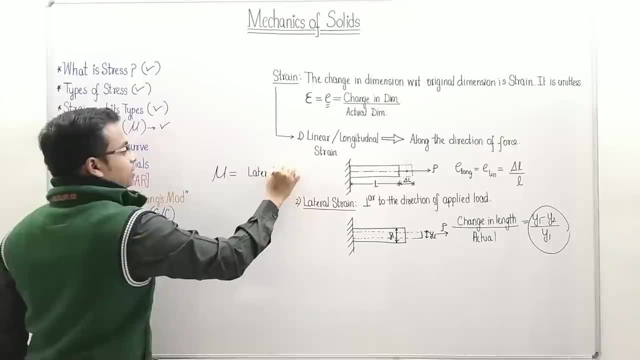 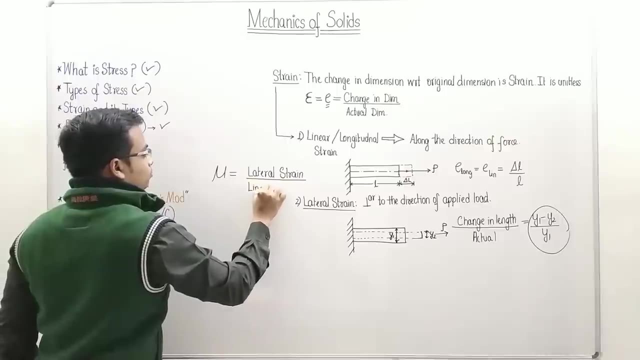 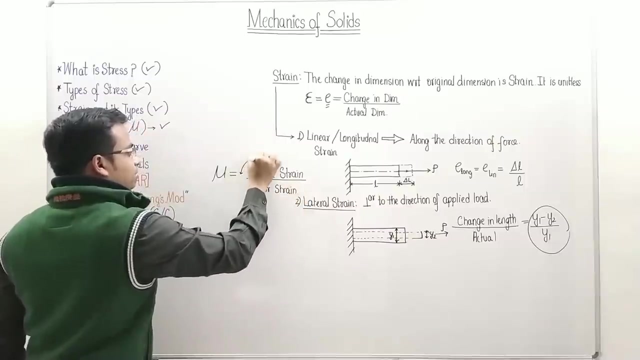 equal to the ratio of 2 different types of strains: lateral strain with respect to linear strain or longitudinal strain for the same material or for the same object. Okay, In some of the books you will see that over here they put a negative sign. 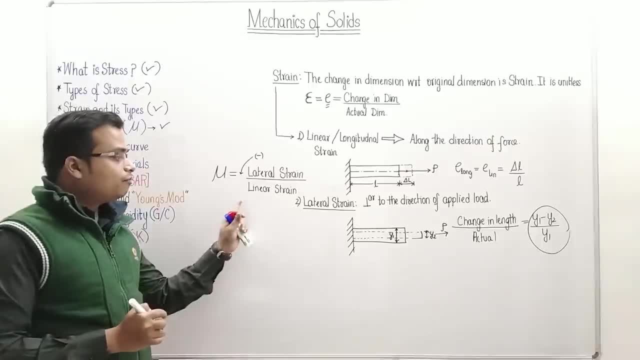 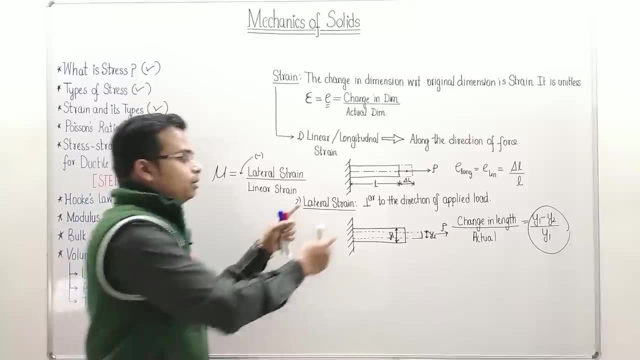 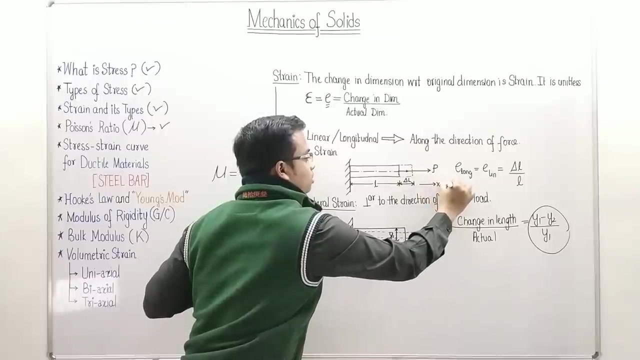 But the reason being very simple: if in one direction there is elongation, then obviously in the perpendicular direction there is going to be reduction. Here you see, Along x direction there is elongation. okay, Along this x axis. what do you see? You see, or you. 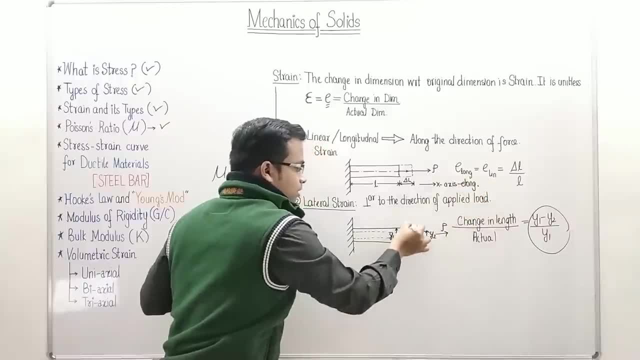 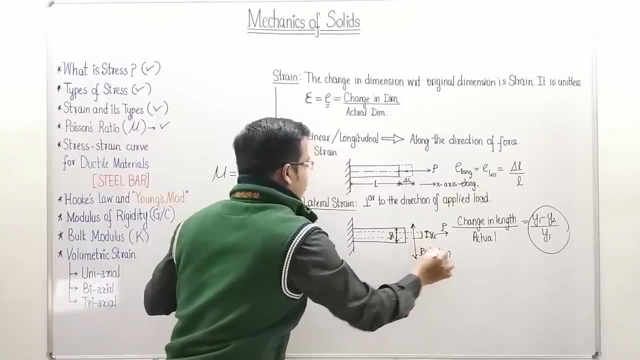 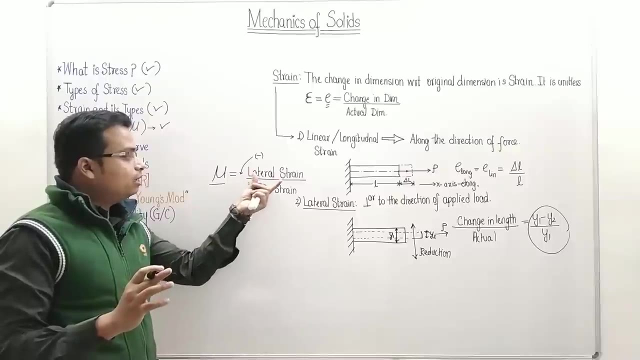 experience elongation. But whereas in this direction, in the y direction, what do you see? You see a reduction. That is why what we actually do is we always put a negative sign in this Poisson's ratio. So Poisson's ratio, remember this, is actually a ratio of lateral. 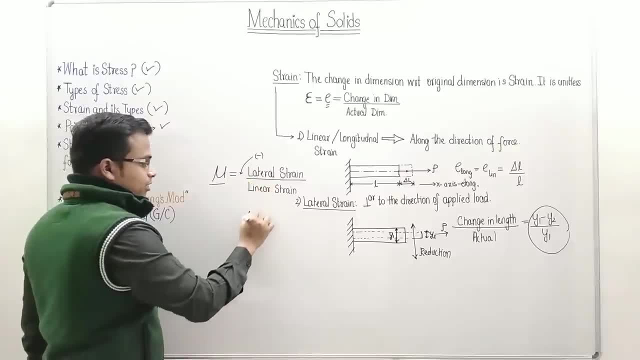 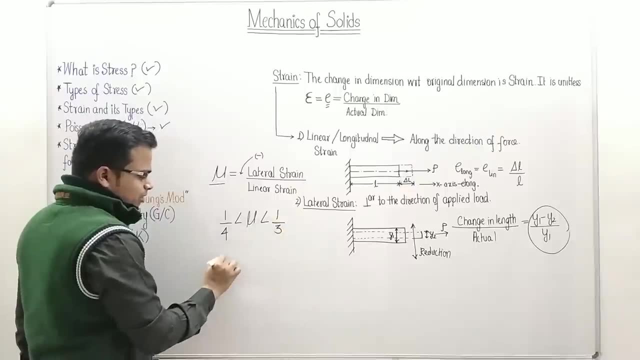 to that of linear strain And for engineering materials. you will realize this: that the value of Poisson's ratio lies between 1 by 4 to 1 by 3.. And, to be very precise, this is somewhere around 0.25, and this is 0.34 or 0.33, whatever right. So that was all about Poisson's ratio. 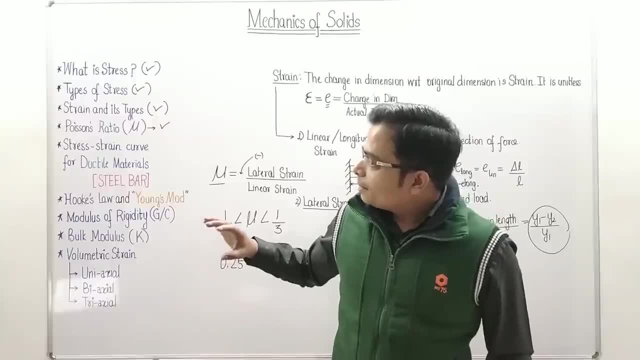 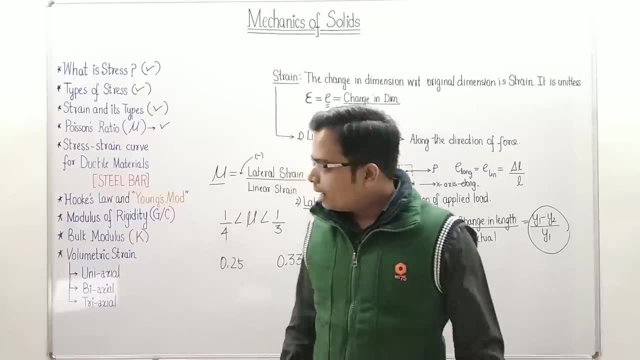 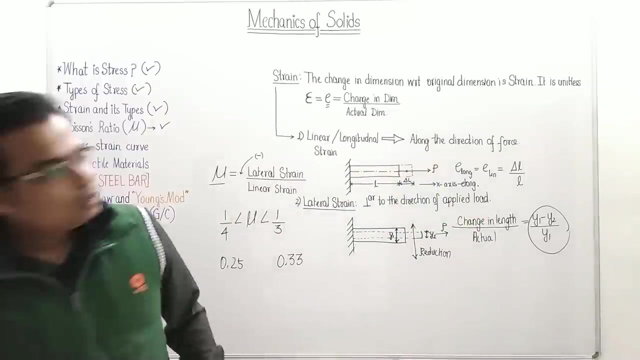 Now, this is the first video, and right now, let us focus upon this stress-strain curve for ductile materials. okay, So let us see how that works out, And here we will be considering a steel bar, And that steel bar will be, let us say, a medium carbon steel. Let me explain how this works out. 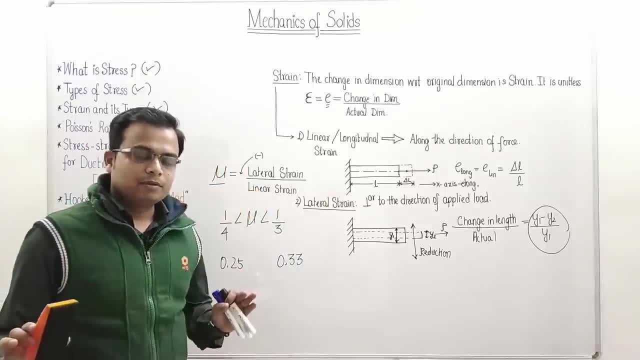 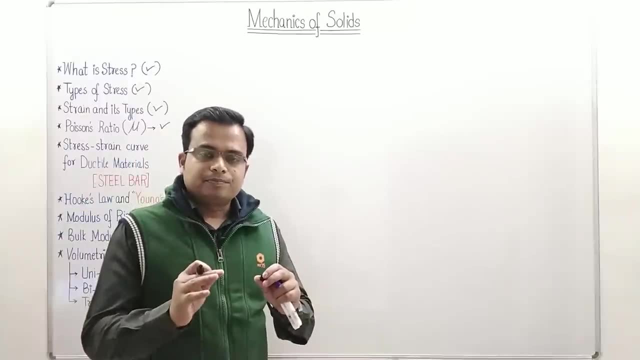 Let me just rub all of this Now. my suggestion to you would be: keep on pausing the video in between, so that you can note all of these things down right. Now let us start with understanding what exactly, or what is the information conveyed by a stress-strain diagram. 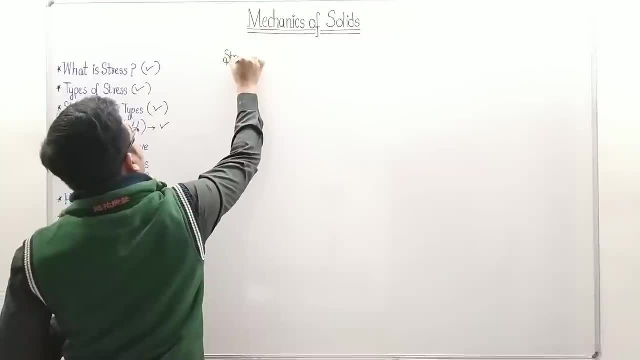 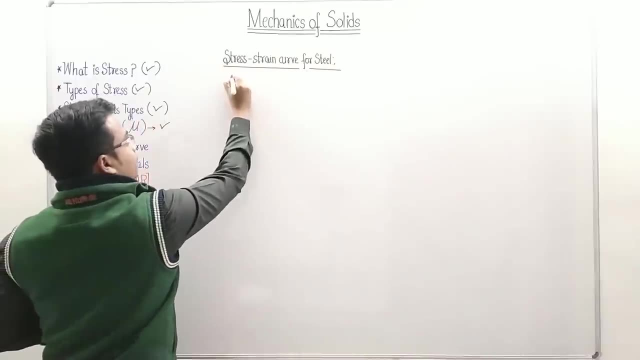 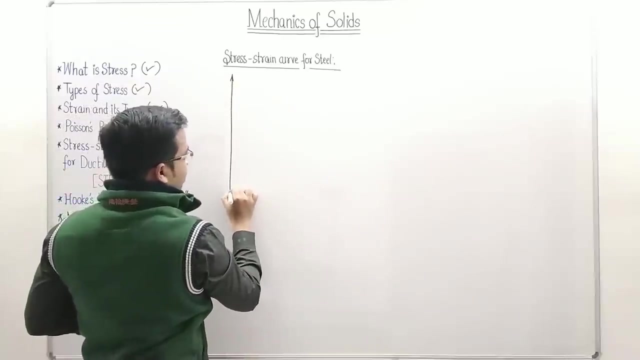 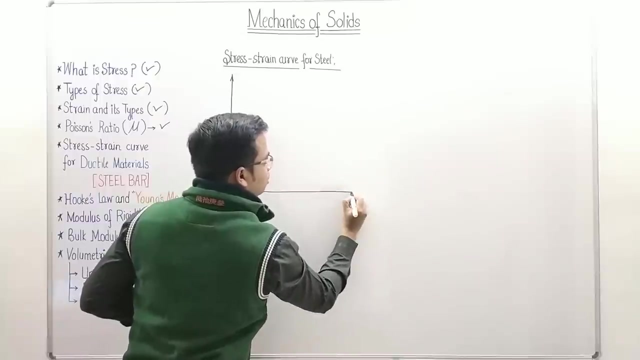 for steel. Let us see. Okay, As far as this curve is concerned, we are going to do this plot along and X Y axis. I think this much. Yeah, that is appropriate. So this over here. let me draw it further. 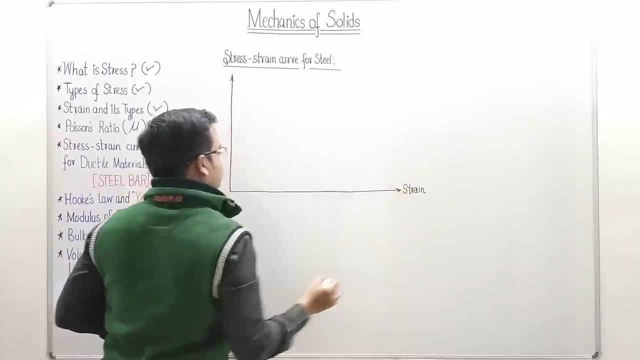 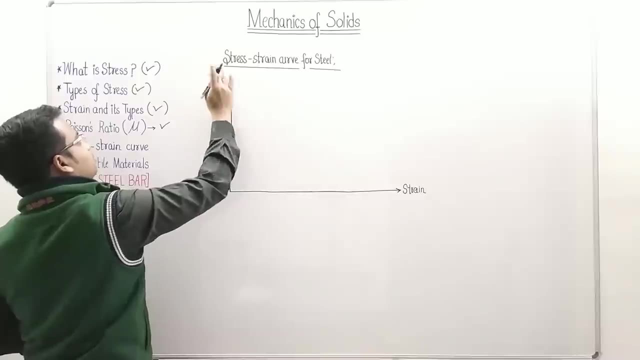 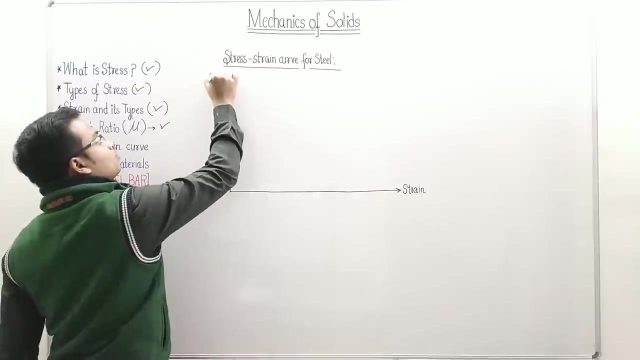 And this is for strain. And this Let me clothes, Let us take this as our movies, Lemme see here- first say: this represents stress along the y-axis. we have stress. we have stress along the y-axis and strain along the x-axis. 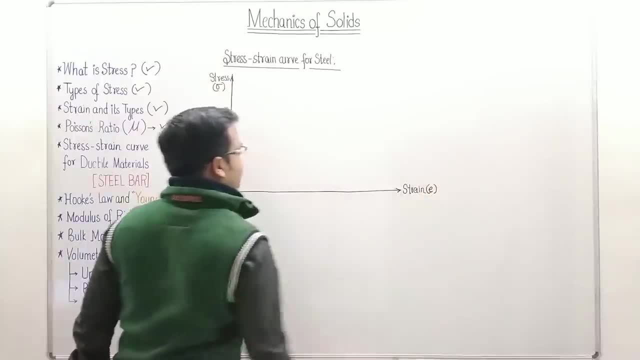 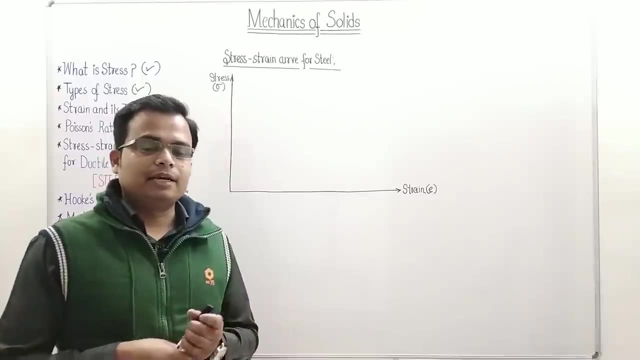 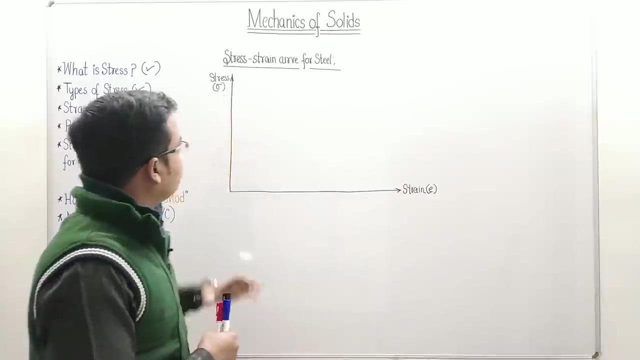 and strain. let's say we represent that by now. in order to understand this, first of all, we actually carry out an experiment. this experiment is basically done in a universal testing machine. okay, so this is basically known as a tension test, and basically what we do is we do a plot. 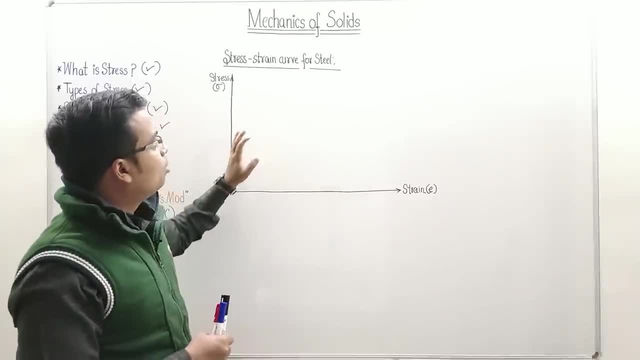 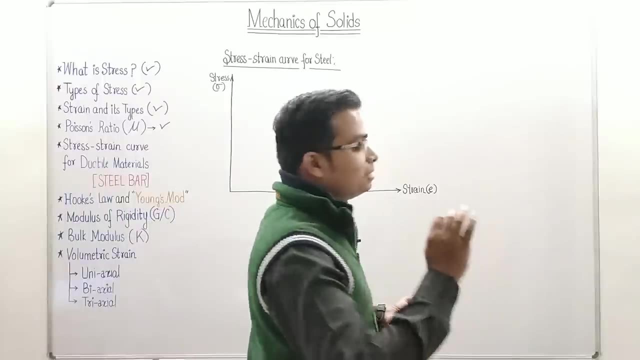 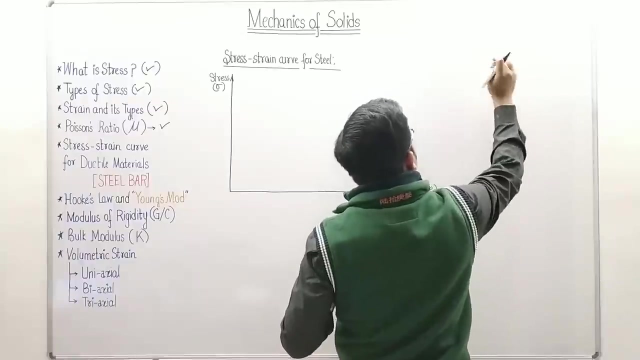 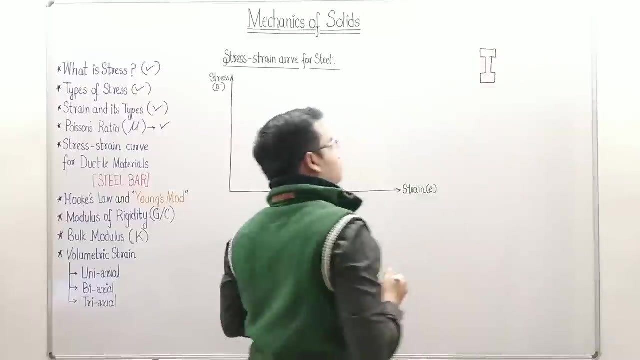 of stress with respect to strain. so this is going to give you a relationship or how stress is associated with strain. now, so, in order to understand this, first of all, let me just make the sample of the specimen that we take into the lab. here we go, right. 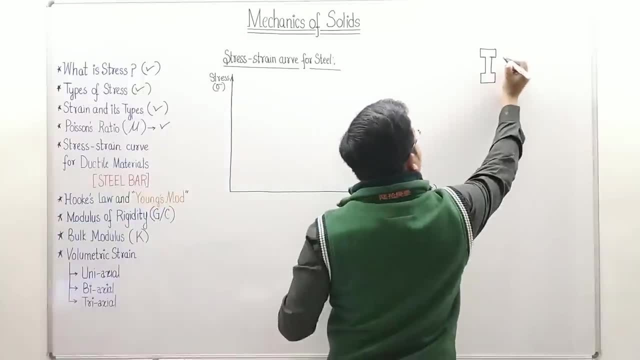 so the specimen is a test that we take into the lab. so the specimen is a test that we take into the lab. so the specimen looks something like this: now, what we do is we actually punch two dots over here, and the length between these two dots is what is. 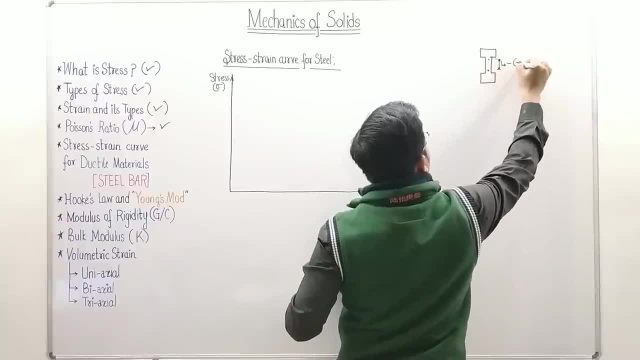 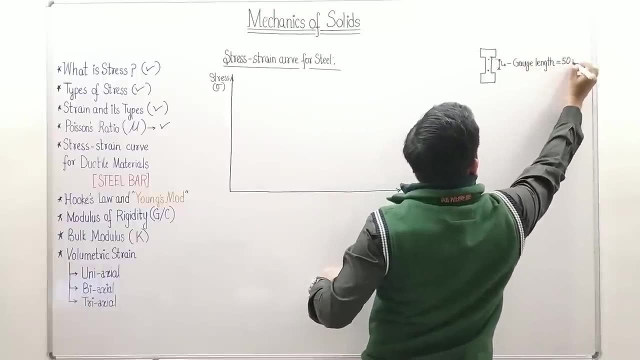 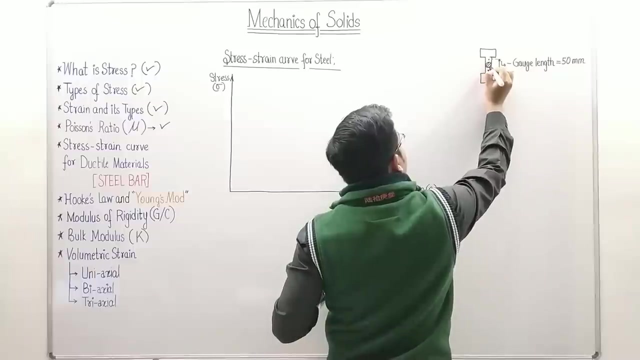 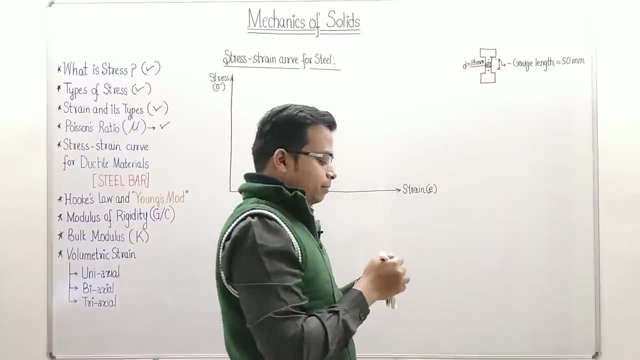 referred to as the gauge length. let me write it over here: gauge length, okay, and this is usually taken as 50 millimeters. now, if you watch carefully, the cross section over here is circular. this is going to have a diameter equal to 13 mm. this is very standard whenever you carry out. 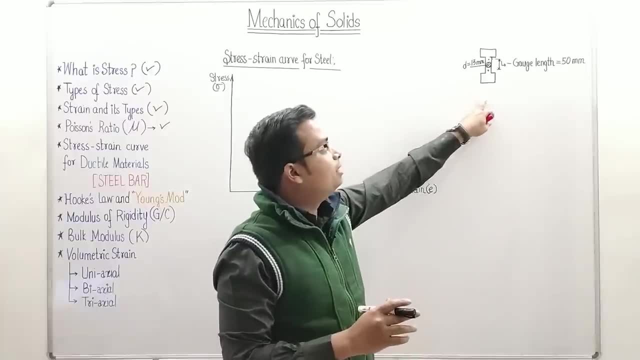 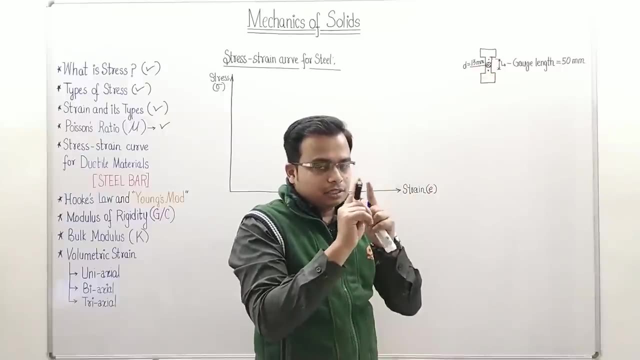 a tension test on a universal testing machine. these are the parameters that you have to work with. the gauge length has always need to be taken as 50 millimeters. you just make two dots and make sure the the distance between them is, or rather two dots are separated by a distance of 50 millimeters. at the same, 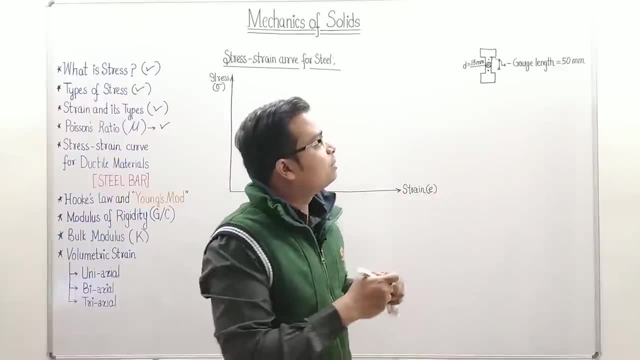 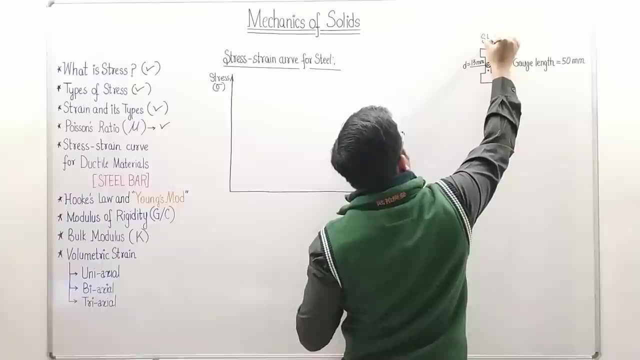 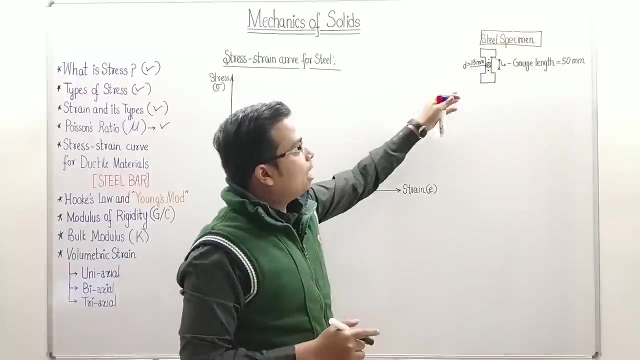 time this specimen over here, the steel specimen over here, is having a diameter this much. i'm talking about this much portion. okay, wide steel specimen: the diameter has to be taken as 13 millimeters. the eagle specimen: I'm going to be drawing this in a sort of timeline form. okay, What we usually do is: 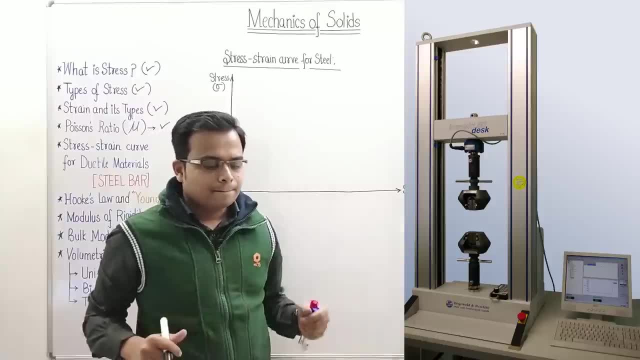 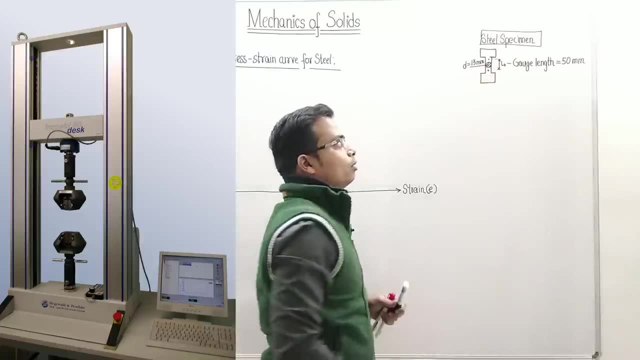 we have the universal testing machine here. you can see it in the figure over here and it has two jaws, an upper jaw and the lower jaw. The lower jaw is actually fixed. So this portion get fixed to the lower jaw and this portion get fixed to the upper jaw Now. 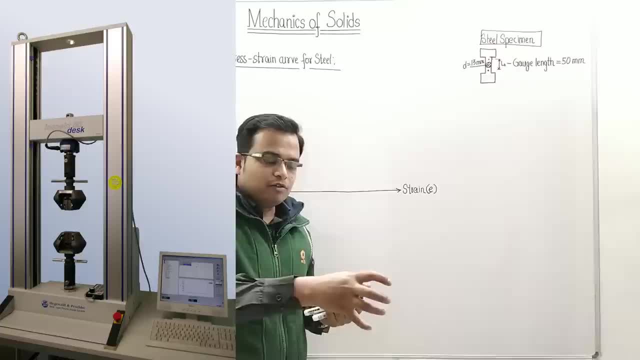 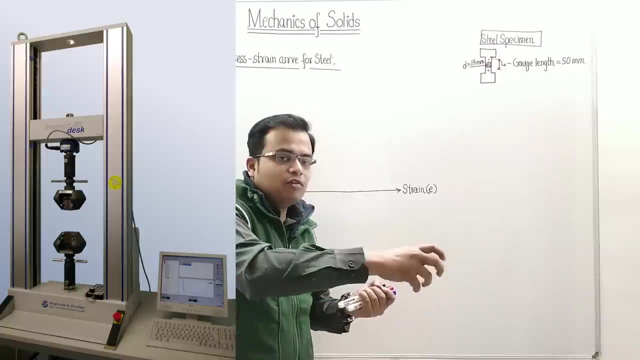 this is an entirely hydraulic machine, okay, So there are valves. if you try to open the valve, the load will increase. In a sense. what I'm trying to say is, when you try to open the valve of the universal testing machine, what will happen is the upper jaw, which is connected to the upper 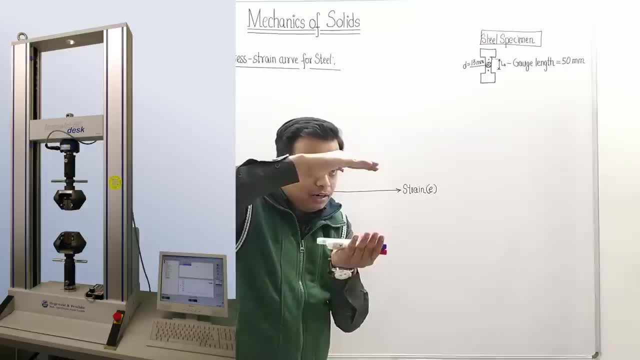 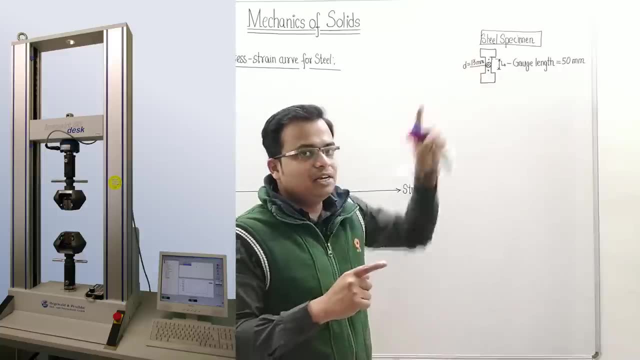 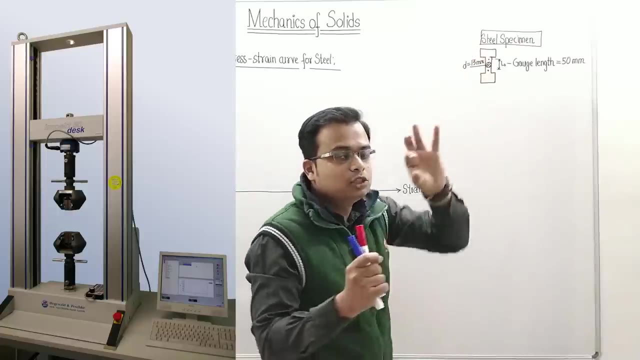 member of the testing machine. okay, or, upper end of the machine will try to gradually move upwards and in that process, since this portion is actually fixed rigidly to the upper jaw, the length over here, this effective length or the distance between these two punched dots, is going to gradually increase. okay, 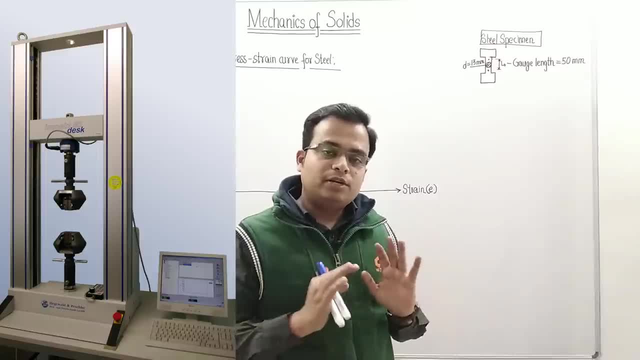 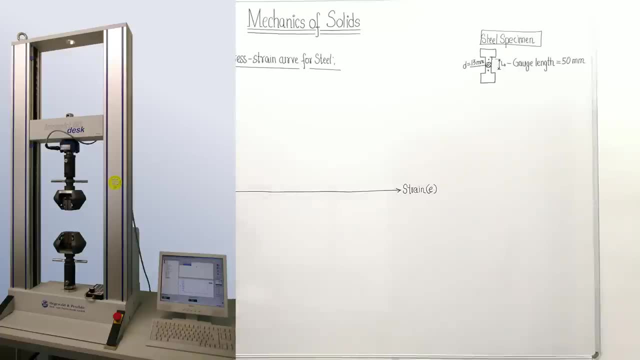 This experiment has to take place at a very slow pace. make sure that you do this at a very slow place. slow pace in order to get a very smooth stress strain curve, and the one which is shown in theory books. and this should actually be similar to that, okay, So what happens? So you've got. 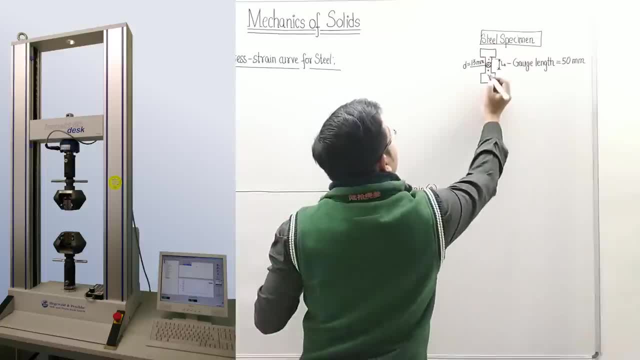 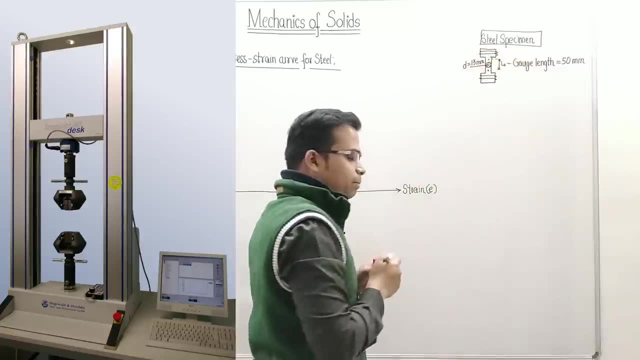 a steel specimen, okay, and this portion actually some kind of a some kind of threading has been done over this portion, okay, some kind of threading. a groove V groove sort of has been cut. some people do the threading, some people actually. 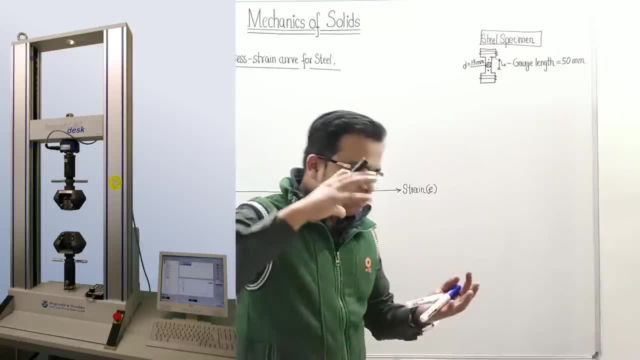 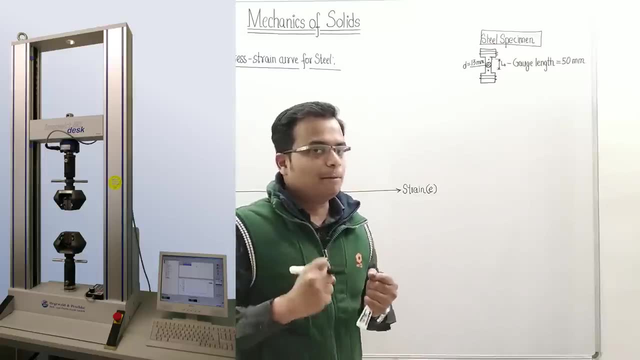 go for knurling operation also, okay. So in order to make sure that when it is fixed to the upper and lower jaw, the- what do you say? the bond is absolutely perfect, it's very rigid, it's very compact. right, there should not be any slip, okay, that is why knurling or threading is done over. 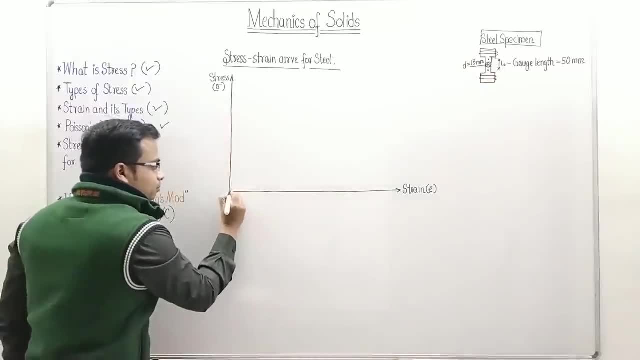 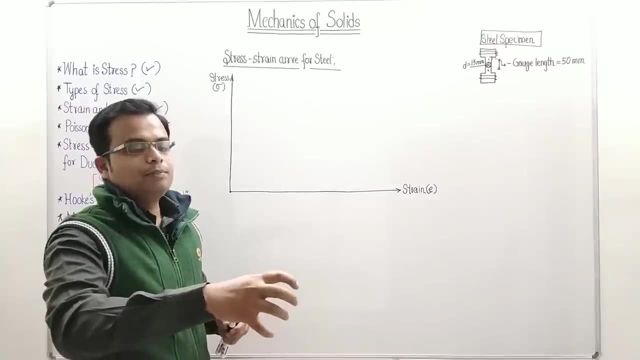 here Now. initially, there is absolutely no problem. there is absolutely no problem. there is absolutely no problem. you just have the specimen. fix it right. What will happen if you keep on increasing? you keep on opening the valve, and what will happen? The load keeps on increasing. 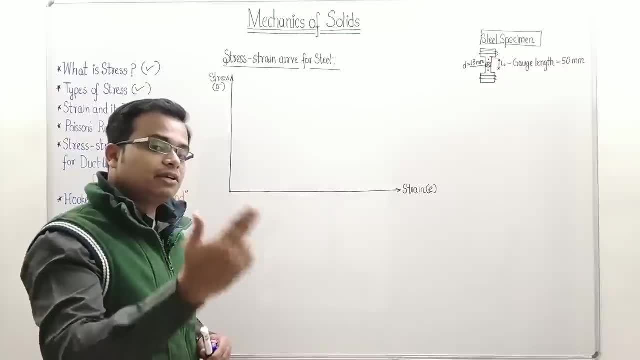 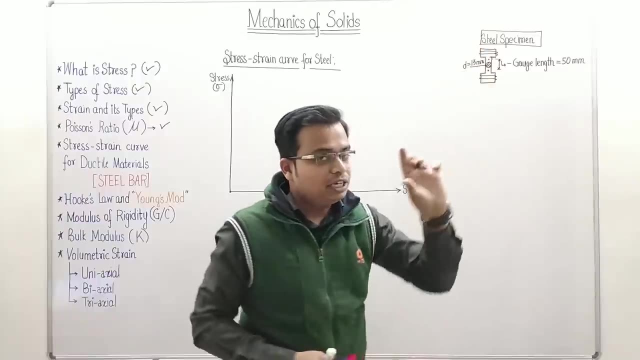 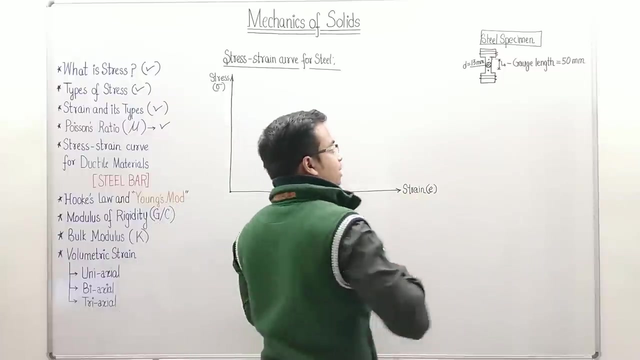 if there is going to be an increase in load, obviously there is going to be an increase in stress, and then there is going to be a change in this length also. that is also going to be changed. if there is a change in length, then you'll see some strain. right Now let me just try it over. 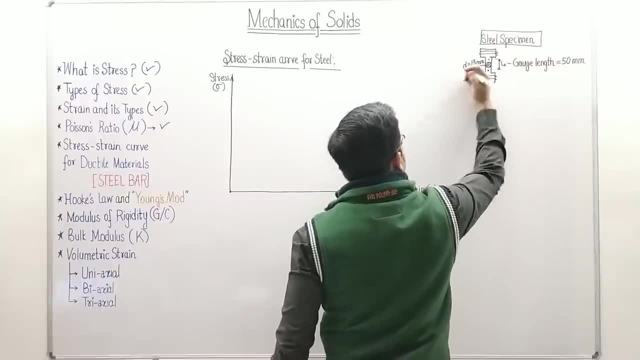 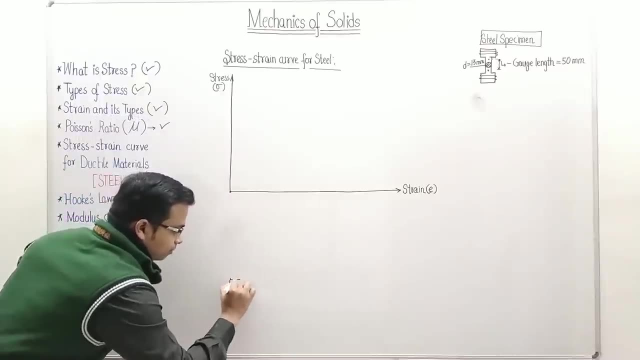 here. So what we are going to work out is the engineering stress. State of writing. here let me just write: the stress that we are going to talk about is the engineering stress, and the strain that I am talking about is the engineering strain. 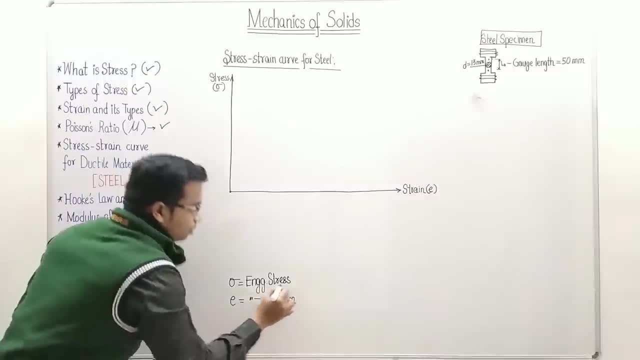 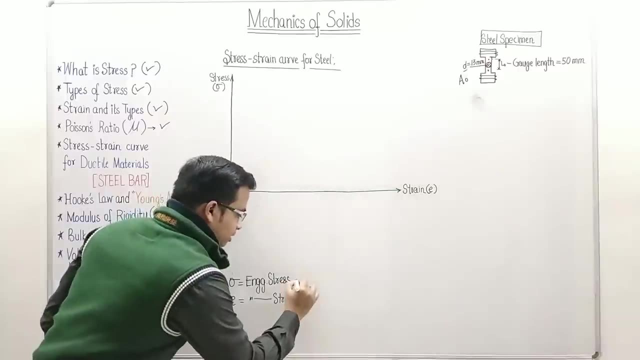 okay. Now this, corresponding to this diameter, you will have an area, let us say A naught, okay. So this engineering stress is equal to the load applied divided by the initial area, or the original area, and the strain. you can work it out very easily, that is. 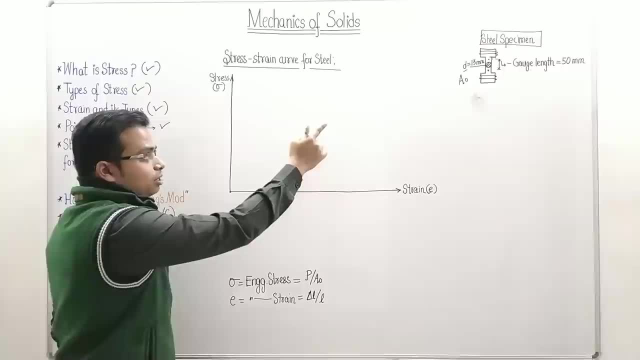 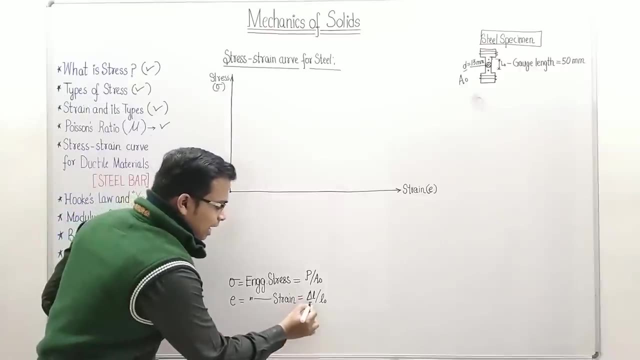 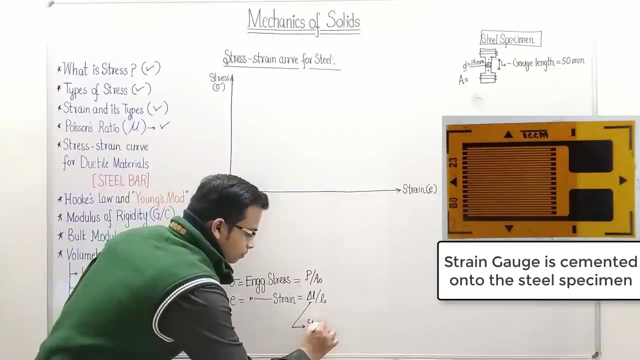 the change in length with respect to the original length. How much is the original length? That is, L naught, 13 millimeters. okay, Now, this change in length can actually be worked out with the help of two ways. One is with the help of a strain gauge. What you can do is you can fix a strain. 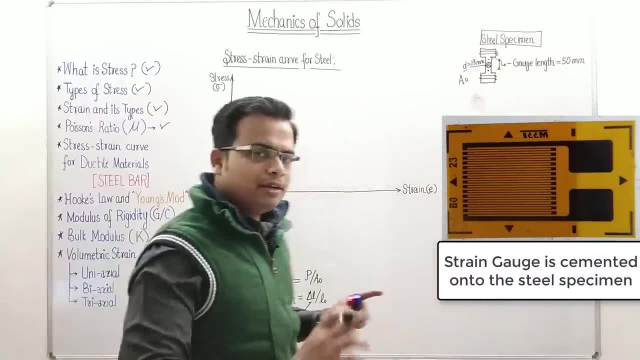 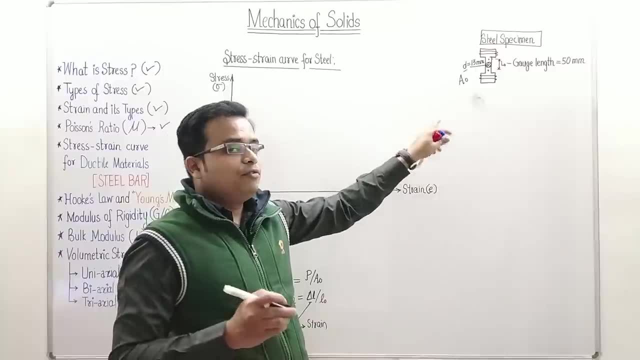 gauge over here and that some change in resistance will happen and you can actually work it out. Rather, in a lot of colleges you must have seen this equipment- universal testing machine- and if you haven't go ahead, go to the testing laboratory and try to do this experiment There. 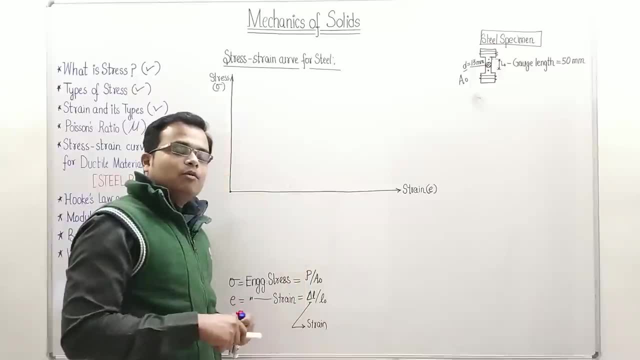 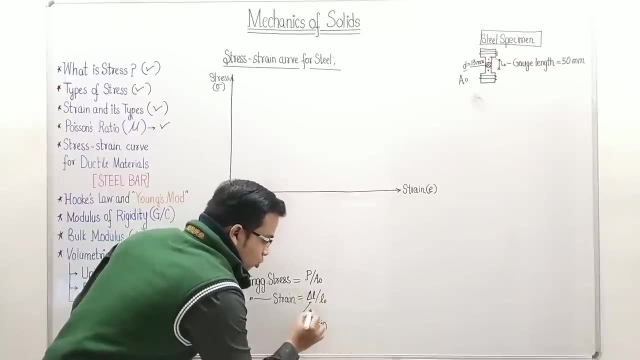 you are going to see that the upper arm of the universal testing machine will be fixed to the extensometer and extensometer directly gives you the value of this change in length. So this change in length can be measured with the help of a strain gauge. 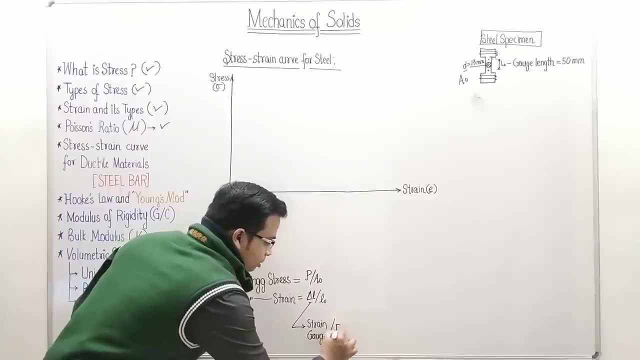 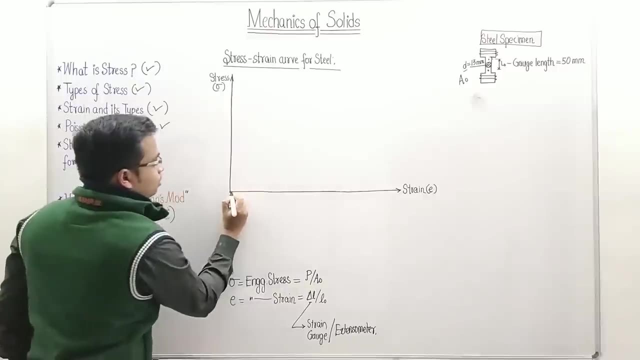 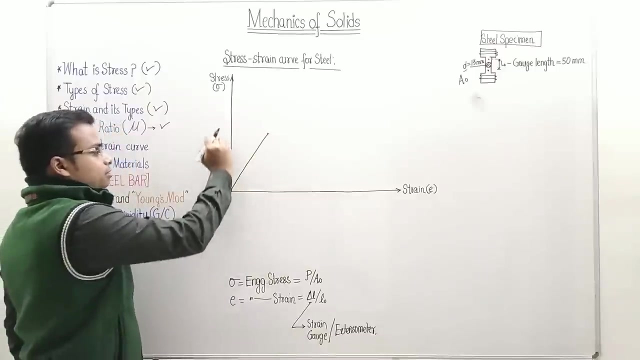 and it can also be measured with the help of an extensometer. Okay, so what really happens? You keep on increasing the load. What will happen? Something like this: Load increases, stress increases. this is going to remain same. this is going to remain same. 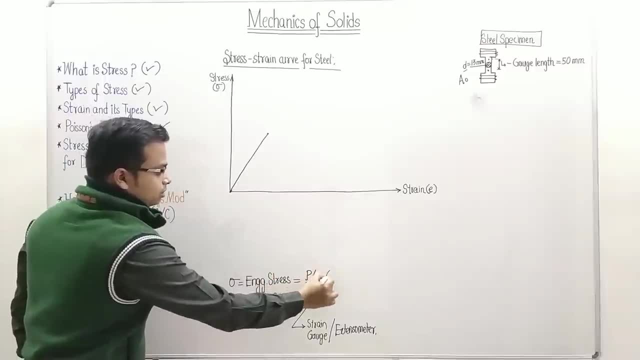 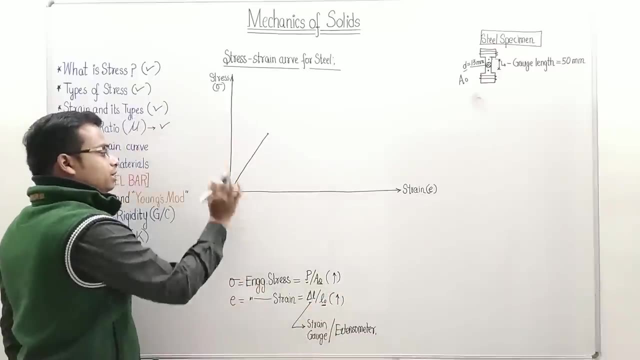 the load increases, so the value of stress also increases, isn't it? Change in length also increases, therefore the strain also increases, and the relationship is such that we actually make the change in length. So what will happen? We keep on increasing the load. So what will happen? 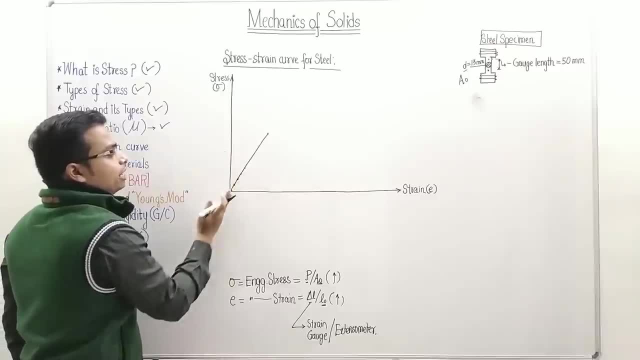 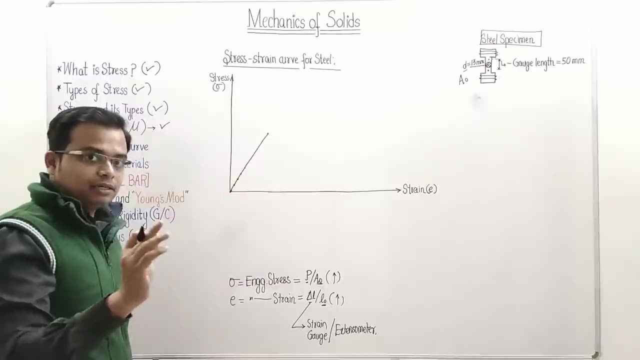 We keep on increasing the load. So what will happen? We continue to investigate with these points and always when you join all these points, you get a perfect line. that is why the relationship of stress versus strain is absolutely linear. But until you reach this point, okay. 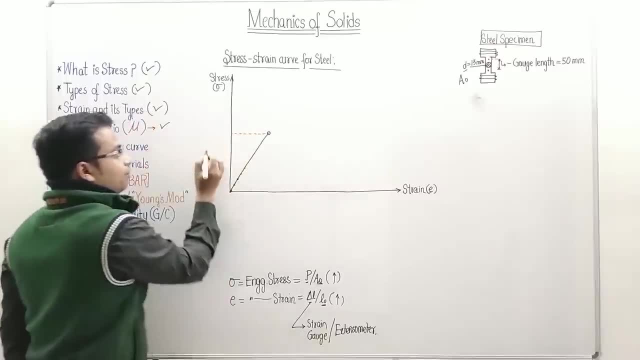 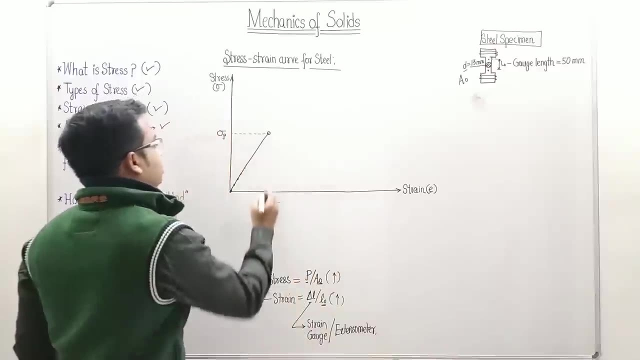 and this point is the proportional limit. sigma p: right. So this is the first point at where we will talk about point number one. point number one is the proportional limit. Let me just write it over here. Hold on, hold, on, hold on. So we will talk about point number one. 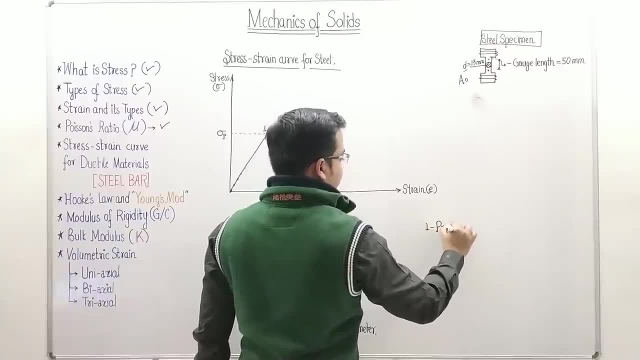 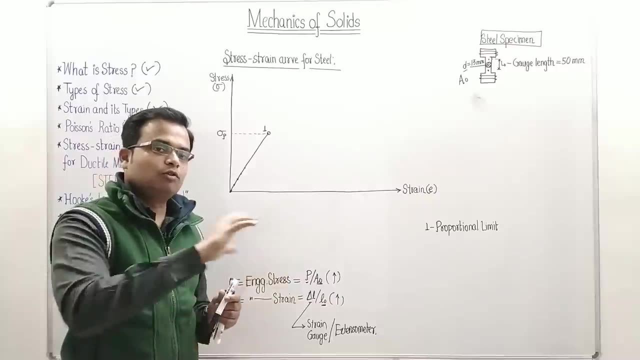 So this is the first point that we are going to talk about, point number one. point number one is the proportional limit. Let me just it over here. Point number one corresponds to the proportional limit. Now the idea is such: if you remove the load, if you close the valve, okay, what will happen? The specimen will regain. 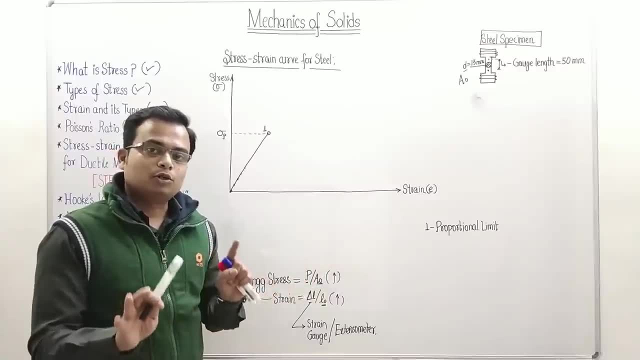 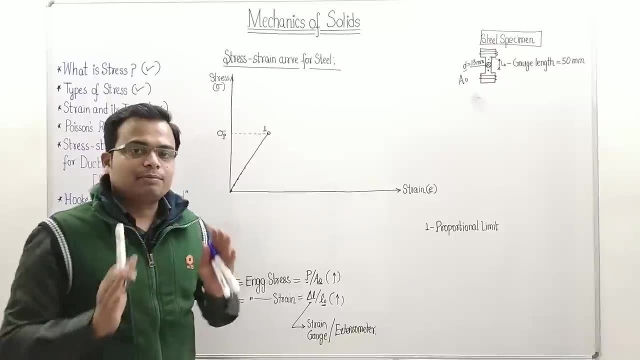 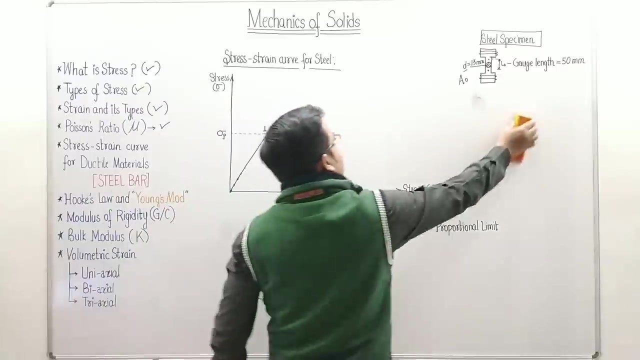 its original shape and size. No problem whatsoever. It is going to exhibit an absolutely elastic behavior. That means it is going to regain its original shape and size, even though you have released all the load that you initially had applied. Okay, what happens if you go further? 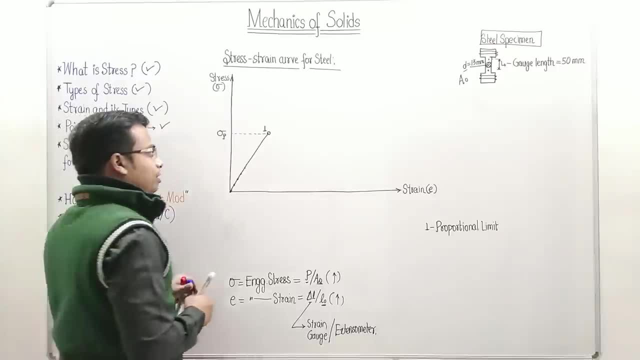 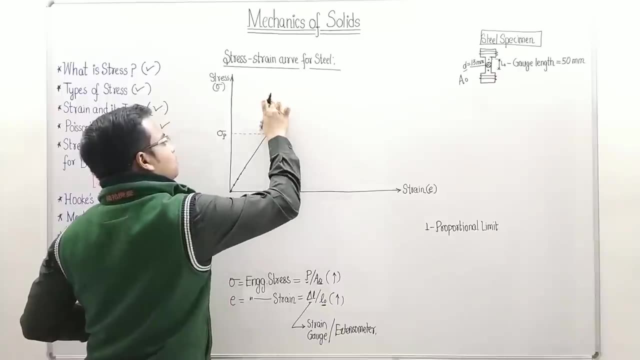 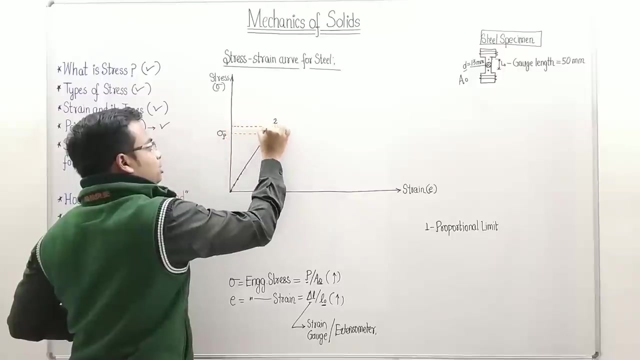 Let us see. Let us see When you go further, what will happen is, after a certain point in time you will get one more point. Okay, this point was one. this point is point two. This over here corresponds to the elastic limit E. 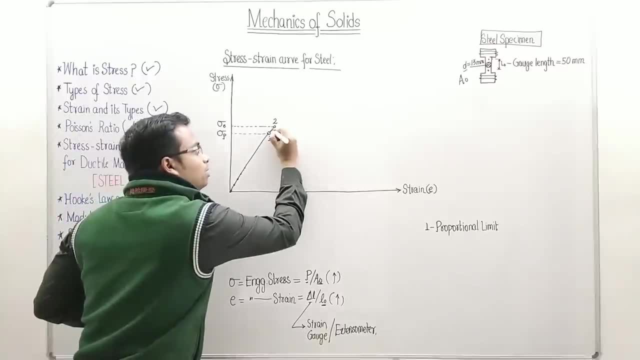 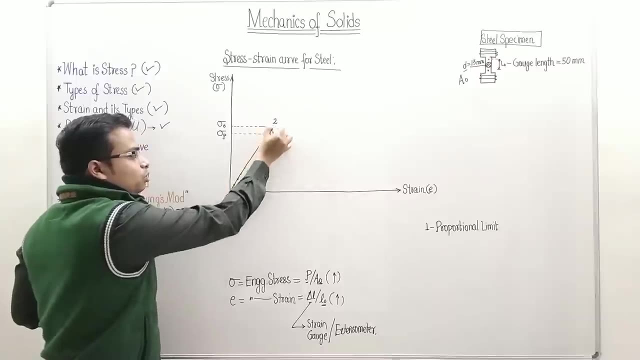 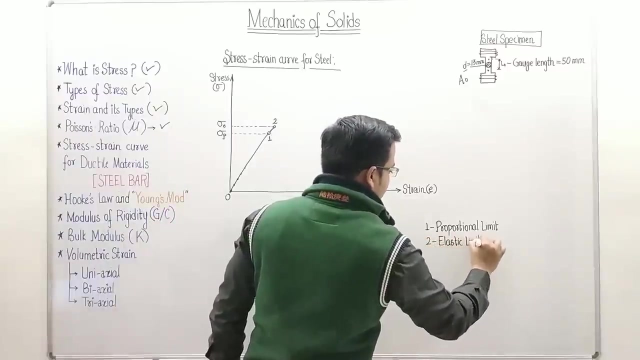 Again the idea is from one to two. there is a very small curve. from one to two, From zero to one, you see an absolute line. from one to two it is a curve. So point two corresponds to the elastic limit. Now the idea is very much mathematical Here. from zero to one, you see a line. that means 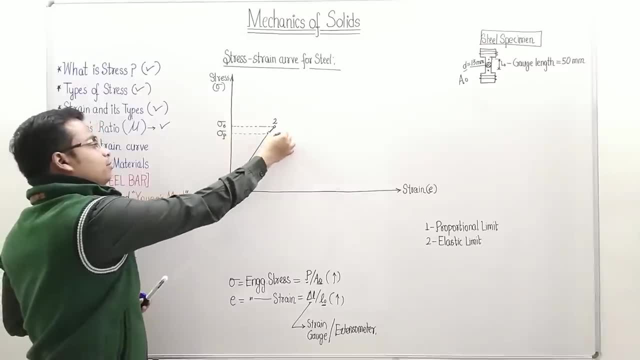 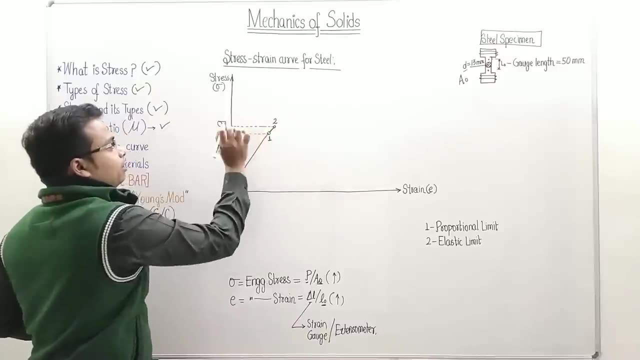 a proportional limit. These two are absolutely proportional And since between one and two we see a curve, they are no longer proportional. Okay, so there is a curve over here until you reach here. Okay, as far as this elastic limit is. 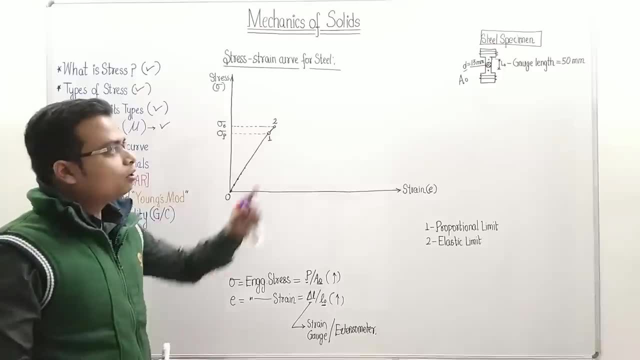 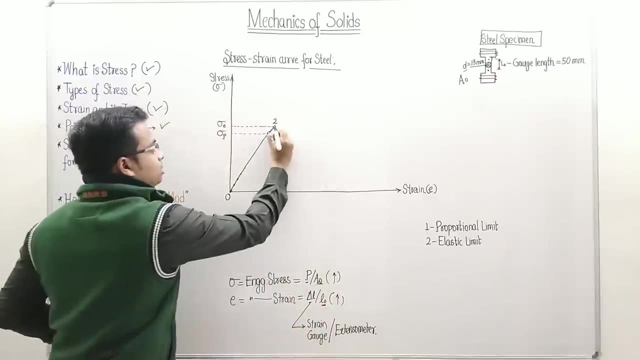 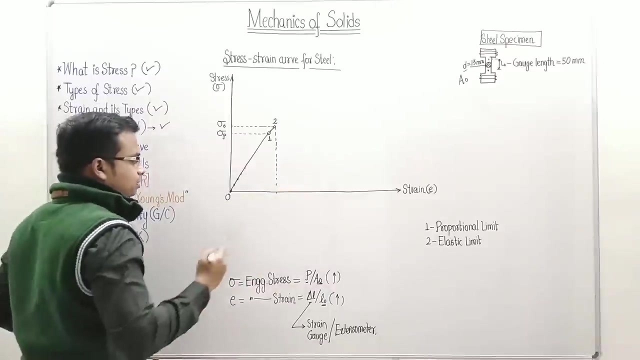 concerned. even if you remove the load, the material is going to, or the specimen is going to, regain its original shape and size. That's for sure What happens if you go further. Now let me just specify this: Between this region, the material exhibits elastic behavior. 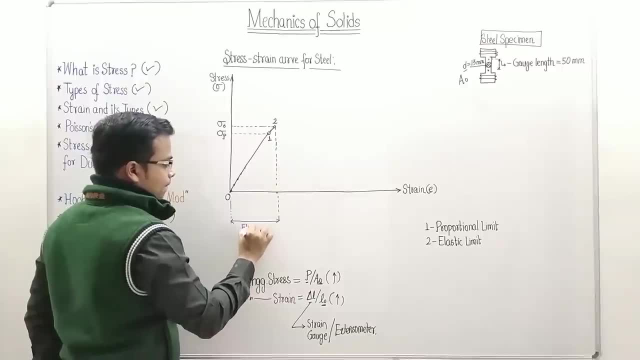 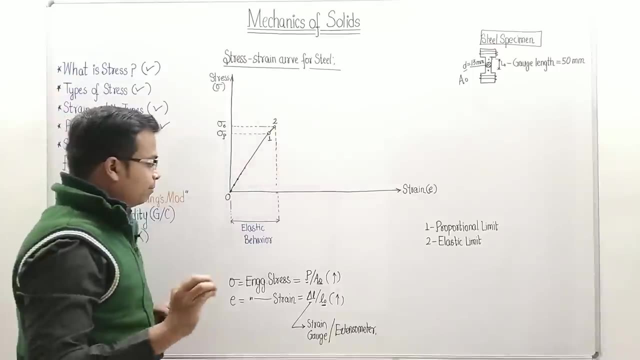 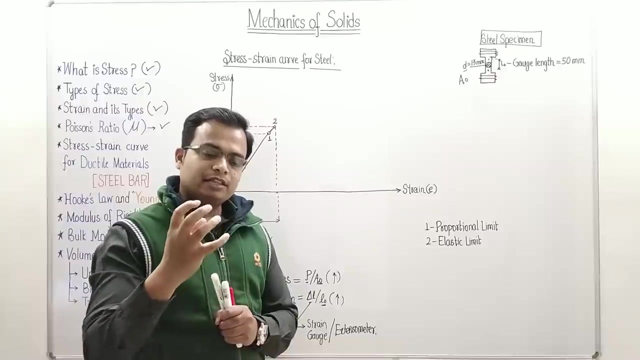 In this region. the material exhibits elastic behavior, Okay, and once you go beyond point two, then the material is going to exhibit plastic behavior. By plastic behavior I mean to say that even on releasing the load- okay, even on getting the load back to zero Newtons- the material or the specimen will no longer be able to. 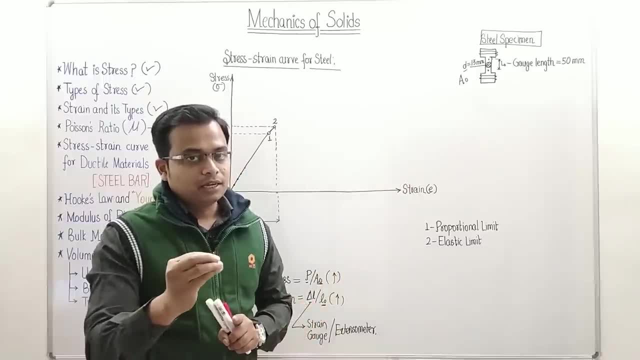 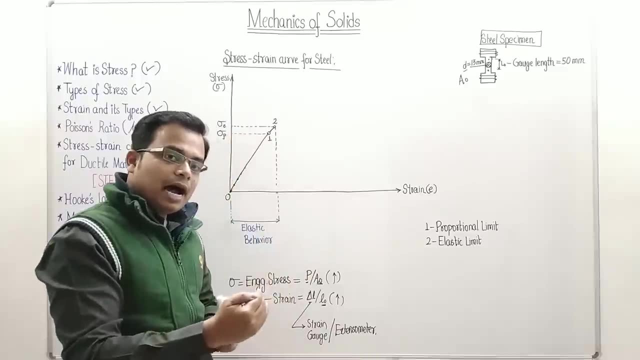 regain its original shape and size. Remember what is plastic. If, on releasing the load, the material does not regain its original shape and size, then it has entered the plastic region. Now if, on releasing the load, getting the load back to zero, it regained its original, 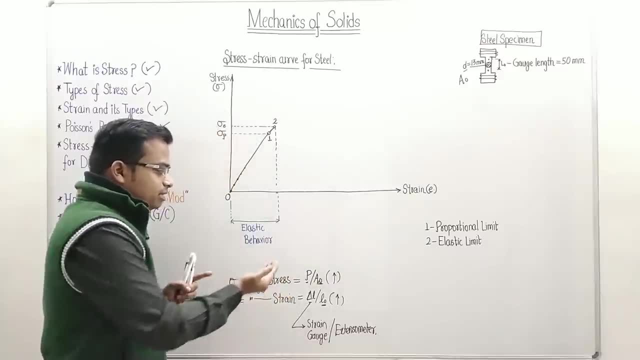 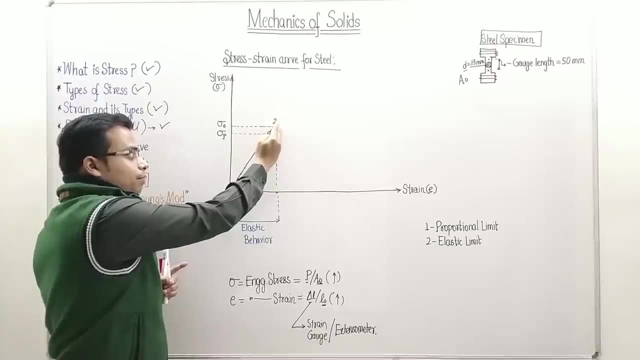 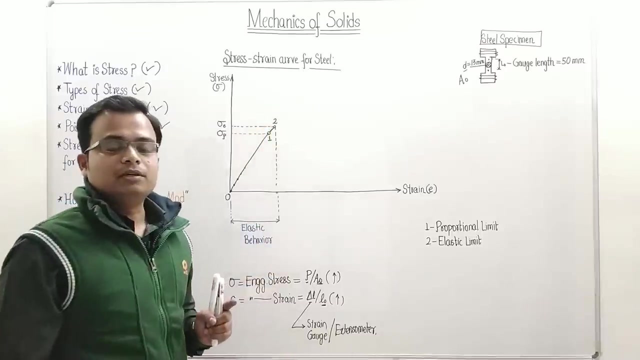 shape and size, then the sort of behavior that the material is exhibiting is the elastic behavior. So this is the saturation point. If you are below this point, then the material is going to remain elastic. if you go beyond point two, well, obviously. well, you are working. 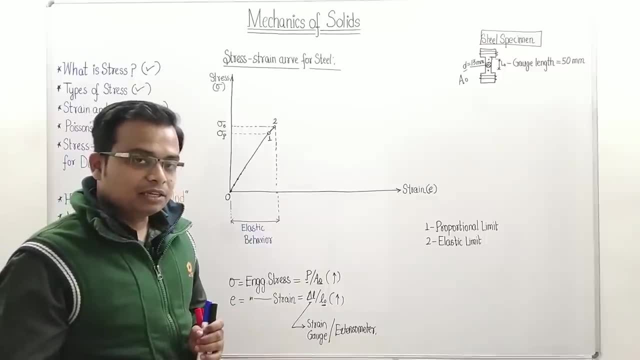 with danger, and that means the material will enter the plastic region, And from where? Well, you cannot digitalize the material and interpret the plastic incident more sympathistically. Well, that is bound to happen when you have a set of products, If you have a set of products, 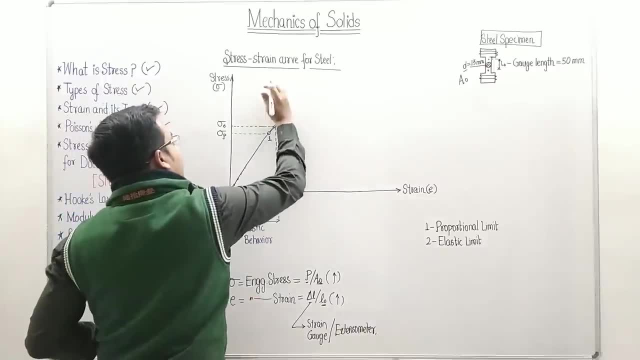 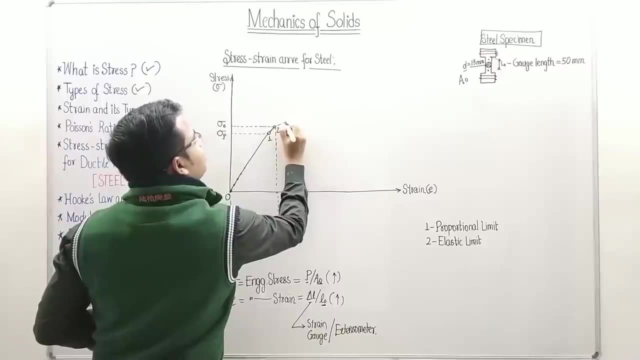 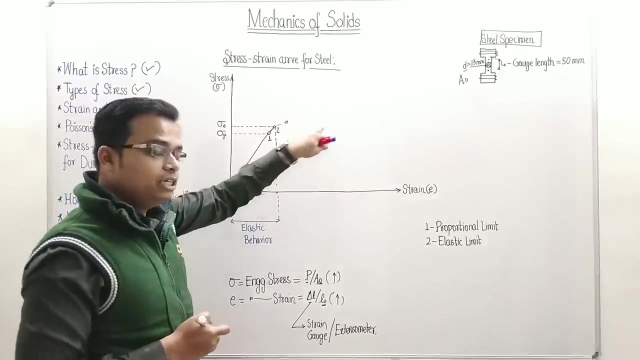 you cannot regain its original shape and size. Okay, Let's see what happens next. Right, Then it's like this: Very, very less difference, In fact, when we used to do experiments when I was in college, I did this experiment when I was a teacher, I mean three to four years back. 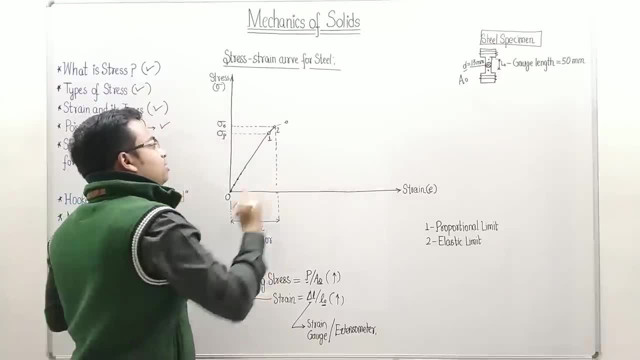 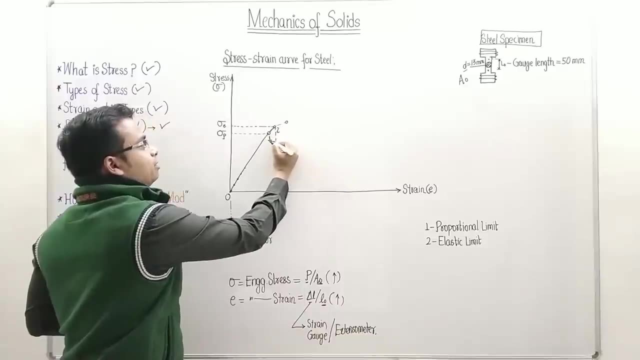 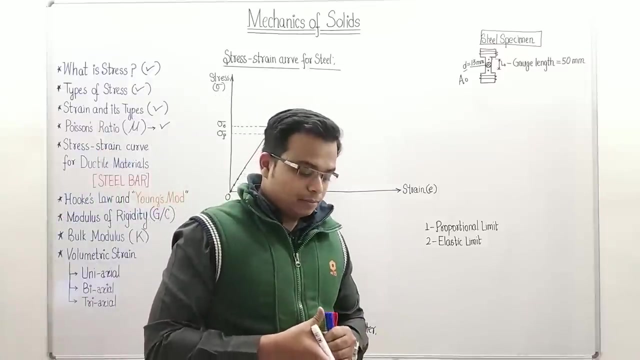 I did this experiment. I have never seen these two points apart. I've always seen that there is absolutely no gap between the elastic limit and the proportional limit. So I would encourage you guys to do the same experiment in a laboratory, in the material testing lab. This is basically a. 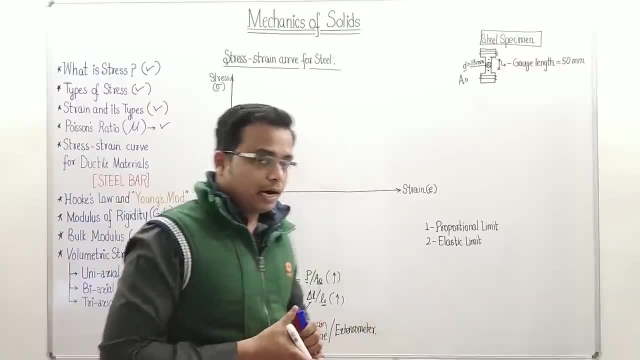 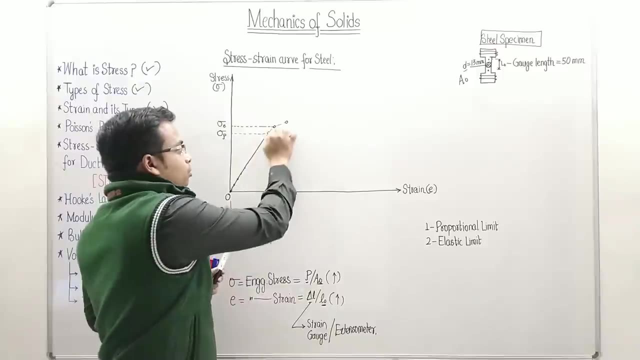 common course for all mechanical as well as civil engineers. Do this and do let me know in the comment section down below if you get these two points separated by a certain distance, or do you get these two points at the coinciding with each other. Okay, Now if we go beyond this, 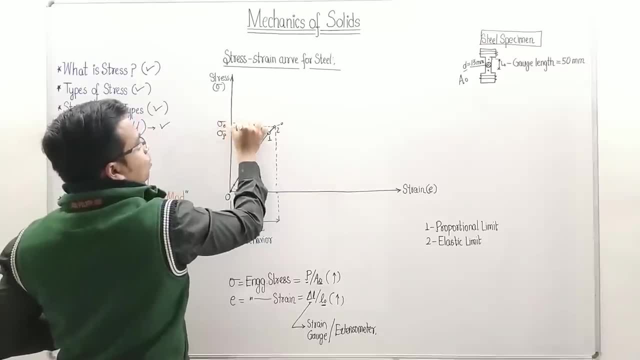 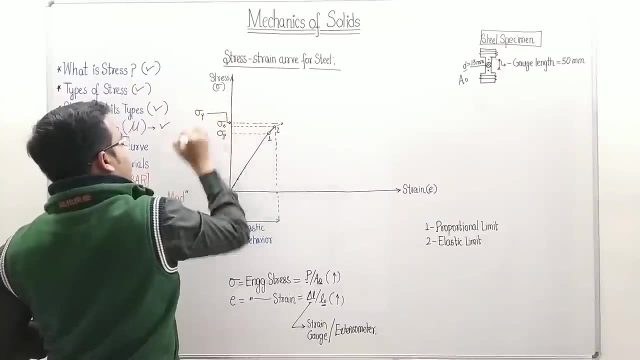 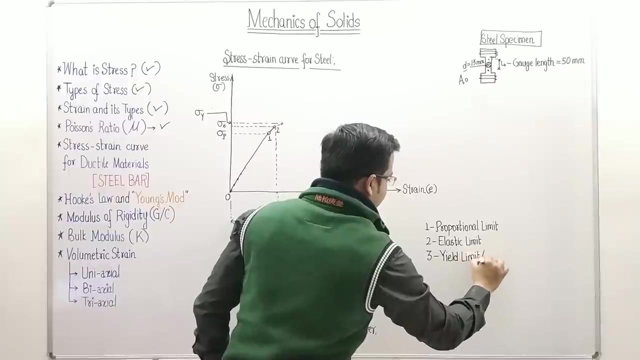 we get one more point And this over here, let me tell you, let me tell you this: over here is the yield point, sigma y, Point 3 is yield point, Yield limit or yield point, whatever you may call it. 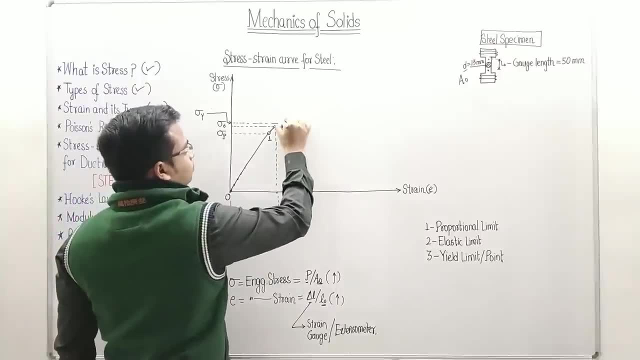 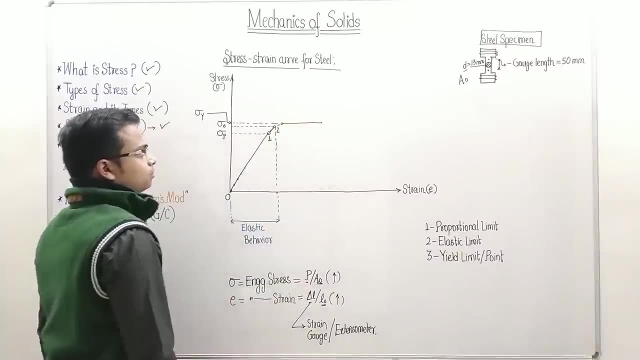 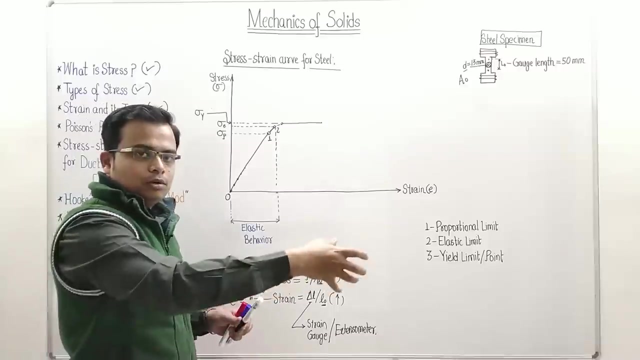 Okay, Now what happens after this? Something very strange happens. You see this: There is absolutely no increase in stress. That means there is absolutely no increase in the amount of load. Okay, So, from here to here, you are actually opening the valve. When you open the valve, 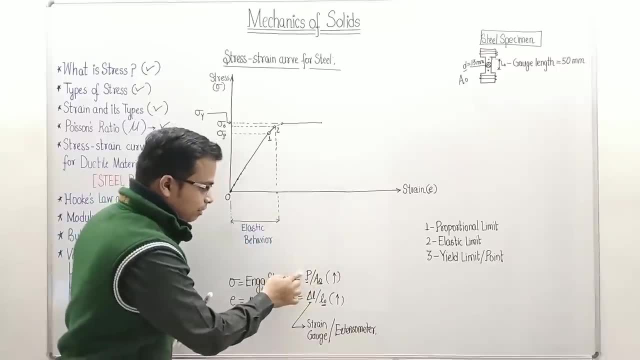 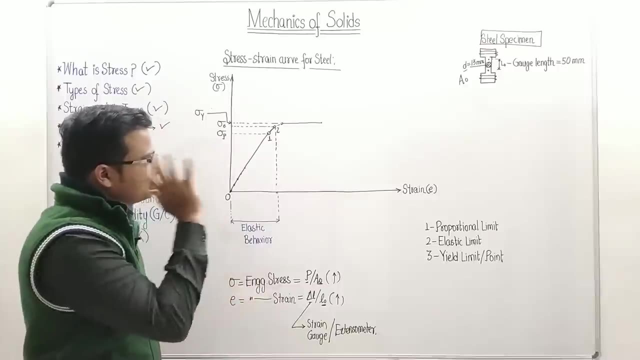 gradually. what happens? The load increases. If the load increases, that means this engineering stress is going to increase, Fine, And correspondingly the strain is also going to increase. But here something actually weird is happening. We are no longer opening the valve further. 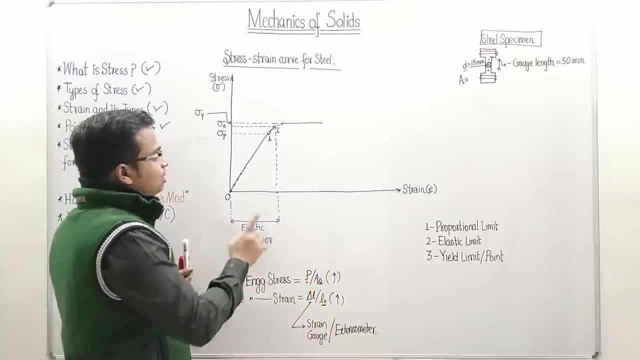 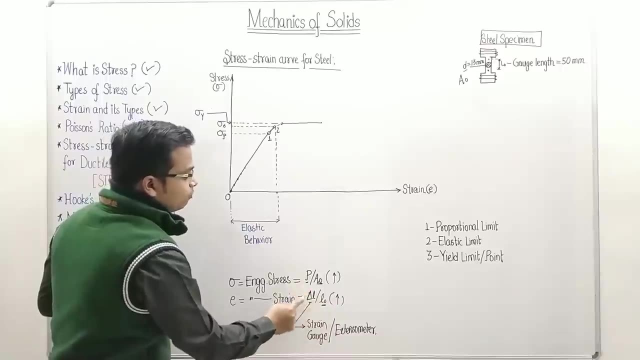 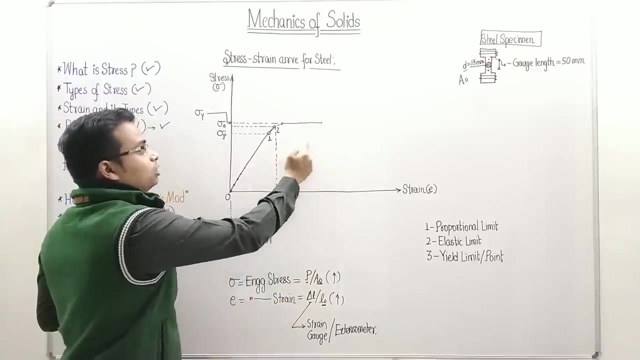 What we do is we remain stationary, but still, you can see, there is an appreciable increase in the change of length. There is an appreciable increase in the change of length, because of which, when you put this into a formula, okay, at different time spans, the value of strain that you are going to get will gradually increase. 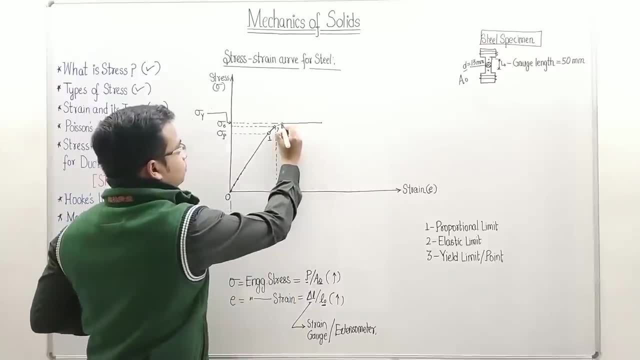 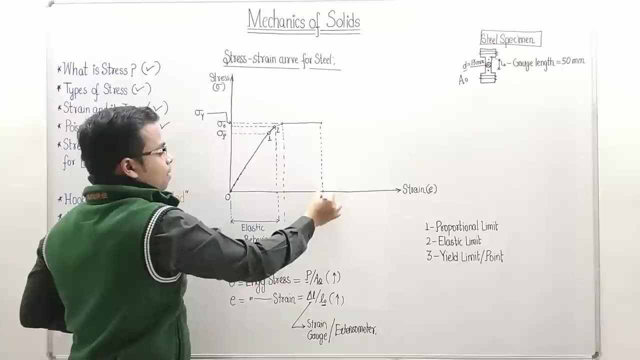 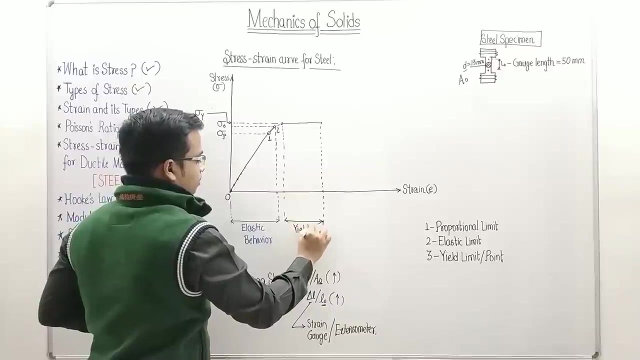 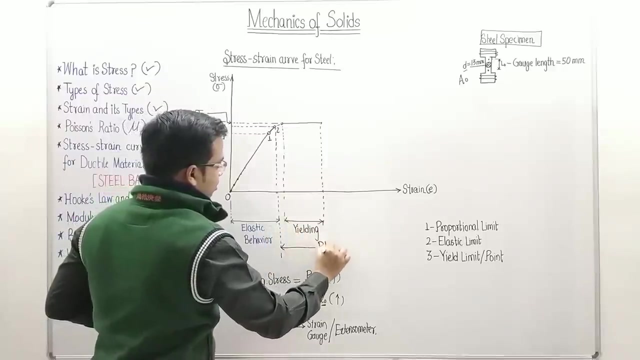 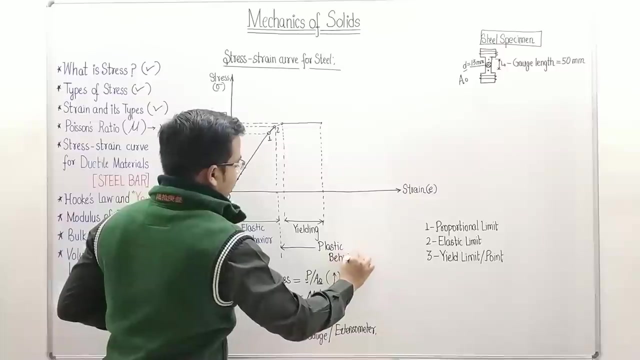 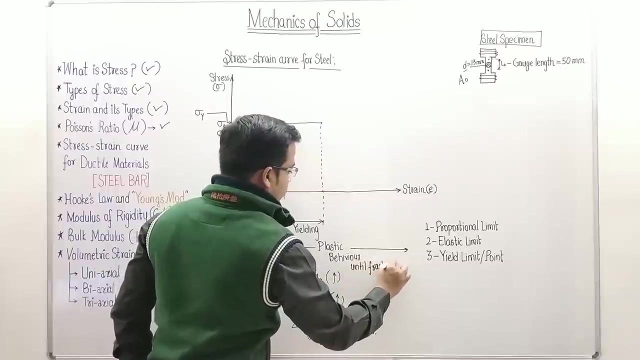 and this process, guys, this process from here until you reach here- this is what is referred to as yielding, Yielding and basically remember this. after you reach here, there is continuously plastic behavior until the mild, until the steel specimen fractures, until plastic behavior until fracture. Now this is going to be very important. try to learn this. here. elastic, here yielding happens. 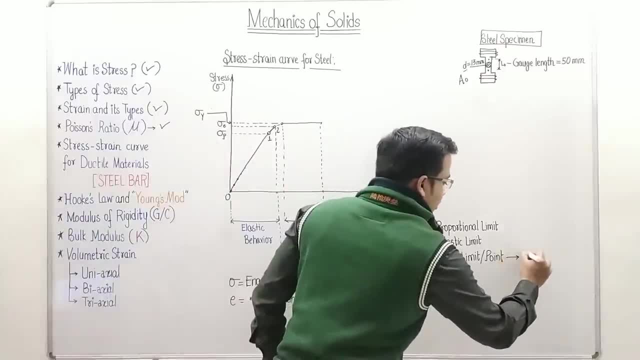 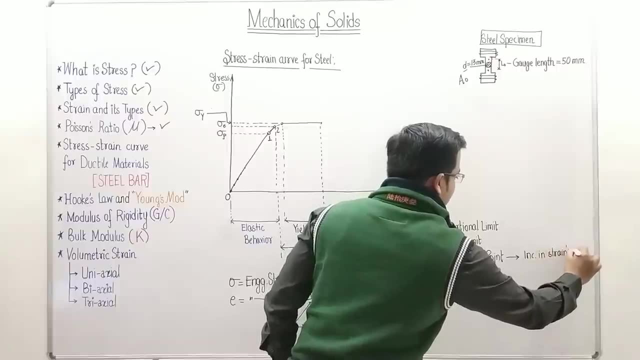 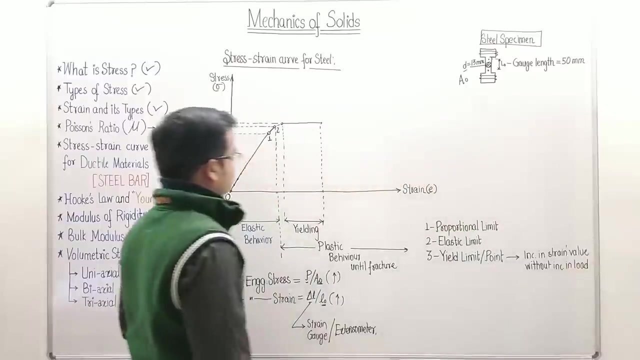 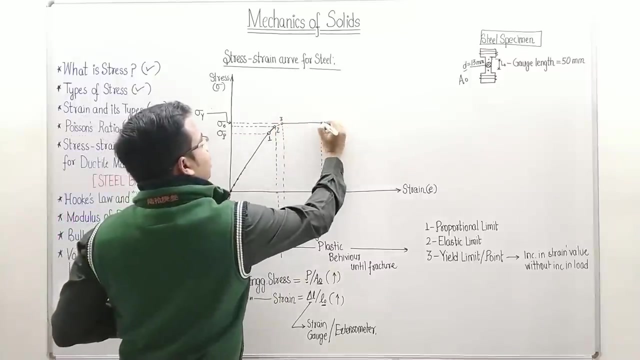 what do you mean by yielding? Yielding Increase in strain, increase in strain. just remember this point: there is an increase in strains value without increase in load. okay, so that was yielding for you. okay, now this is point number three. again point number four. this is going to get very interesting now. some of you 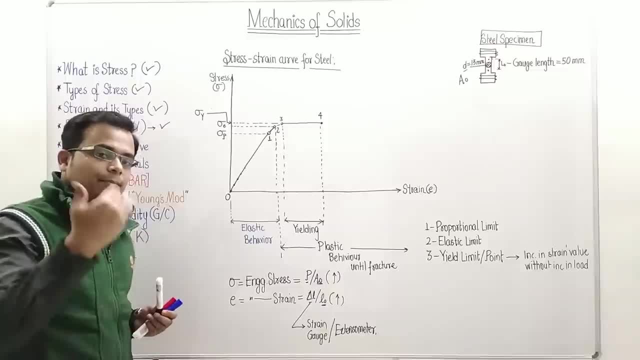 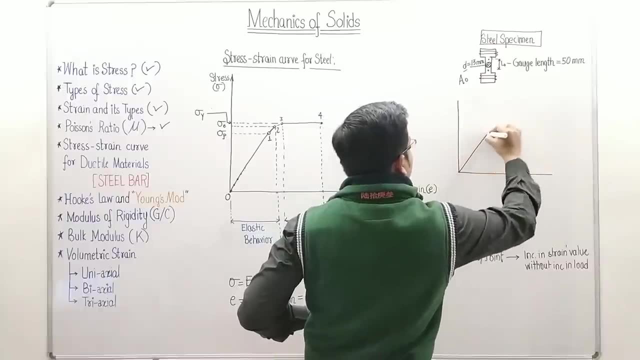 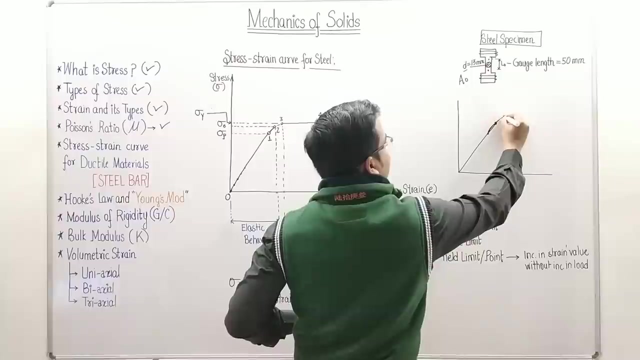 might be wondering that they must have heard about two yield points, an upper yield point and a lower yield point. let me just draw one more stress strain curve over here. proportional limit, sort of slightly curve elastic limit yield point. yield point: this is upper yield point and there is a lower yield point, yielding fracture. and 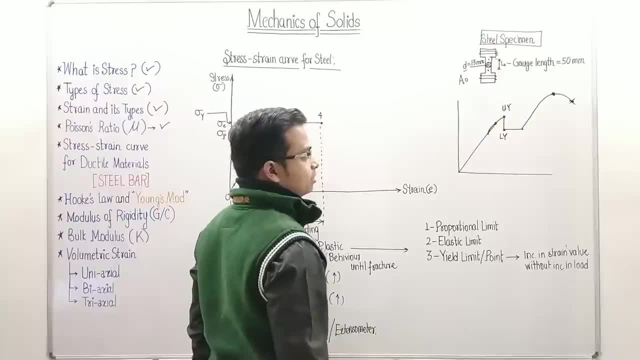 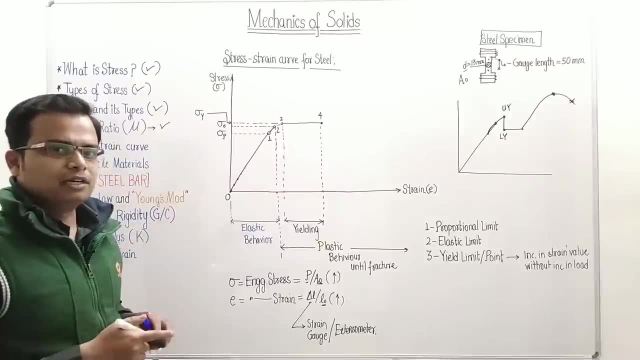 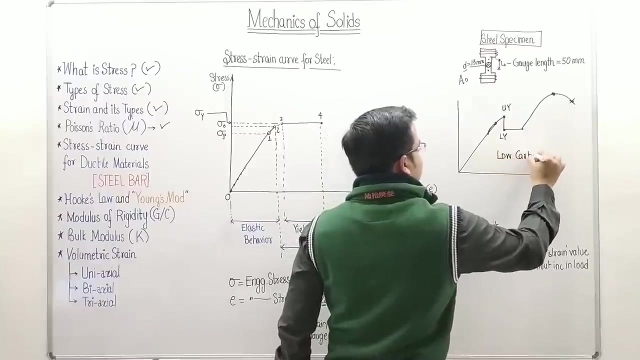 this is the maximum stress. okay, or the ultimate stress Now in this experiment has been done on a steel bar. okay, of a medium carbon steel. if you do this experiment, let's say for a low carbon steel, for a low carbon steel. by low carbon steel I mean to say: 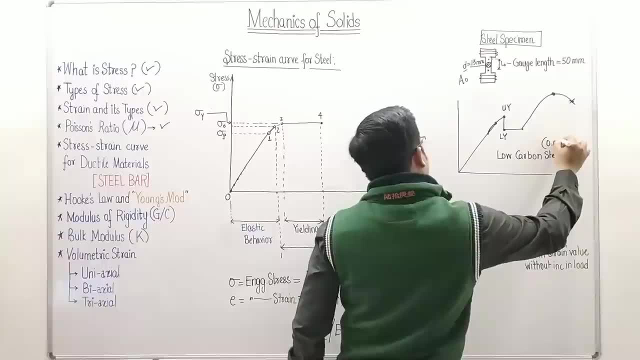 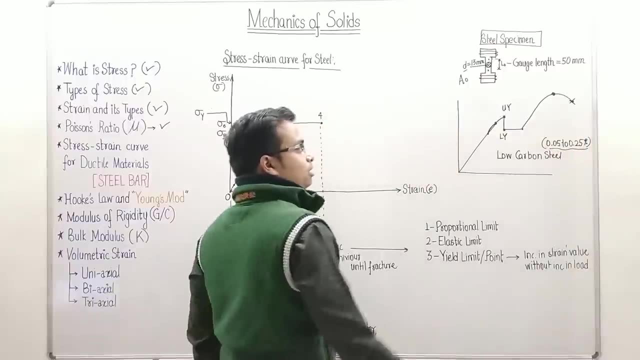 that the carbon content is going to be somewhere around 0.05 to 0.25 percent. if the carbon content in the steel is somewhere around this region, then obviously you are going to get two yield points. okay, there is going to be a sudden drop. this is the upper yield point, and then there is the lower yield. 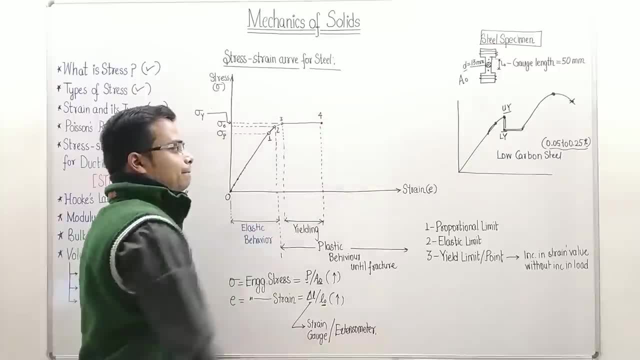 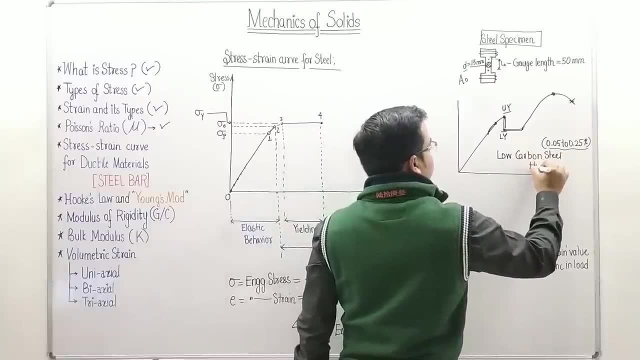 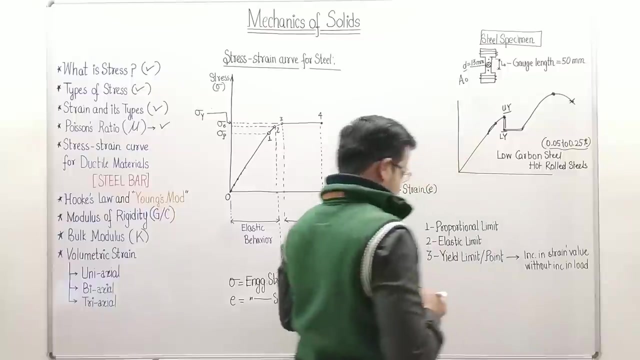 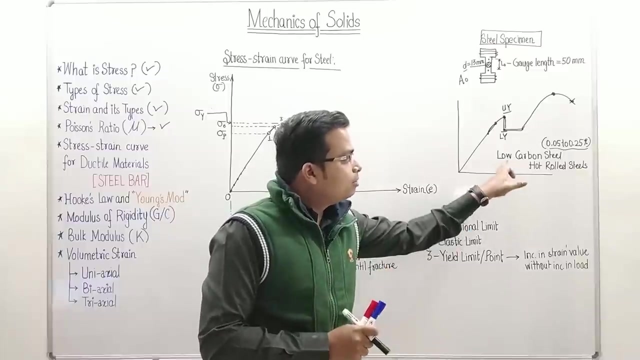 point and then the remaining stuff is same. you'll see this happening right in case of low carbon steel and also rolled hot rolled steels. so question might be asked you: in which of the following options do you get the upper and lower yield point, and maybe this will be an option or this will be an? option: Hot rolled steels or low carbon steel. so now you know the answer. okay, for low carbon steels and hot rolled steels. whenever you do the tension testing on that specimen, you will always get two yield points. one is going to be the upper yield point, one is going to be the lower yield point. and this is the process. 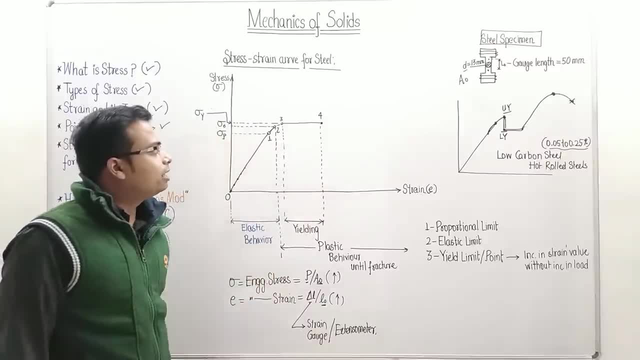 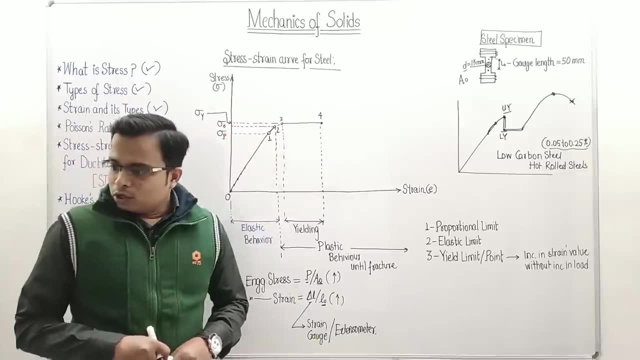 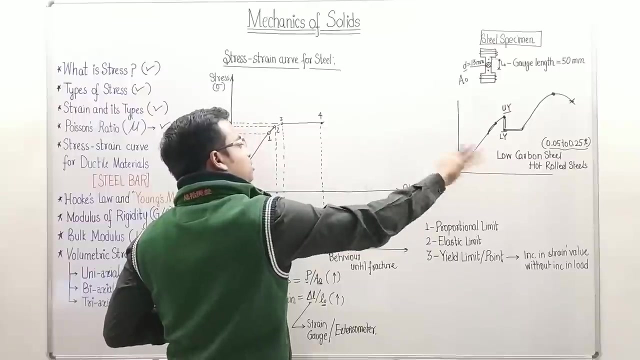 of yielding, where we see an appreciable increase in strain without any increase in the load. what happens next? let's see. So here we go. let me go further. let us increase the valve further. okay, let us open the valve further. if you open the valve in the universal testing machine, what will happen? something like this will. 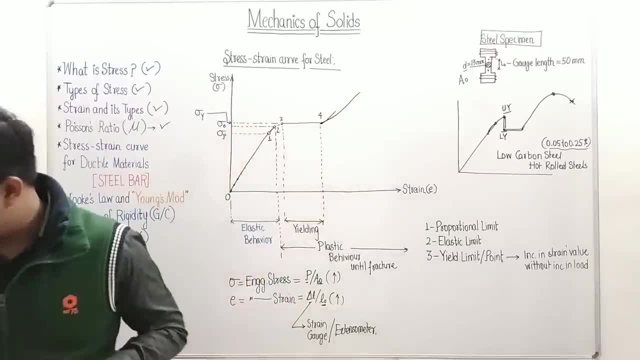 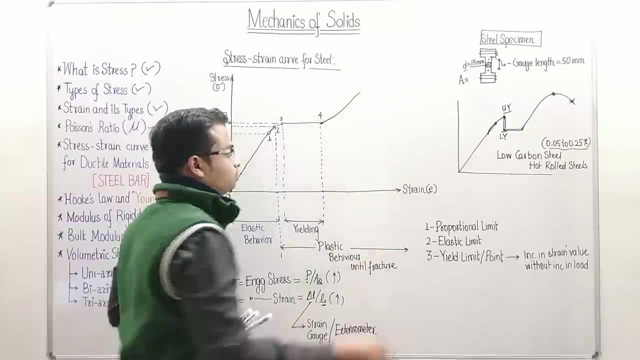 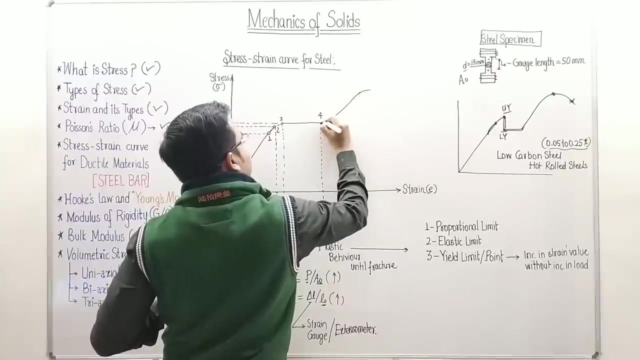 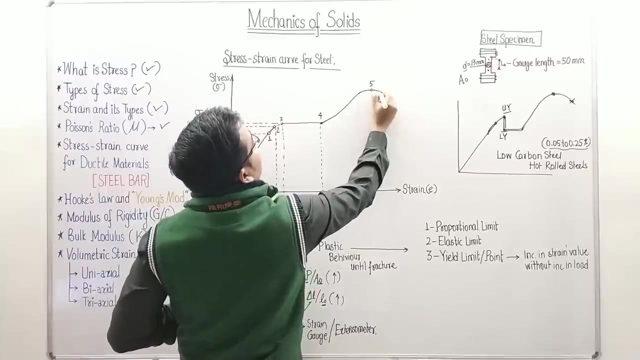 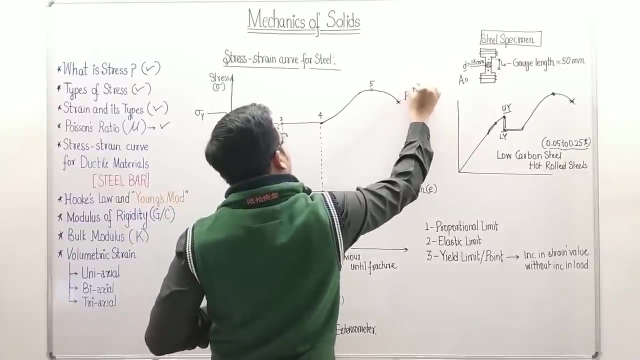 happen. okay, it is the duster. here we go and we'll get a point over here like this: it will absolutely. first there is going to be rise in the curve As you keep on grazing the load by opening the valve, and then it will try to flatten out. okay, then there is a point, point five. I'll let you know what that point is right, and then after that here there is failure or mechanical engineering terms. let me just write it as fracture. 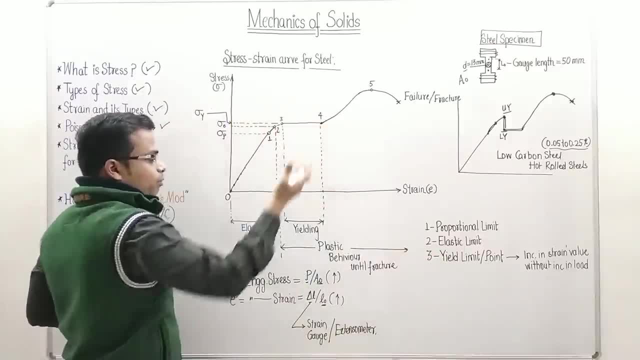 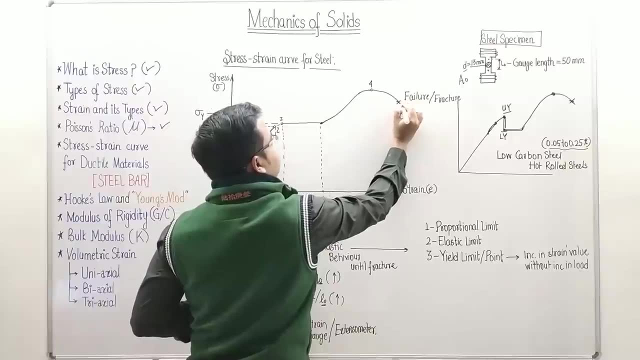 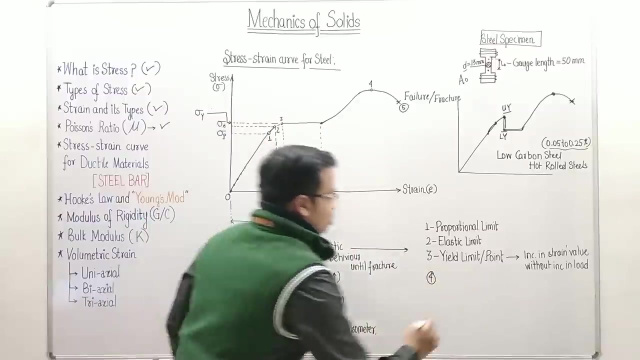 So you can clearly see point three and four are along the same line. so that is the yield point, Obviously, after which you can. you can see that this should be named as point four. let's say this is point five. okay, where the material actually breaks or fakes. point number four: this corresponds to the ultimate stress. 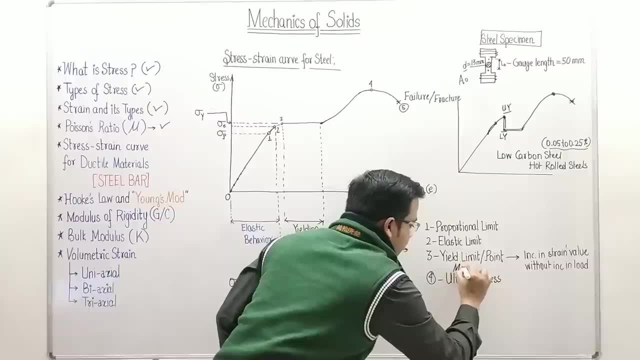 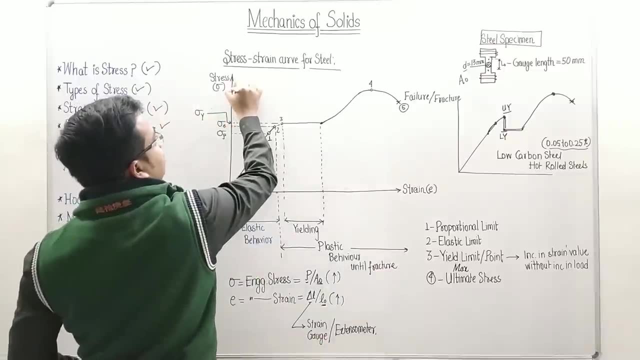 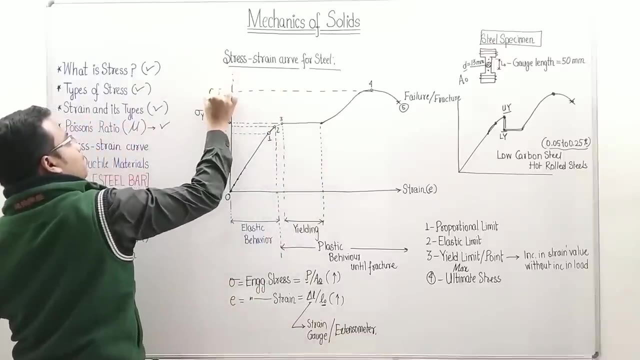 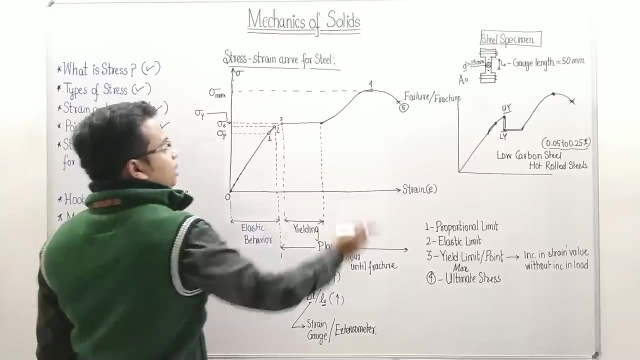 Or you can also say that this is going to be the maximum stress that this specimen will be undergoing. that is the maximum value of stress- and let me just write it over here- corresponding to the maximum stress of this specimen, to this 0.4.. This over here is going to be sigma max. Let us extend this sigma And, if you go, 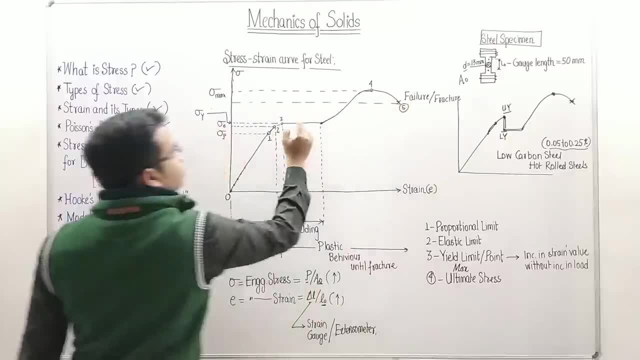 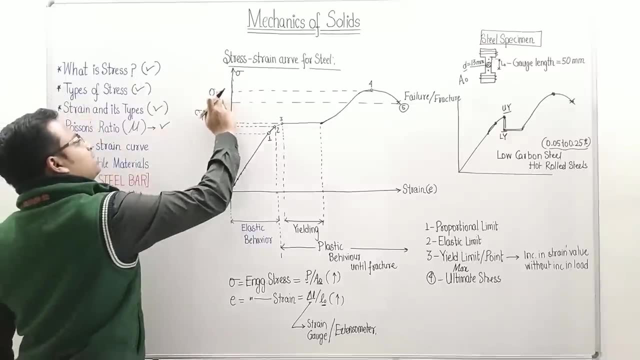 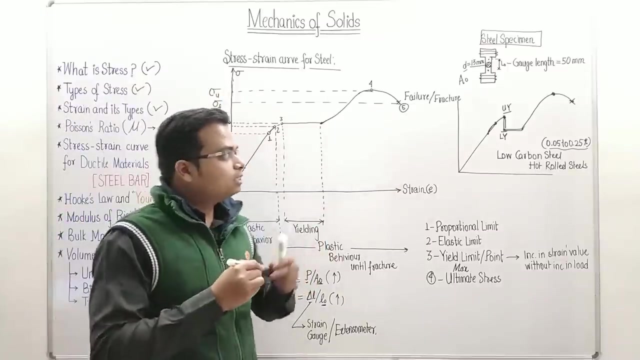 further. what will happen? At 0.5, this specimen will fracture. So sigma f, Some people actually write it as sigma max and you can also write it as sigma u. This is the ultimate stress And if you go beyond that, well obviously the specimen would fail. What is happening here? 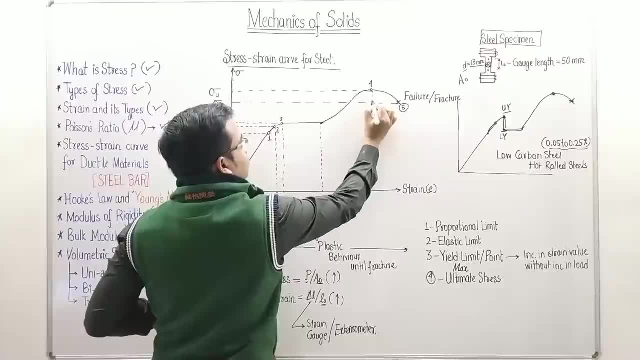 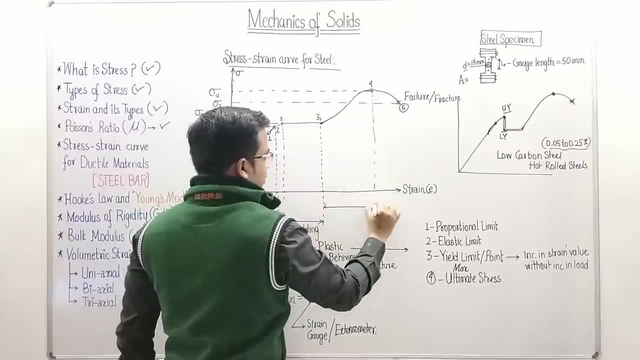 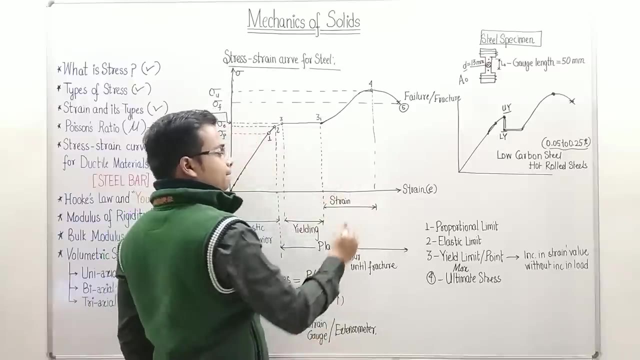 Actually, during this phase, during the phase, let us call this as 3.1.. Okay, This is the phase of strain hardening. Obviously, there is going to be permanent deformation or plasticity, But this process is during this region. we call this as strain hardening. And 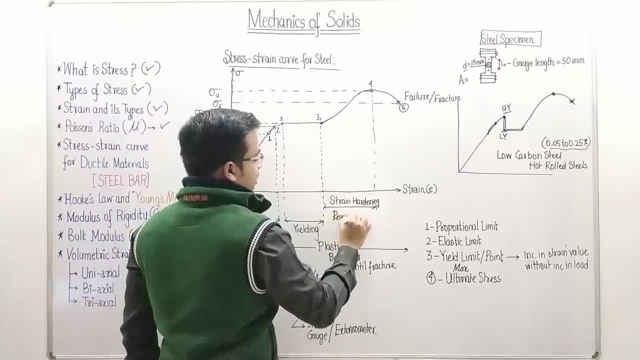 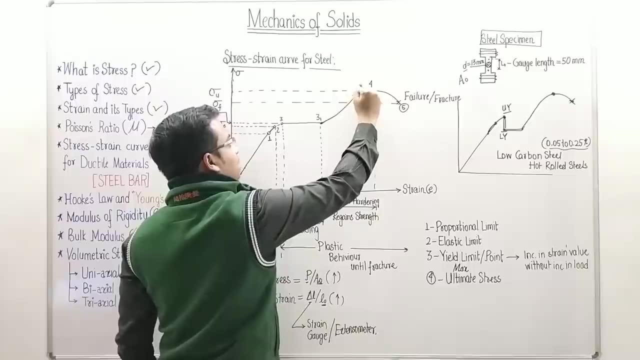 this is where the material regains its strength. Okay, And that is why it is known as strain hardening- Regains its strength. So initially there is a rise in curve and then it flattens out. Okay, And at 0.4,. 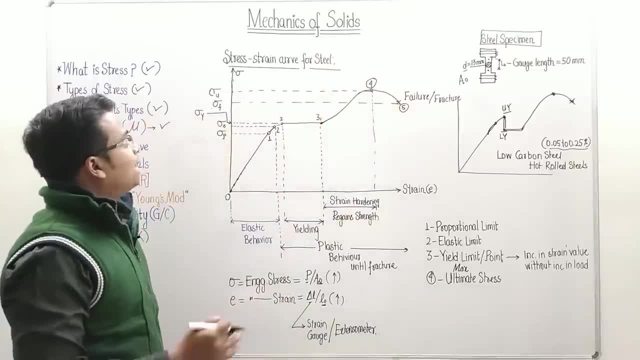 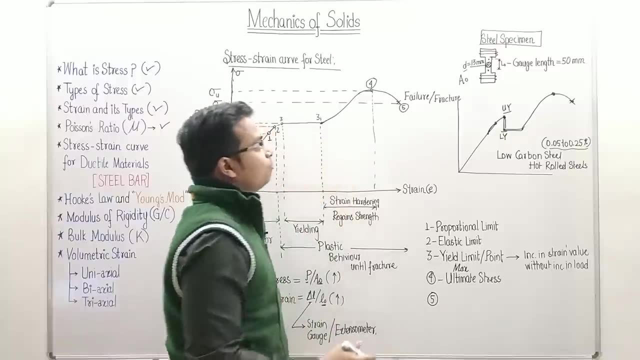 the value of stress reaches its pinnacle. Okay, That is going to be absolutely maximum. And then at 0.5,, at 0.5,. if you go on further increasing the load, then there is going to be a fracture. So 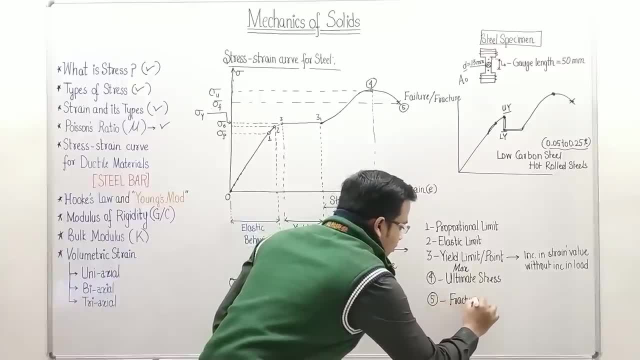 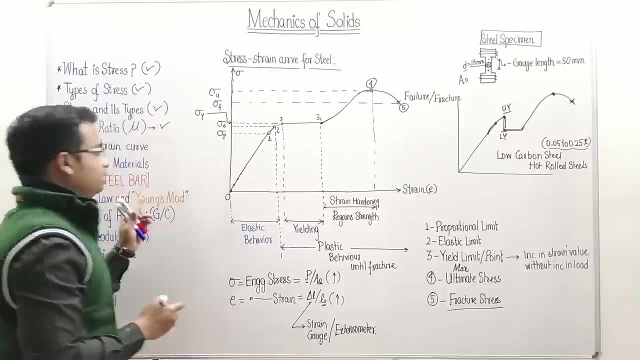 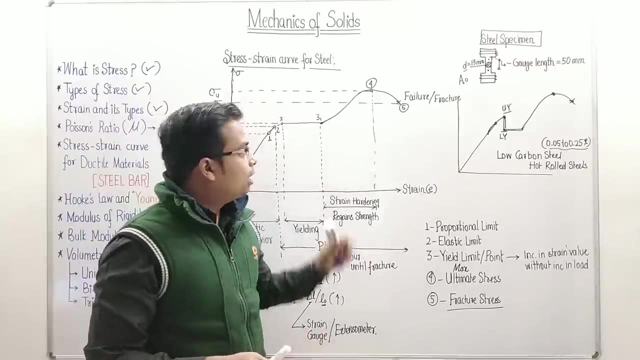 0.5 corresponds to fracture. Fracture stress or failure stress, whatever you may call it. So this is basically the stress strain curve for a steel bar, for a medium carbon steel, let us say, And that is the stress strain curve for a low carbon steel, And you will see these: 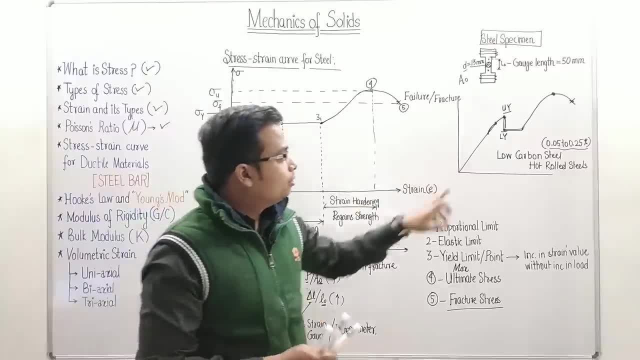 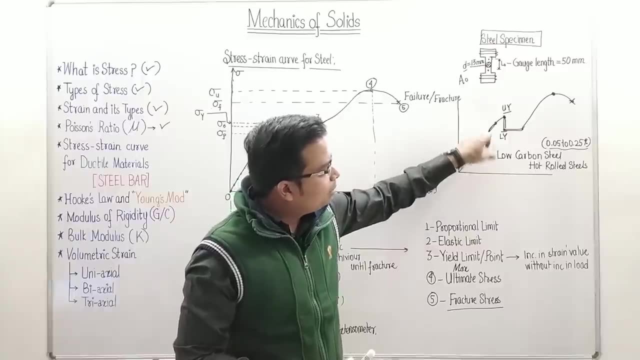 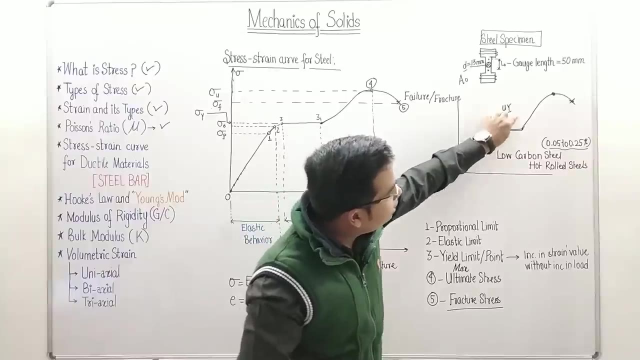 two diagrams in different, different books. Okay, Nothing, no load. Elastic limit: No, not the elastic limit, but the proportional limit Here. proportional, this is the proportional limit, This is the elastic limit. This is upper yield point, lower yield point And then this over here is the point where the maximum stress is induced. 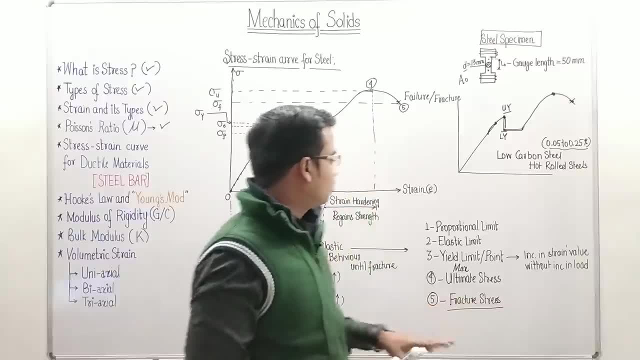 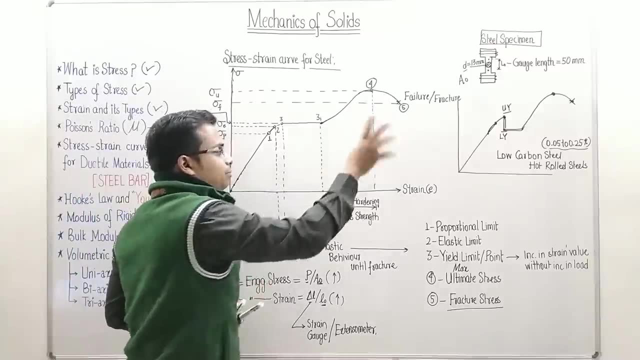 And this is where the material or the specimen fractures. Okay, So this, these were all the points. Now, some of you guys might be wondering why there is a dip. Let me just show you. First of all, let me. 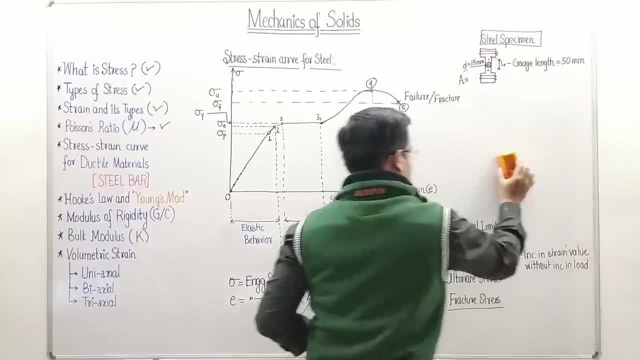 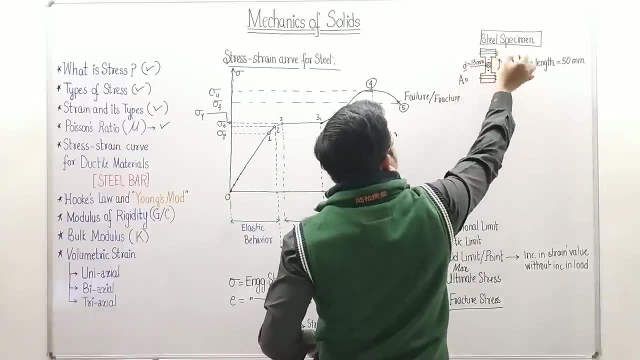 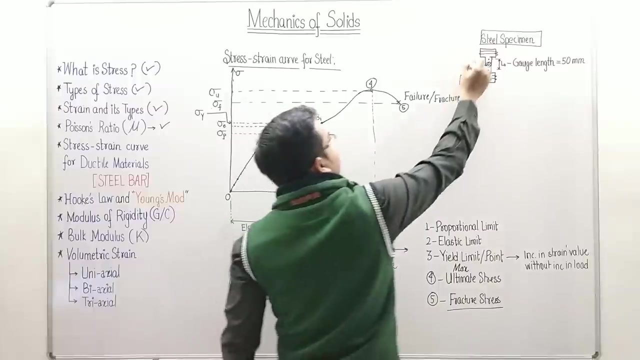 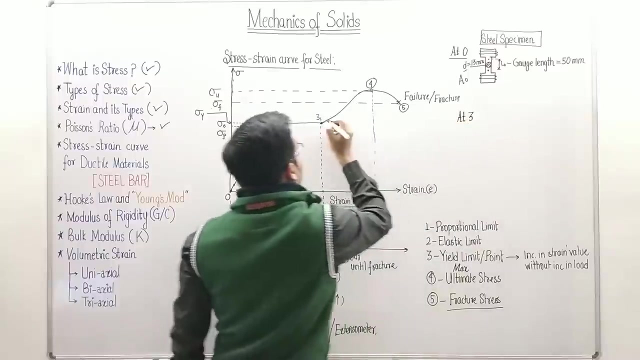 okay, Okay. So just watch this carefully. Take a look at this. Let me just make a timeline. timeline of this steel specimen. Now, what will happen At at 3, 1.. Okay, This right here. at the starting, we are at 0. So when we reach at 3, what? 3, 1.? What will happen? 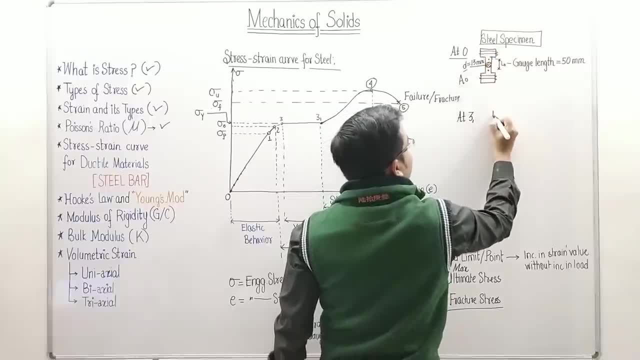 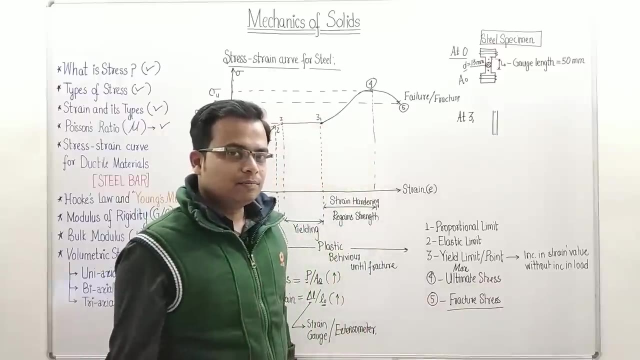 Obviously the distance between these two points would have increased, isn't it? Just try to make only this portion. A distance between these two points would have increased by a certain amount And this area would have decreased, isn't it? The cross section area would have decreased, But again, we are doing it. 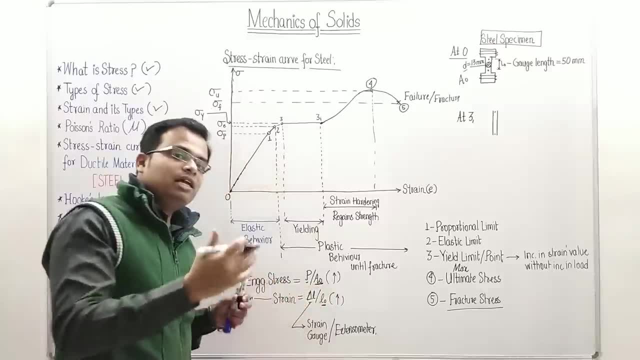 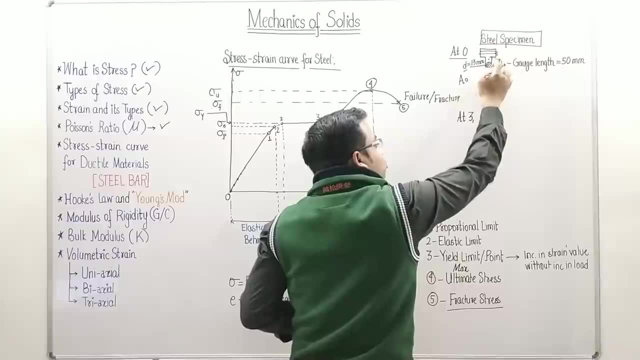 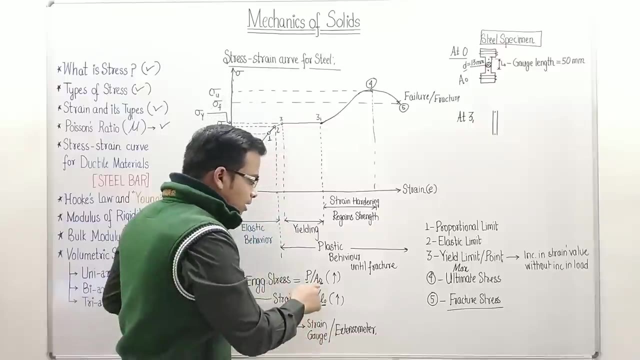 very theoretically, we are always going to follow the original area and not the dynamic area or the instantaneous area. The area across the entire length between these two dots, across the entire length has been reduced. We are assuming a uniform decrease in area Right, But still we are using A0, that is, the original area of cross section into consideration. 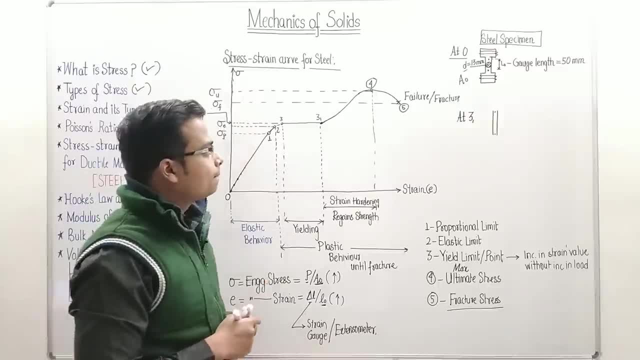 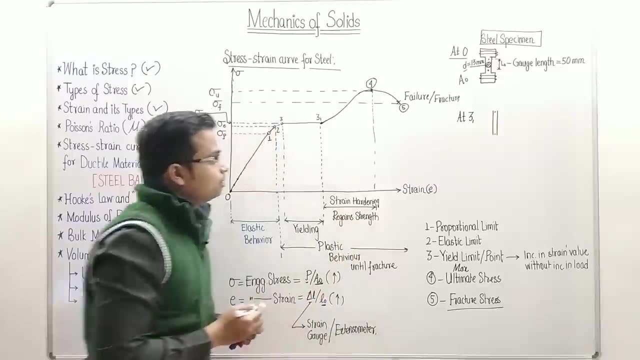 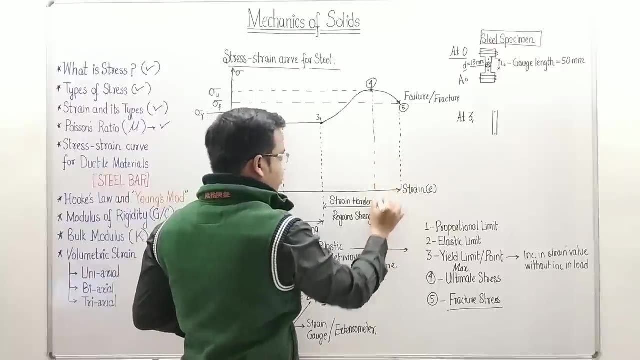 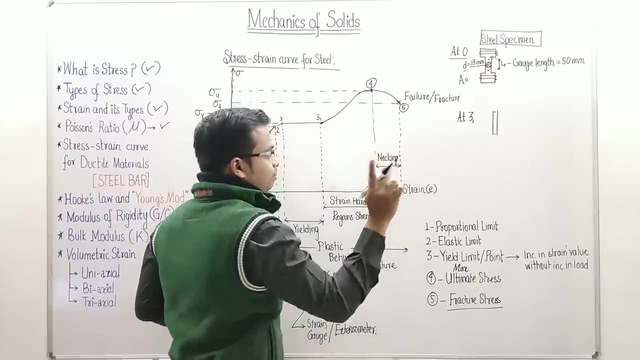 for getting the value of stress. Okay, Now what will happen here? What really happens is between point 4 and 5, this region, this region- where should I write this? In this region, neck begins to form. What is this neck? Let me just show you. 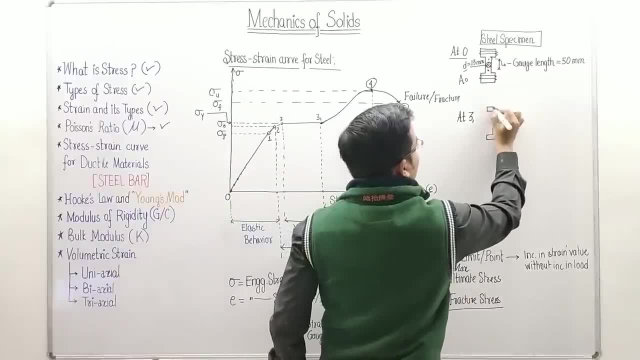 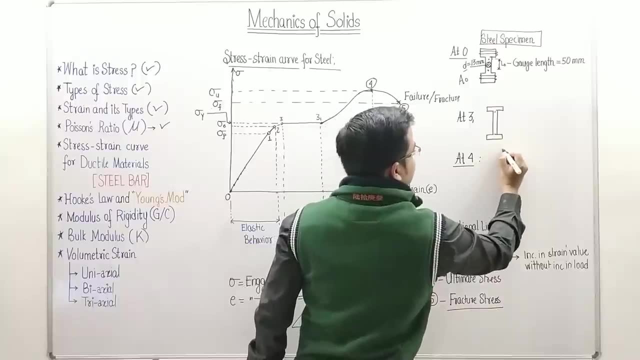 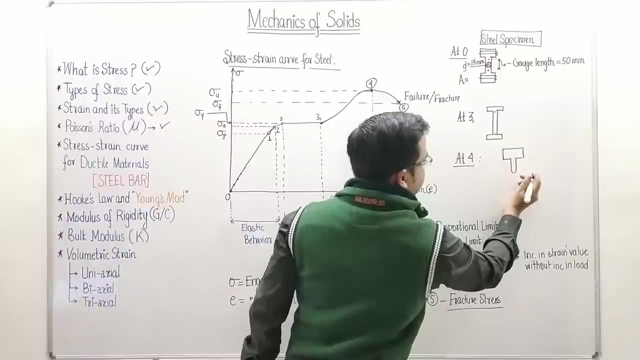 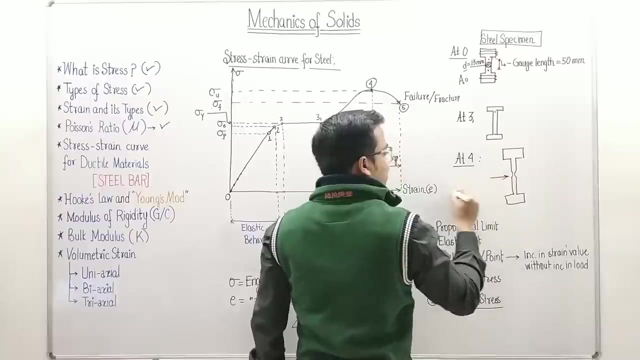 So what really happens is okay, let me just draw this roughly at 4.. At 4, what happens? Just watch: This is being fixed to the upper jaw And something like this happens. You see this cross section area getting narrower, isn't it? And what will I write over here is necking begins. 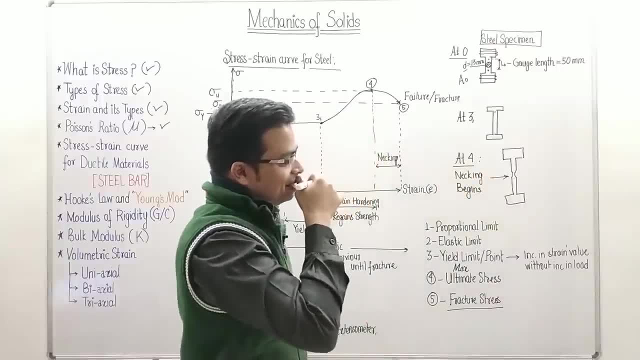 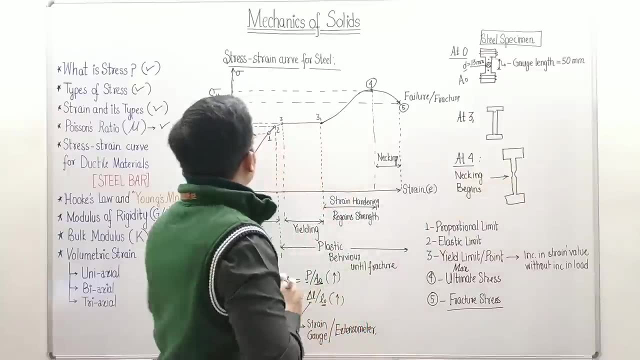 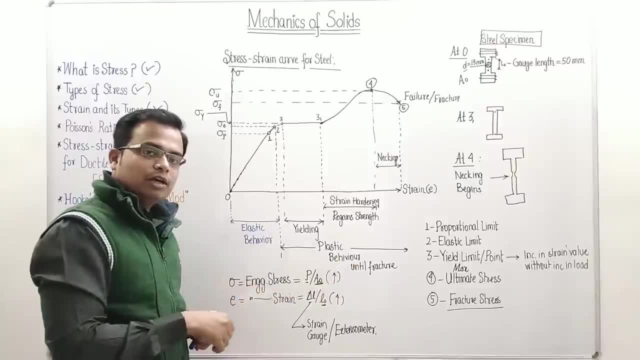 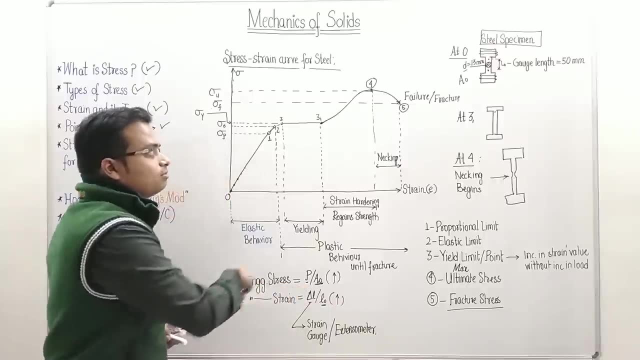 to have lower value of stress. what will you do? You will close the wall. If you close the wall, what will happen? The load is going to decrease. If the load is going to decrease, then the stress will also decrease. That is why you get a dip like this: Okay, But in reality, in reality. 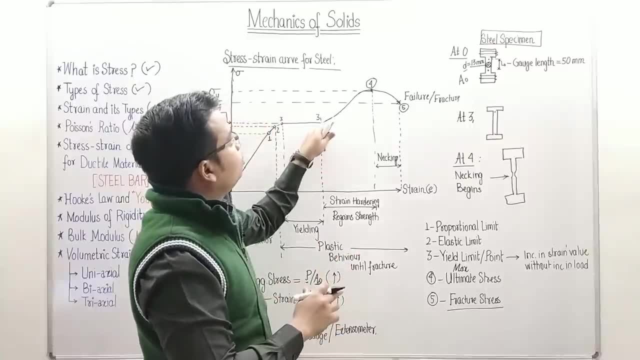 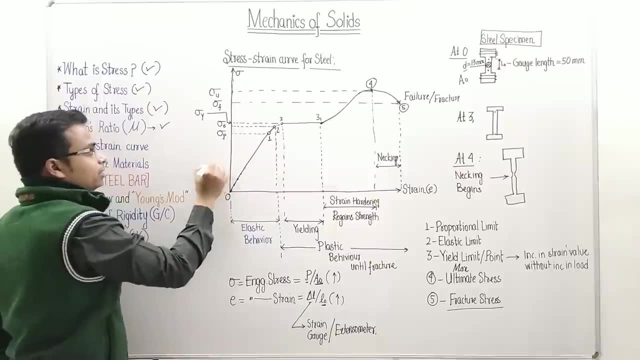 that does not happen And I'm going to explain to you how these two stress will happen. Don't worry, everything will fall in place. This is the conventional stress strain diagram. Let me write it over here. This is the conventional stress strain diagram. There is one more diagram. 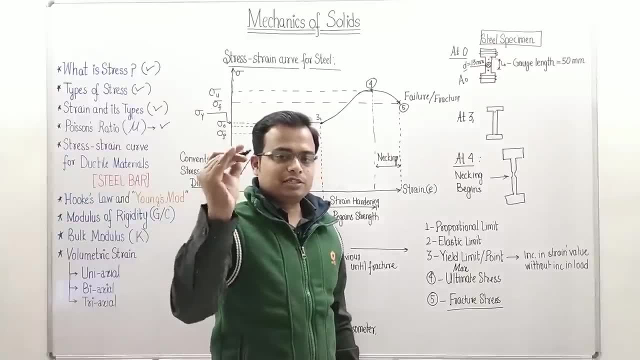 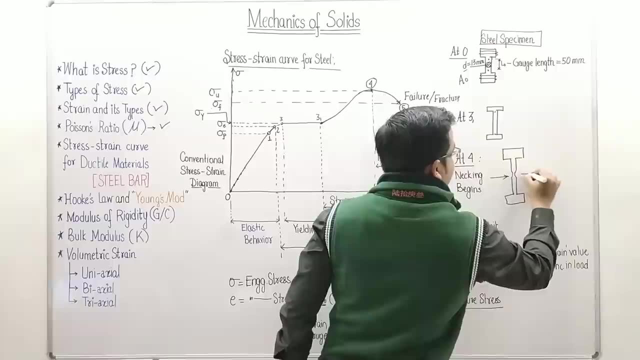 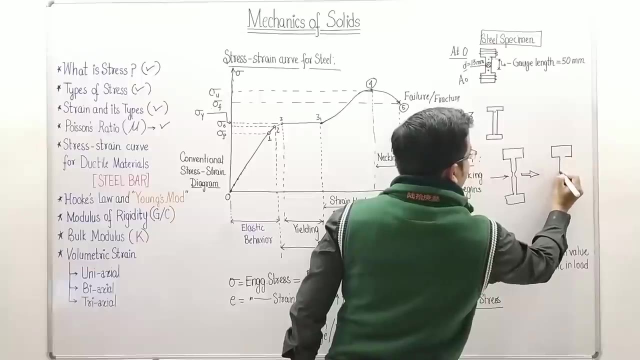 or one more curve, which is known as the true stress strain curve. Okay, we will see that also. don't worry Now when necking forms, okay, something which the material eventually fails and the failure is absolutely a cup and cone failure like this. Let me just show you: This is the cone and this over here is the cup. 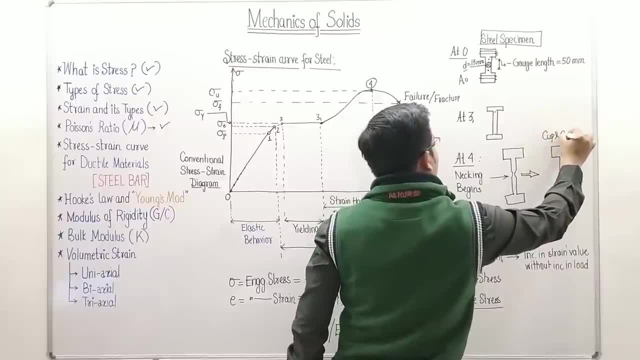 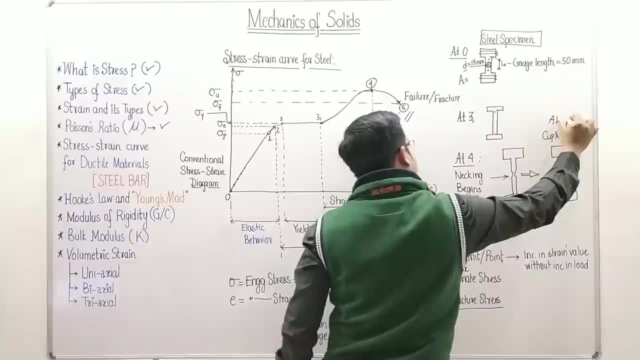 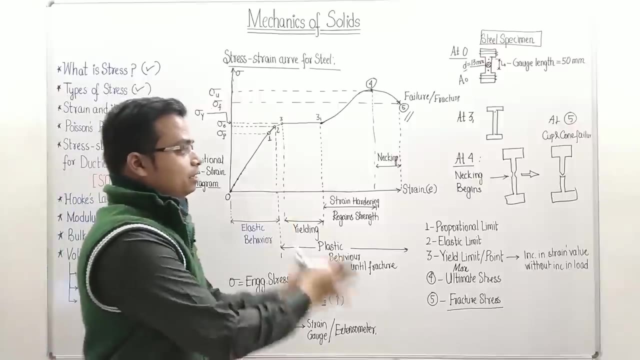 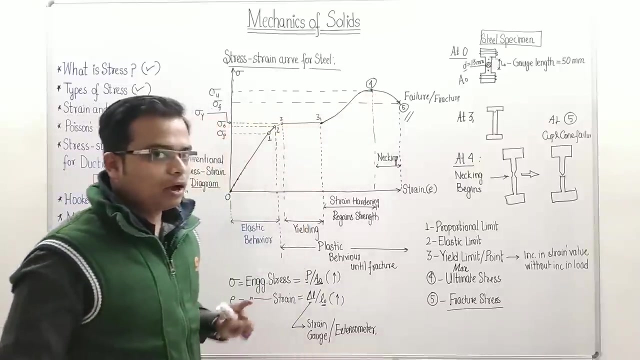 So this is finally cup and cone failure where, at point F, when you reach the fracture stress, cup and cone failure happens, especially in case of a tension test. Okay, this is conventional stress strain diagram. Now, had this been a low carbon steel, you would have got two yield points. 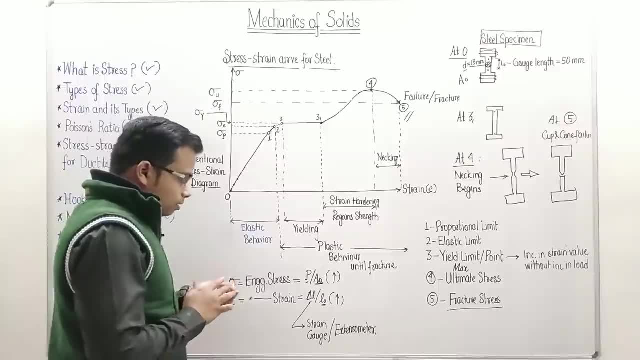 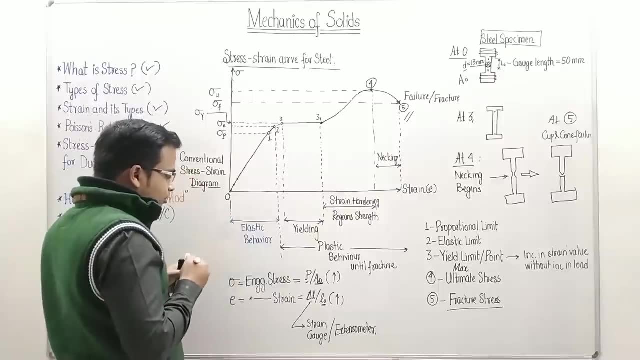 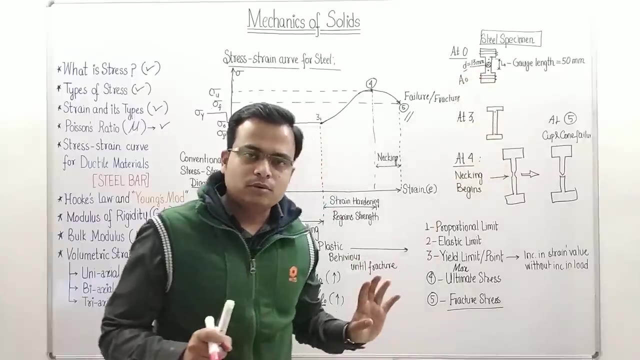 upper and a lower yield point. Okay, now let me choose a red color Again. one thing that we need to realize is this cross section will always decrease. That is quite true, But do we take the reducing cross section or the reduced or instantaneous? 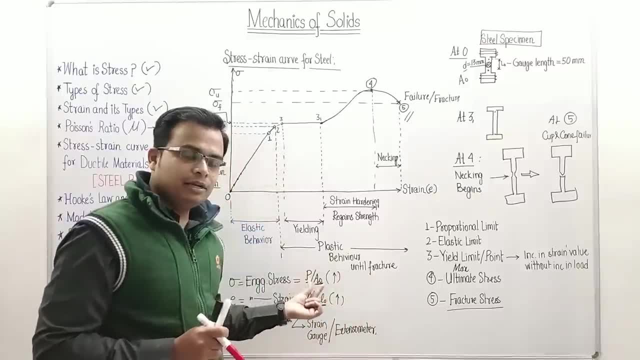 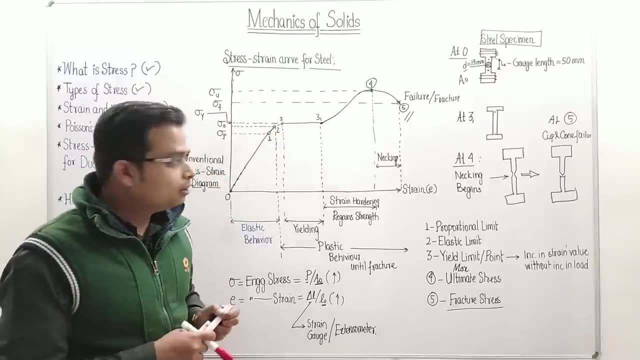 cross section? No, we don't. We always take the original cross section into consideration And based on that we have got these values and we have made a plot. But in reality that does not happen. And when you take the instantaneous cross section into consideration, you will pretty much 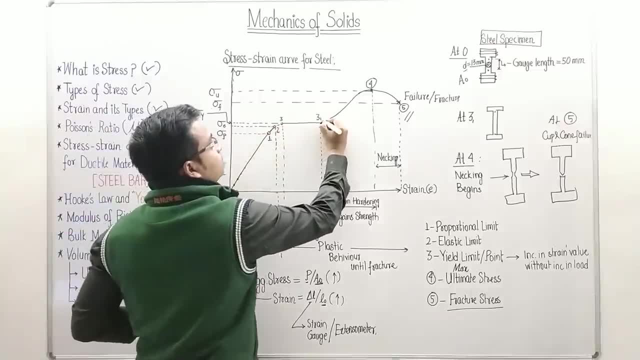 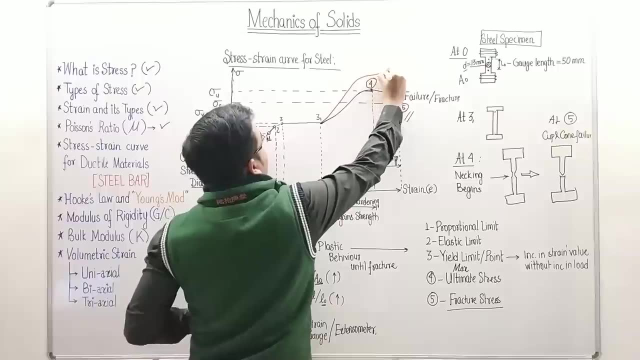 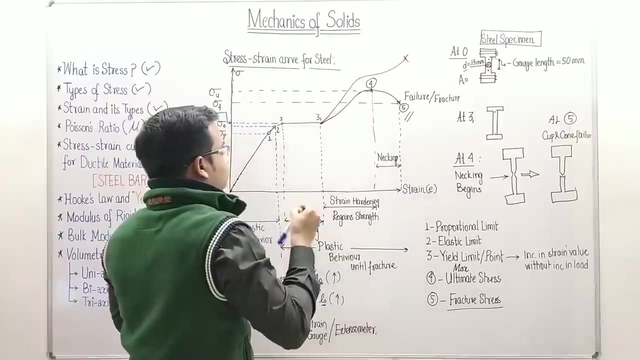 have the same curve until you reach here, But after this, 3,, 1,, 3, subscript 1, well, things are like this: Okay, and here the fracture is going to take place here. So, guys, this there is not. 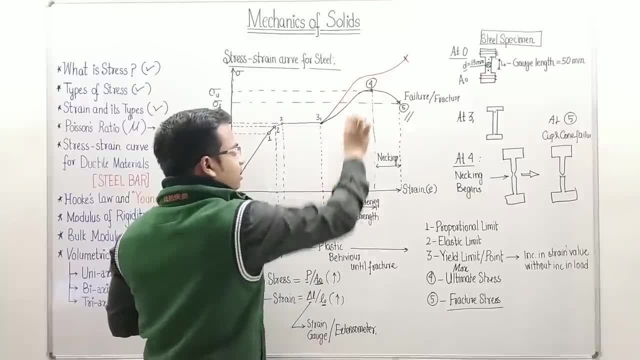 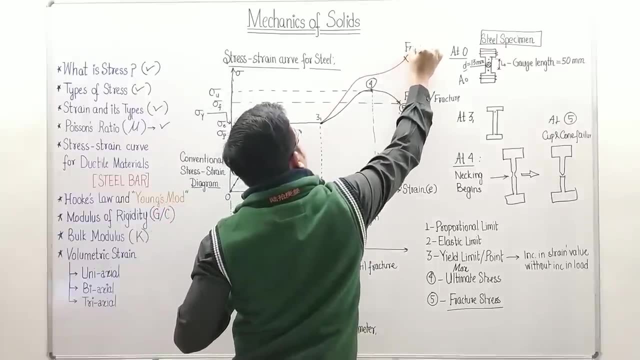 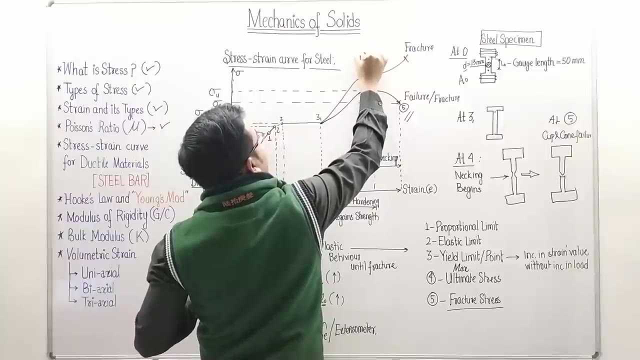 much of a difference between 3, 1,, 2, 4.. Okay, in the region of strain hardness, although there is a difference, but the difference isn't that much magnitude wise, this is going to be the fracture And this curve over. here is what we're going to represent. the true 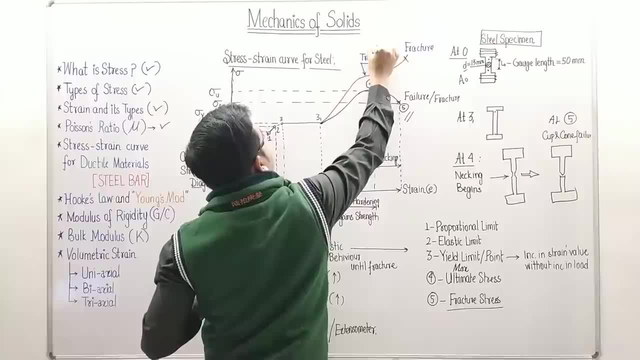 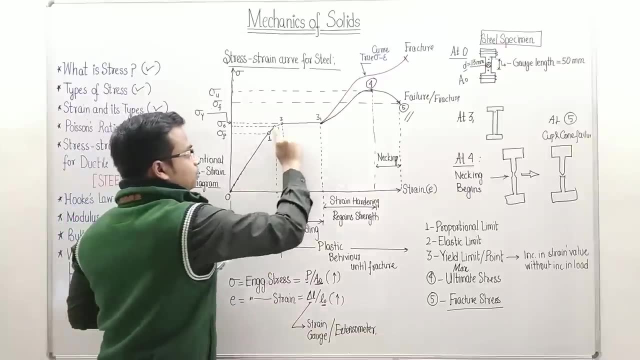 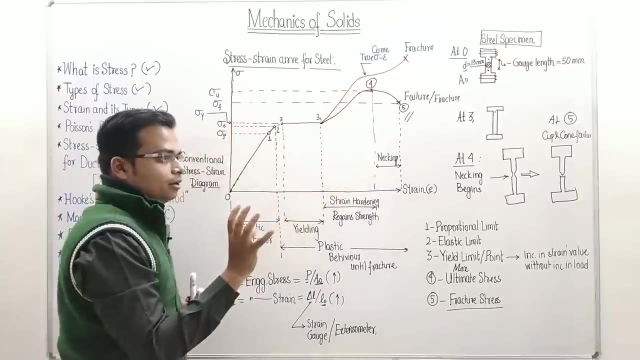 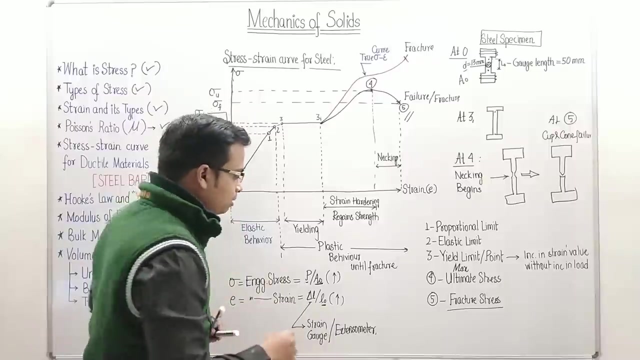 stress Strain curve or true stress strain diagram. So let me just treat it. This is the conventional stress strain diagram And this is the true stress strain diagram, where we keep on putting in the instantaneous cross section or the reduced cross section. Just think about this After this point. 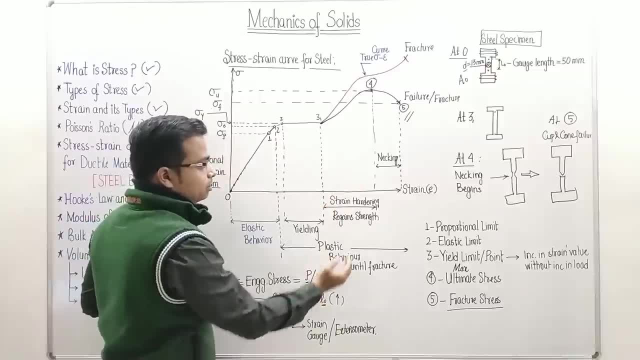 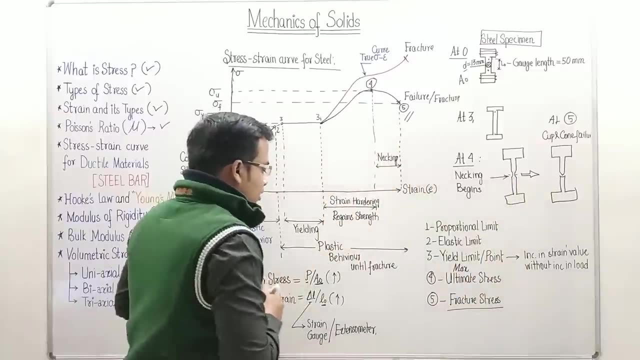 let's say, after this point, after point 4, when necking actually happens, when necking happens here, somewhere, here, what will happen? The area will keep on decreasing. So if you keep the decreased value in the denominator, if you decrease the value, what will happen? The stress value is: 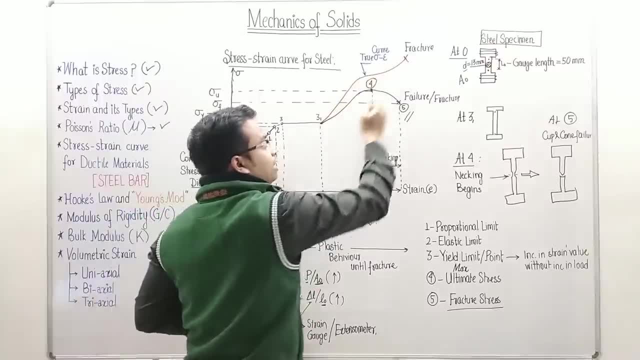 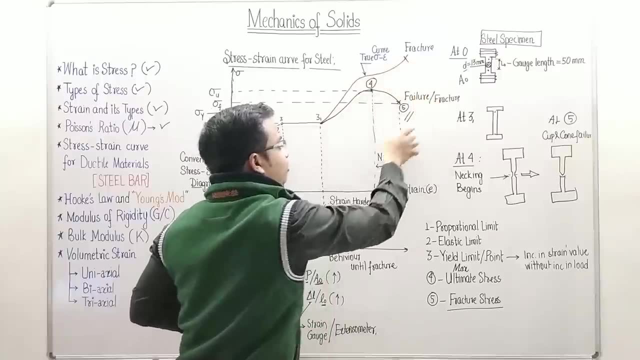 going to increase. That is why you see an increase over here. And finally, the material: the fracture stress, in case of a true stress strain curve, is going to be far greater than the fracture stress which is obtained in a conventional stress strain diagram. So this was the entire idea. 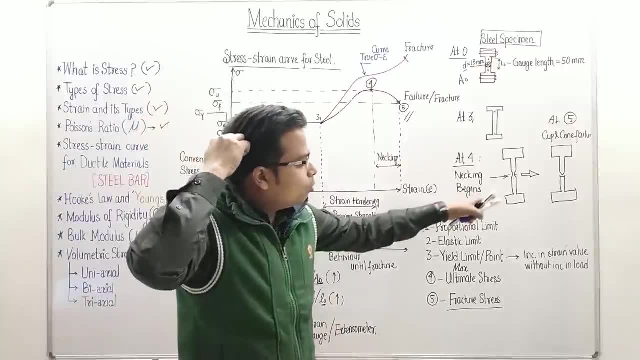 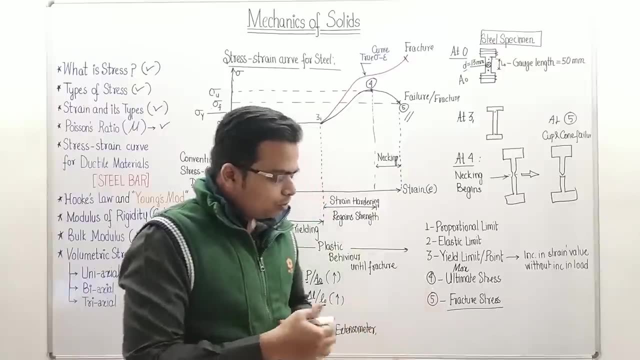 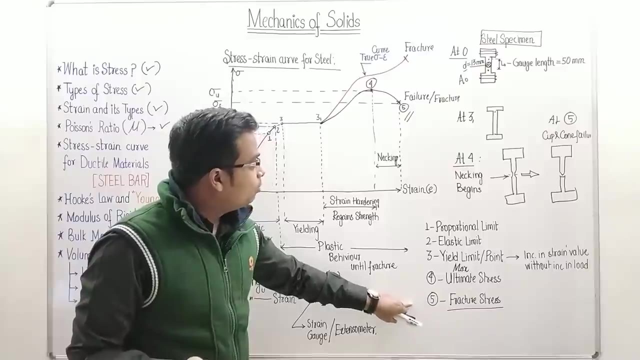 Now some of guys, some of you guys, might be wondering: why does a failure happen? why does a failure happen and what is the entire mechanics behind a failure? So just try to understand this. Where can I write this? there is absolutely no space. Okay, I am pretty much sure. 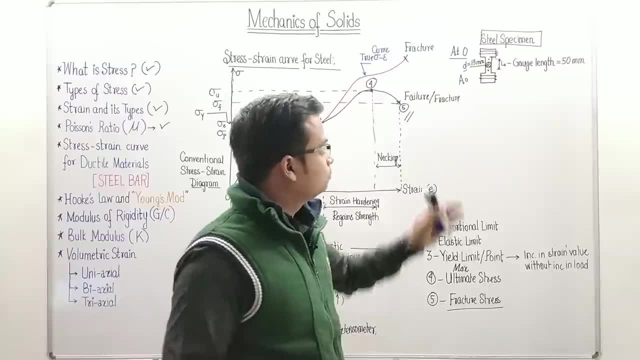 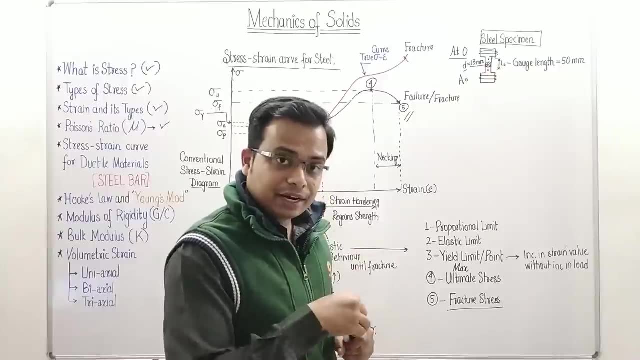 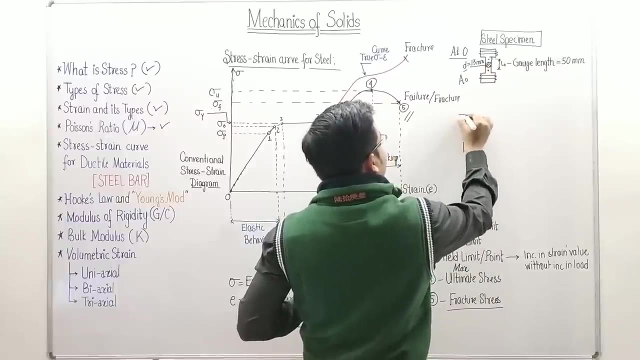 that you guys must have written down all these things. No material is absolutely perfect. No specimen is absolutely perfect. There are always imperfections, And imperfections actually aggravate. Let me just show you So, So, So. Okay, This was the mild steel specimen, isn't it? 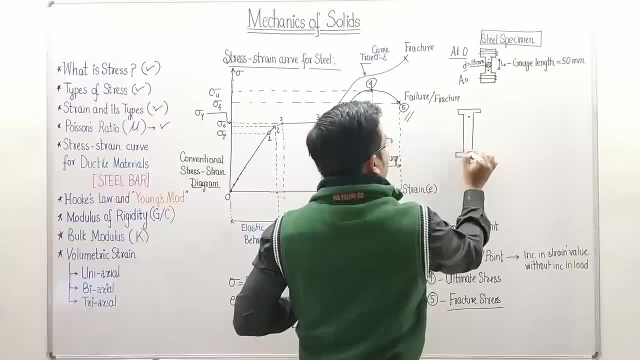 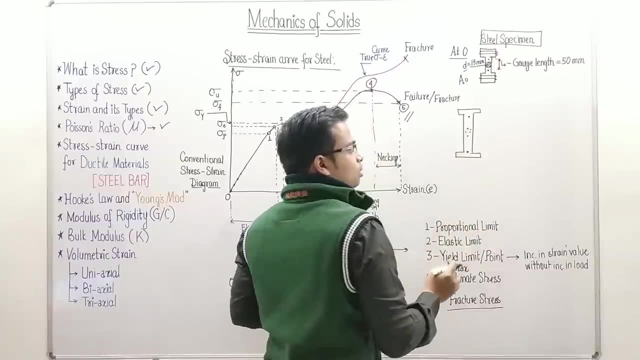 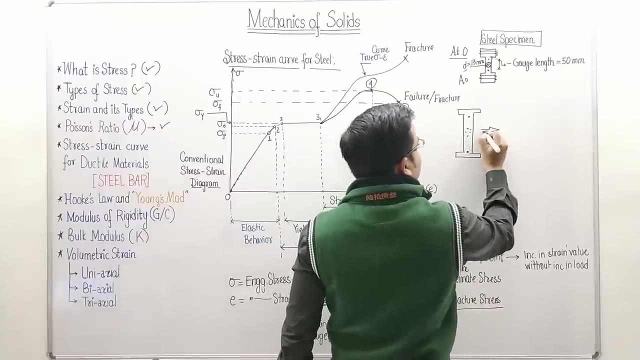 So what happens? These were the two dots which we had actually punched. There are voids, very small voids, Okay. So what happens? You are pulling it, You are doing a tension test. So in that case, these voids get together, get closer. 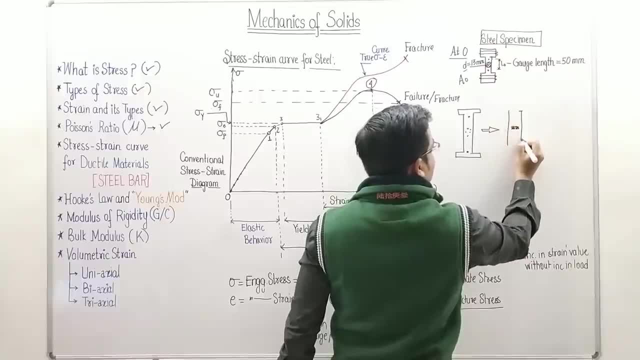 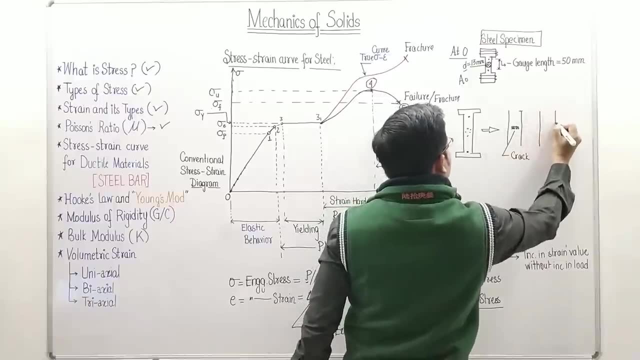 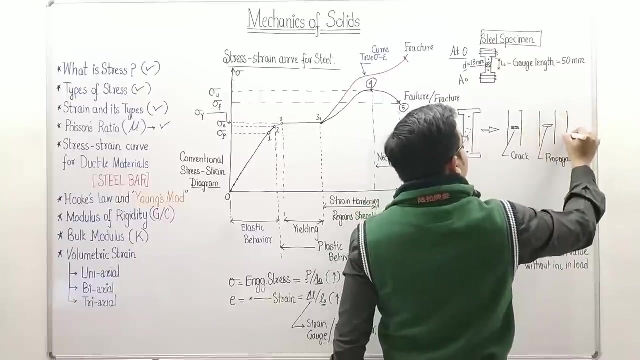 And they coalesce, they combine, They actually combine and actually form a crack. And if you further increase the load, what will happen? This crack will actually propagate, Will actually propagate, Okay, Propagate, And it will propagate to such an extent that it will cover the entire cross-section area. 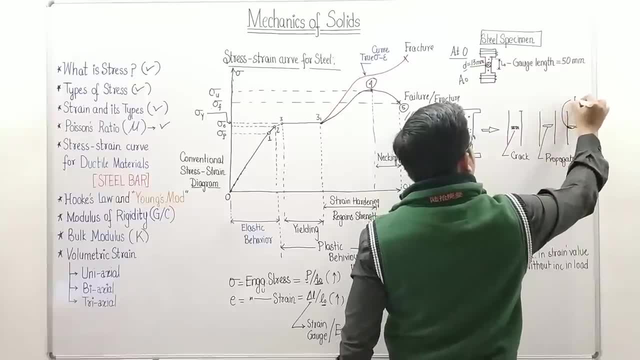 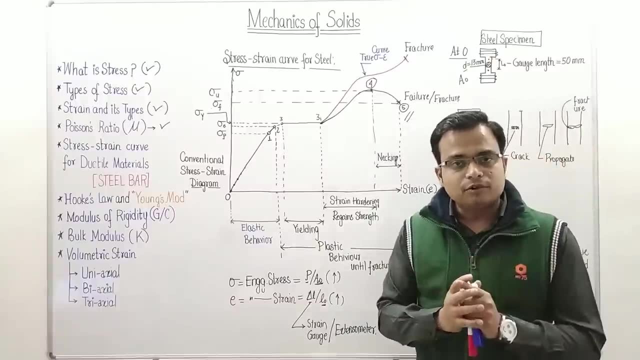 And when it covers the entire cross-section area, what happens? You know what happens: Fracture. So, guys, that was all About the stress-strain curve for a steel specimen. This was the conventional diagram And this one was the true stress-strain diagram. 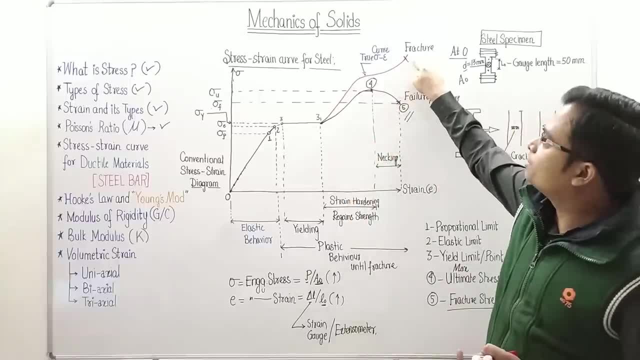 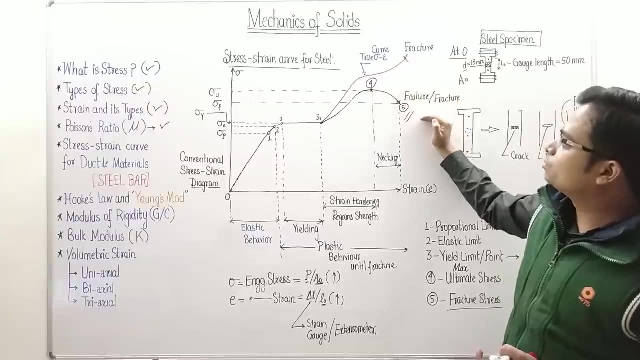 And the fracture stress- remember- this can be asked as a question- Fracture stress achieved in case of a true stress-strain curve is going to be more or far greater than the one which we have achieved in case of the conventional stress-strain diagram? 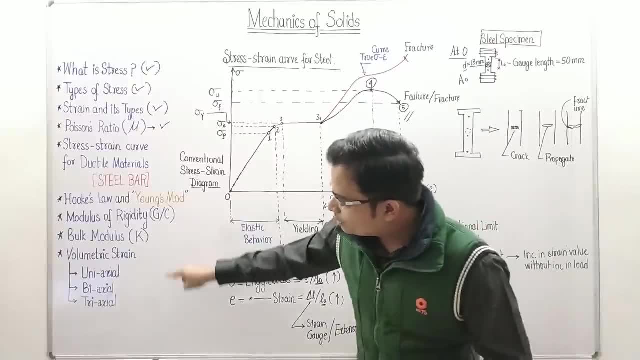 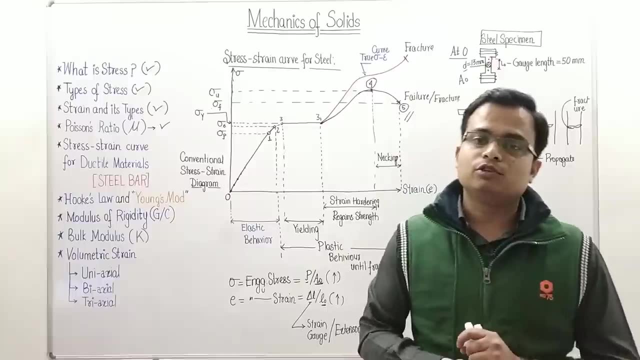 That's for sure. So, guys, that was all for today. The remaining topics I am going to be covering up in part B of simple stress and strain. So you have got to join me again. I am going to be uploading that video also very soon. 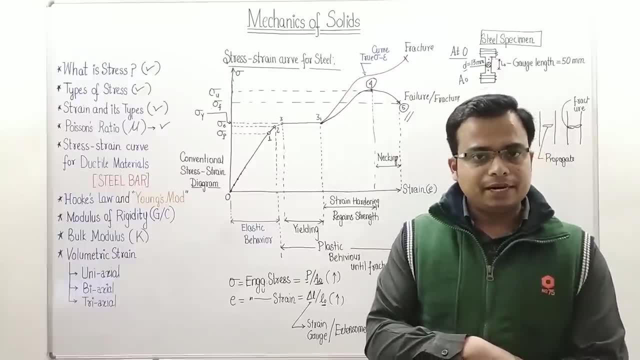 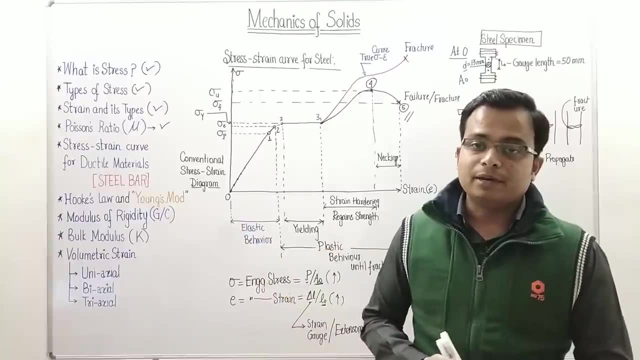 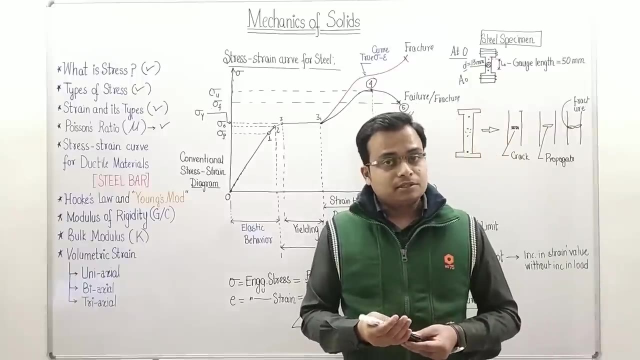 That is going to be more in the mathematical sense, Right, And there are even some more topics. I have absolutely no space to write it down, So don't worry, All the things will be covered up And once this simple stress and strain we get over with, we will start off with thermal stresses.